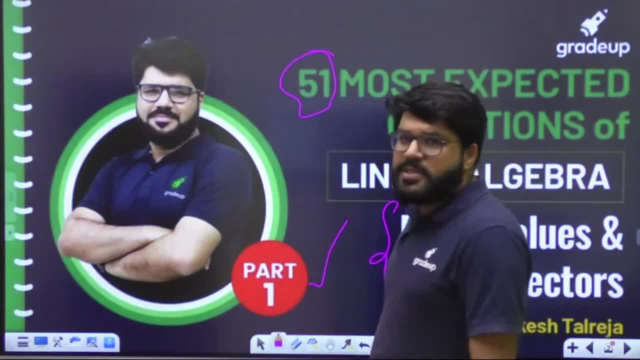 day, you can say most important of the linear algebra. Many of the questions can be expected: Little, good questions, tricky questions that can be expected from this particular topic. Right right, Very, very good evening. Keep joining the session and keep sharing, guys. 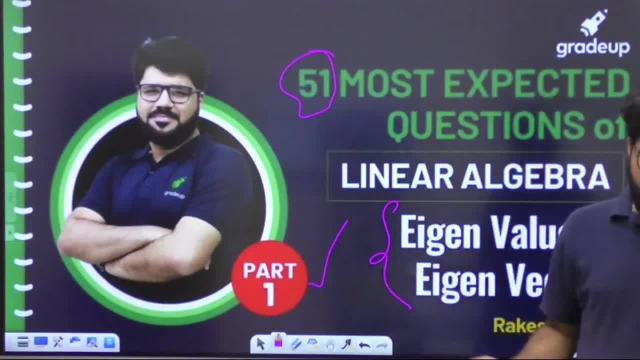 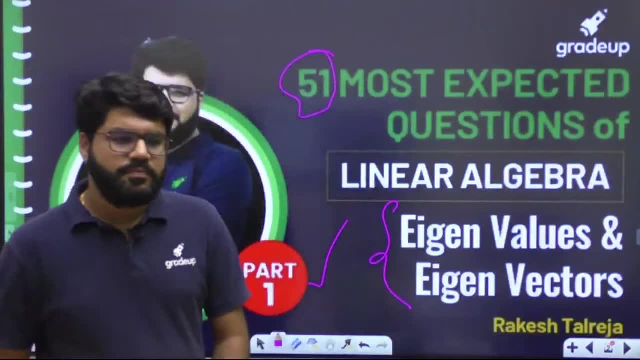 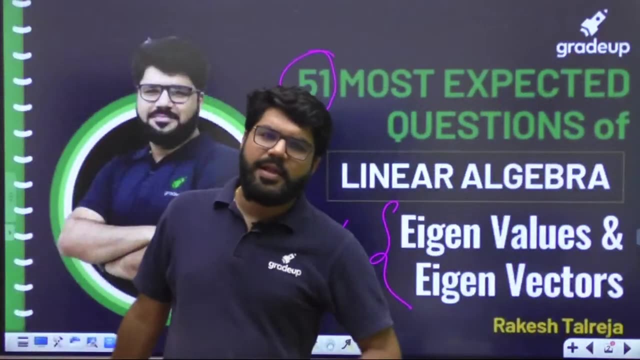 How's the josh at 11.17 pm at the night? Yes, very, very good evening. Very, very good evening. Keep joining. Yes, So with respect to the linear algebra, other than the eigenvalue eigenvector, we have 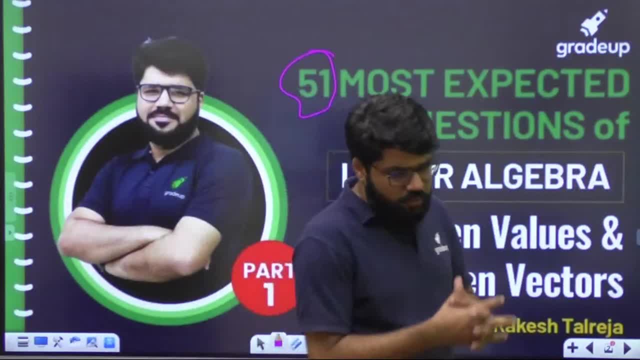 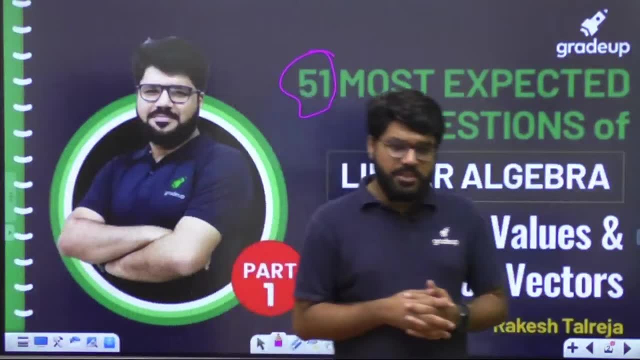 completed. we have taken the most expected questions of rank: non-homogeneous system of equations. homogeneous system of equations. And I have one more, one more event to be disclosed to you. Okay, one more event that we are going to conduct with respect to linear. 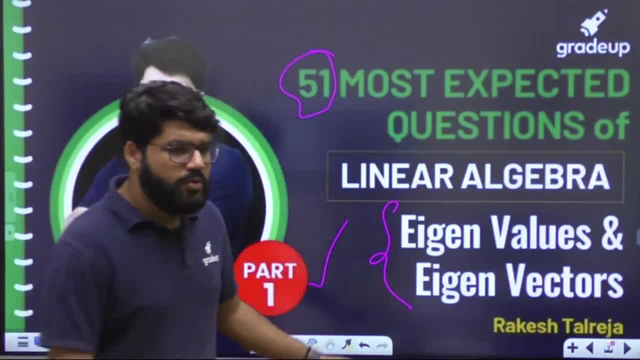 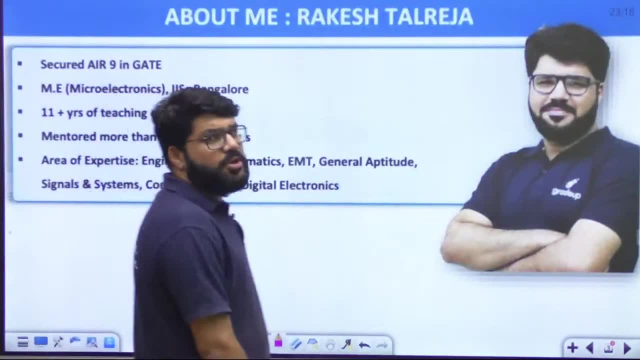 algebra. Okay, that will be beneficial for you. So, very good evening all. Keep joining, keep joining. Come on, guys. Little slow, The crowd is little slow today, Is it so, guys, The crowd is little slow. I want to see the. 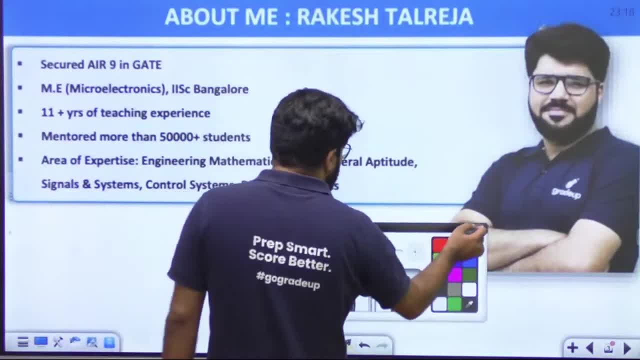 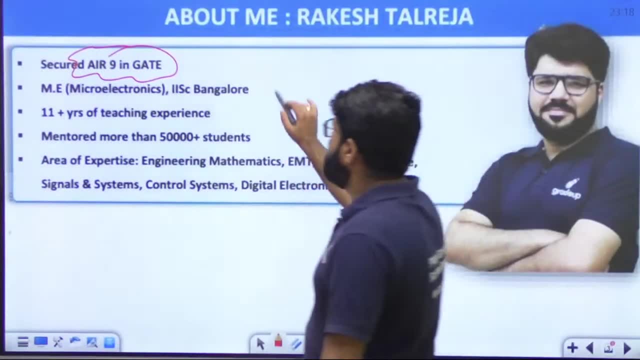 high josh. So this is a brief intro about your mentor and educator, Rakesh. If you are joining me for the first time, brief intro about me. I have secured all India rank 9th in the GATE examination and completed my masters from the Indian Institute of Science, Bengaluru. 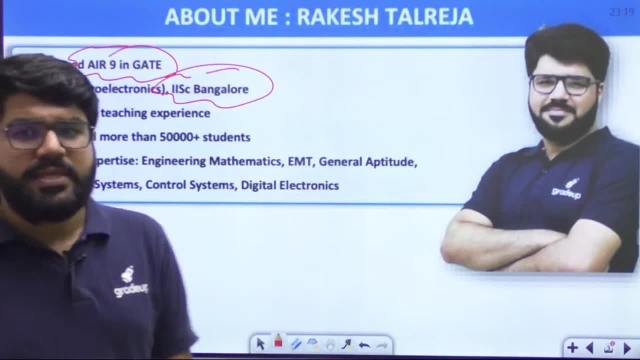 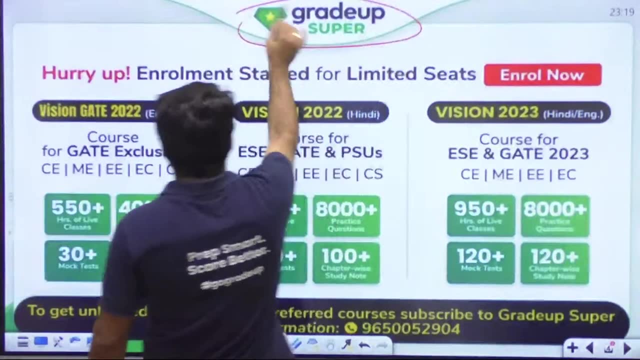 More than 11 years of teaching experience for ESC, GATE and various technical based examinations. Yes, So grid up, Superb, So Vision GATE 22,- exclusive course for GATE. Vision 22,- a comprehensive course for ESC GATE. 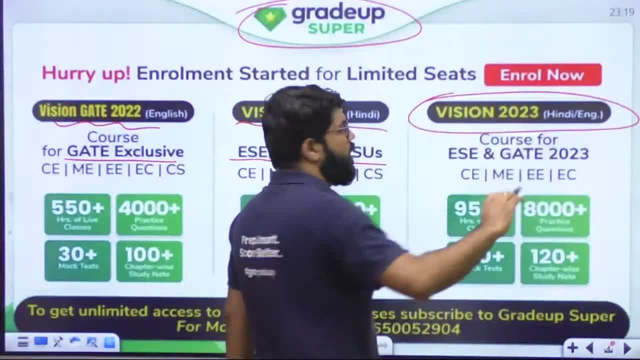 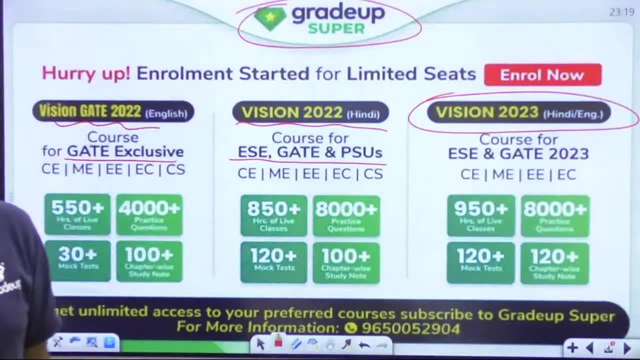 PSUs and the Vision 23.. Vision 23, a full-fledged long-term course for the ESC, GATE and PSU 2023 examination Right. Yes, yes, yes. Very much important for CSC GATE as well, Chandan. 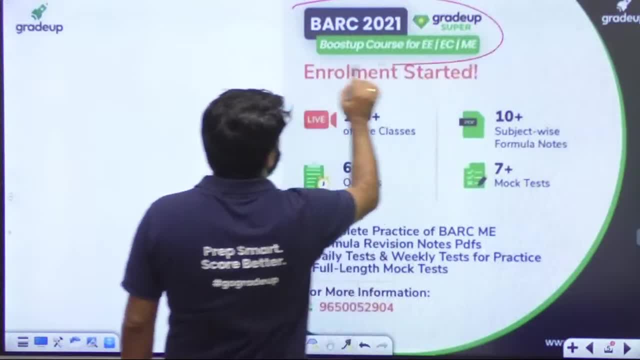 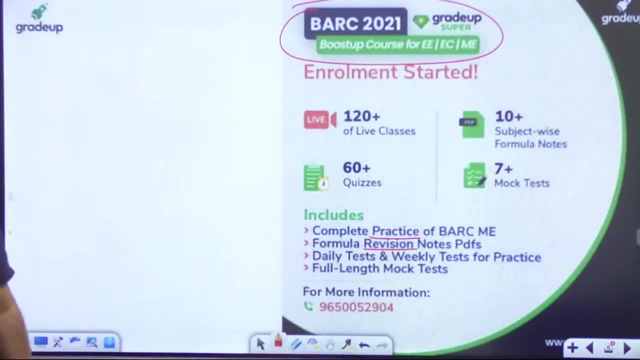 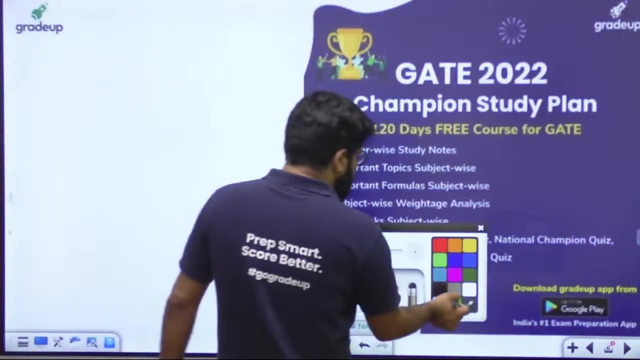 Okay, So boost up BARC course. As you know, the BARC online technical examination is on the September, coming shortly, And we have the complete practice And revision module available on the grid of super for electrical, electronics and mechanical and the GATE 22 champion study plan. The GATE 22 champion study plan: 120 days free crash. 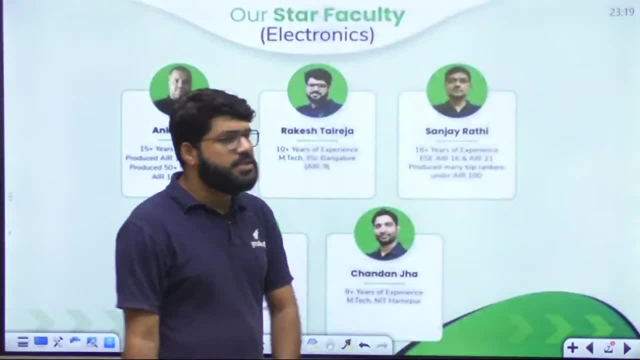 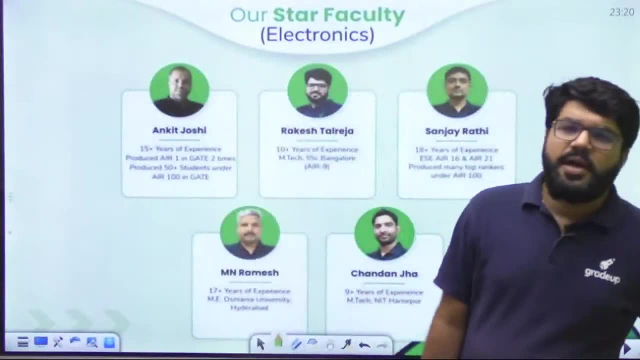 course, also available with the grid up app and the grid of YouTube channels. This is the star. This is the star faculty team of electronics and communication engineering space. The vector, space and base is important And in the syllabus of only electronic Shiva. 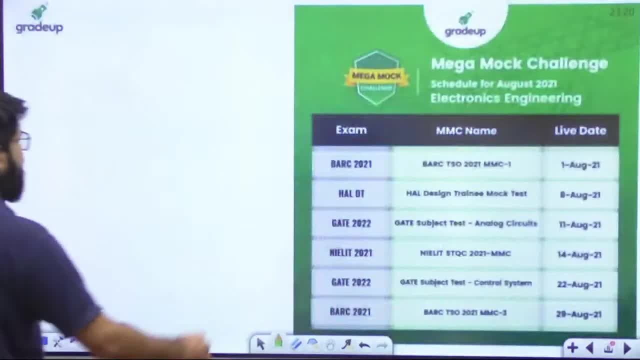 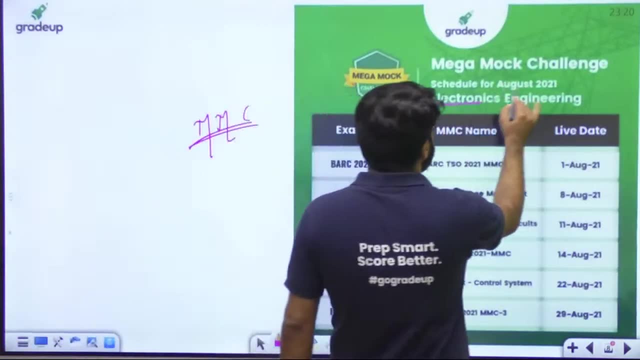 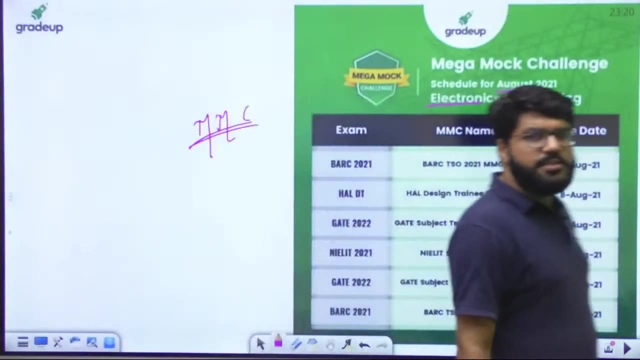 Kumar, All right, This is the MMC, the mega mock challenge for electronics and communication engineering for the month of August. The electronic students can take a snapshot of this and appear in the examinations on these specified dates, on these specified dates, Right. 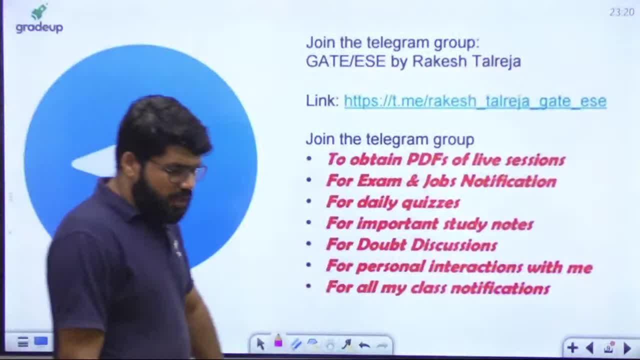 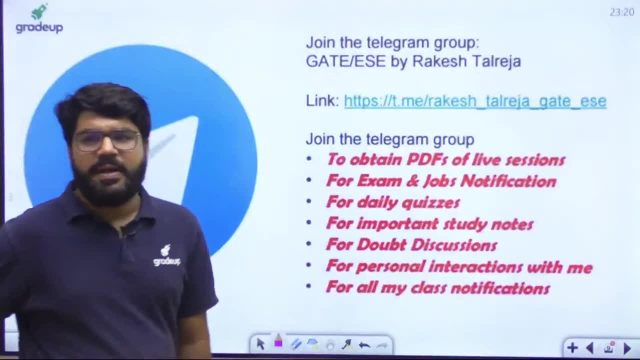 Moving ahead. Yes, guys, as you know, the daily PDF of whatever session we are conducting here, The daily PDFs are available on my telegramcom. GATE slash ESE by Rakesh Talreja. Yes, yes, Kylie Hamilton theorem is there. Very important for GATE syllabus. 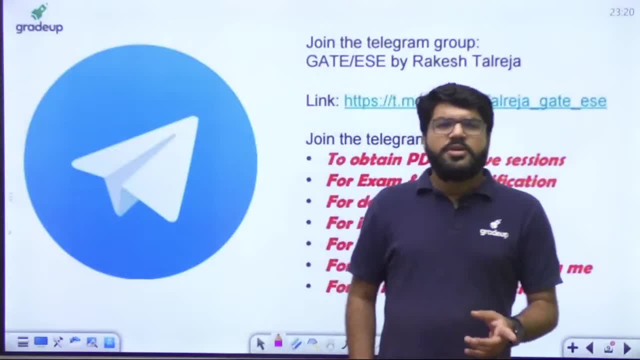 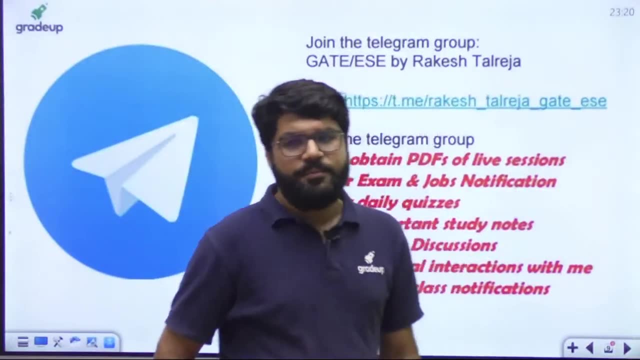 Okay, Kylie Hamilton theorem is studied with eigenvalues, So probably the second class eigenvalues. tomorrow I will cover up the questions of Kylie Hamilton also within that. Don't worry, We'll cover up the questions of Kylie Hamilton theorem as well, Right? 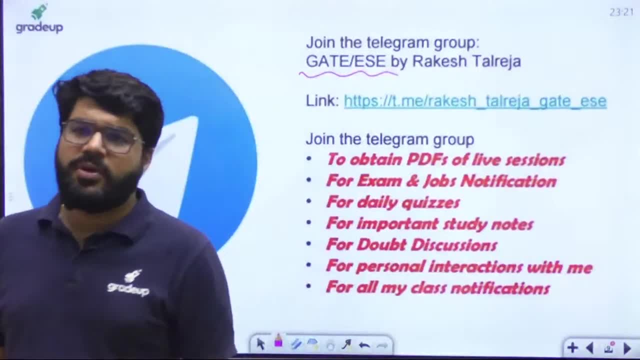 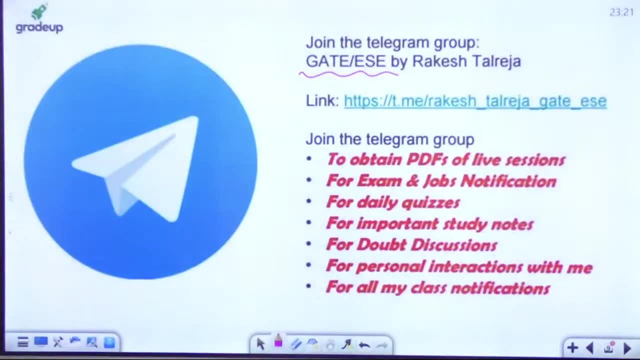 So this is my telegram group, GATE slash ESE by Rakesh Talreja. You can join this telegram group to obtain the PDFs of the live session: Quizzes, Doubt discussions, Personal interactions with me and etc. Right. 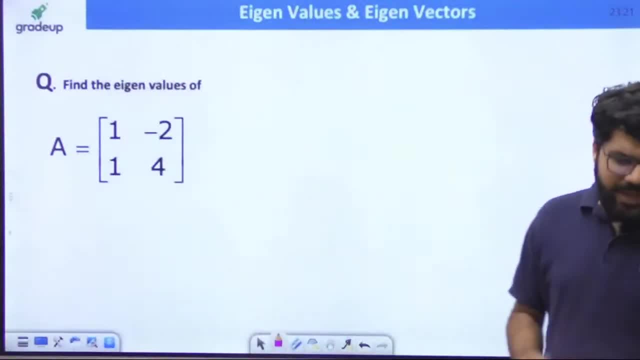 Okay, guys, First question here on your screen, The first question. Let us get started with the question series. Find the eigenvalues of the Matrix A1 minus 2,1,4.. Starting with a real matrix. Starting with a 2 cross 2 real matrix. 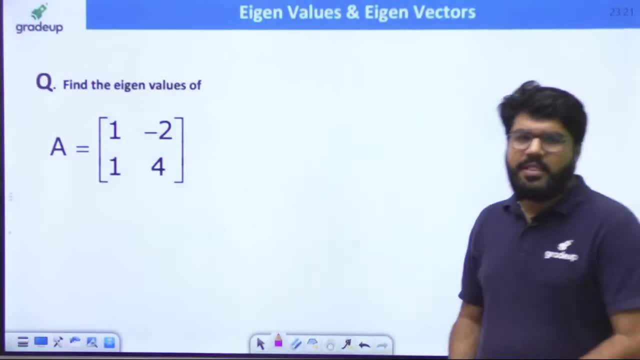 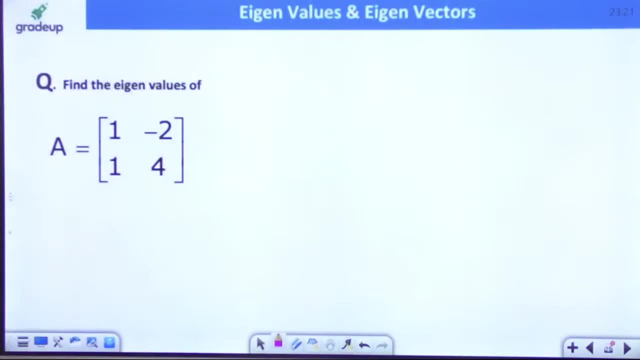 Hi, Hello, Namaskar, sabhi log kko and start karate hai in an enthusiastic manner with the first question of the day. Okay, first question. What is this? Okay, first question of the day. Yes, that is also in the syllabus. LU Priyankite is there for the 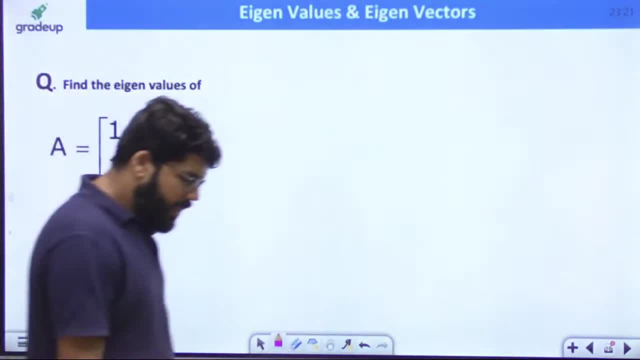 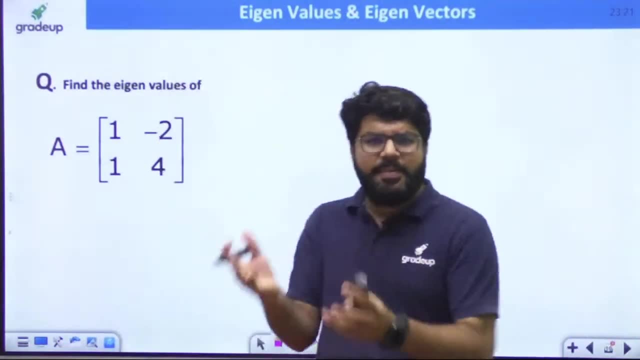 CSE, specially 1, minus 2, 1 and 4.. So, guys, when I want to talk about the eigenvalues, you know what is the equation you have to solve. a brief idea: Let's take a because theory, ma zyada detail pe. 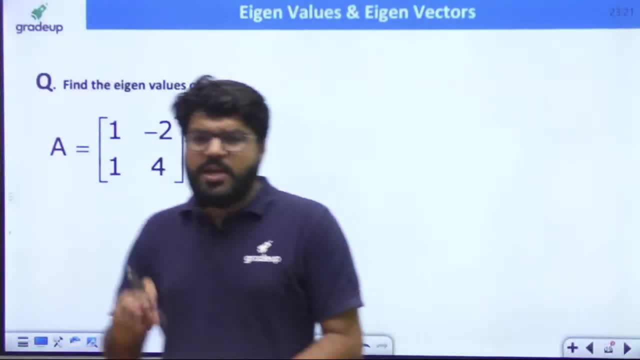 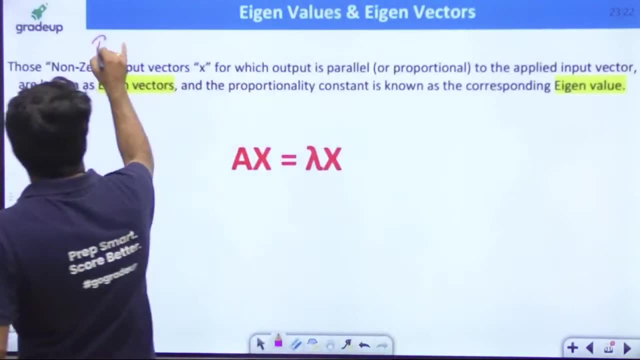 nahi jayenge. but let's take a brief idea and let's come to the question. as always, So little bit, 5-10 minutes. I'll tell you the brief theory required. So, as we know, okay, as we know, everybody can try to recall the definitions, the non-zero input vectors, x, for which the output Now, what is the? 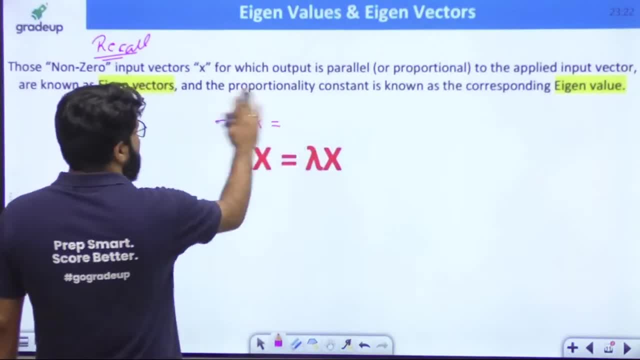 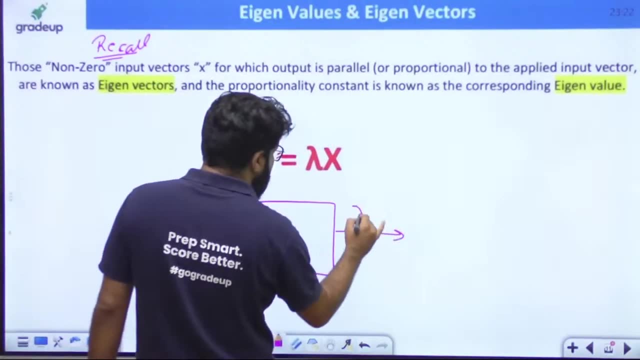 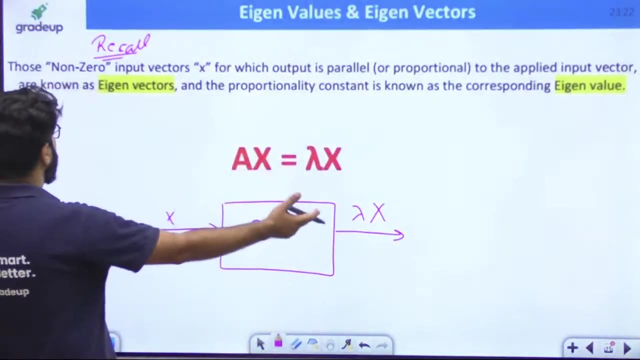 output of every linear system of equation A- x. Okay, A into x. So there is a system described by the matrix A. You apply the input x and you get the output proportional to x. The non-zero input vectors, for which the output is proportional to the applied input vector, is known as the. 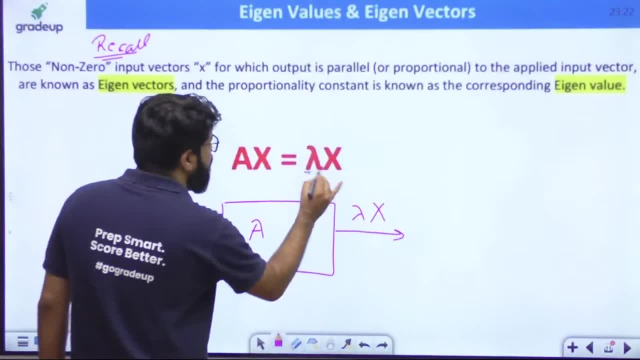 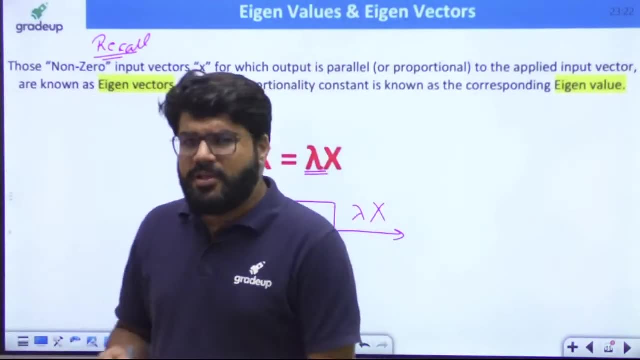 eigenvector. So the x is named as the eigenvector and this proportionality constant and the proportionality constant lambda is known as the corresponding eigenvalue. Okay so, just revising the basic theory point because questions most and most questions we have to do here. 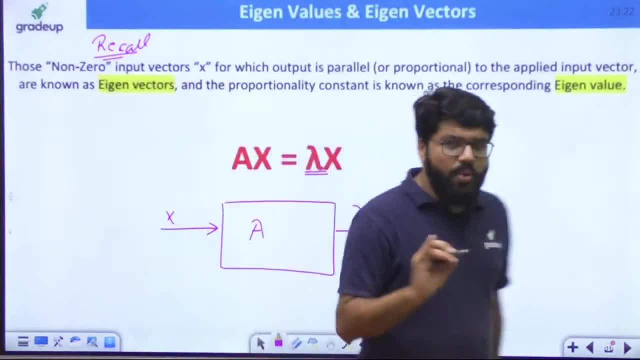 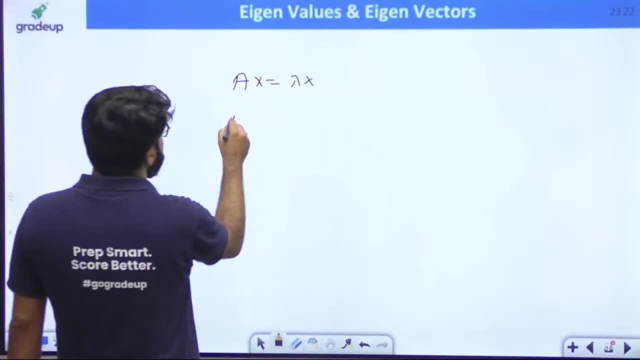 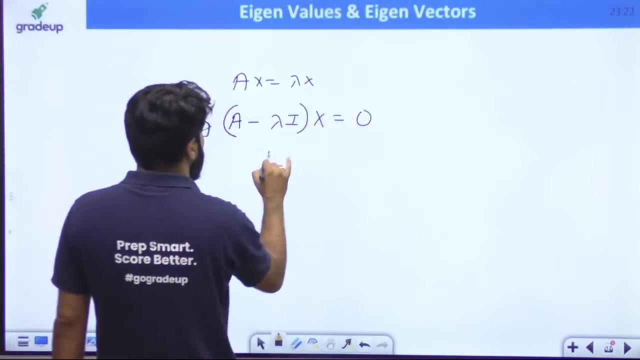 Chalo, so answers are already coming up on the screen. Okay now A x equal to lambda x leads to a simple result: A x equal to lambda x. or I can say that A minus lambda, but A is a matrix, lambda is a number, So I need to write lambda i into x equal to 0, which is like B. 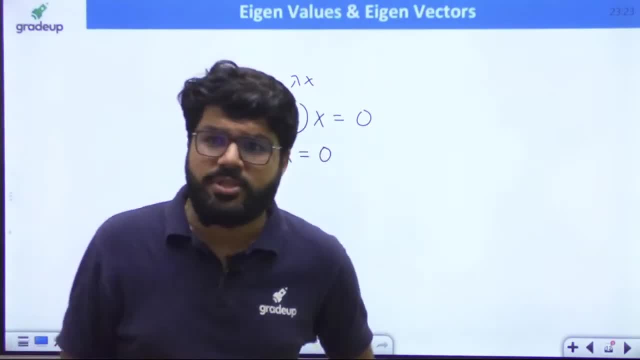 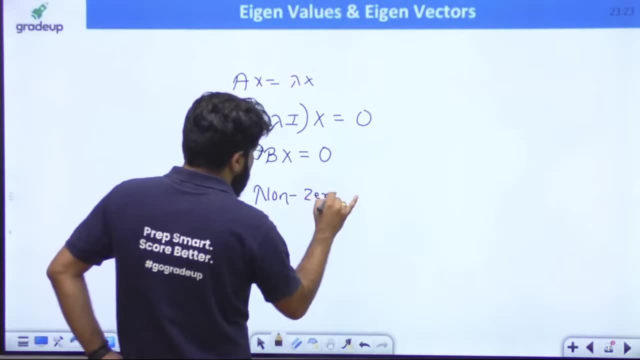 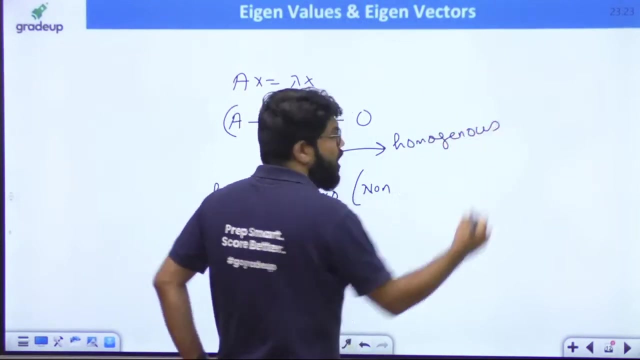 x equal to 0.. Right, and you need what You need: the non-zero solution. Right, you need the non-zero. Okay, and that is the non-trivial solution, because this becomes the homogeneous system of equation. You can relate with the last class, Okay, or eigenvalue: tricks se nikalenge, We are not going. 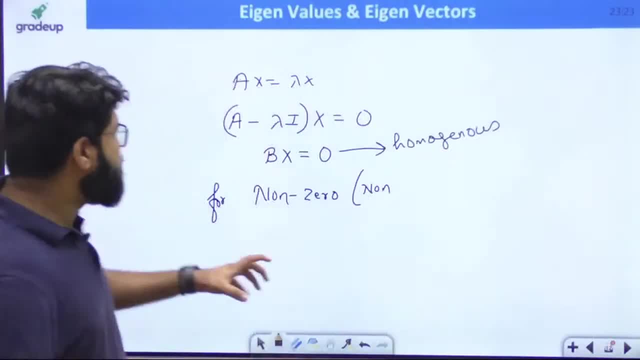 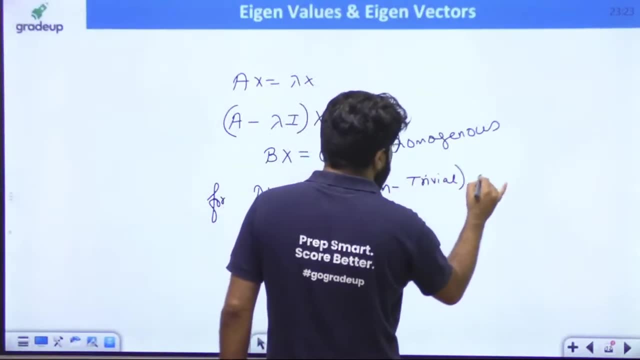 to solve it up in a lengthy manner. We will have the simplest tricks here. Okay, just stay tuned. So for non-zero, right? or I can say that non-trivial solution. So this has two types of cases: trivial and non-trivial. So for non-trivial solution, we want. 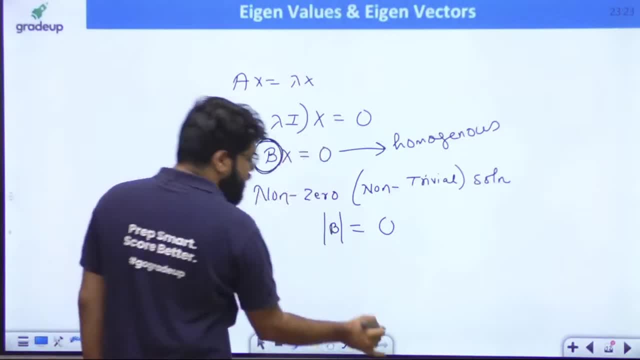 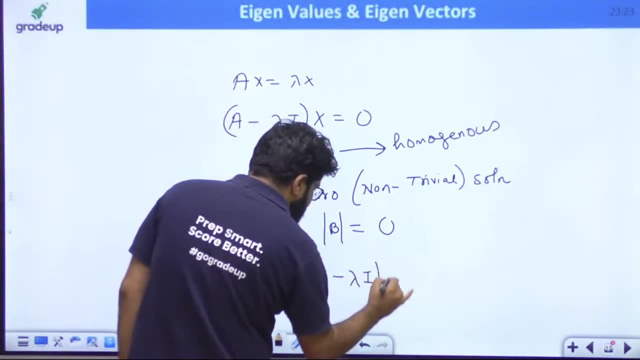 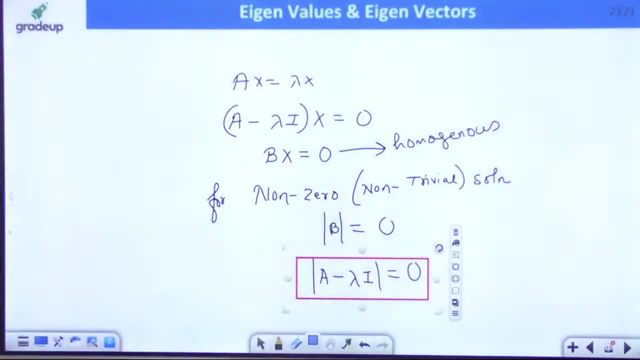 the determinant of the matrix. Which matrix The system is B x equal to 0.. We want the determinant of B equal to 0. That means we want the determinant of A minus lambda i equal to 0, and this is what is the first important thing to be discussed here. Mod of A minus lambda i equal to 0 is basically: 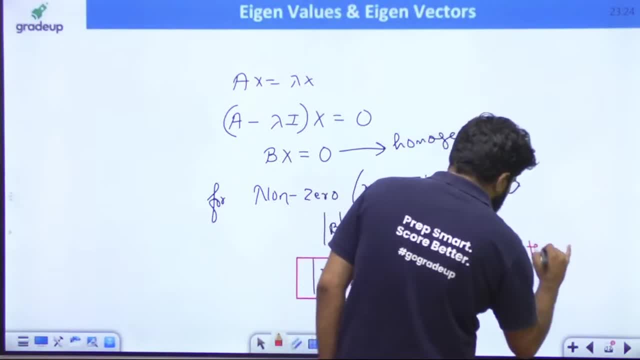 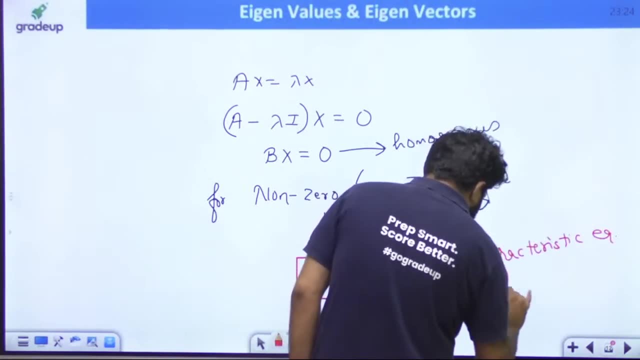 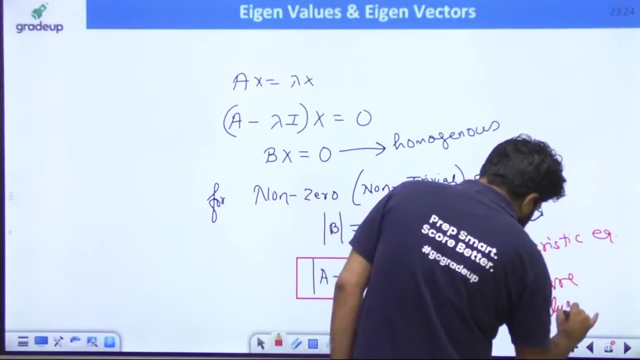 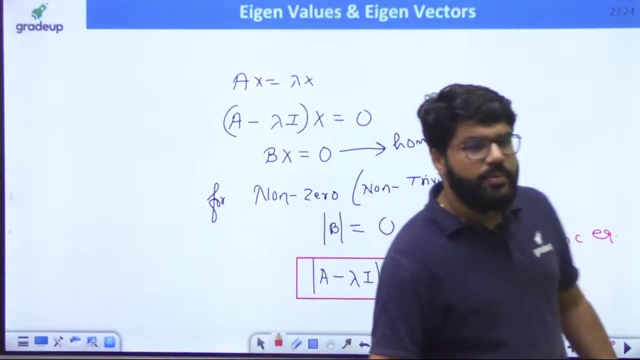 named as what Is basically known as the Characteristic equation of the matrix A and its roots are. The roots of the characteristic equation are the eigenvalues. The roots of the characteristic equation are known as the eigenvalues. The modulus of A minus lambda i, equal to 0, is known as the characteristic. 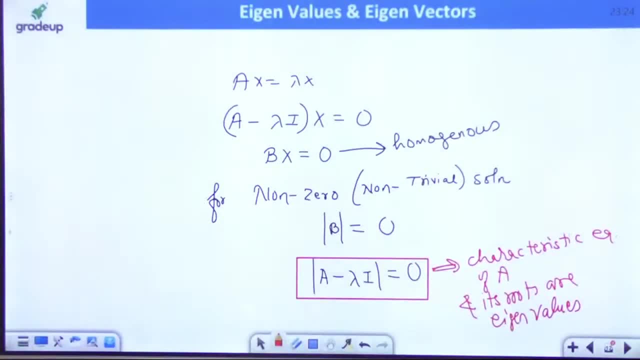 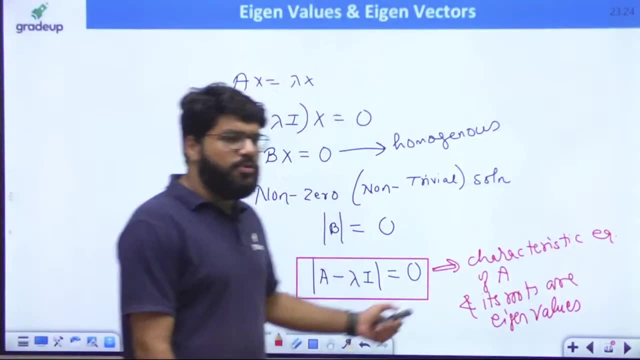 equation of A and its roots are known as the eigenvalues And its roots are known as the eigenvalues. everybody Correct. So this is what. So, to solve any eigenvalue based problem, we need to find the roots of the characteristic equation, simply Chalo. so now this question. 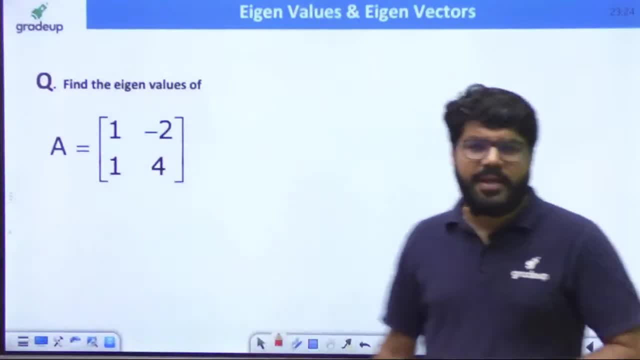 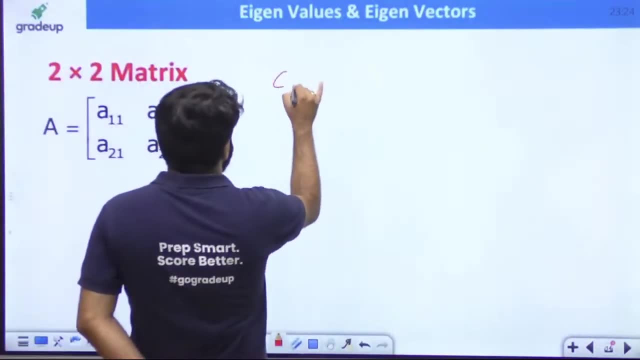 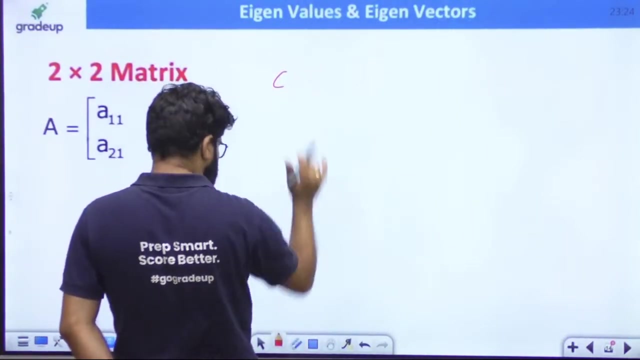 is on a 2 cross 2 matrix. Okay, theory ko ekdum concise mein summarize karna hai. So now, whenever I have a 2 cross 2 matrix, Whenever I have a 2 cross 2 matrix, Just a second, Okay, it's. 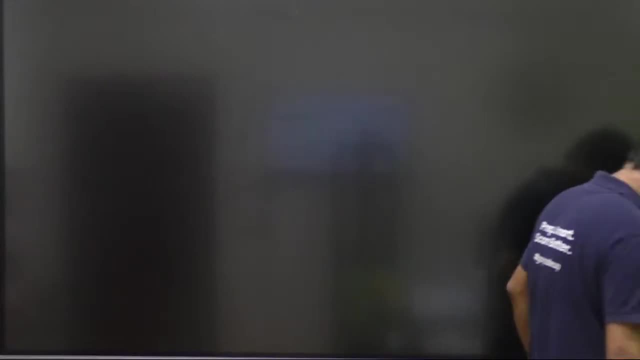 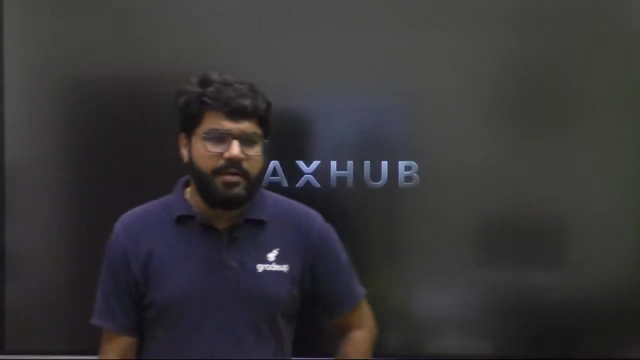 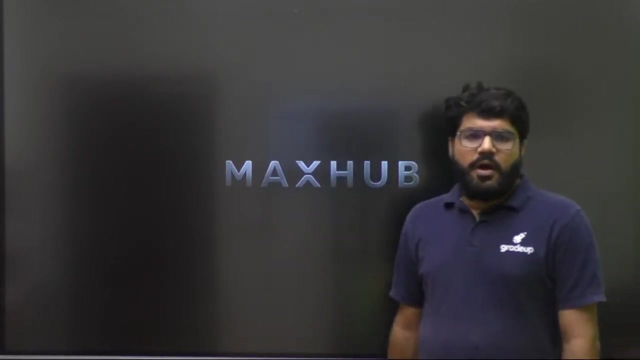 is just one second why this smart board is off. I think there is some some issue happened. ha, let's just wait for a moment. let's just wait for a moment, guys. alright, just quietly kindly wait for a moment. I think it suddenly restarted. yes, yes, yes, Priyanka, if you are a CSE student, then yes, LU decomposition is there. 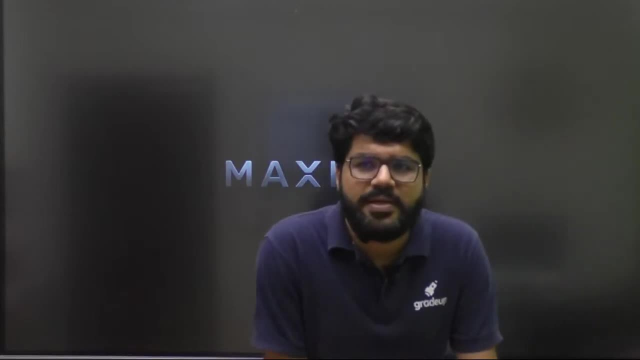 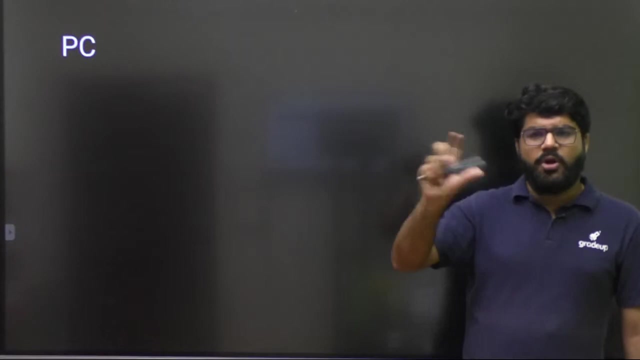 it suddenly restarted. we will wait a little, guys, no worries, because 2 cross 2 or 3 cross 3. I am not going to solve a minus lambda. i equal to 0. I am not going to solve that. I am going to give you the direct result for 2 cross 2 and 3 cross 3. 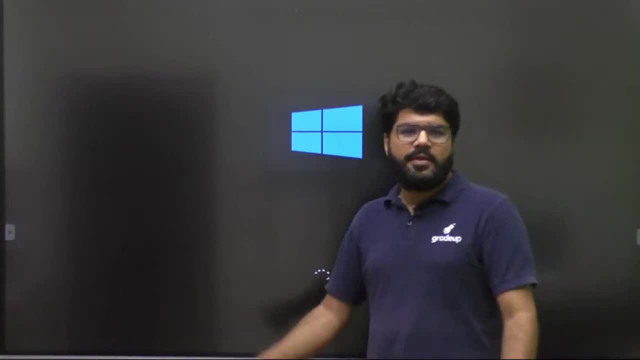 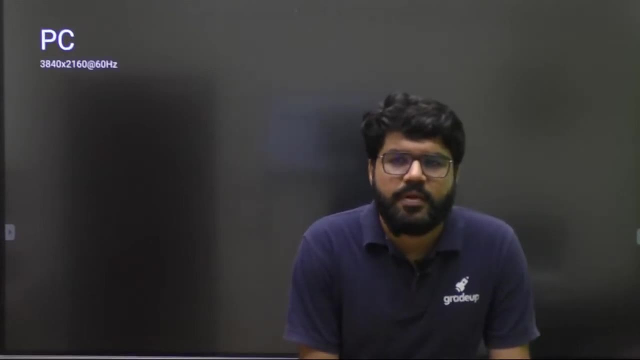 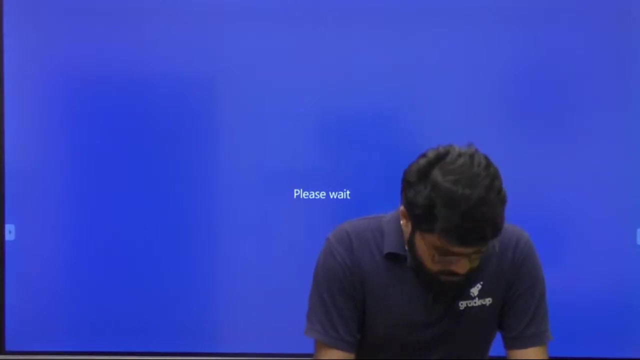 that direct result was coming that there is some barrier in our path, but no issues. no issues, we can just create it up easily. so yes, by the time, if any doubt is out, then you can comment on it. comment up the doubt, we can discuss up the doubt. by that time, no issues, it is usually some, some it does not. 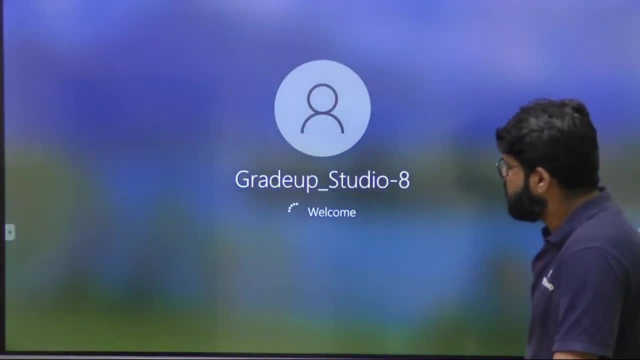 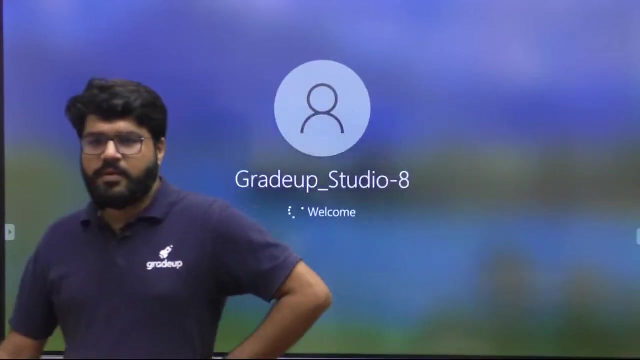 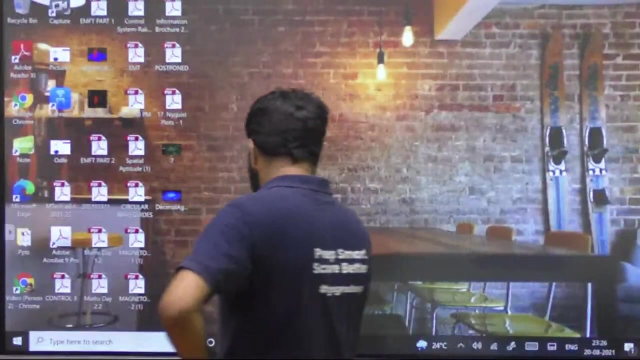 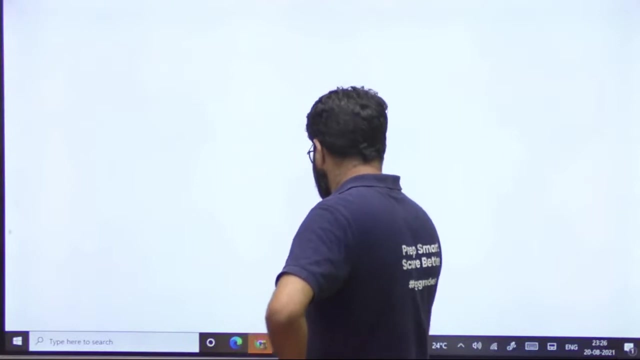 take much time. it is usually taking some longer time even to start up. yeah, nothing to worry about, and we, if at least if guys have any concern, that's all good. so, thanks, agr, thank you, that's all I have to say, and see you tomorrow, okay, bye. 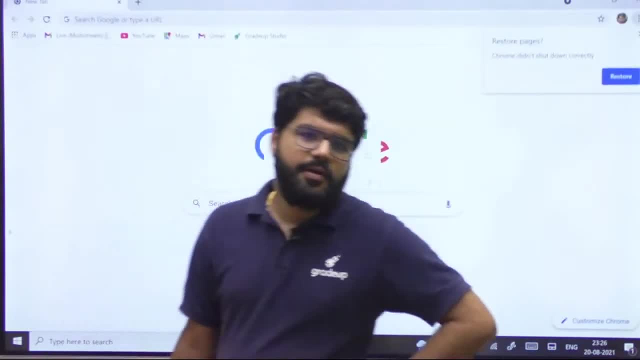 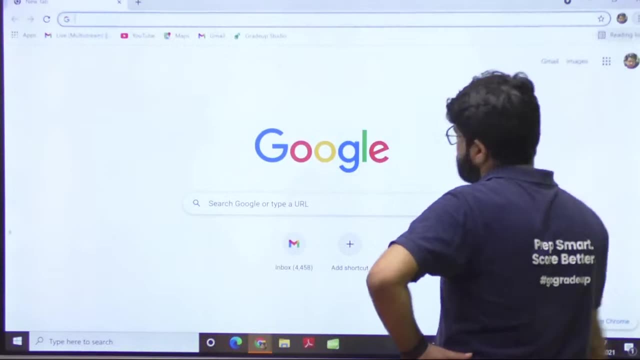 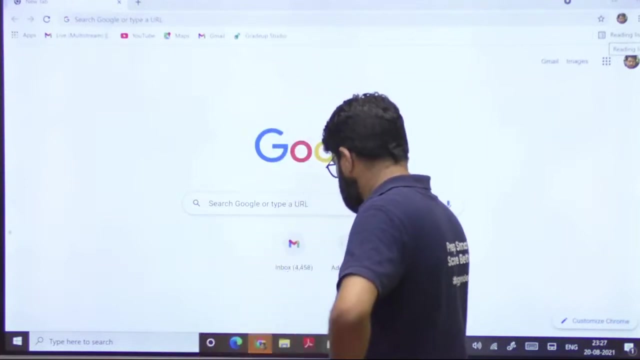 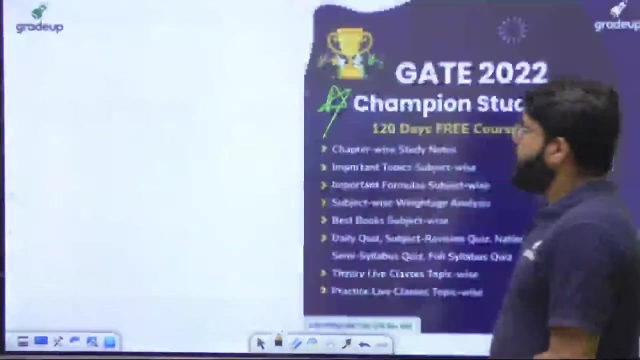 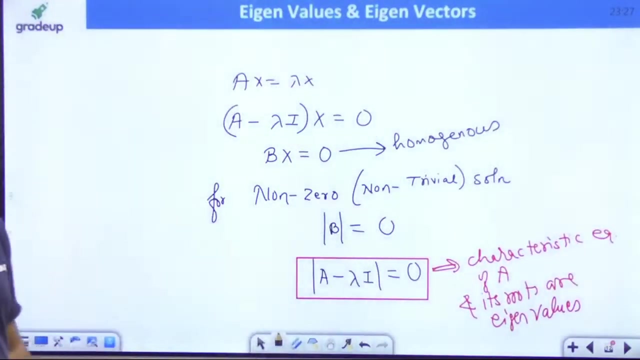 have a great day. you good night, bye, bye, bye. just maybe another one minute or so. maximum note is still not starting, so thank God, we have even our document saved with us. ha, so we have the document also saved with us. no issues, take care, we have the document also saved, so very 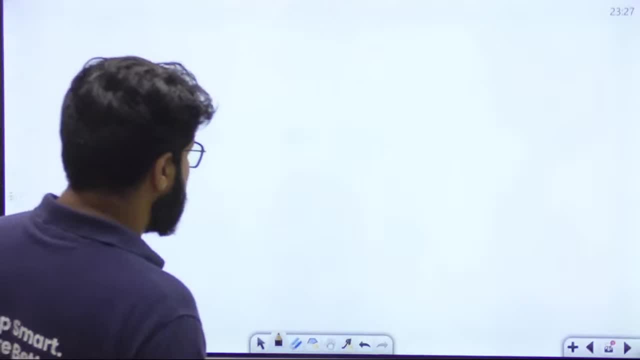 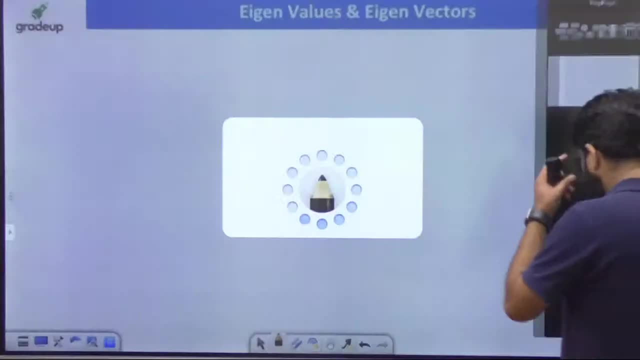 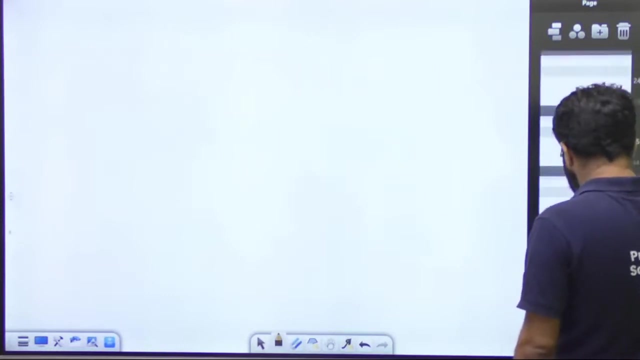 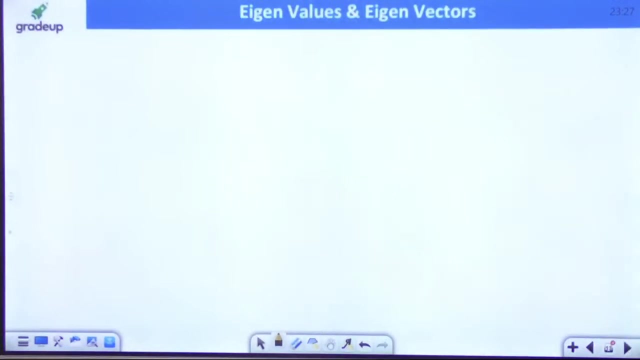 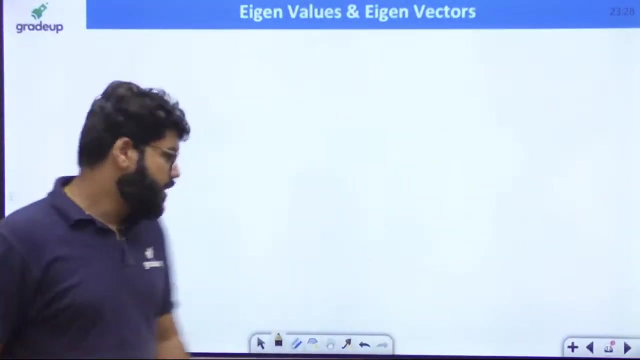 good, no, no, no, no, no, no, no. which the problem why? some issue has happened. where is the rest of the thing? so the co-issue knee, this is there with me after this one. so I'll import the PPT again. some issue is there. I'll import the PDF again. 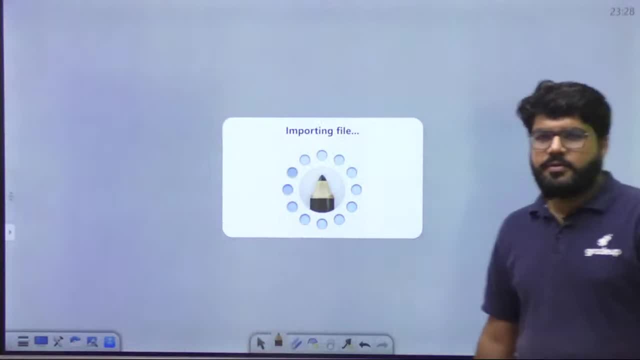 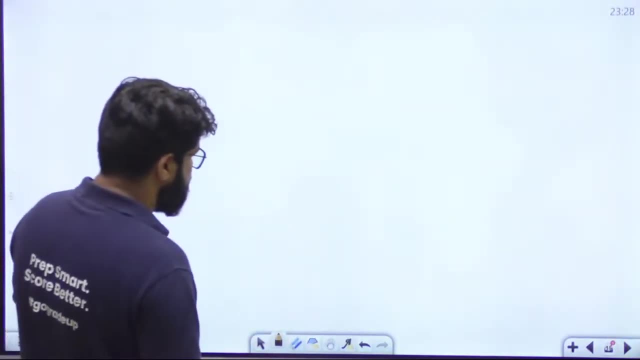 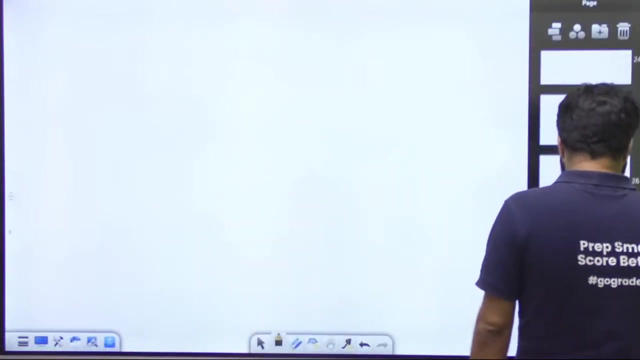 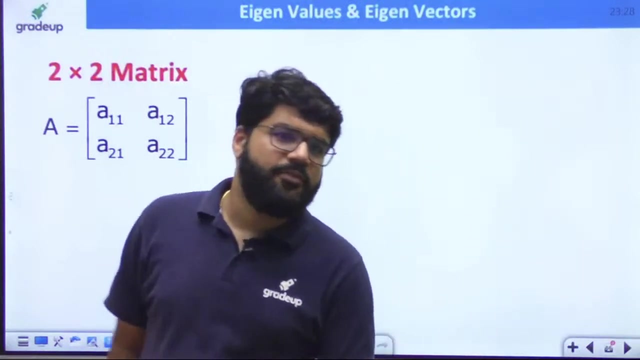 okay, it might be there in the last game. yes, yes, okay, so we need to restart from here. okay, no issues, guys, so sorry for the inconvenience. some technical issue with the board sometimes, so you just need to do this. you just need to just do it. do one thing. 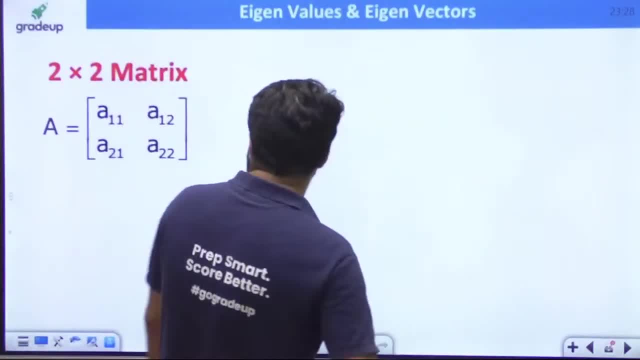 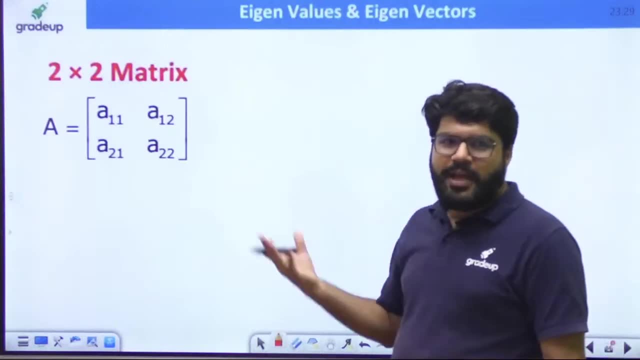 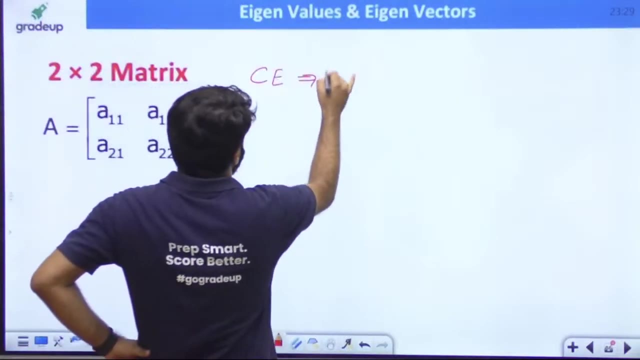 it may be tired, working since morning 11 am continuously okay, so i've already taken four classes on it today, so maybe board is also sometimes tired, maybe we are not tired, but this machine is tired, yeah, yeah. so what i was telling? the characteristic equation in general is modulus of a minus lambda i. 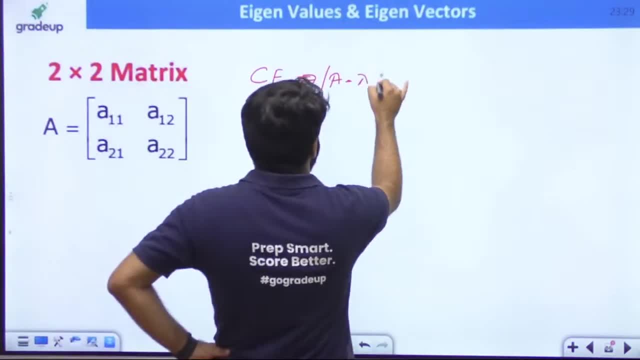 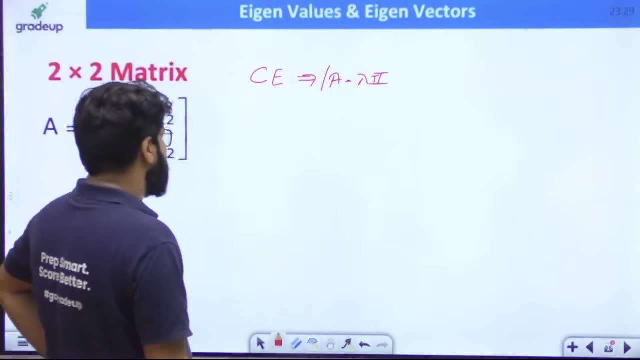 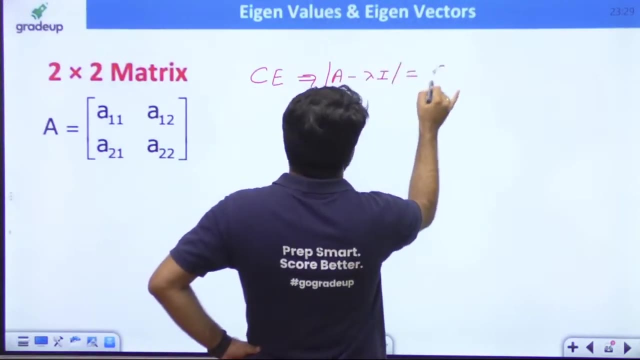 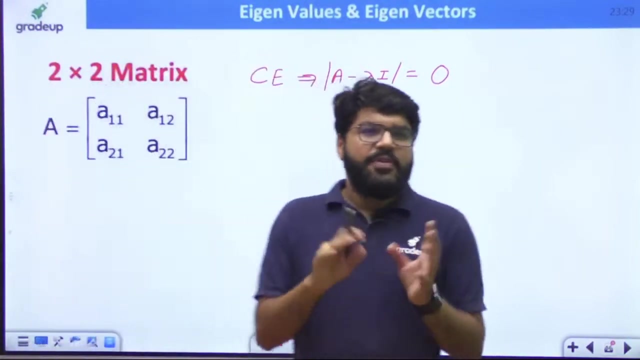 modulus of a minus lambda i equal to the zero. just wait a second, guys. now it is fine. modulus of a minus lambda i equal to zero. that is what is the general characteristic equation i told you right then. then, for every type of matrix, do i need to solve this equation? always, okay, i don't. 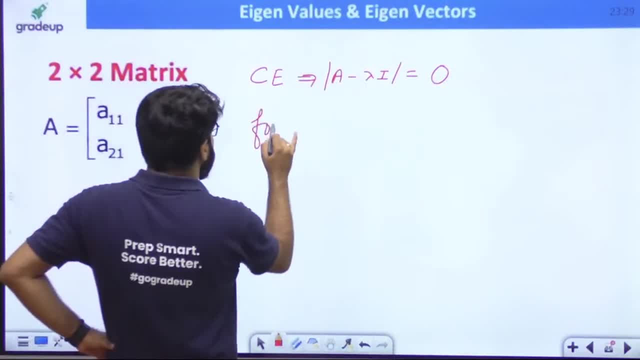 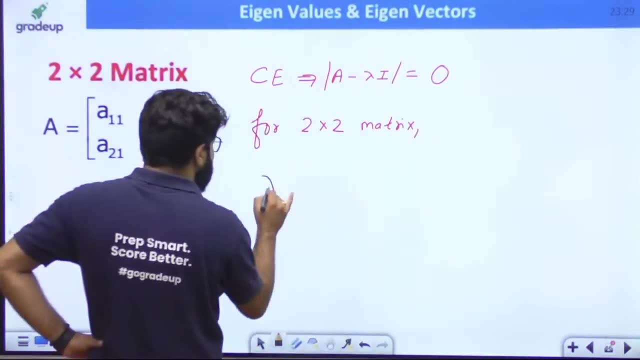 think i need to solve the equation always for a two cross two matrix. direct result for two cross two. after solving: i'm going to solve it for a two cross two matrix. i'm going to solve it for a two. i'm giving you the direct result, no need to derive. it will be written as lambda square. 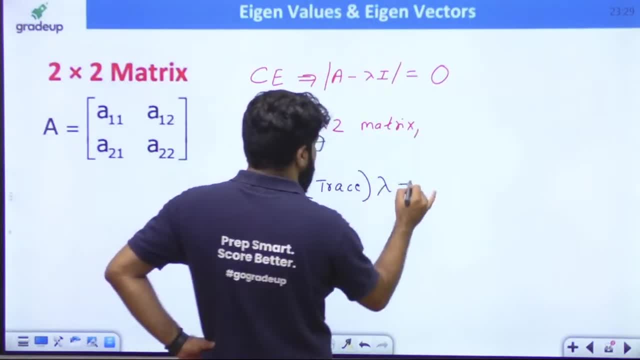 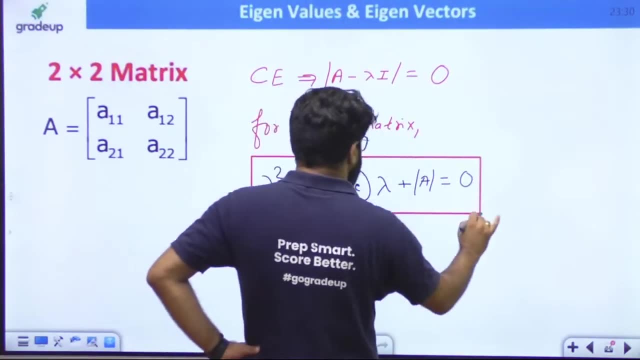 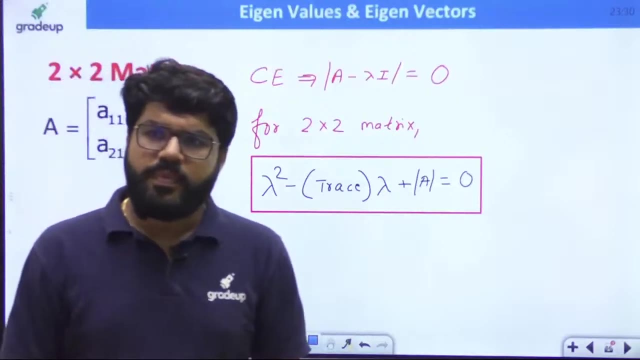 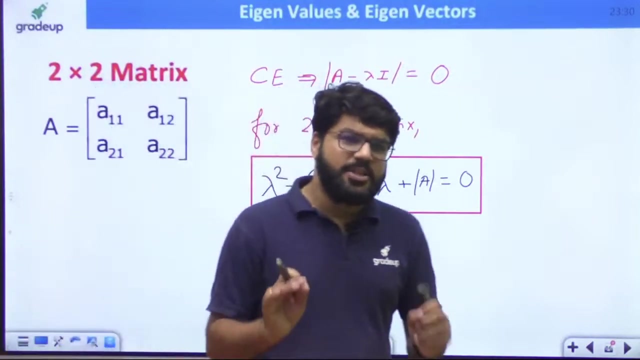 minus trace of the matrix into lambda plus determinant equal to zero. lambda square minus trace into lambda plus determinant equal to zero is equal to zero. wait, rohan, your branch, please. okay. lambda square minus trace of lambda plus determinant equal to zero directly. this is the shortcut you have to take to solve the two cross. 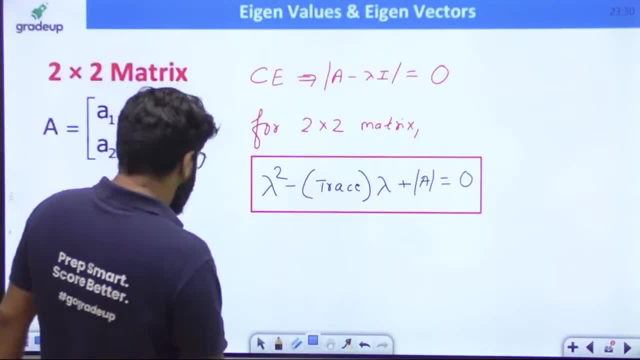 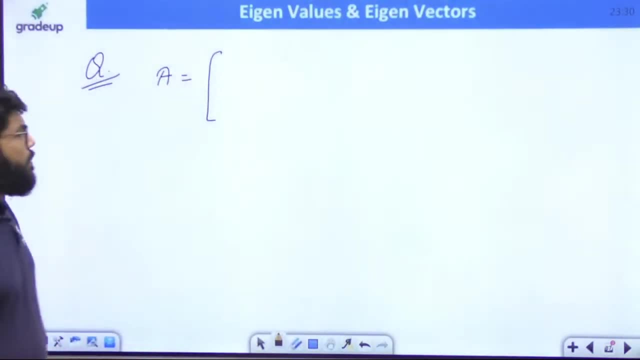 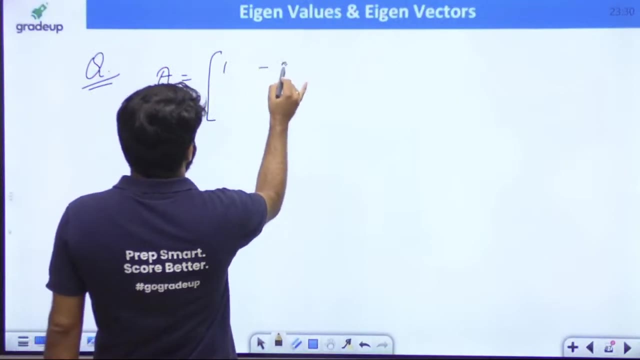 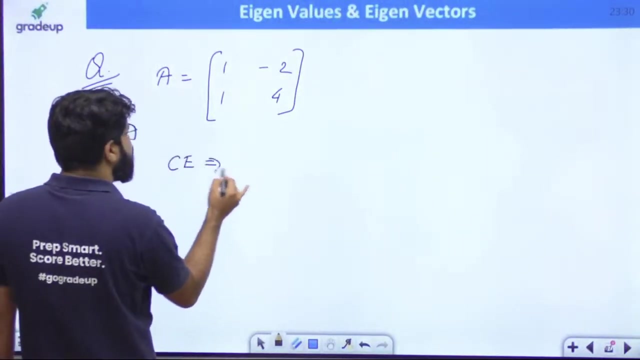 you have to take to solve the two cross two question. so what was my question? actually? my question was: okay, my question was the matrix a. okay, my matrix a was that pdf. my matrix a was that pdf. where is that question? 1 minus 2, 14, 1 minus 2, 1 and 4. this was the matrix. 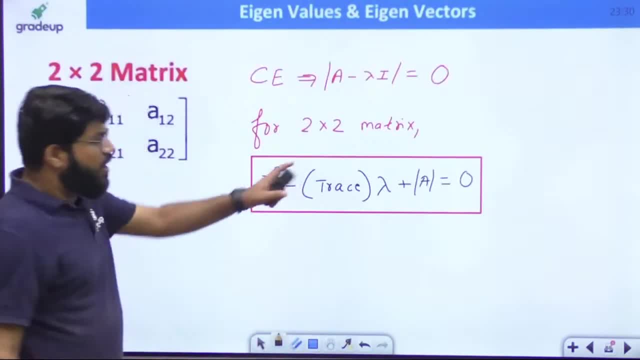 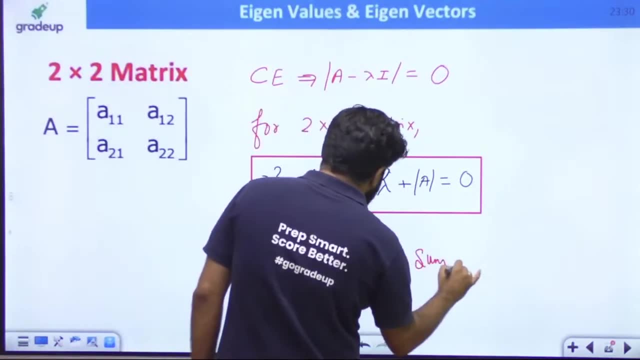 so what is the characteristic equation? in short, i have to write lambda, square minus trace. now, everybody, whatabe. what do you mean by this trace? When I write down trace, what do you mean by the trace? What do you mean by the trace? Trace means sum of. I will just tell you what is meaning of trace. 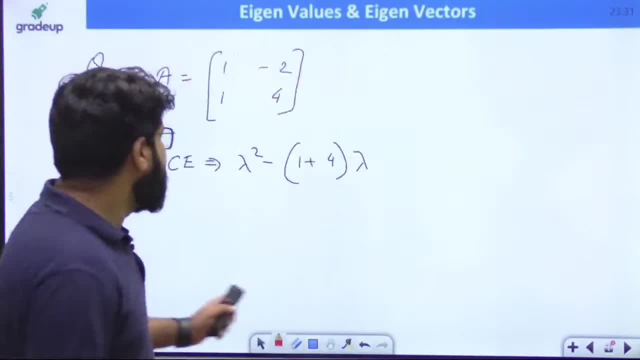 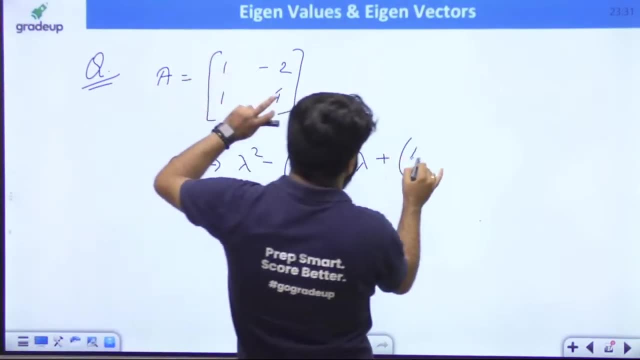 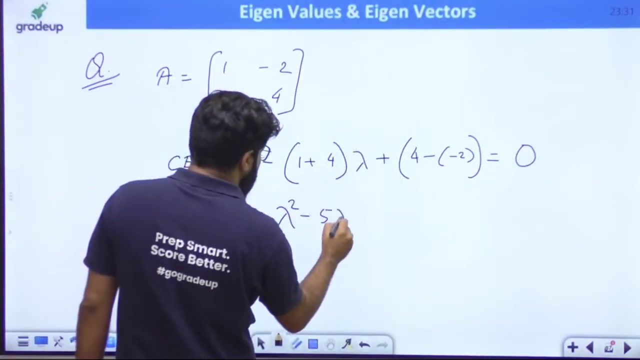 Trace means sum of diagonal elements. Trace means the sum of the diagonal elements. right. The sum of the diagonal elements is 1 plus 4 plus the determinant of the matrix. So determinant cross multiply 4 minus minus 2 equal to the 0.. So eventually I have lambda square minus 5 lambda. 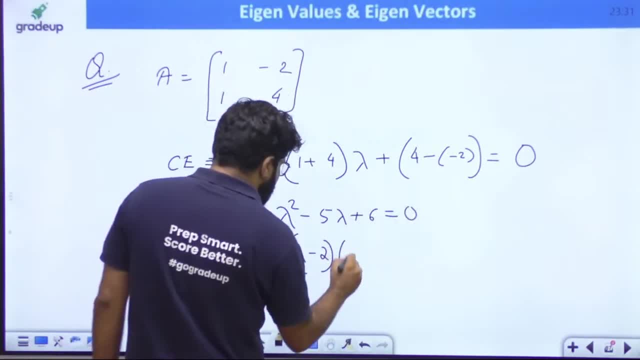 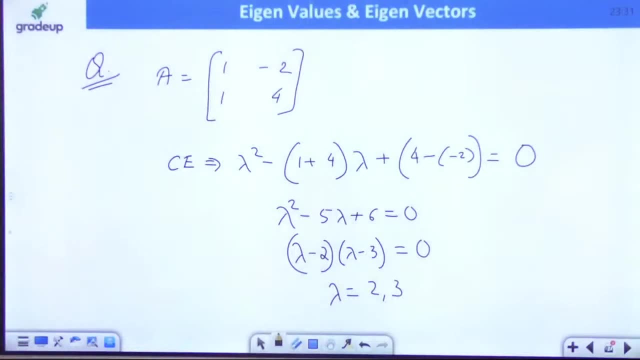 plus 6 equal to 0, and this will be factorized as lambda minus 2, lambda minus 3 equal to the 0, and lambda is 2 and 3.. This is what is the eigenvalues Correct Pragya. Coming to the 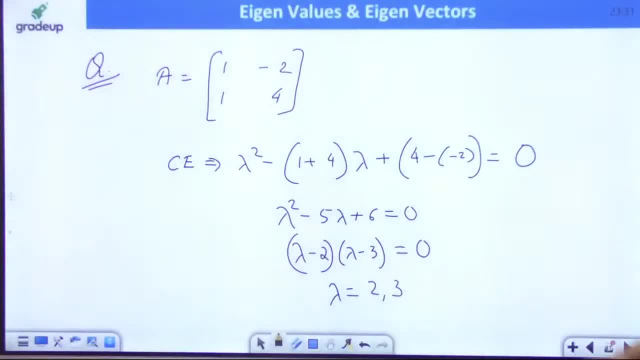 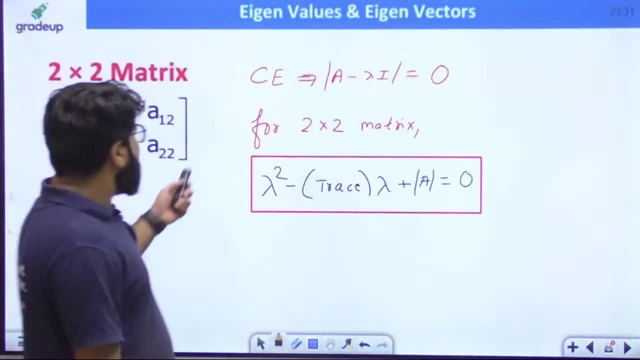 properties also. We will come back to the properties also very quickly. So what is this? lambda is equal to the 2 and 3?? Lambda is equal to the 2 and 3.. Now, this is how simply you are going to take a 2 cross 2.. This is going to be very useful. 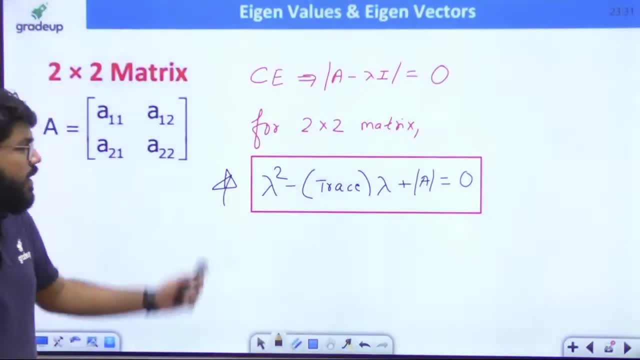 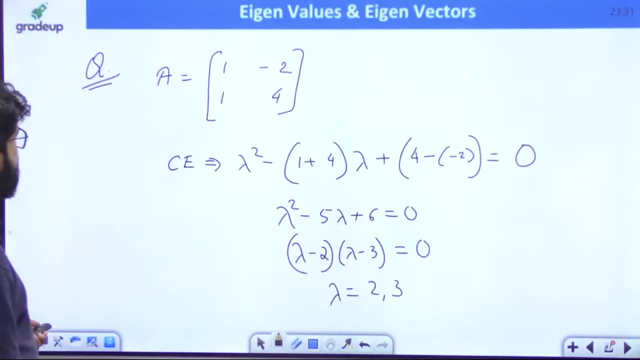 Directly remember. lambda square minus trace into lambda plus. determinant is 0.. When I come to a 3 cross 3 case, yeah, when I come to a 3 cross 3 case. So in general, again, I am writing. 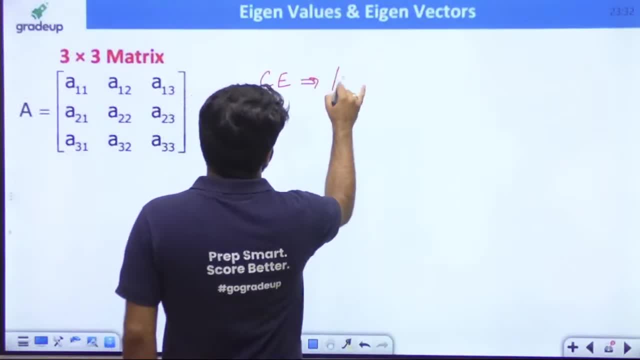 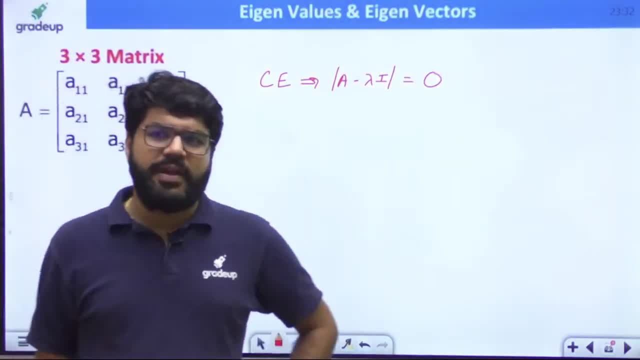 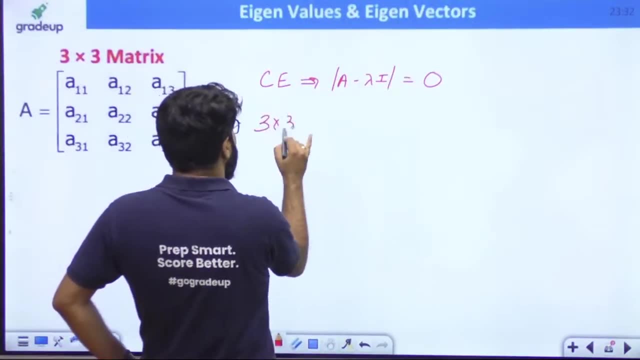 Rohit, Yes, Rohit, Yes, Rohit, Yes. Ah, okay, Got it. So I mean I can plan a separate session on the vector space and basis independent dependent vectors. modulus of a minus lambda i equal to the 0. But for 3 cross 3 matrix, especially For a 3 cross 3 matrix specially. 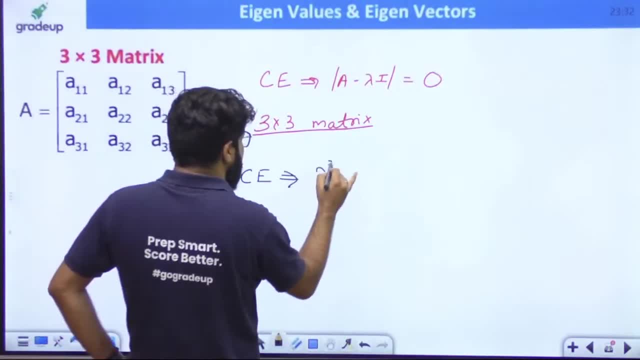 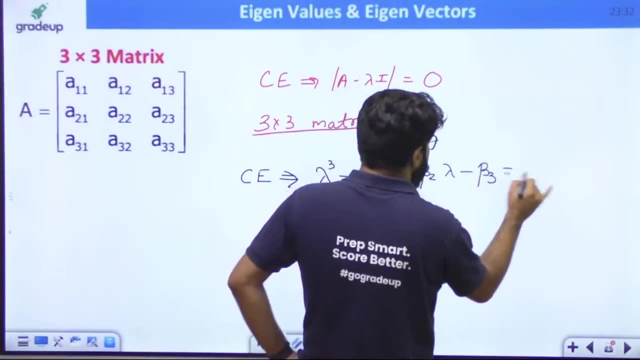 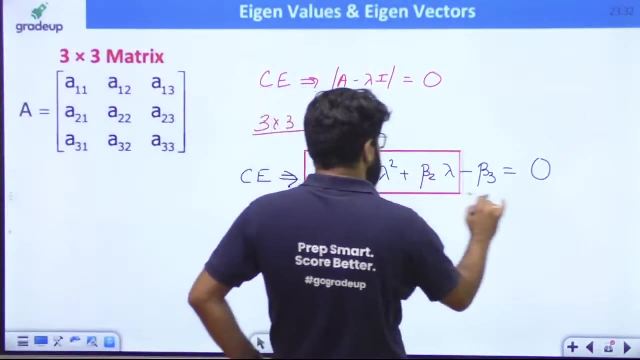 write down the direct characteristic equation which is given by: lambd cube minus beta 1. lambda square plus beta 2. lambda minus beta 3 equal to 0.. Lamda cube- look for the сколько lambda cube minus beta 1. lambda square plus beta 2. lambda minus beta 3 equal to 0.. Direct 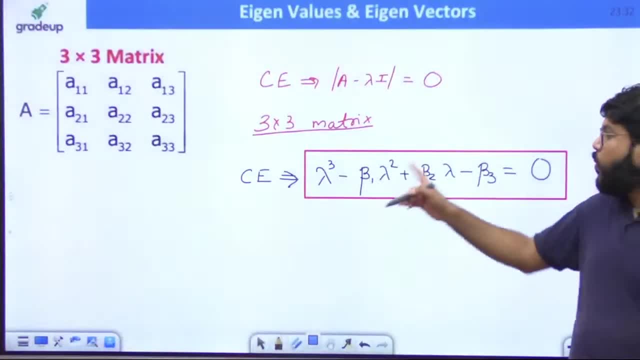 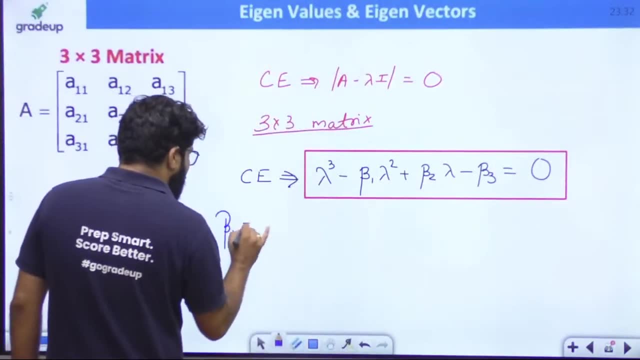 characteristic equation will help you to solve the questions very quickly. But what is beta 1,, beta 2,, beta 3?? Okay, Let us write down. So what is, sir, beta 1?? Beta 1, the first element, that is. 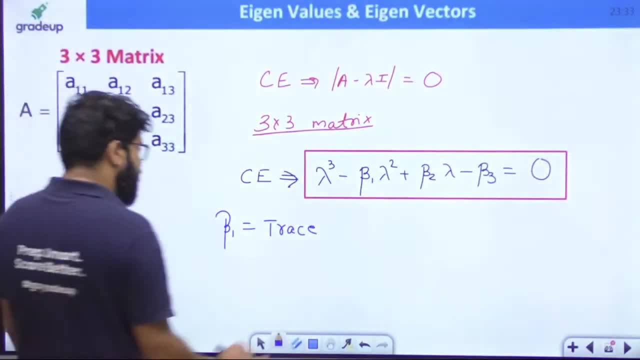 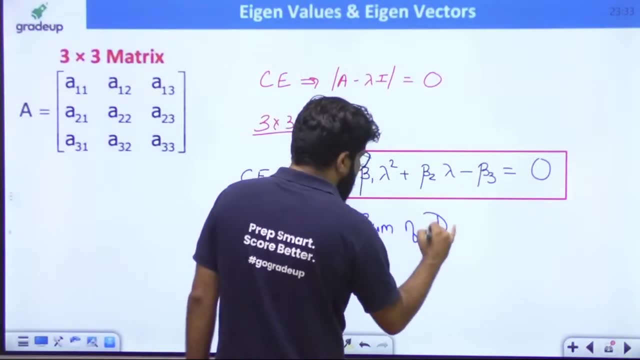 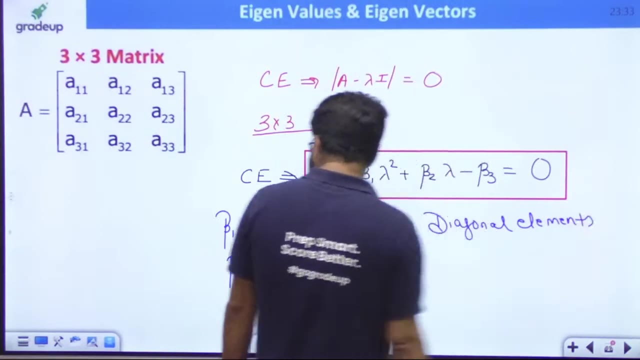 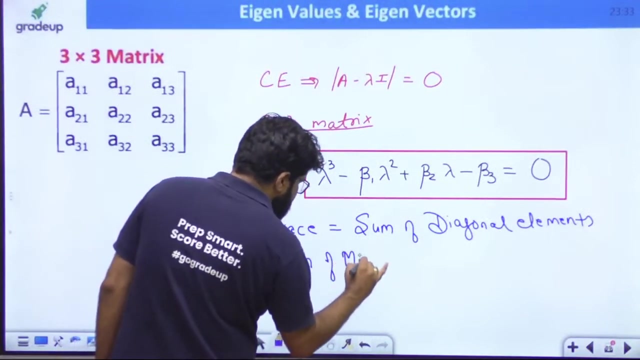 again the trace That is again known as the trace of the matrix. Okay, Beta 2.. As we know, what is trace? Trace means sum of diagonal elements. Trace means the sum of the diagonal elements. What is beta 2?? What is the beta 2? It is equal to sum of the minors. 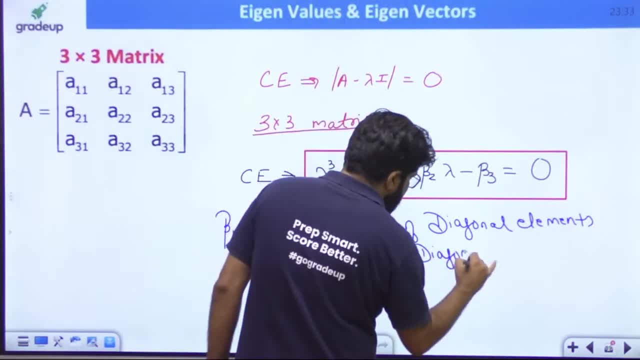 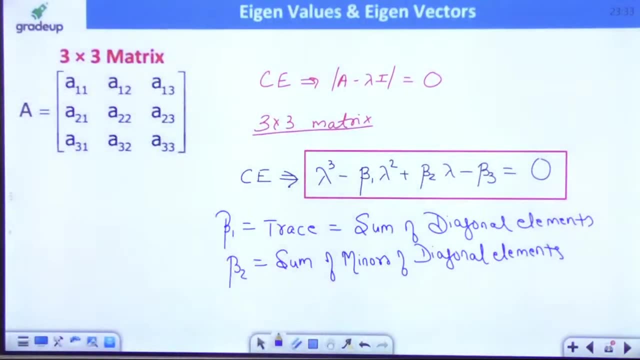 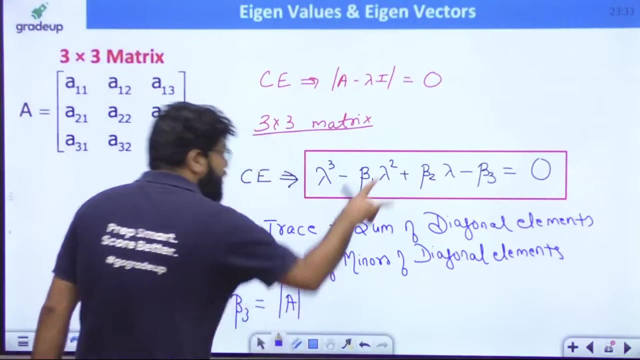 Sum of the minors of the diagonal elements, Some of the minors of the diagonal elements, And what is beta 2?? what is beta 3?? What is beta 3?, Sir, the beta 3 is equal to. again, the last term is the determinant. 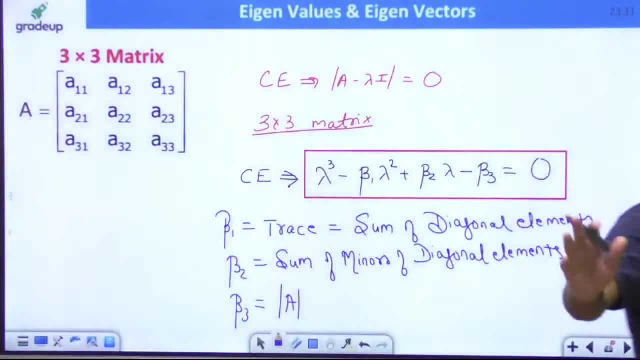 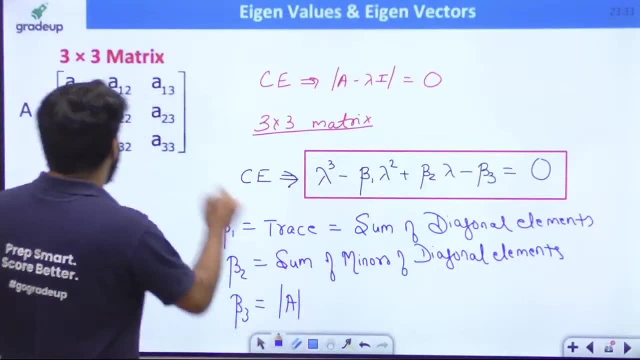 of the matrix. The last term will be the determinant Direct 3 cross 3 questions to be solved directly by this equation. How to apply? What is beta 2, specially Sum of minors? Matlab: this is a diagonal element. find out its minor, Calculate this minor and put here, But not only. 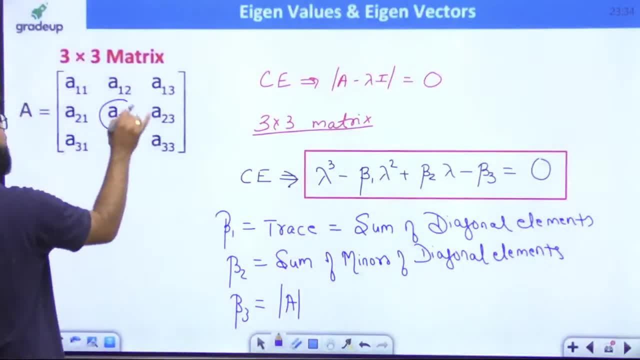 one minor sum of the minors of all diagonal elements. So second diagonal element a to 2.. What is the minor? How do you calculate the minor? Delete the second row and second column, Then you get the remaining numbers. Calculate the minors from the remaining numbers and etc. 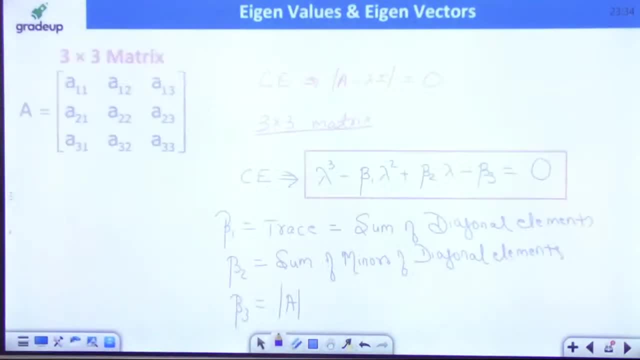 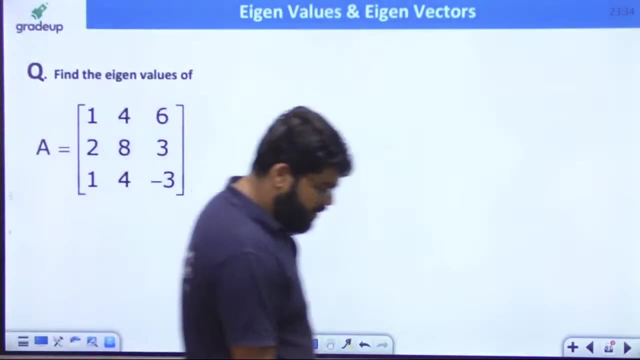 And etc, etc, etc. Okay, So this is what is the 3 cross 3 matrix? A question on the 3 cross 3 matrix. A question on the 3 cross 3 matrix. Everybody have a note here. A question on the. 3 cross 3 matrix. Find the eigenvalues of 1,, 4,, 6,, 2,, 8,, 3, 1, 4, minus 3.. Okay, 2 or 3 direct questions, and then we are going to the properties and property based questions. 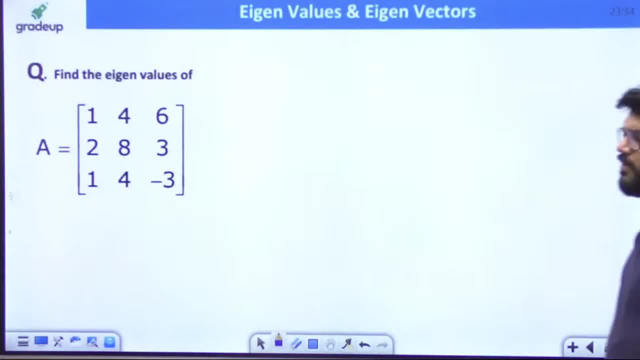 So everybody, find the eigenvalues of 1,, 4,, 6,, 2,, 8,, 3,, 1, 4, minus 3.. 1, 4, minus 3, and tell me the answer: 1,, 4,, 6,, 2,, 8,, 3,, 1,, 4 and minus 3.. Everybody Okay? So let us try to calculate. 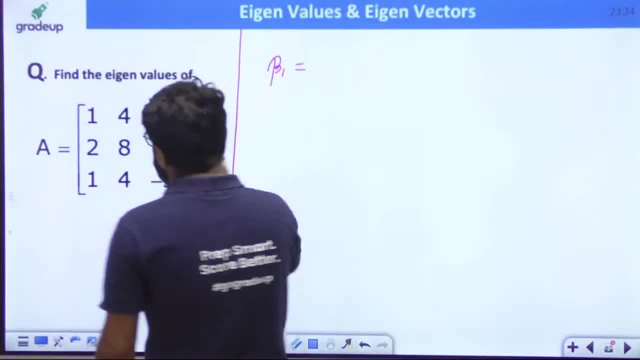 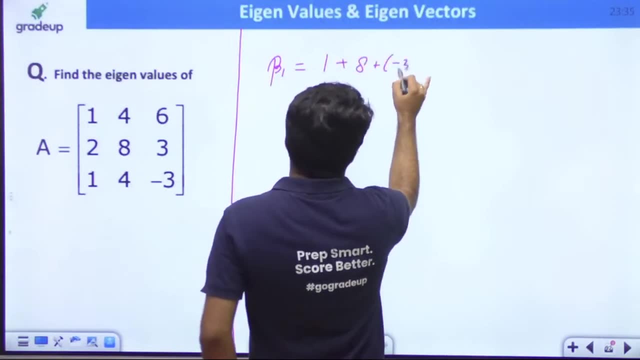 Let us try to calculate What is beta 1, beta 2, beta 3?? Everyone now pay attention here. One question: make the things clear. Okay, Beta 1, 1 plus 8 plus minus 3.. 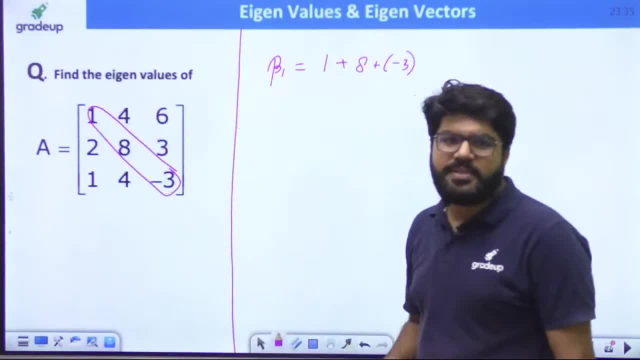 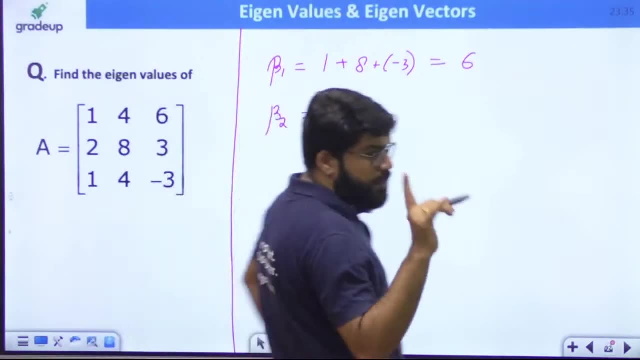 As I told you, beta 1 means the trace of the matrix, and trace means the sum of the diagonal numbers. Correct, So this is equal to the 6.. What is beta 2?? Now everybody see beta 2.. Beta 2,, as I am explaining you, sum of the minors of the diagonal element. This is the first diagonal 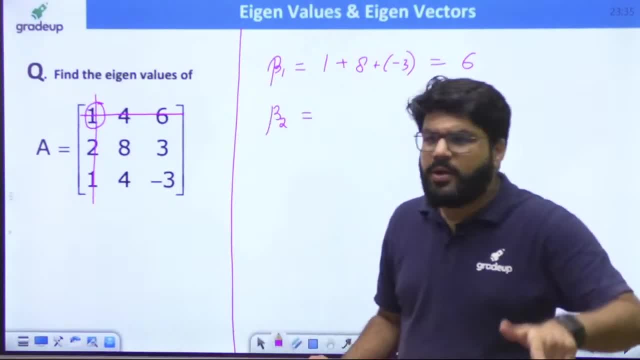 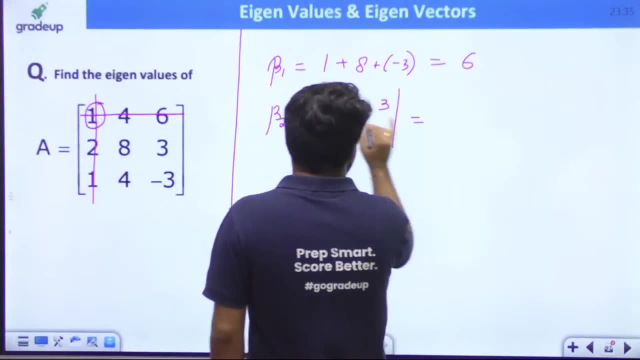 element To obtain the minor. what do you do? Delete the row and column. Row and column could delete. So what is the minor that is coming is 8, 3, 4 and minus 3, and this is minus of 24.. 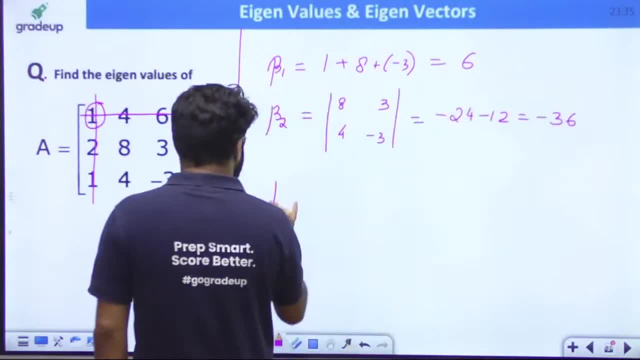 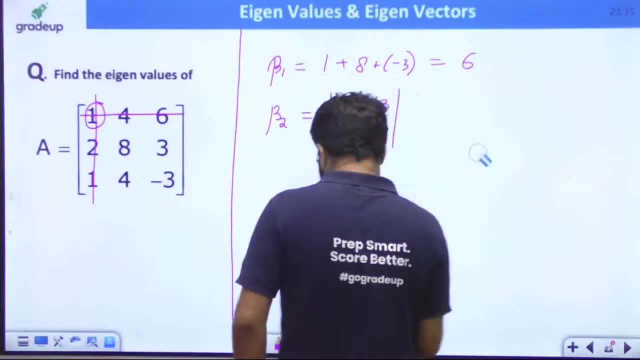 Minus of 12, that is minus 36.. What is beta 3?? Sorry, beta 3,, beta 2 is not complete. Okay, We will calculate in the last Plus. Okay, Let us not complete it like this, Okay, So. 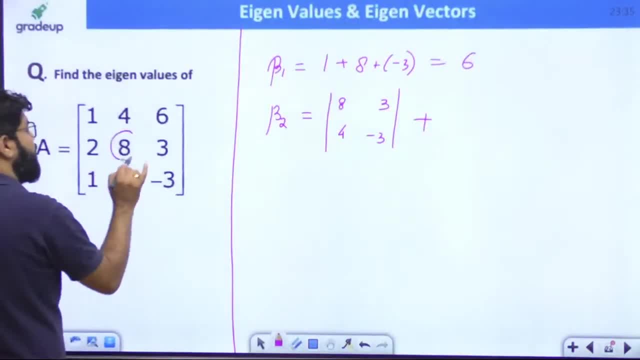 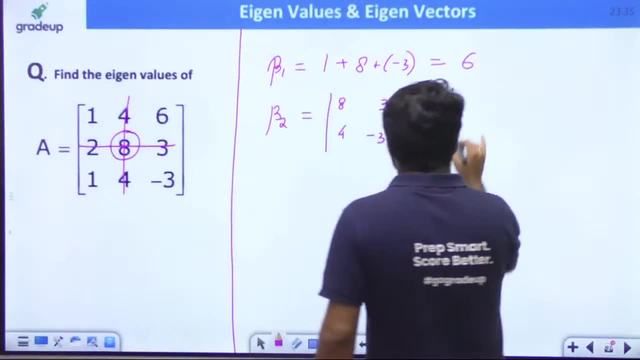 this is one of the minor But sum of the minors of all diagonal element. This is the second diagonal element. Delete the second row and second column. Delete the second row, second column. What are the numbers left? Put it in the minor: 1, 6, 1, minus 3.. Okay, Plus. 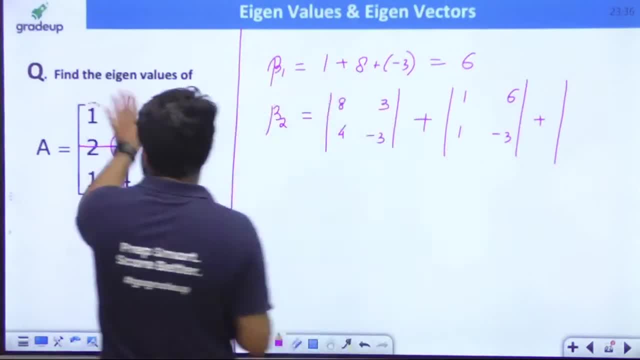 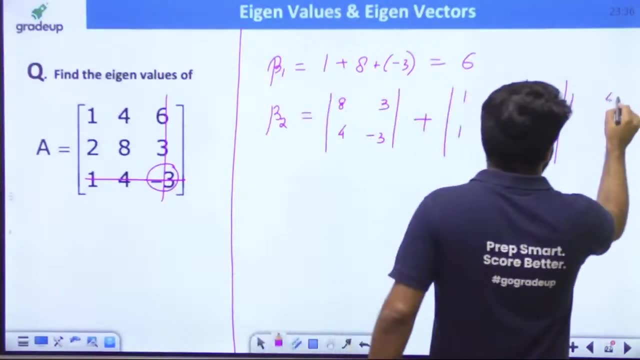 Plus Third diagonal element and the third minor. Take this Okay, This is the third diagonal element and it is minor, So 1, 4,, 2 and 8.. I have written 1 and 4 and 2 and 8.. 1,, 4,, 2 and 8.. 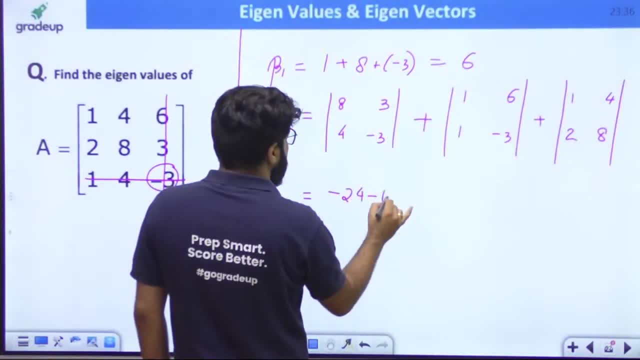 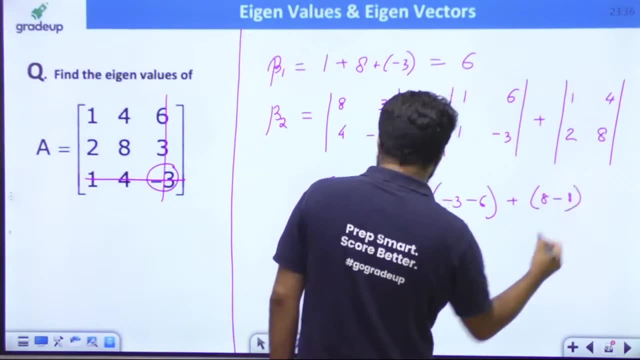 So what is eventually? beta? Minus 24,, minus 12.. Plus, next element, minus 3, minus 6.. Plus next 8, minus 2,: 8 are 4.. 2, 4 are 8.. Right, So this is minus 36, minus 9,. 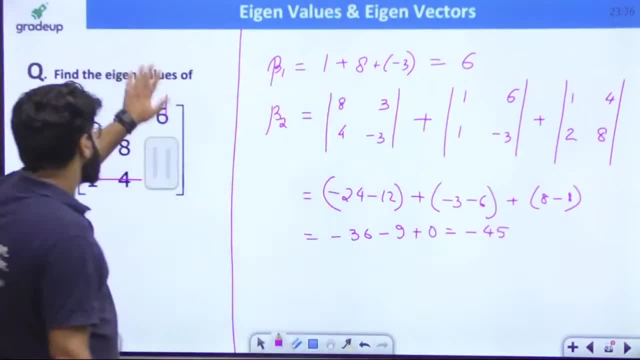 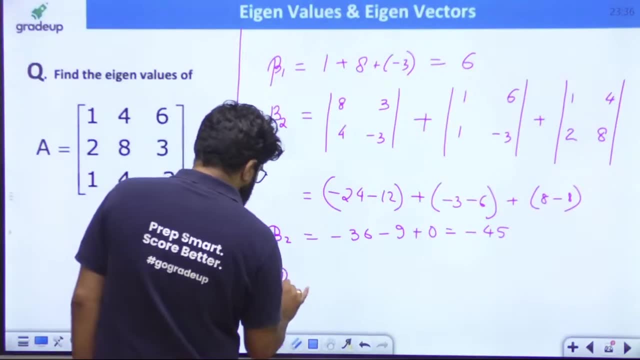 and 0. Answer is the minus 45. Answer is the minus 45. That is beta 2.. What should be the value for beta 3?? What should be the value for beta 3?? So everybody now write down beta 3. 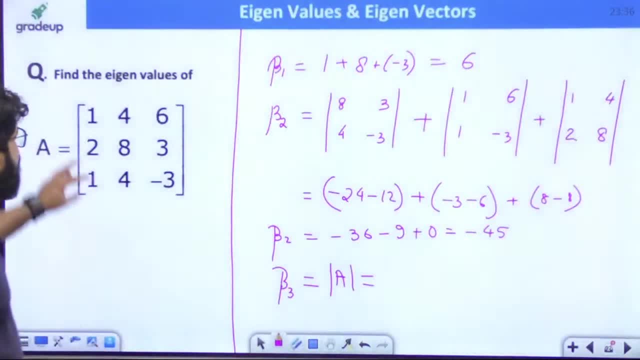 means modulus of the A. Now, what is the modulus of the A? I will show you one simple thing here. I will show you one simple thing if you are able to observe. Otherwise we can calculate the determinant. But here there is a property: If you add up R1 and R3, what is the result? 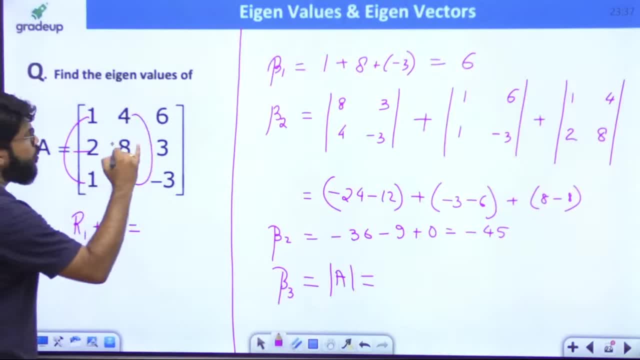 1 plus 1.. Everybody see, 1 plus 1 is 2.. 4 plus 4 is 8.. 6 plus minus 3 is also 3.. So when I add the R1 and R3,- all dear students, when I add the R1 and R3, I get R2.. That means that means there. 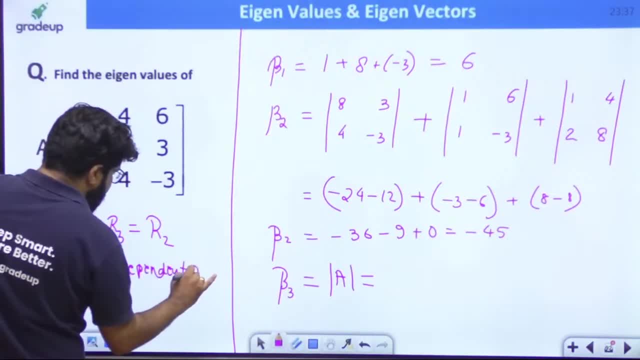 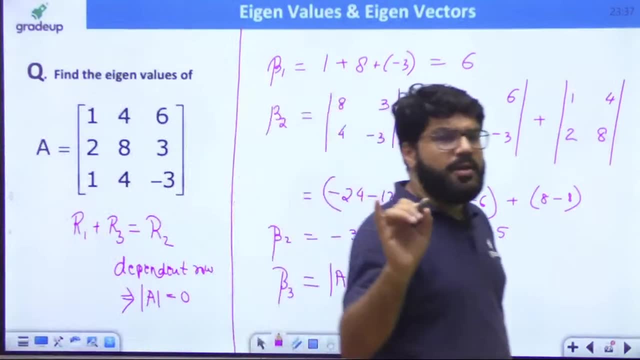 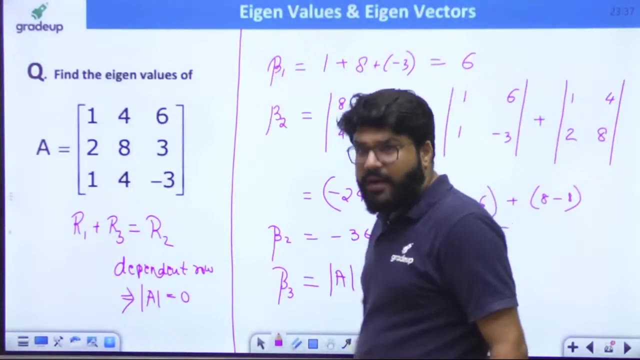 is a dependent rows, And whenever the rows of a matrix are dependent, its determinant is always 0.. Whenever the rows or the columns of a matrix are dependent to each other, then its determinant is 110% 0.. Okay, So let me write it as 0.. 110%- 0.. There is no doubt in that. So now coming to the 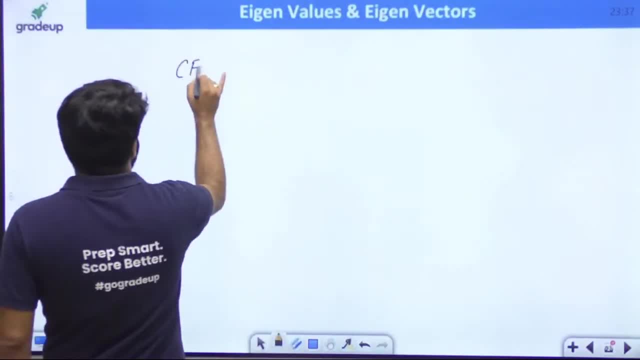 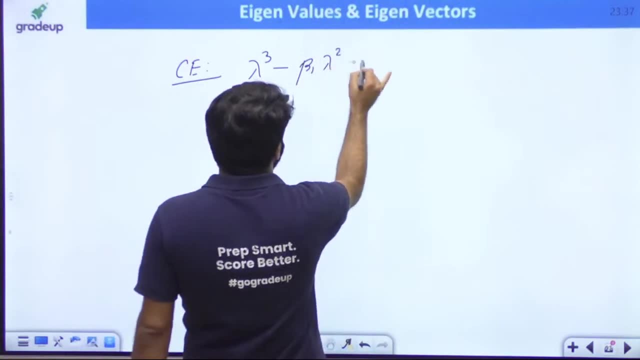 characteristic equation Coming to the characteristic equation Lambda cube. Direct characteristic equation for 3 cross 3.. Minus beta 1: lambda square, plus beta 2: lambda minus beta 3 equal to 0.. So I will write it as 3 cross 2.. And I will type it like this. So I will write it as: 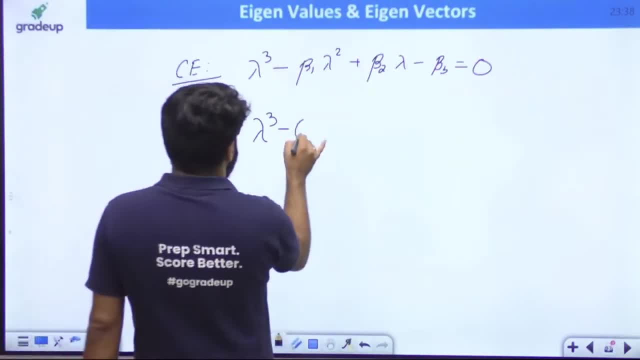 lambda square minus 1. lambda square plus beta 2. lambda minus beta 3 equal to 0.. So I will add up: have lambda cube minus beta 1, beta 1 is 6: 6. lambda square plus beta 2: lambda beta 2 is minus 45. 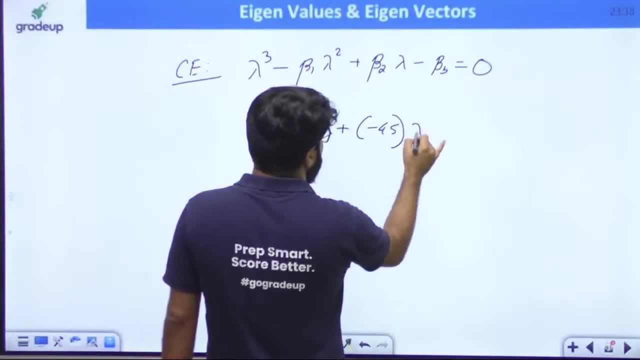 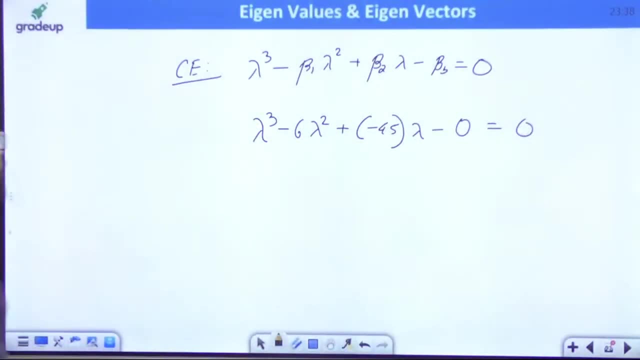 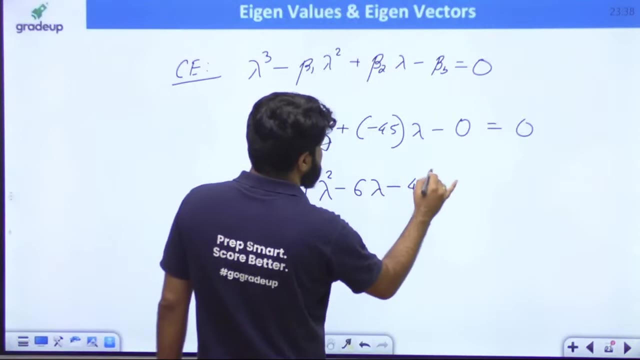 minus 45. lambda minus beta 3, that is minus 0 equal to 0. beta 3 stands to be 0, correct? so so only the first three terms are there. just may say lambda commonly are. so i have lambda square minus 6. lambda minus 45, equal to the 0, equal to the 0. so what is lambda? it is either. 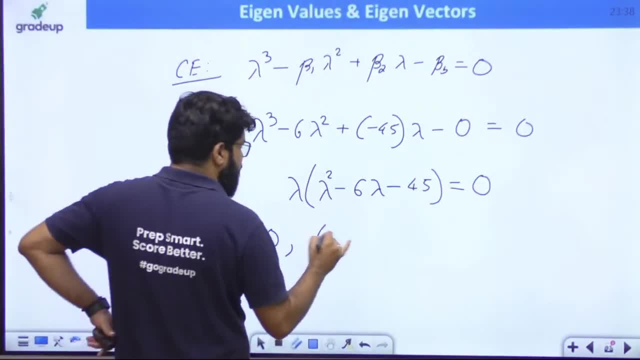 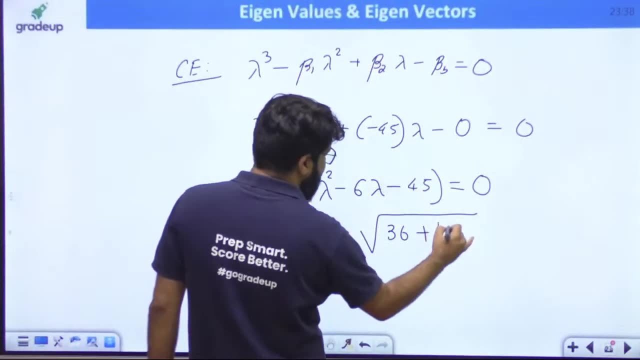 equal to 0 or the roots of this quadratic equation. the roots will be minus b plus minus root over b square, that is, 36 minus 4ac. the minus minus plus and 4 into 45 is 180 divided by 2a. so this lambda. 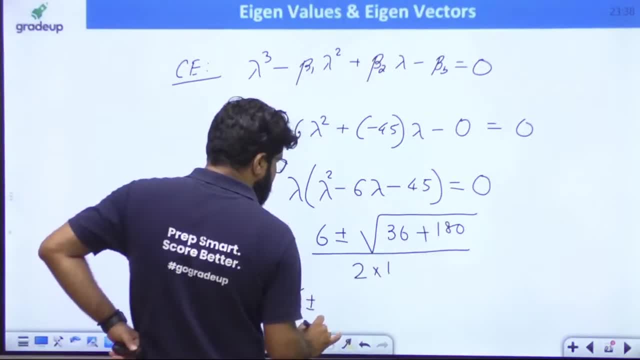 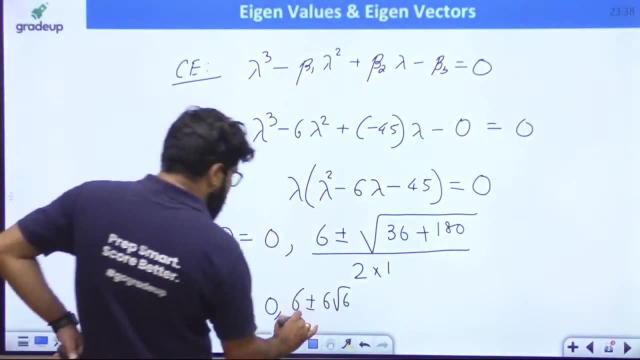 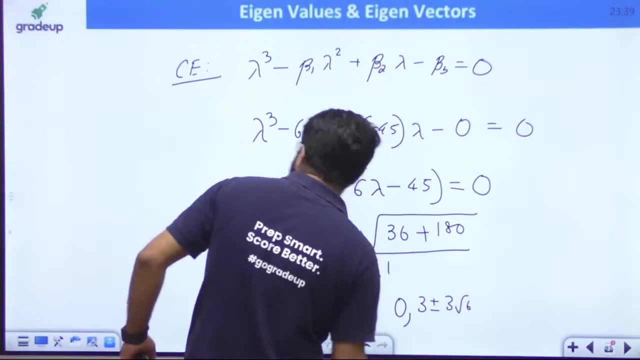 is 0 or 6 plus minus 180, plus 36, 216, 216, 6 cube is 6 cube, so 6 cube under root of 6 cube is 6 root 6. now this is divided by 2, so ultimately 0 and 3 plus minus 3 root 6. so what are the eigenvalues? 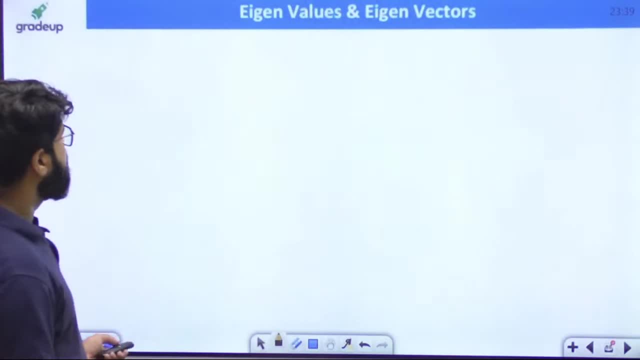 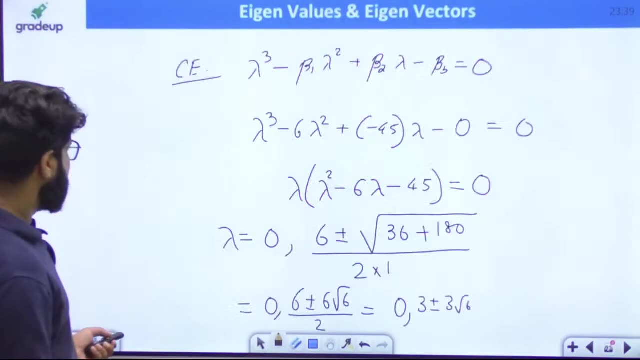 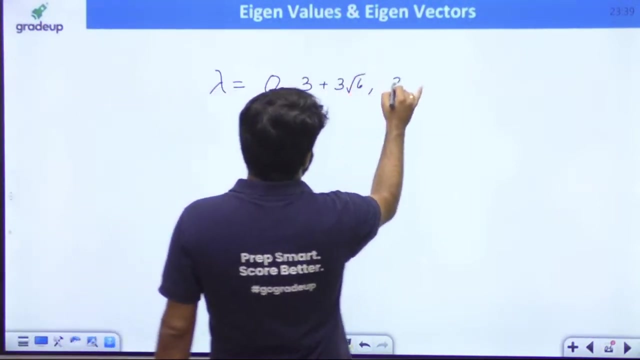 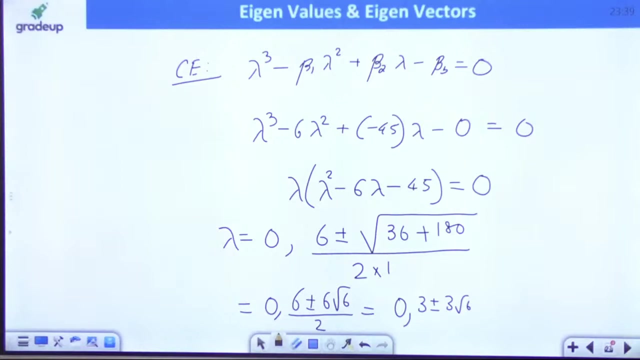 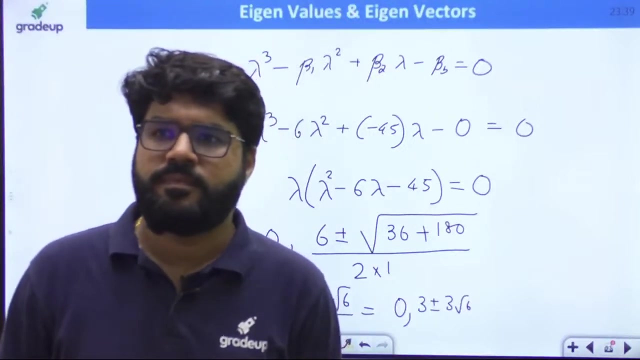 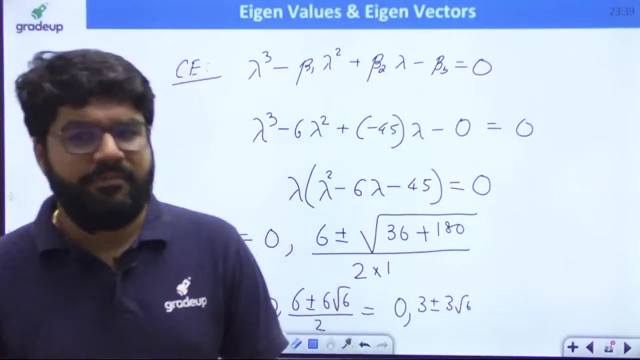 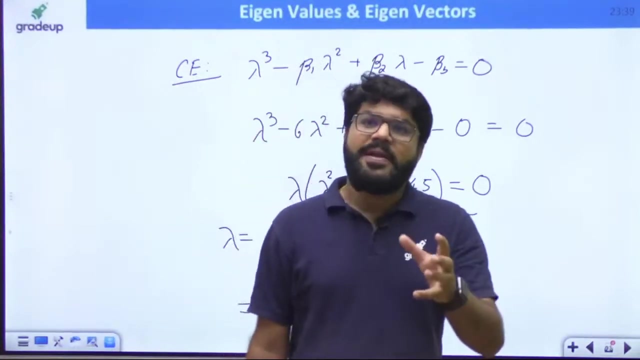 yes, so what are the eigenvalues? 0, 3 plus 3 root 6, 3 minus 3 root 6.. these are the three eigen values right right now. if you i have seen for n number of questions, this is much, much, much. because shortcut means not the final shortcut. the property are apply. over. so we will see with the properties if there is any. a minus lambda seem for n number medical and this is go to number of questions. this is much, much, much, because short cut means not a final short cut property, other apply per se. well, i will see with the properties if i will. 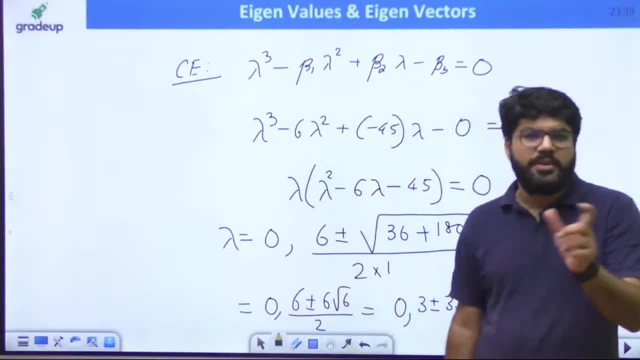 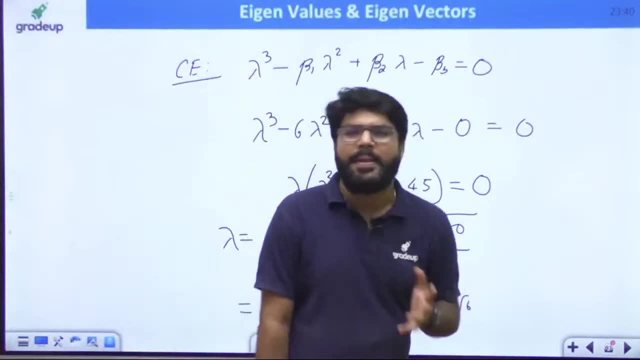 properties. If the question is like MCQ question, some of the questions will be MCQ. But if the questions are NET in nature, we must know this method when we need to solve all the eigenvalues compulsorily. But for MCQ questions, of course, properties we are going to see, and several. 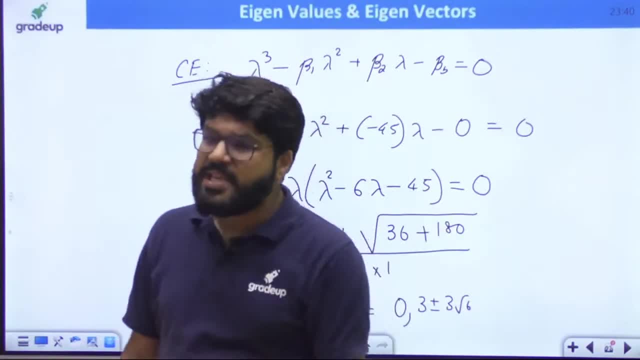 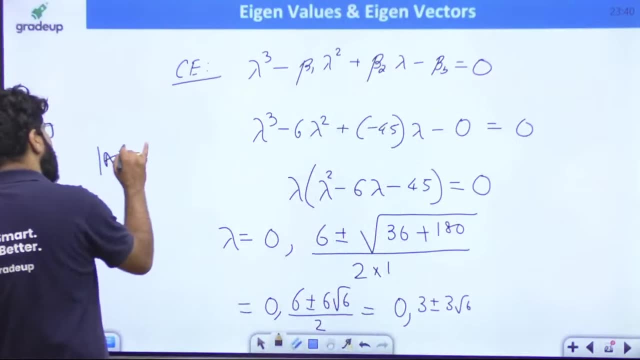 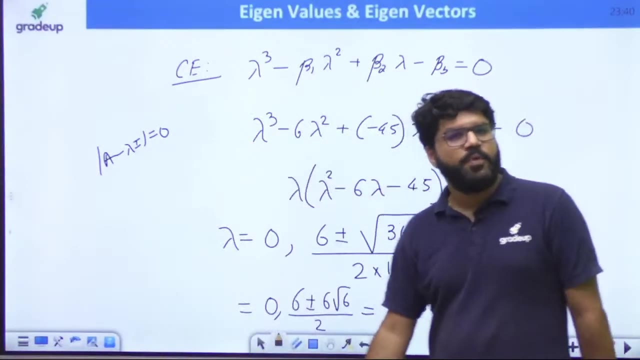 properties will make you solve the question in 10 seconds. But yes, if you actually want to find out all three eigenvalues, then directly solving modulus of A minus lambda I equal to 0, I think this is much better than the direct case Compared to this direct case, Pragya- Okay, At least. 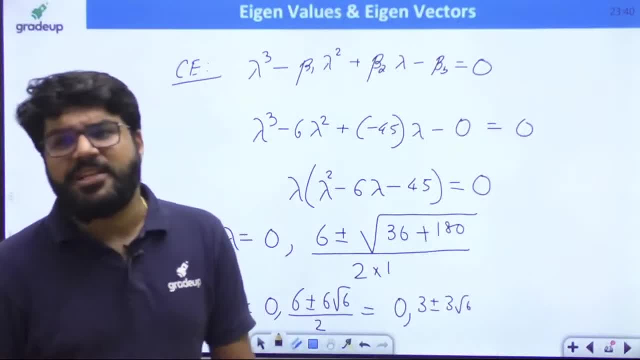 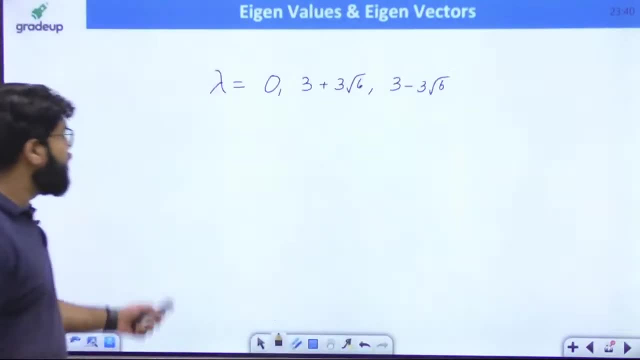 compared to this direct case, But there can be several questions where properties will help you. What properties and what indirect question? There are lots of questions. That is why two parts kept here. Okay, There will be a lot of questions. Let's take another case then. Okay, Let us practice. 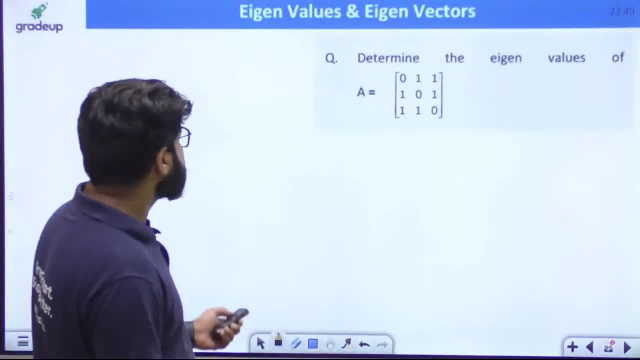 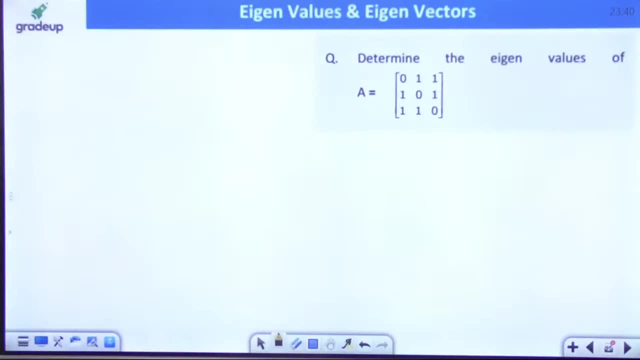 few direct questions and then let's go to the indirect questions. also Determine the eigenvalues of the matrix A: 0, 1, 1, 1, 0, 1 and 1, 1, 0.. Okay. 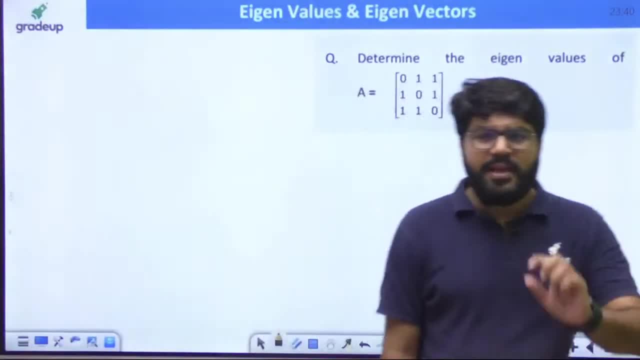 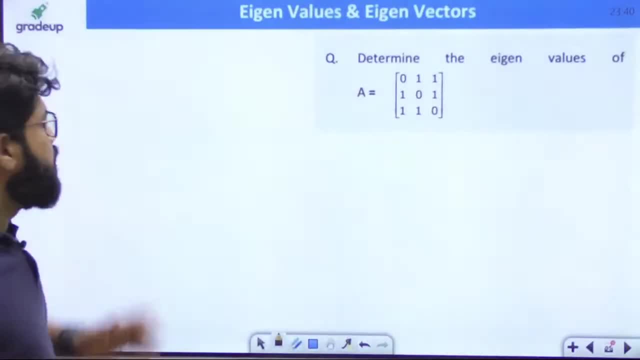 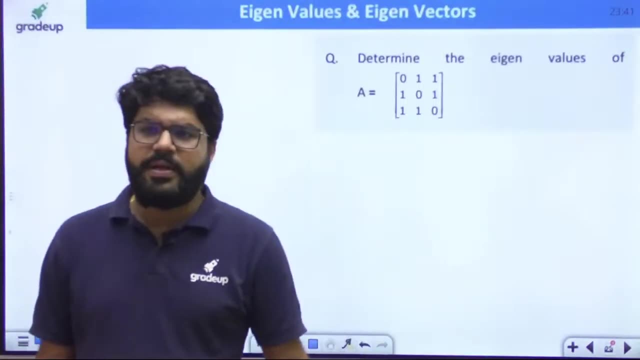 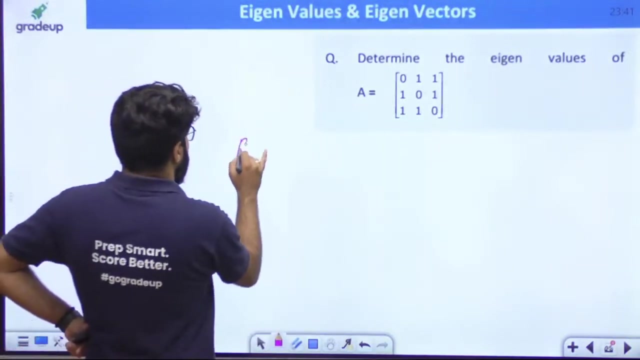 the properties and indirect questions. Okay, So once again, guys, if I take up beta 1, beta 2, beta 3.. If I take up beta 1,, beta 2, beta 3.. Right, Yes, Jignesh Chance hai. What is the beta 1?? 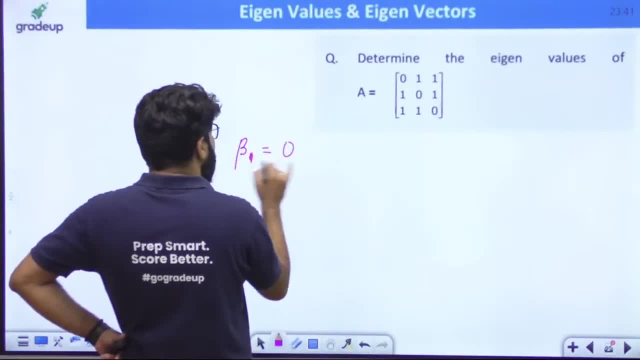 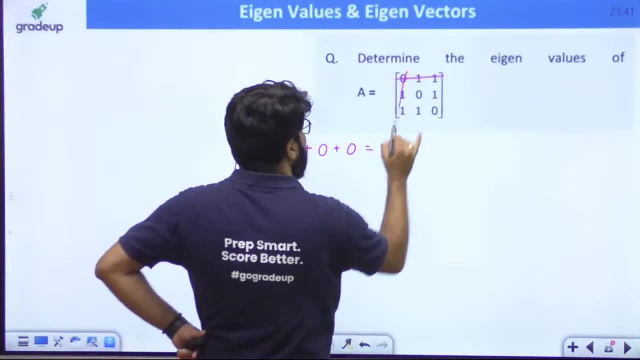 Trace. Okay, That is very simple actually, And I think beta calculation mein koi zyada time bhi nahi lagta, Koi zyada Khas time nahi lagta. This is 0. Beta 2. Sum of the minor: Toh pehla minor kitna hua. 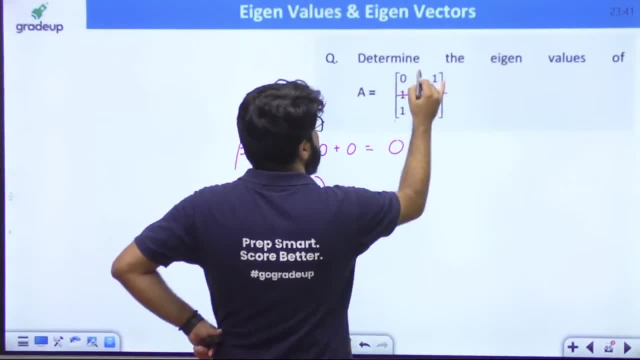 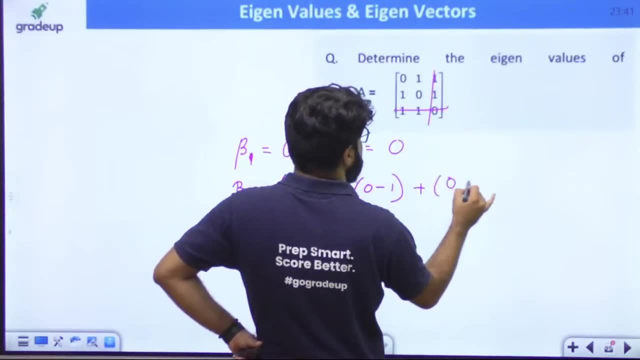 Directly, I am writing: 0, minus 1.. Next Second row, second column: delete kia 0, minus 1.. Next Third row, third column: delete kia. Toh, again 0, minus 1.. Okay, Then what is beta? 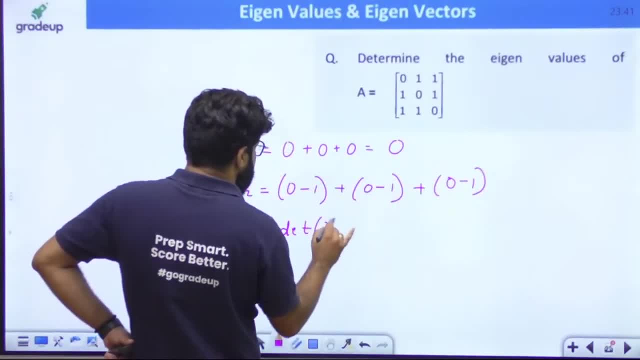 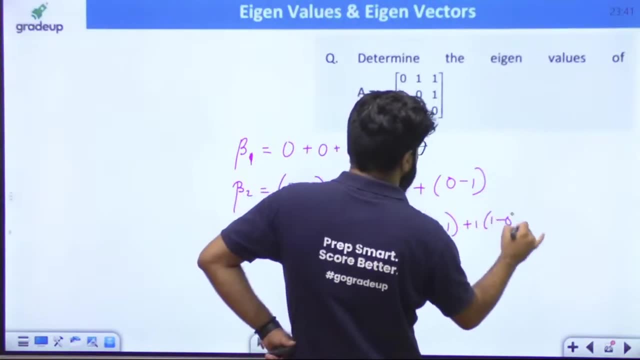 3?. Beta 3 is the determinant of the matrix hai and determinant First element is 0. Then minus 1.. 0, minus 1 and plus 1 into 1, minus 0. So eventually, minus 1, minus 1, plus 1 and plus 1, 2.. The determinant value is the 2.. 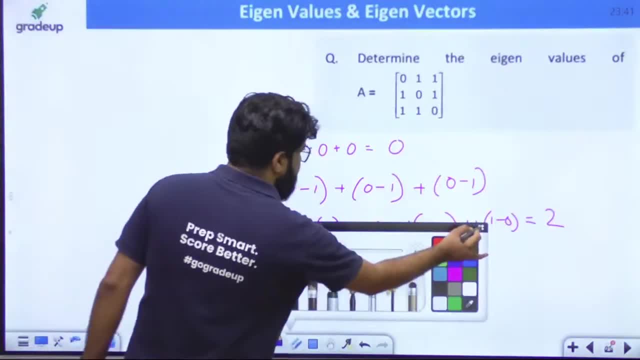 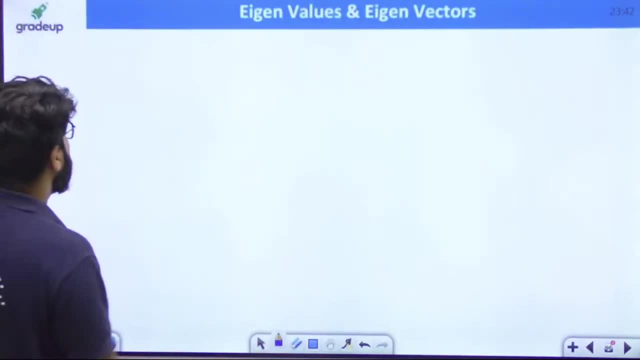 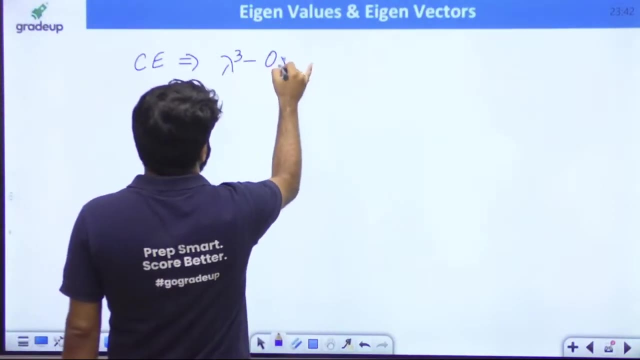 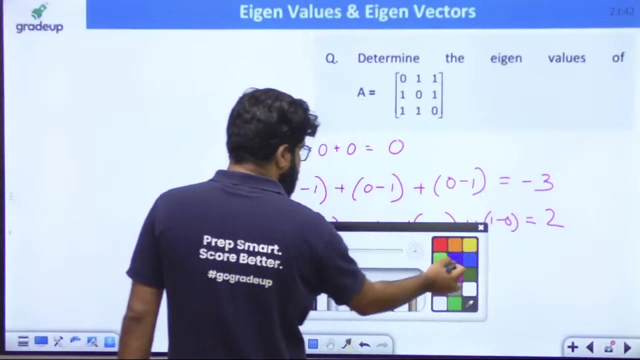 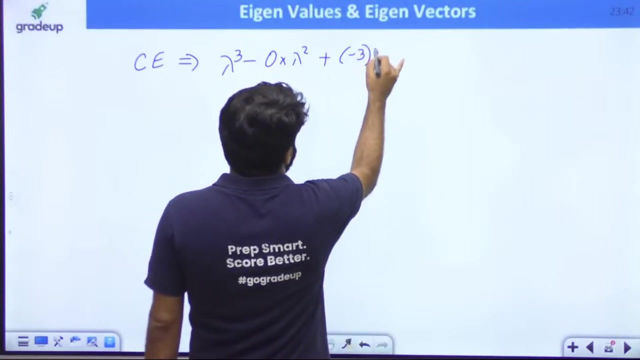 The determinant value is the 2.. Okay, So direct characteristic equation, guys. Direct characteristic equation: Lambda cube minus beta 1. lambda square plus beta 2. lambda Beta 2, kitna hua Minus 3.. So plus minus 3 lambda, Okay, Minus beta 3.. That is minus 2 equal to 0.. So you have. 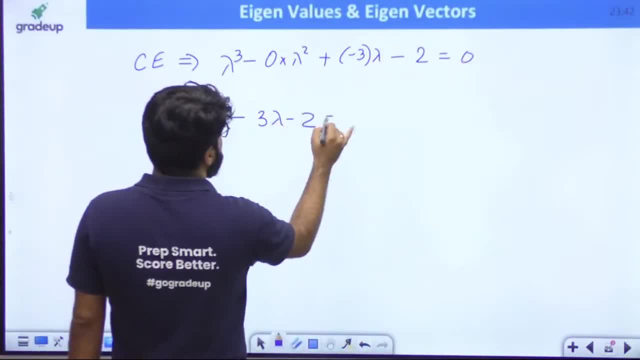 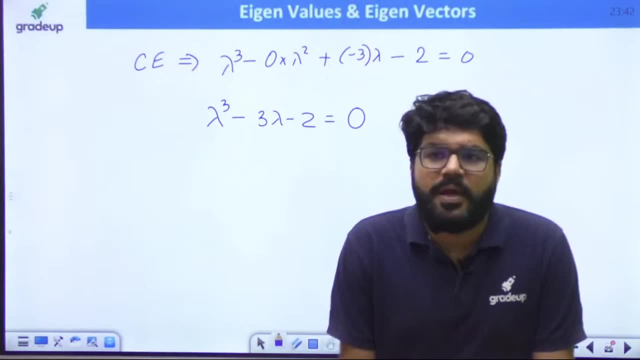 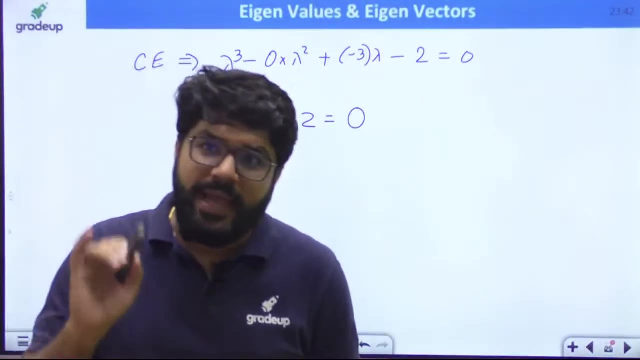 lambda, cube minus 3, lambda minus 2, equal to 0. and then you will say that, sir, this comes a cubic equation, Right, Thank you. thank you, Pathan. So there comes to be a cubic equation. Now, of course, we know that, since I am taking up the gate. 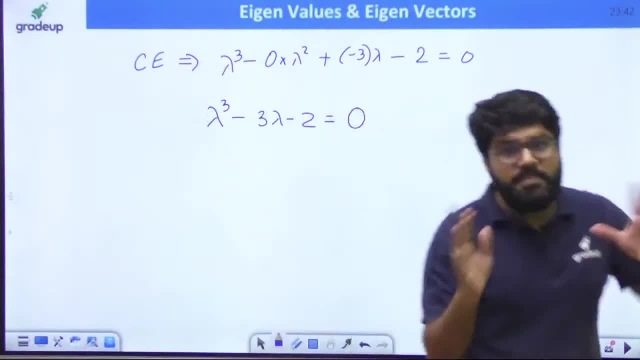 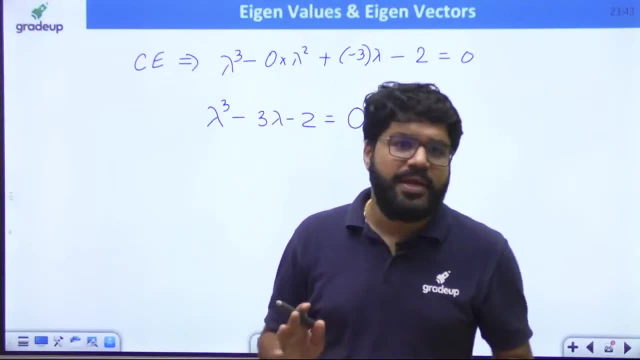 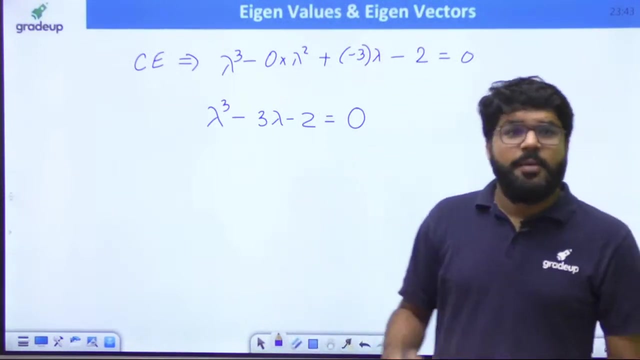 Questions relevant to the gate. There can be sometimes equations, Okay, There can be sometimes the equations which are cubic. I know scientific calculators are not allowed. Virtual calculator mein you cannot solve the cubic equation. If it is MCQ question then you can satisfy the option. But suppose it is a NET equation and I ask you: find the largest? 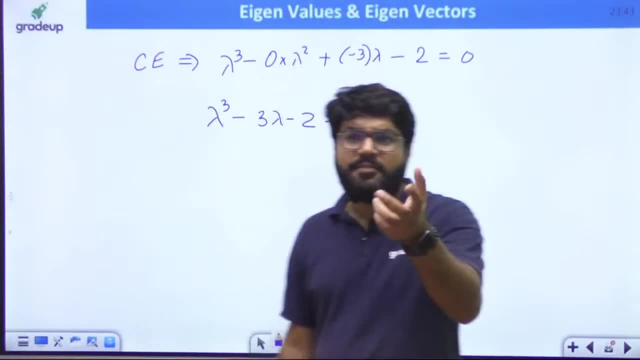 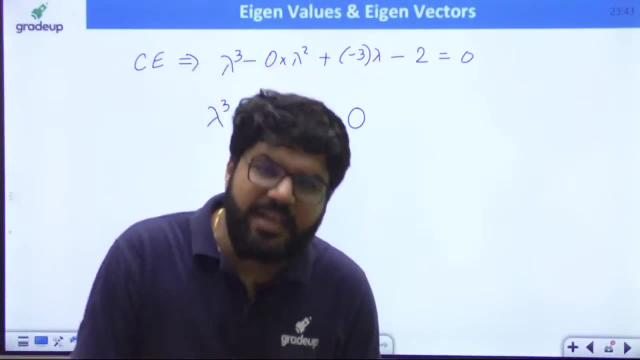 eigen value of this matrix. Question NET mein convert kar sakte hai. Find the largest eigenvalue of this matrix. Find the largest eigen value of this matrix. Find the largest eigen value of this matrix. Ya, find the smallest eigen value of this matrix, then what I am going? 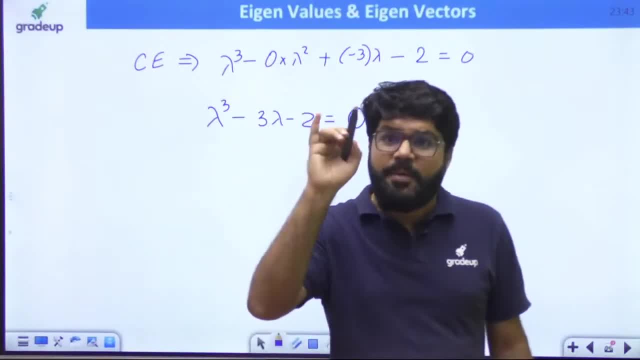 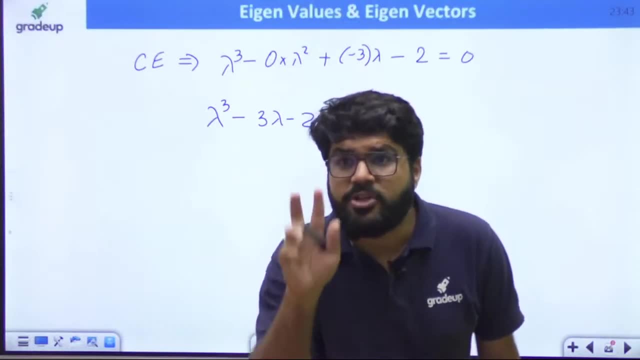 to do. Okay, So by chance, if you have a cubic equation, take my words, it will be a cubic equation which can be factorized. Now, it should not be 2 eigen value, Shivangi and Shiva, There should be 3 eigen value, 3 cross, 3 matrix. So, even by chance, cubic equation, aaya it. 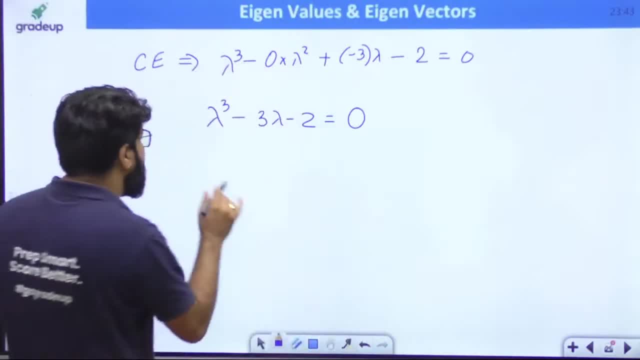 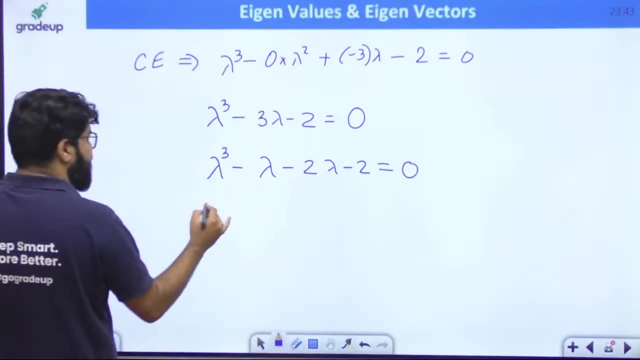 will be such a cubic equation that you can factorize up easily. Zaada complicated nahi hoga. How? Let's take lambda cube minus lambda minus 2, lambda minus 2 equal to 0. Thoda bahut lambda common. then i have lambda square minus 1 from here minus 2 common. so i am left with. 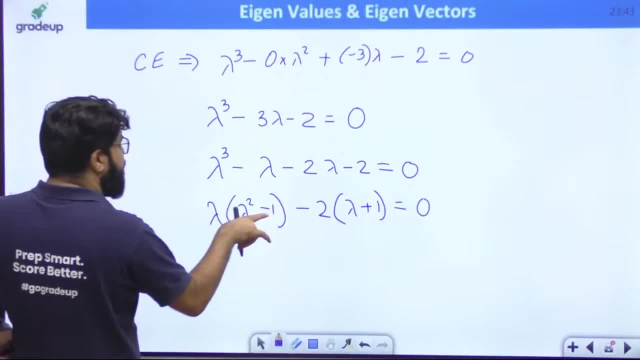 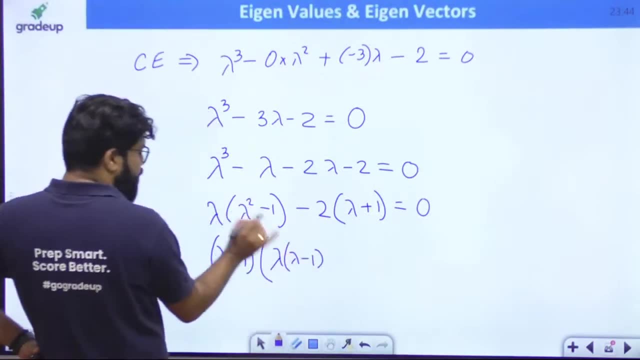 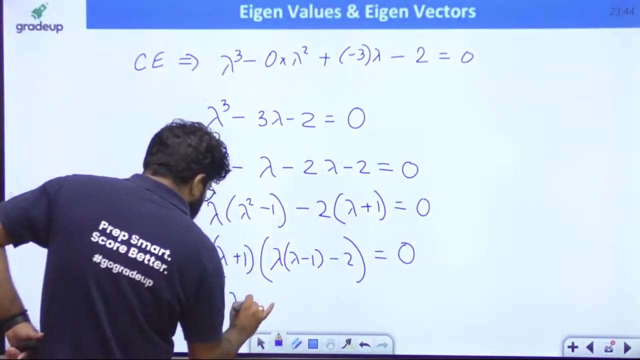 lambda plus 1, now lambda plus 1. this is also containing lambda plus 1, lambda minus 1. so lambda plus 1 is the common. then i have lambda here. lambda minus 1 will be left, minus 2 is left and equal to the 0, equal to the 0, right. so i have lambda plus 1 and then lambda square minus lambda. 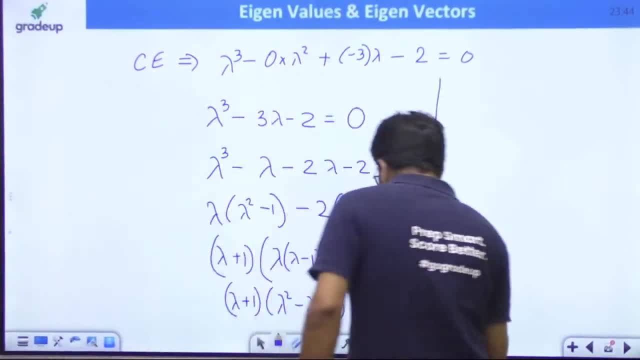 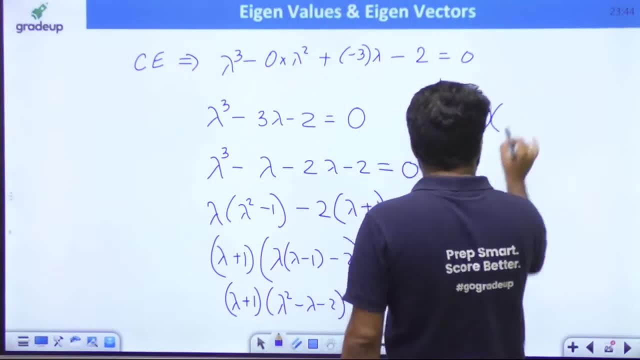 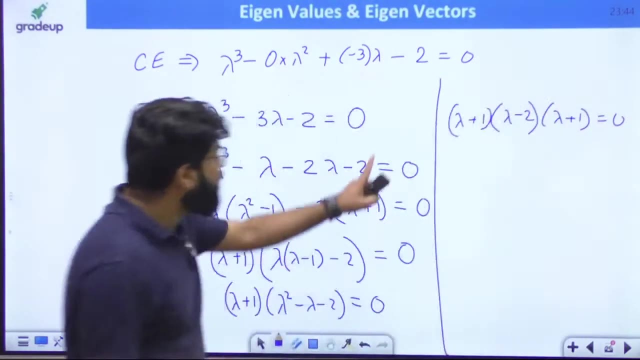 minus 2 equal to the 0. right then eventually i have lambda plus 1, lambda square minus. lambda minus 2. so i can factorize this as lambda minus 2. lambda plus 1. minus 2. plus 1 is minus 1 minus 2 into 1 will become minus 1. oh sorry, minus 2. so eventually lambda plus 1, whole square lambda. 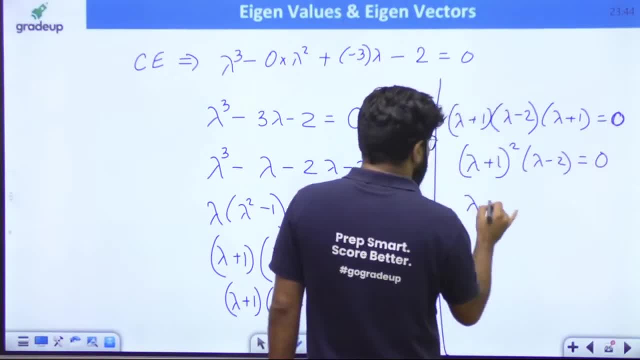 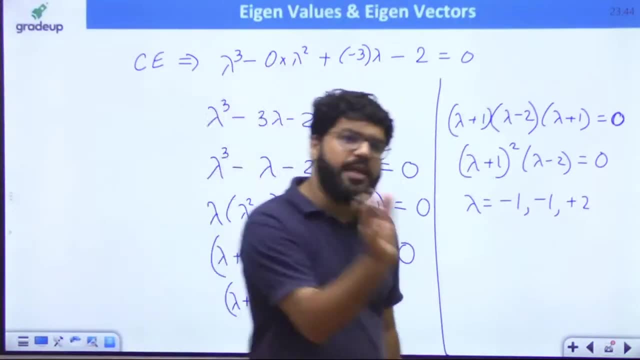 minus 2, they go factorize: okay, equal to 0, okay, so lambda is minus 1 minus 1 plus 2. so you must know this variety also. suppose by chance, if the cubic equation it will be a factorizable cubic equation, because even the iit knows that iit, kharagpur knows that you don't have 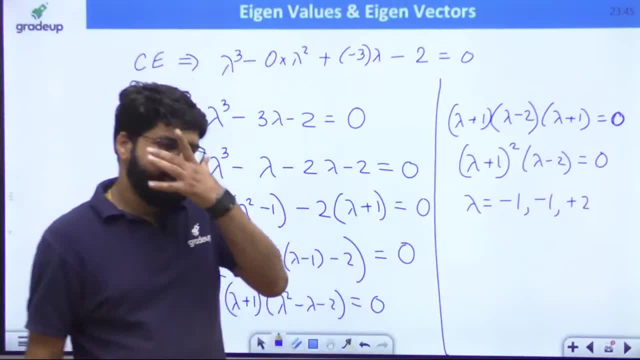 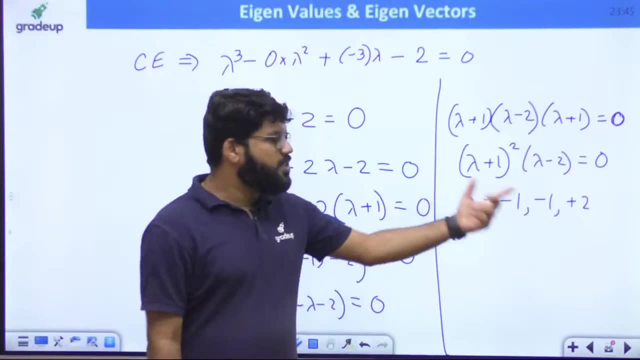 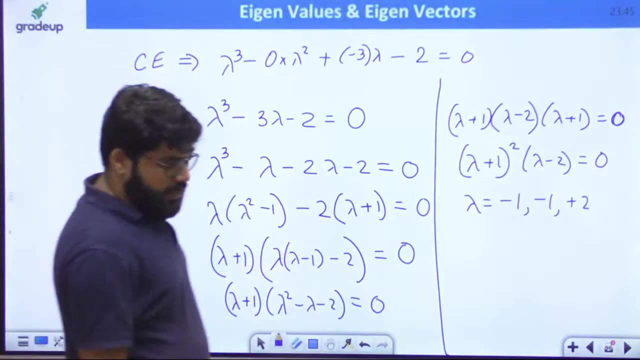 the scientific calculator. okay, minus one. but how many times minus one is coming pk. and what is the other one then okay? so that is why i just factorize it easily: minus one, minus one, two, right, thank you, pk. that's it. these are the three eigenvalues, that's, it's all. 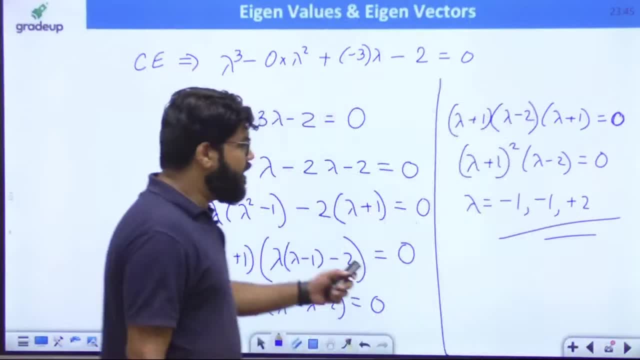 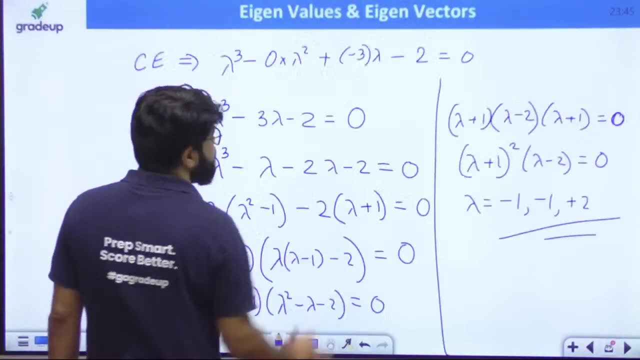 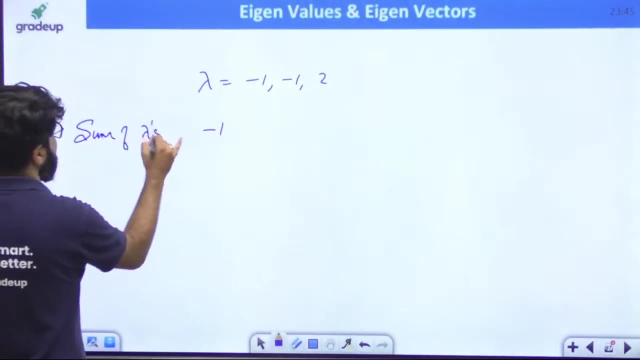 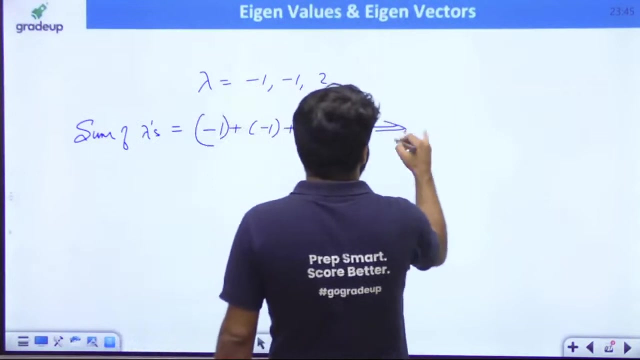 now very, very, very, very important observation, very, very important observation: lambda is minus one, minus one and plus two. what is the sum of lambdas? what is the sum of the lambdas minus one plus minus one, plus two is zero and that is actually equal to the trace of the matrix, if you have a look at the trace also. 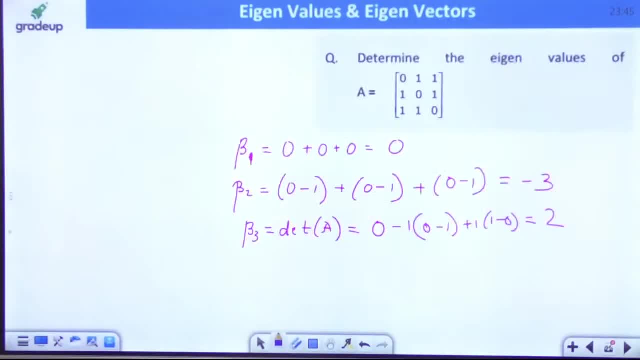 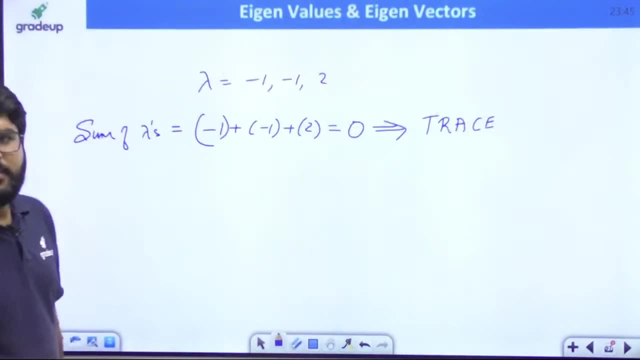 yeah, where is the question gone here? the trace is zero, beta one, that is, the trace of the matrix, is also zero, right? take it then. then, what is the product of eigenvalues? what is the product of the lambdas that is equal to, that is equal to how much? minus one into minus one, into two, and 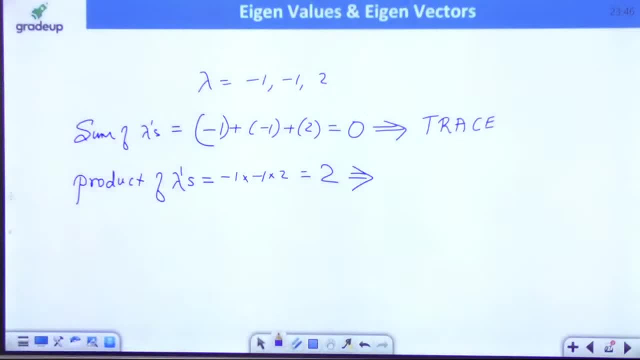 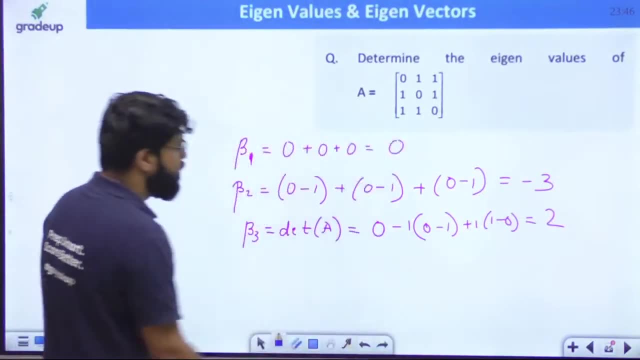 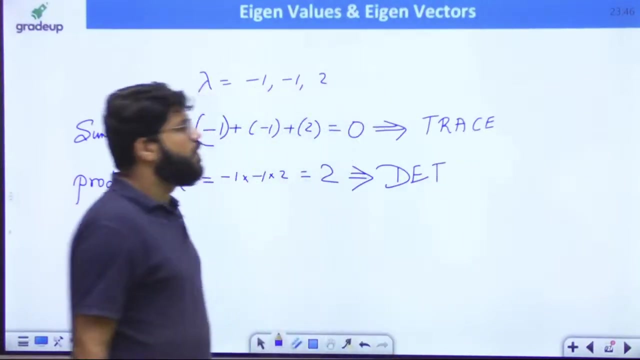 that is equal to two, that is equal to what that is equal to two, and this two is nothing. this two is the determinant of a correct. this two is known as the determinant of a right. not only for this question. not only for this question. this is always true. you can go. 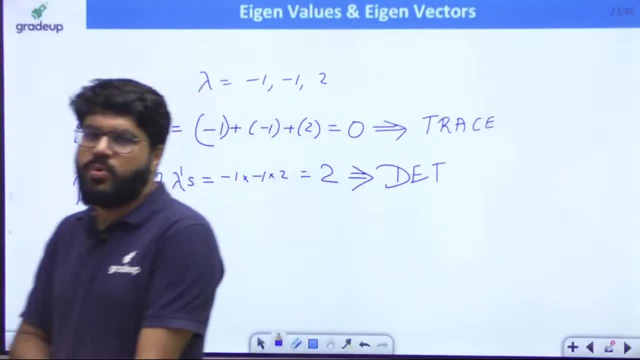 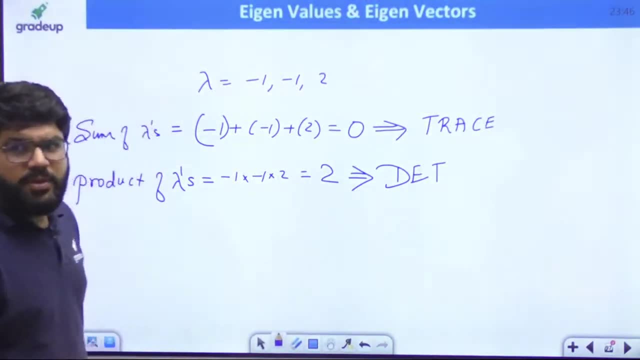 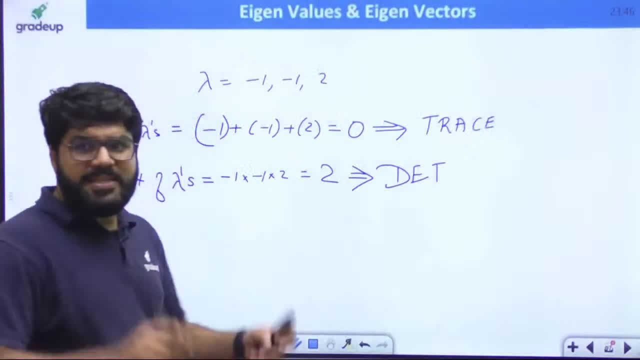 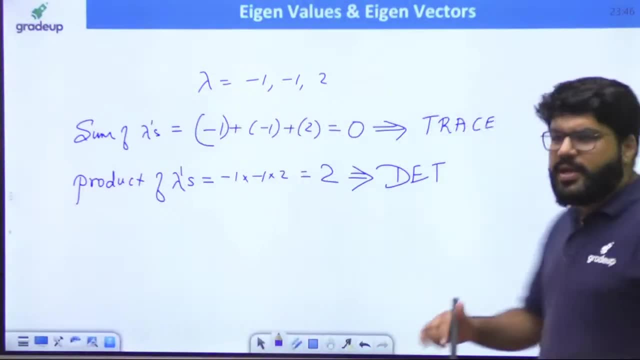 so we'll go to these properties. we'll go to these properties, but we will go to the properties and, but we will go to the properties and we will see all possible properties coming up here. we will see all property possible properties coming up here. okay, so let's go step by step. let's go to: 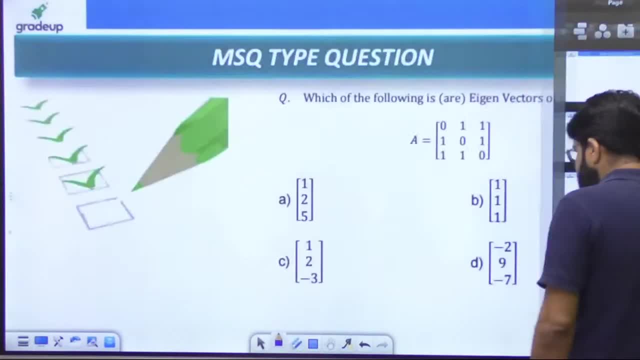 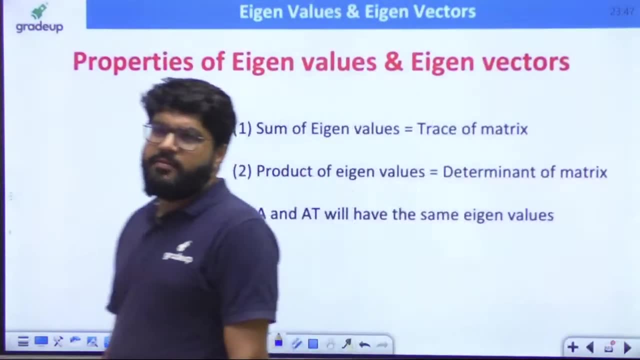 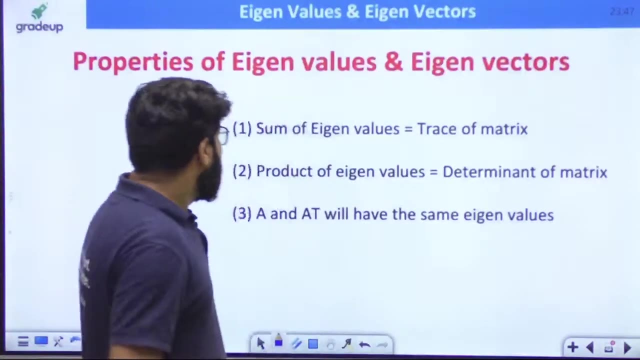 step by step to the properties. we will come to this question a little later. property is properties of eigenvalues and eigenvectors. eigenvector ka question. we will be taking eigenvector ka question. we will be taking eigenvector question also. okay, sum of eigenvalues is equal to the trace of the matrix, always, and product of eigen values. 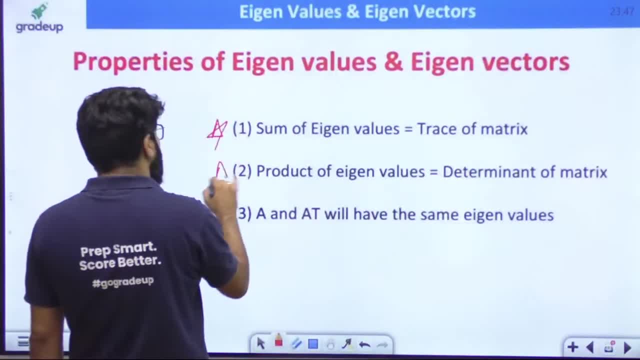 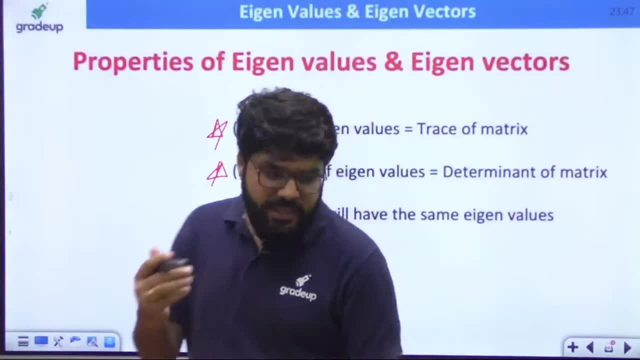 is always equal to the determinant of the matrix, and this two are the most simplest- you can say most simplest- and also the most expected properties which will appear on the questions you can expect, the questions that can be directly solved by this. what questions we will cover on this? 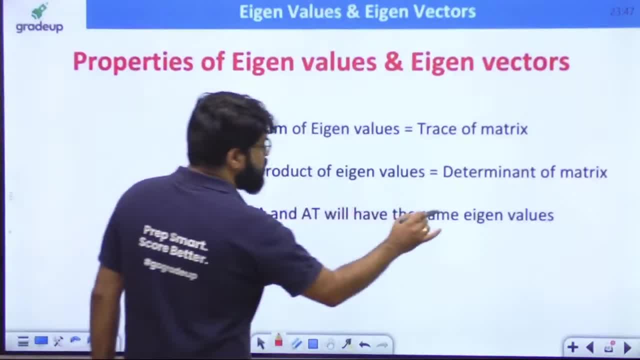 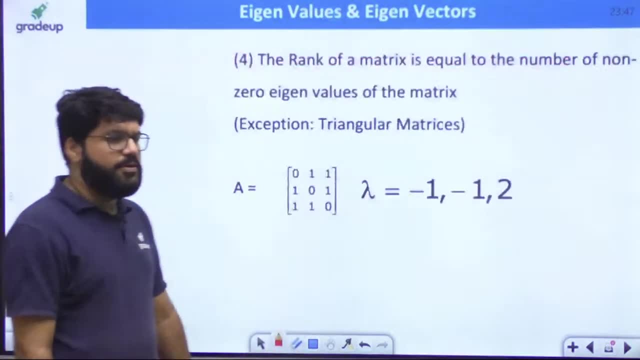 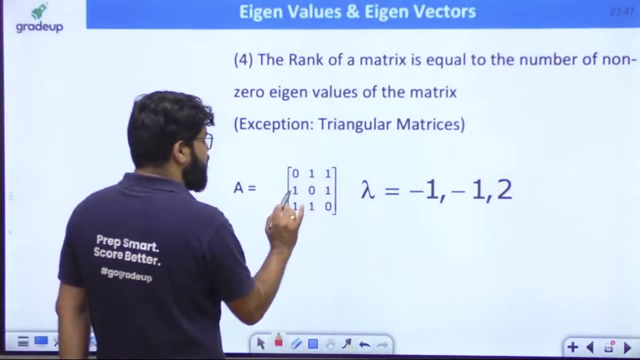 the all questions also. Okay, A and A transpose will always have the same eigenvalues. Right, A and A transpose will always have the same eigenvalues. Okay, The rank of a matrix. Have a look at the same matrix, The same example, just we solved The matrix. A was 0, 1 1, 1, 0, 1, 1, 1 0 and. 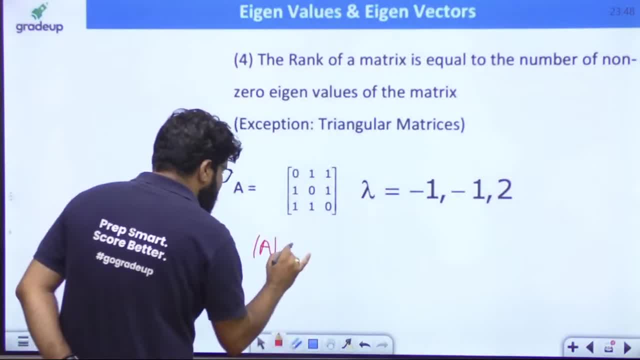 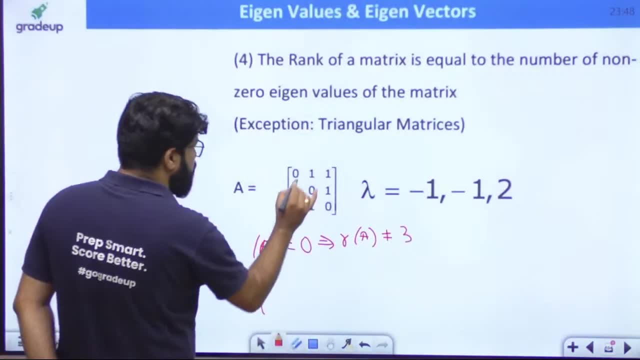 lambda is minus 1 minus 1 minus 2. We check that the determinant of the matrix is 0. So of course, if the determinant is 0, rank is not equal to 3.. Okay, But then I will check a 2 cross 2. 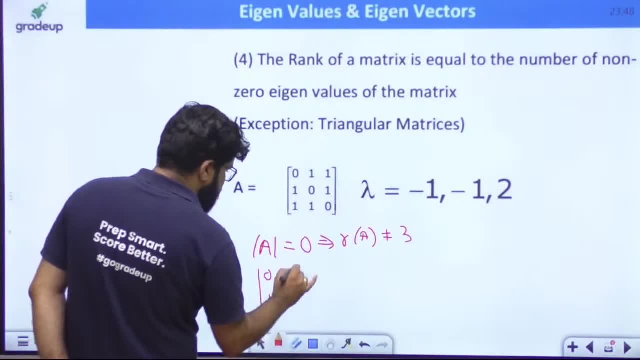 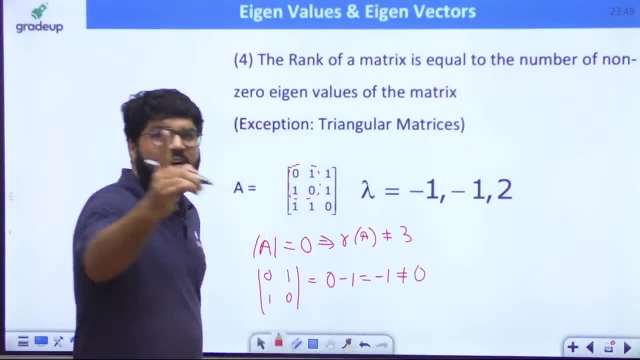 minor: 0, 1 0 0, 1, 1 0.. Let me test this: 2 cross 2 minor. Okay, And this is 0 minus 1, which is minus 1, non-zero. And if I have a 2 cross 2 minor, which is non-zero, If I have a 2 cross 2 minor. 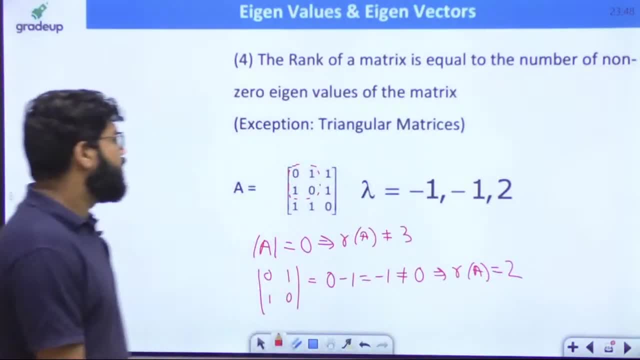 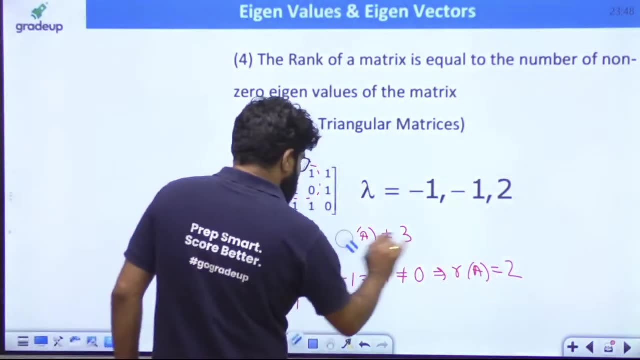 which is non-zero. So the rank will be 2.. So the rank will be equal to 2.. Okay, The rank will be equal to 2.. Sorry, I took the wrong data, I think. sorry. The determinant of this matrix is 0. So the rank will be equal to 2.. Okay, The rank will be equal to 2.. Sorry. 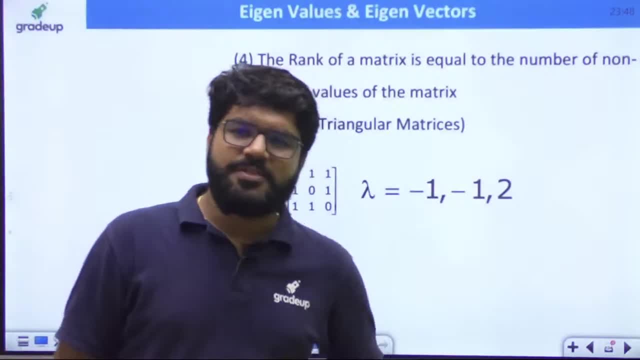 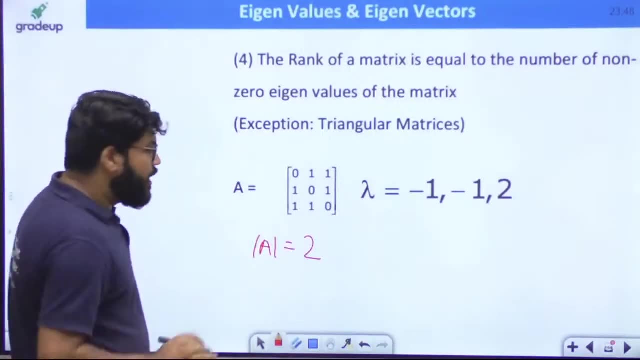 The determinant of this matrix was actually equal to 2.. The determinant of this matrix was actually equal to 2.. Okay, Now the determinant was equal to 2.. Just now we calculated Determinant if non-zero is there. If the determinant of a non-square matrix is non-zero, 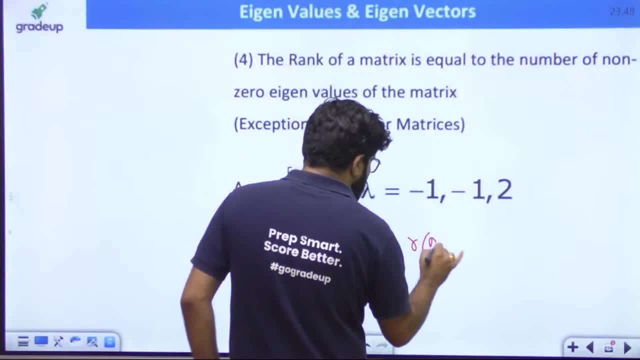 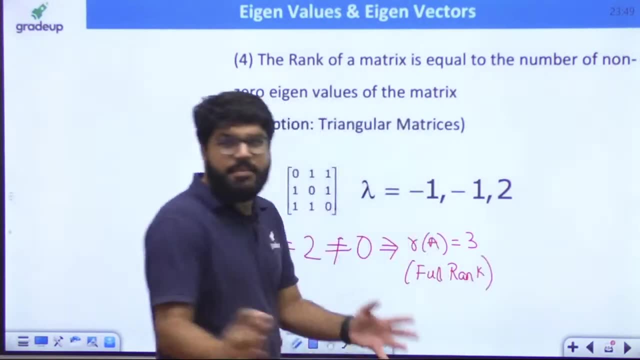 then we should know that, then we should know that the rank of the matrix is full rank. This is the full rank case. Full rank means maximum possible rank. And what is the maximum possible rank for a 3 cross 3 matrix? Sir, it is equal to 0.. So the rank of the matrix is 0.. So the rank of the matrix? 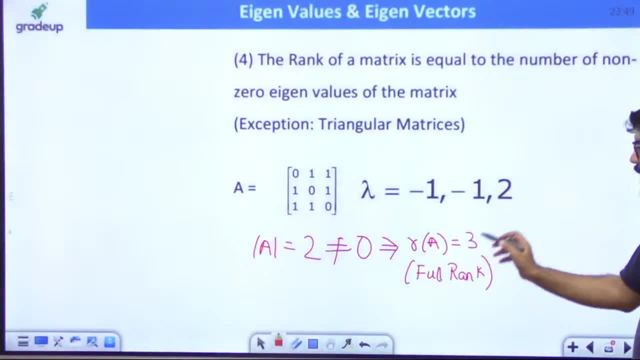 is equal to 3.. Right, Sir, it is equal to 3.. So I have full rank that is equal to the 3.. And now see the relation of the rank with the eigenvalue Rank. already we have discussed some questions in the 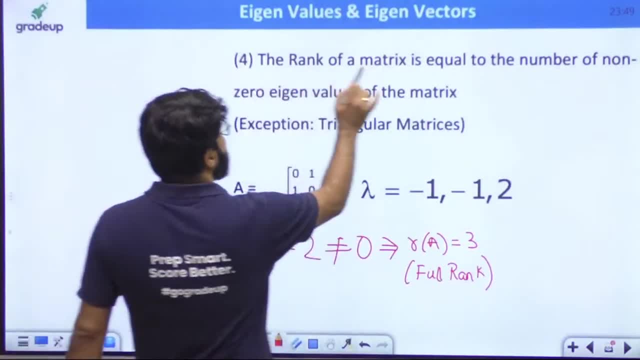 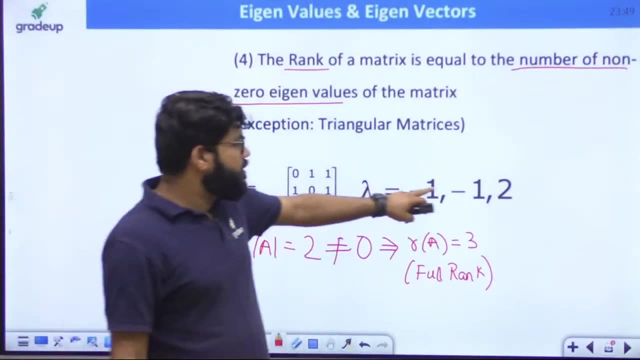 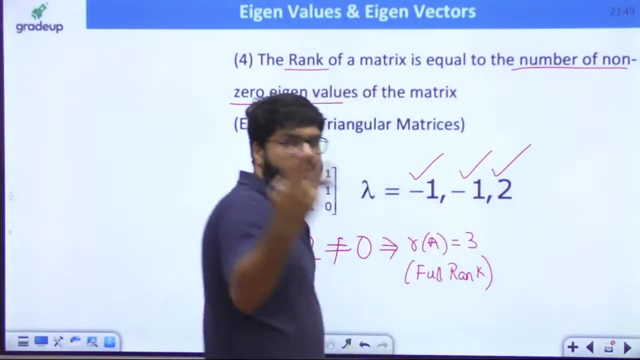 earlier classes. But rank relation with eigenvalue. Rank of a matrix is equal to number of non-zero eigenvalues of the matrix. Now this eigenvalues are 3.. There are 3 eigenvalues, But how many are non-zero, Sir? this is non-zero. This is non-zero. This is non-zero. All 3 are non-zeros. All 3 are. 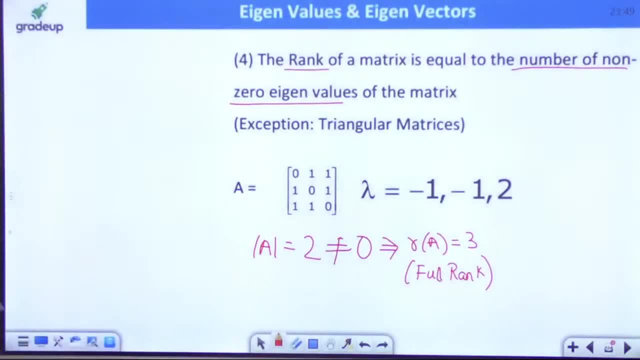 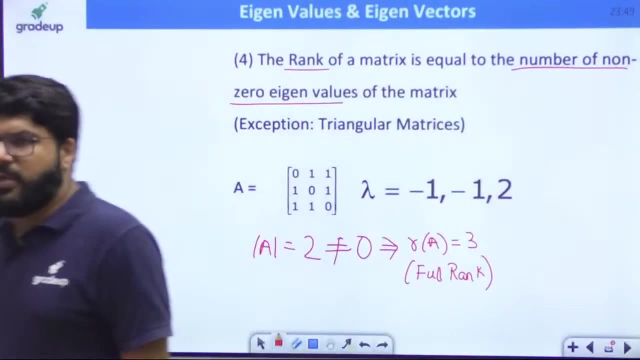 non-zero eigenvalues. Ok, So that is why the matrix rank is also equal to 3.. 3 non-zero eigenvalues and the rank is also equal to the 3.. The rank is also equal to the 3. Everybody, Ok, Right, Not the. 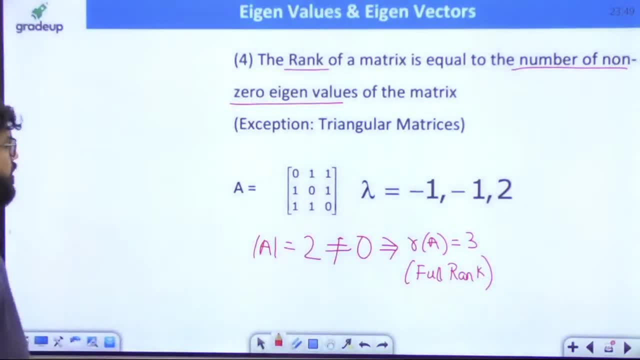 order of the matrix. Rank is equal to number of non-zero eigenvalues of the matrix. Only one exception to the property can be triangular matrices. Ok, But what is the rule for triangular matrices? See this: What is the rule for triangular matrices? See this: What is the rule for triangular? 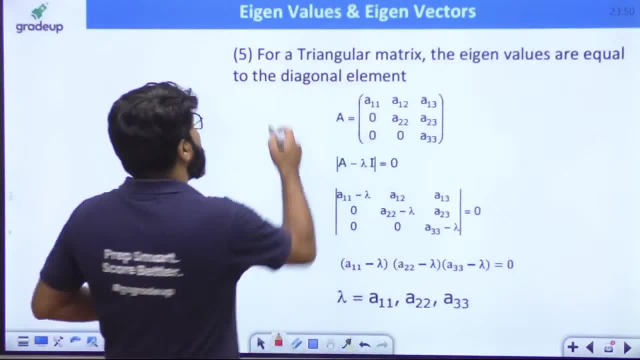 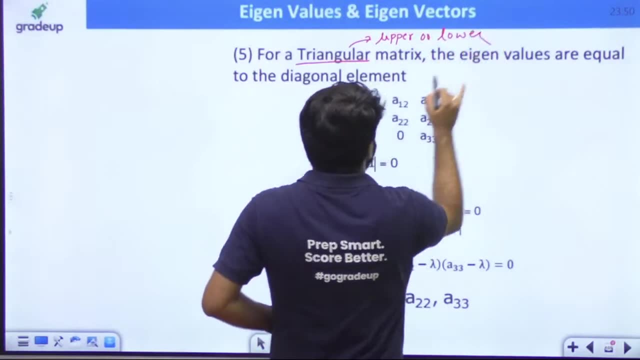 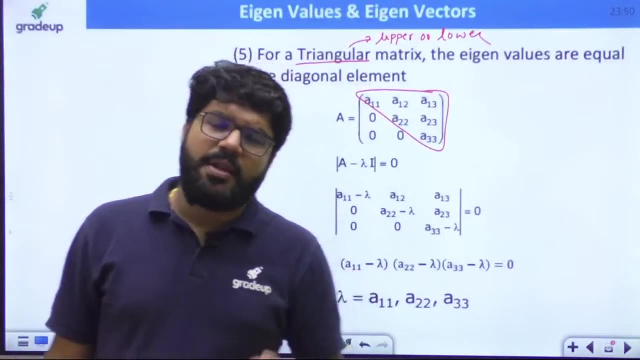 matrices. It is very simple: Given any triangular matrix, upper or lower, Whenever I say triangular matrix, it could be upper or lower, Any category. Look into this. Here I have taken a upper triangular matrix. Ok, The eigenvalues of a upper triangular matrix is directly equal to the. 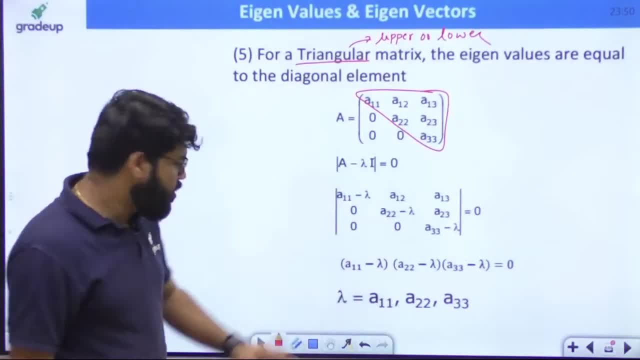 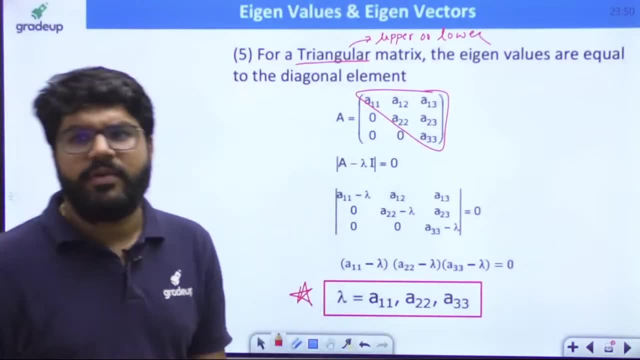 diagonal elements. Ok, You can see this description, But that is directly equal to the diagonal element. Ok, Whatever may be the order of the matrix, Guys, Whatever may be the order of the matrix, Ok, So basically the fig is the eigenvalue. Ok, Yes, yes, yes, SGK. Repetition no. 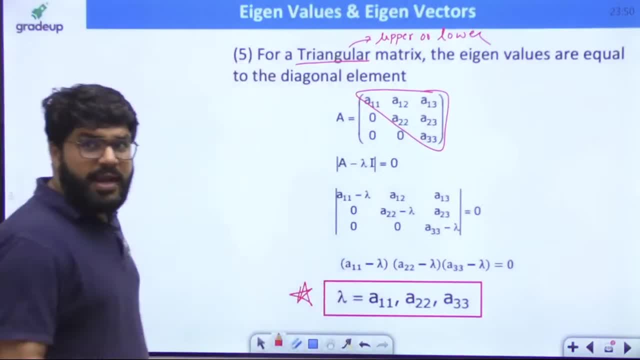 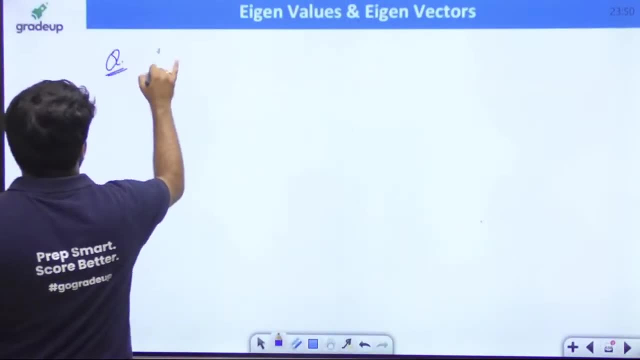 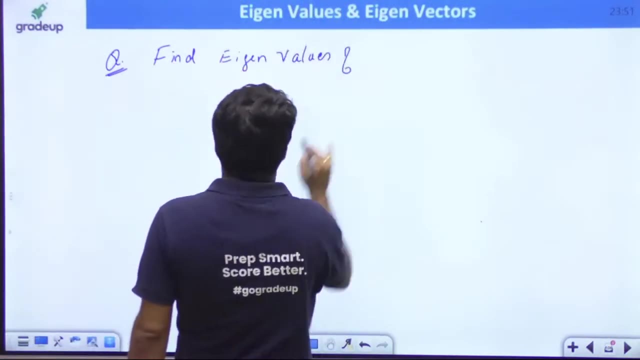 repetition: Non-zero eigenvalues need to be seen for rank Ok, For rank Non-zero, Whether it is repeated or not, Ok Say, for example: you know, if I give you a question here, Find the eigenvalues of, Find the eigenvalues of. Now sometimes you know you may see a big. 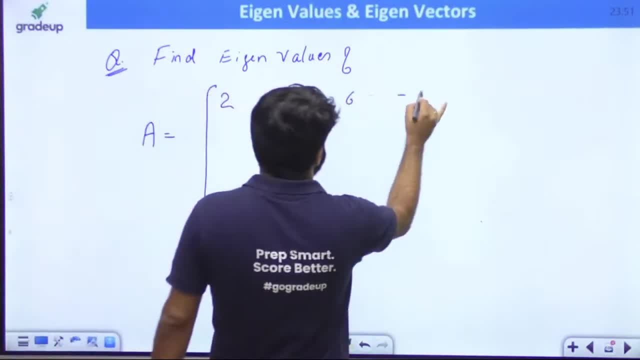 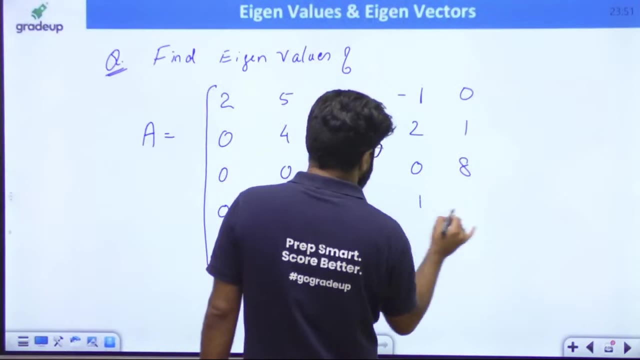 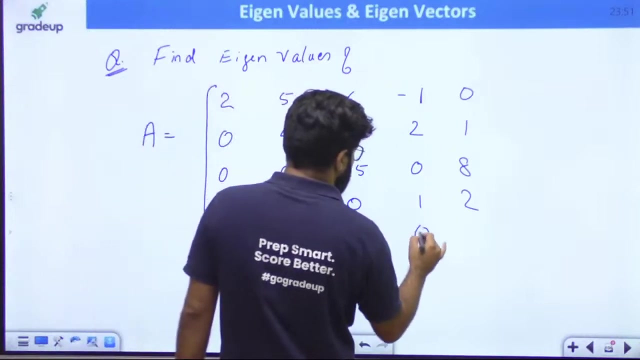 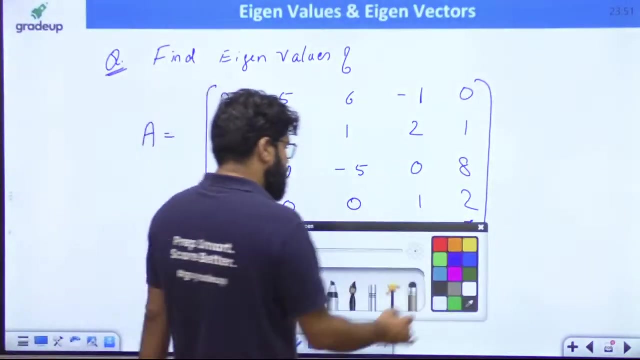 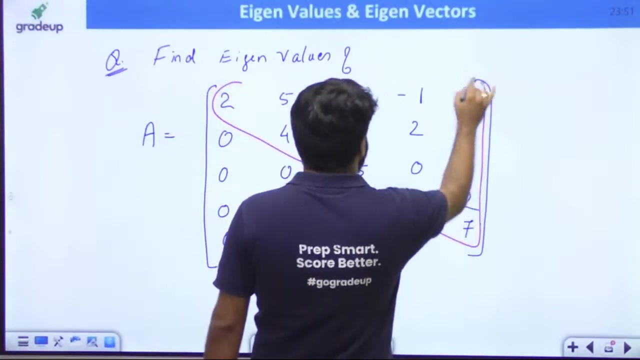 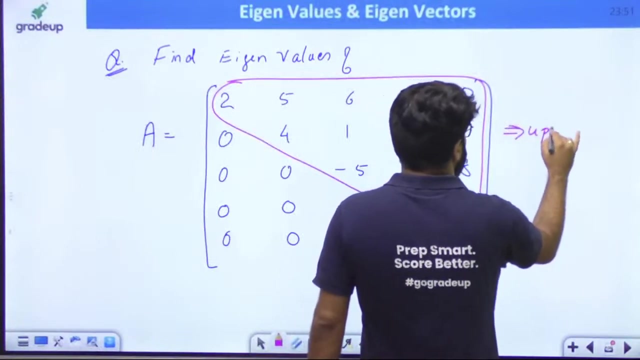 question which has been asked by the people. Which question is this? Tell me what is given. Have a look into this. have a look into this. so what should be, what should be this matrix? what should be this matrix? this is clearly a upper triangular matrix. this is the upper triangular matrix. so 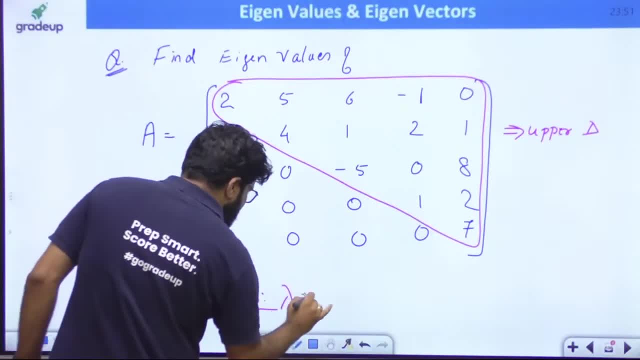 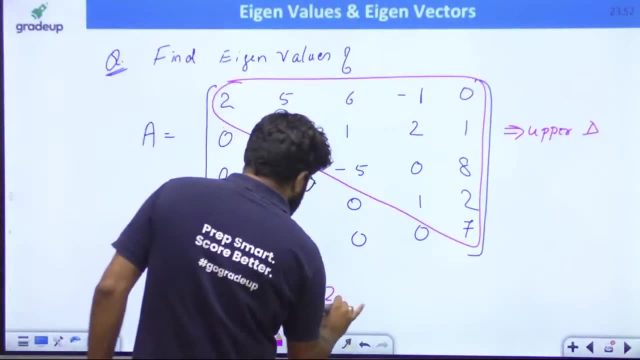 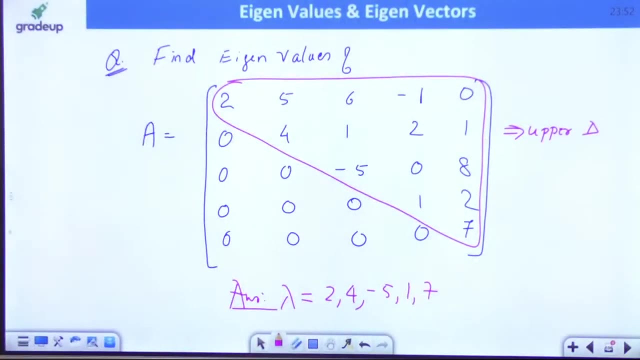 what are the eigenvalues? answer is in front of you. only. the eigenvalues of any triangular matrix are always equal to the diagonal numbers, or always equal to the diagonal numbers 2 and 4 and minus 5, and 1 and 7, 2, 4 minus 5, 1, 7, 2 4 minus 5, 1, 7. that's it simple so. 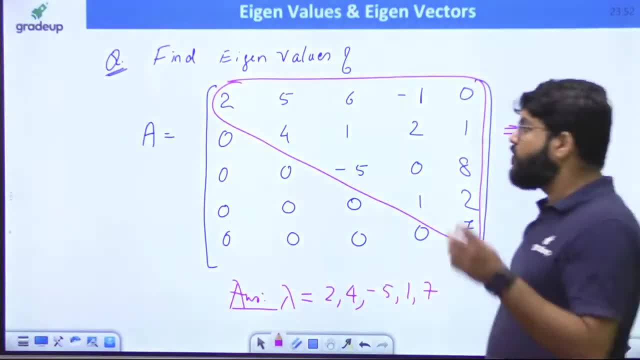 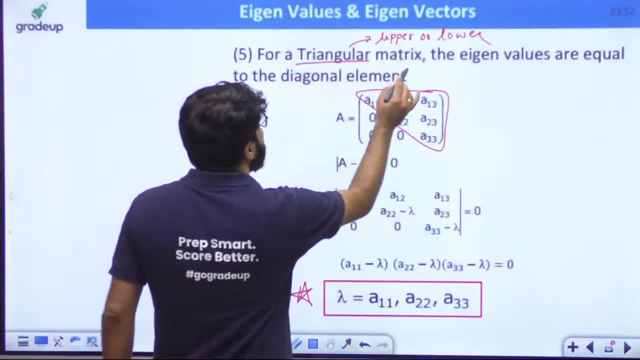 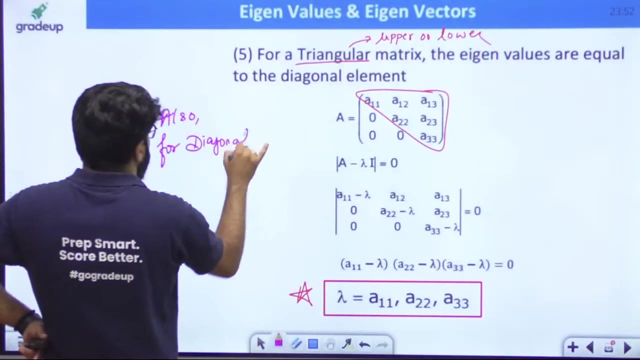 whether it is 3 cross 3, 4 cross 4, 5 cross 5, any type of triangular matrix. okay, eigenvalues are diagonal, are equal to diagonal elements and not only triangular matrix. this should also be applicable for a diagonal matrix. this is also applicable for a diagonal matrix. this is also applicable for a diagonal matrix. this is: 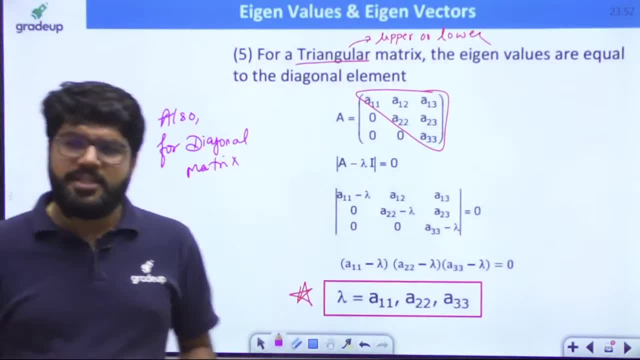 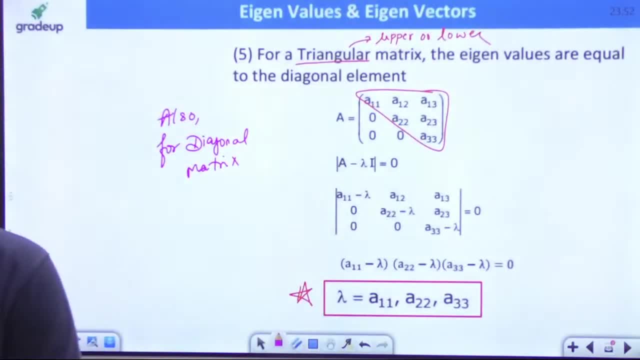 just a special case, okay, special case of this. haha, PK, I'm gay, what question you this? haha, PK, I'm gay. what question you this? haha, PK, I'm gay, what question you are. the frame of 5 cross 5 car question. are the frame of 5 cross 5 car question? 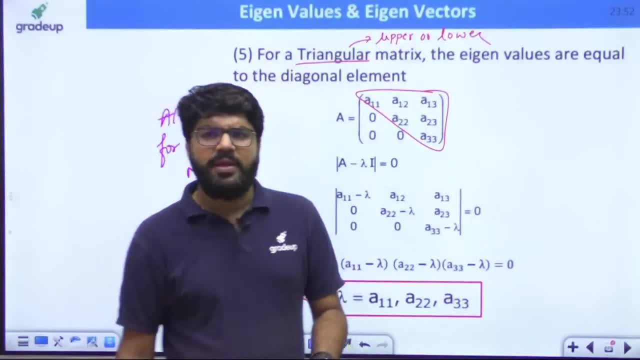 are the frame of 5 cross 5 car question: hey gate miss simple, a very simple. hey gate miss simple, a very simple. hey gate miss simple, a very simple. properties case are dying, I don't worry. properties case are dying, I don't worry. properties case are dying, I don't worry. PK: 3 cross, 3 key maximum eigenvalue: 5 cross. 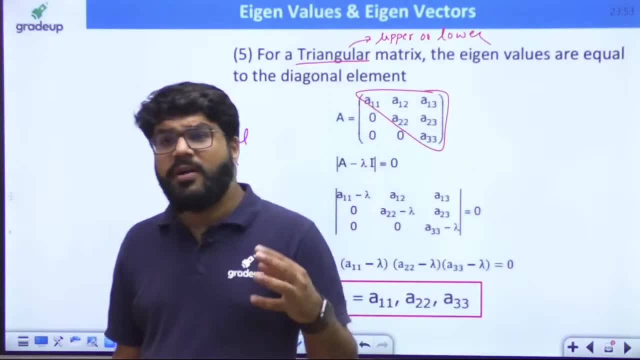 PK 3 cross 3 key maximum eigenvalue. 5 cross PK 3 cross 3 key maximum eigenvalue. 5 cross 5 eigenvalue. so they are all related with 5 eigenvalue. so they are all related with 5 eigenvalue. so they are all related with the trick. so we'll cover up some. 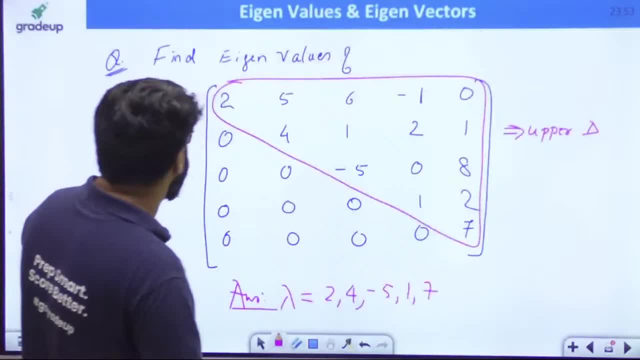 the trick, so we'll cover up some the trick. so we'll cover up some properties and then go all the questions properties and then go all the questions properties and then go all the questions with the king and most probably with the king, and most probably with the king and most probably Kalta Kapoor a time. I'm a repass now. next. 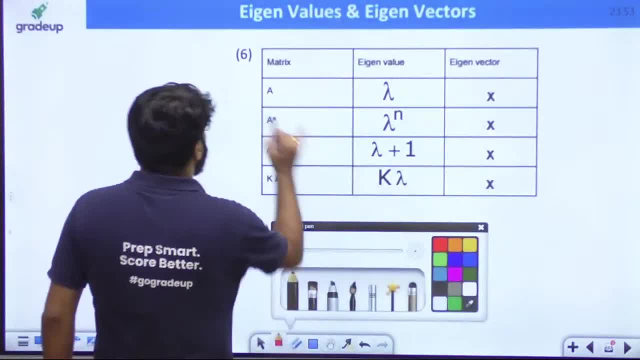 Kalta Kapoor a time. I'm a repass now. next, Kalta Kapoor a time. I'm a repass now. next, one very important property. this is a one very important property. this is a one very important property. this is a very important property, on to which: 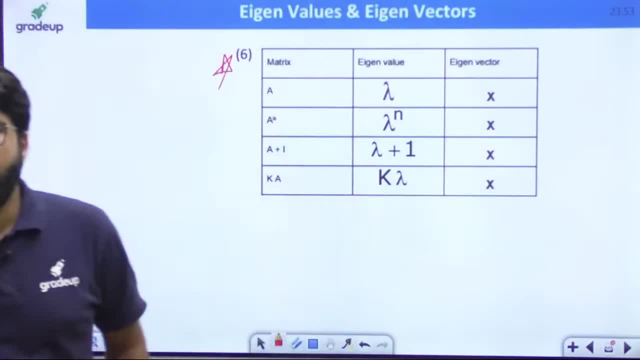 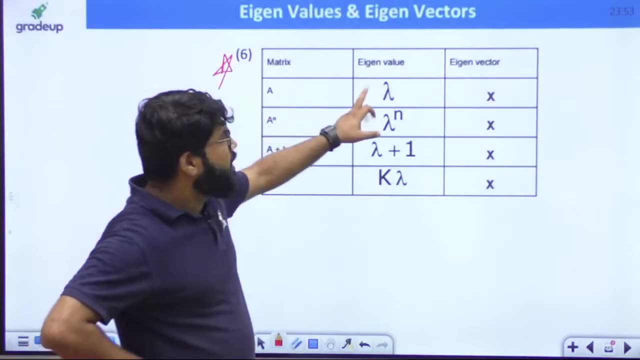 very important property on to which? very important property on to which questions are made, okay, okay now. a very important property on to which questions are made. okay, now, a very important property on to which questions are made. okay, now, a matrix a. a matrix a has eigenvalue. 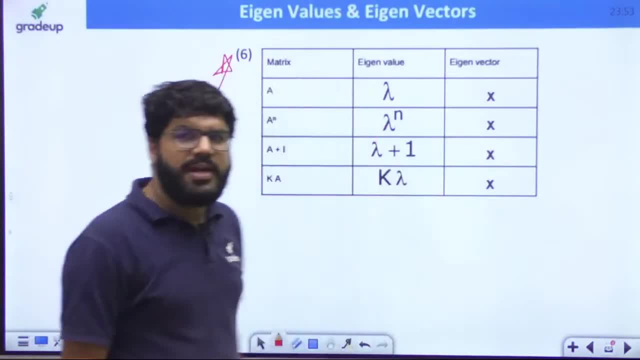 matrix a: a matrix a has eigenvalue. matrix a: a matrix a has eigenvalue. yes, yes, Oscar, rank 5 over Satan. because, yes, yes, Oscar, rank 5 over Satan. because, yes, yes, Oscar, rank 5 over Satan. because determinant itself is non-zero okay, determinant itself is non-zero okay. 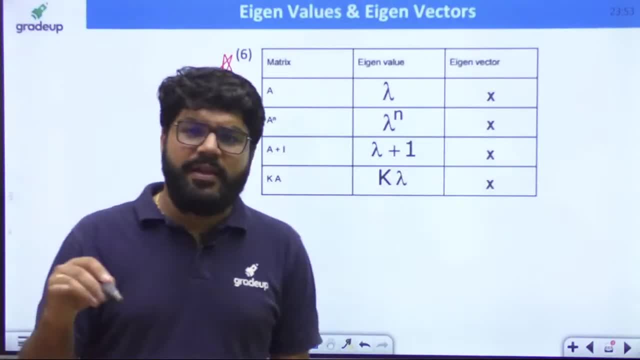 determinant itself is non-zero. okay, directly triangular matrix: Anna for rank. directly triangular matrix: Anna for rank. directly triangular matrix: Anna for rank: you don't need to check the eigenvalues. you don't need to check the eigenvalues. you don't need to check the eigenvalues. the determinant is product of diagonal. 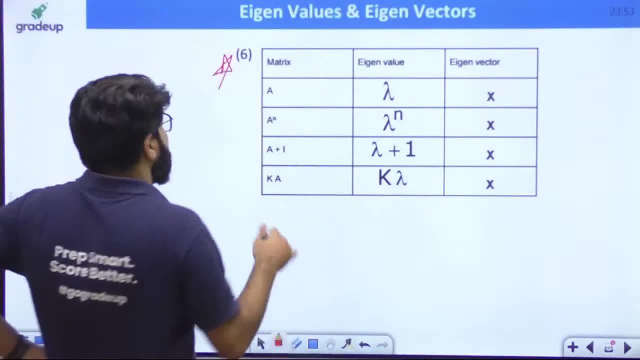 the determinant is product of diagonal. the determinant is product of diagonal numbers determinate non-zero, so rankful numbers determinate non-zero, so rankful numbers determinate non-zero, so rankful. Chetan okay, matrix a has eigenvalue. Chetan okay, matrix a has eigenvalue. 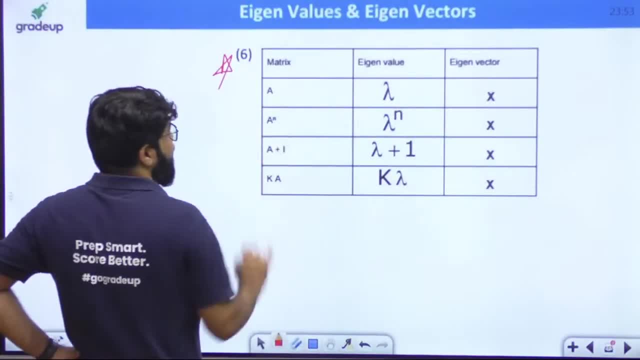 Chetan, okay, matrix a has eigenvalue, lambda and eigenvector X. okay, then, lambda and eigenvector X. okay, then lambda and eigenvector X. okay then, matrix a key power n matrix, yes, I, yes. matrix a key power n matrix, yes, yes. matrix a key power n matrix, yes, yes, I thought a photo, photo again, I'll write. 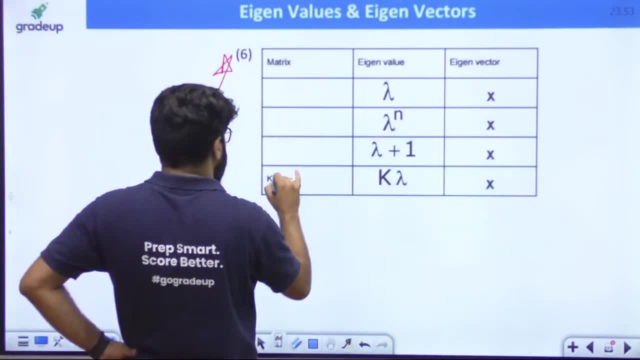 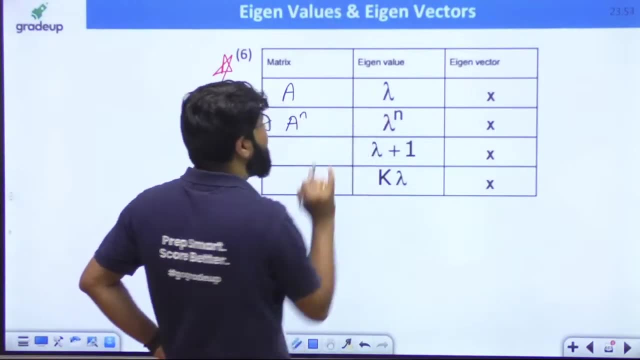 I thought a photo photo again, I'll write. I thought a photo photo again. I'll write it up clearly. matrix a has eigenvalue- it up clearly. matrix a has eigenvalue it up clearly. matrix a has eigenvalue- lambda, then matrix a key power and has lambda, then matrix a key power and has. 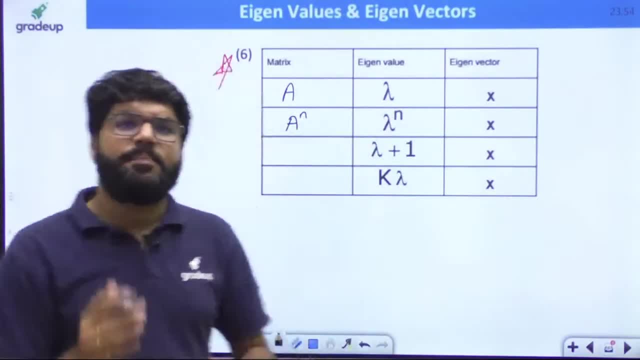 lambda, then matrix a key power and has eigenvalue lambda key power- n okay. same eigenvalue lambda key power n okay. same eigenvalue lambda key power- n okay. same power applied to the eigenvalue. the power applied to the eigenvalue. the power applied to the eigenvalue. the matrix a plus I. eigenvalue lambda plus one. 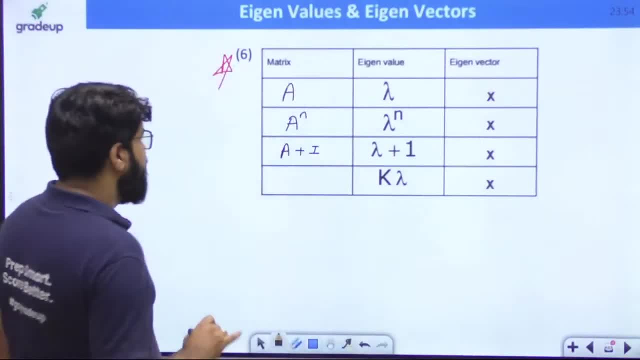 matrix a plus I eigenvalue lambda plus one. matrix a plus I eigenvalue lambda plus one matrix: may plus I number. may plus one matrix may plus I number. may plus one matrix: may plus I number. may plus one. okay, if the matrix is K into a, the eigen. 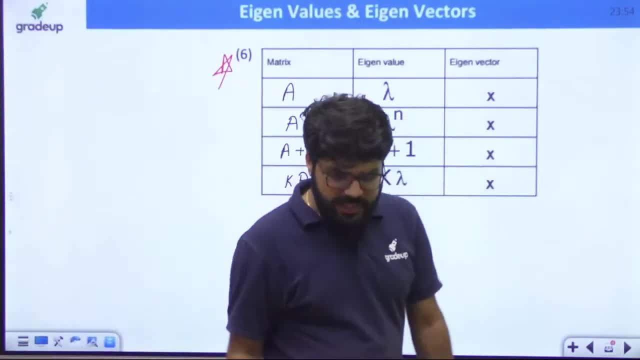 okay. if the matrix is K into a, the eigen okay. if the matrix is K into a, the eigen value is K into lambda, but in all of the value is K into lambda, but in all of the value is K into lambda, but in all of the cases eigenvectors unchanged, although. 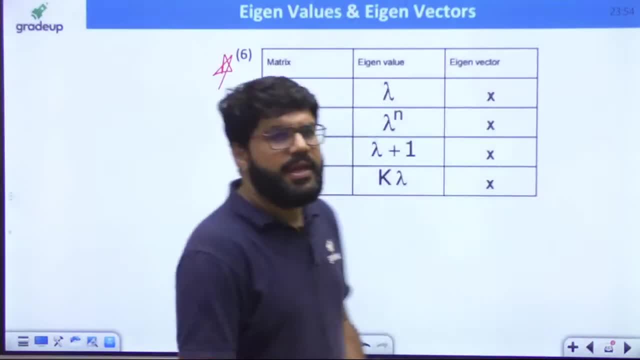 cases: eigenvectors unchanged. although cases eigenvectors unchanged. although direct question of eigenvectors. I have direct question of eigenvectors. I have direct question of eigenvectors. I have not taken will be lunga, maybe okay that not taken. will be lunga, maybe okay that. 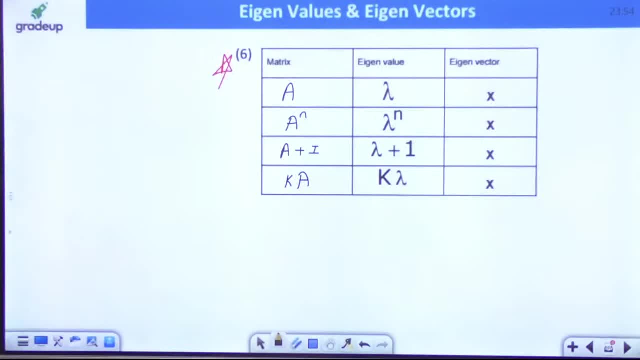 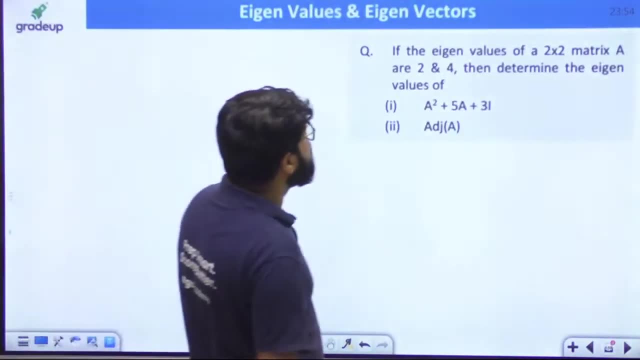 not taken will be lunga, maybe. okay, that also I will consider, don't worry okay. also, I will consider, don't worry, okay. also I will consider, don't worry okay, right. so, for example, for example, have a right. so, for example, for example, have a right. so, for example, for example, have a look at this question- if the eigenvalues 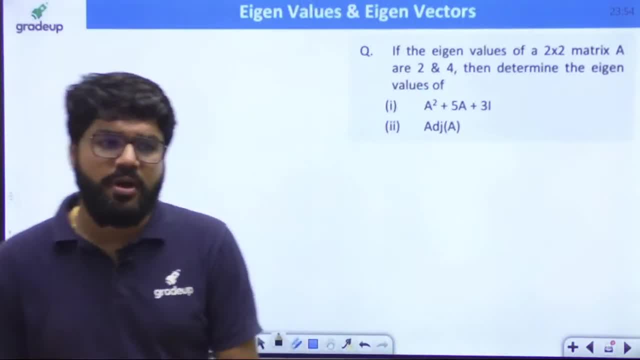 look at this question. if the eigenvalues- look at this question- if the eigenvalues of a 2 cross 2 matrix a are 2 and 4, of a 2 cross 2 matrix a are 2 and 4. of a 2 cross 2 matrix a are 2 and 4, determine the eigenvalues of determine. 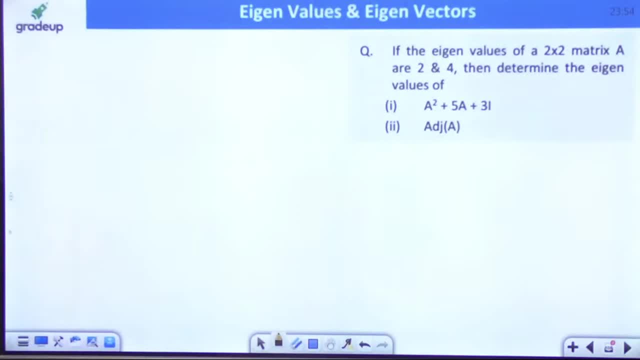 determine the eigenvalues of: determine. determine the eigenvalues of: determine the eigenvalues of a square plus 5: a. the eigenvalues of a square plus 5: a. the eigenvalues of a square plus 5. a plus 3: I and adjoint of a: a square plus 5. 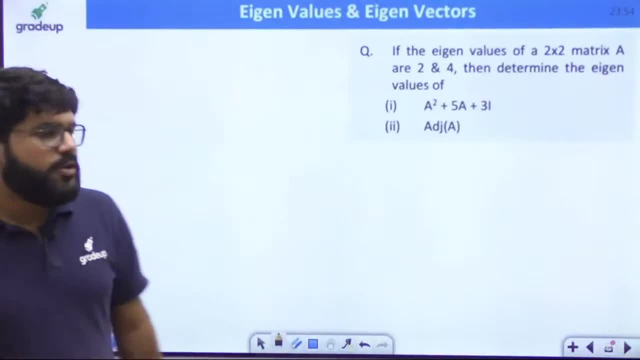 plus 3 I and adjoint of a a square plus 5 plus 3 I, and adjoint of a a square plus 5. a plus 3 I and adjoint of a and adjoint a plus 3 I and adjoint of a and adjoint. 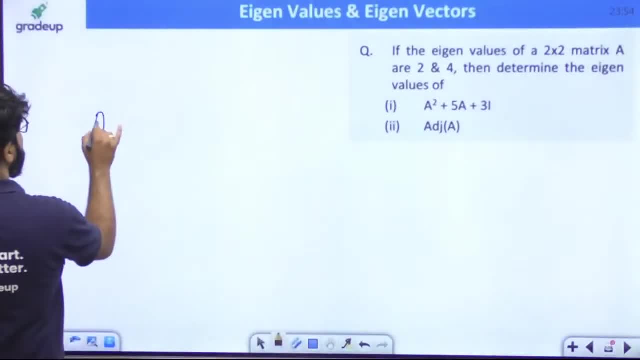 a plus 3. I and adjoint of a and adjoint of a question number one. okay. the of a question number one, okay. the of a question number one. okay. the eigenvalues of a matrix are 2 and 4, okay. eigenvalues of a matrix are 2 and 4, okay. 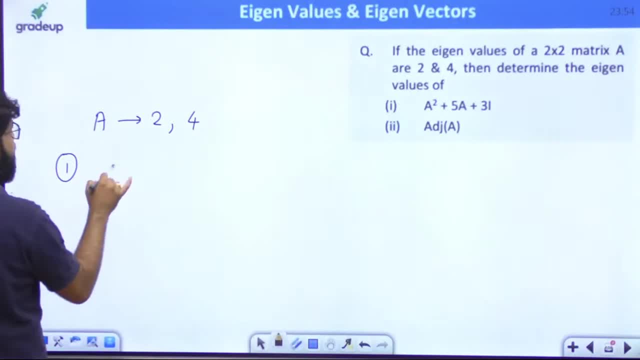 eigenvalues of a matrix are 2 and 4. okay, right 2 and 4, so question number one: right 2 and 4, so question number one: right 2 and 4, so question number one: what should be the eigenvalues of a? what should be the eigenvalues of a? 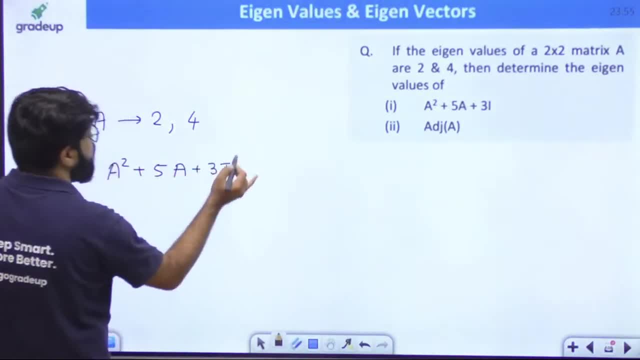 what should be the eigenvalues of a square plus 5 a plus 3i? so what does the square plus 5 a plus 3i? so what does the square plus 5 a plus 3i? so what does the previous property tells you if you take? 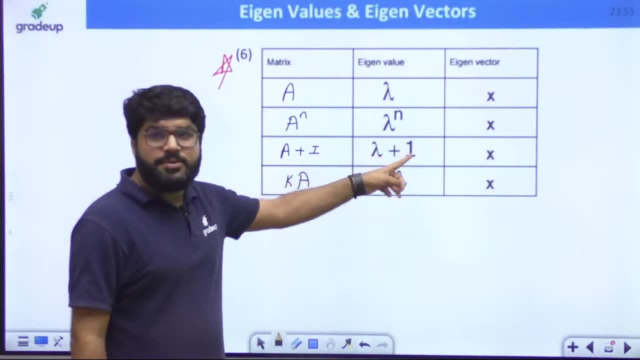 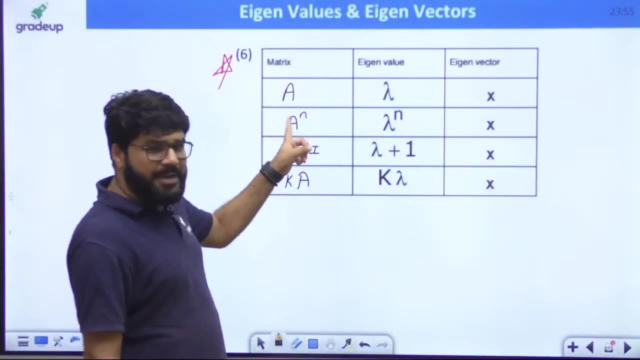 previous property. tells you if you take previous property. tells you if you take property you are applying to a whatever property. you are applying to a whatever property. you are applying to a whatever operation. you apply to a same. apply to operation. you apply to a same. apply to. 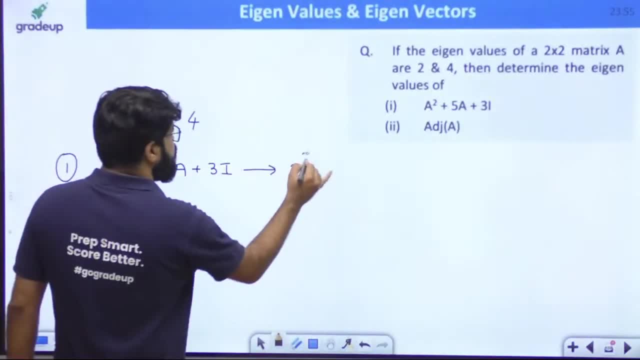 operation you apply to a same apply to lambda. that means a square. so 2 square lambda, that means a square. so 2 square lambda, that means a square, so 2 square. first eigenvalue 2 square, then plus 5. first eigenvalue 2 square, then plus 5. 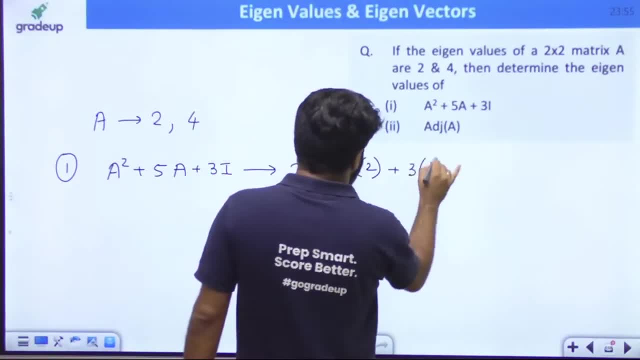 first eigenvalue, 2 square, then plus 5 into a, the 5 into lambda, plus 3 into I, I into a, the 5 into lambda, plus 3 into I, I into a, the 5 into lambda, plus 3 into I. I keep the given I got, I keep the given. 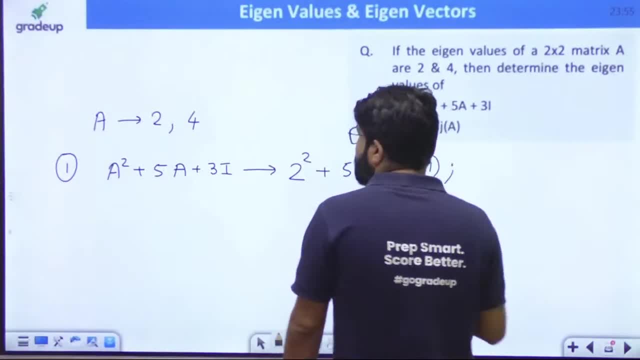 keep the given I got. I keep the given. keep the given I got. I keep the given. I got okay comma. this is the first I can. I got okay comma. this is the first I can. I got okay comma. this is the first I can value. next will be for the matrix. 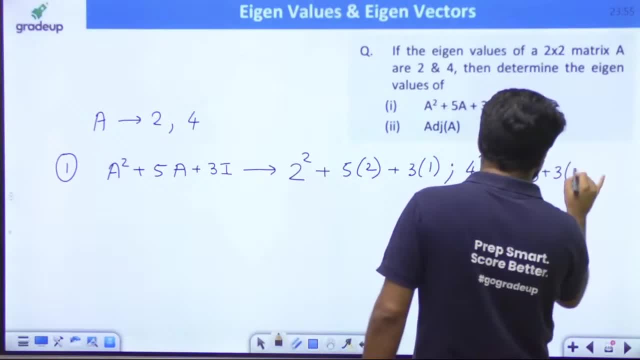 value. next will be for the matrix value. next will be for the matrix square: the 4 square plus 5 into a to 5 square. the 4 square plus 5 into a to 5 square. the 4 square plus 5 into a to 5 into 4, 3 into I to 3 into 1, that's it. 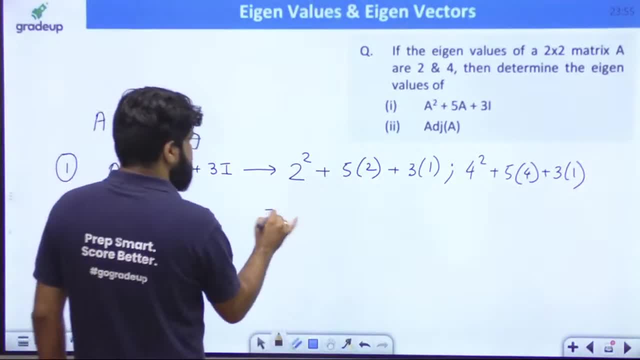 into 4. 3 into I to 3 into 1. that's it into 4. 3 into I to 3 into 1. that's it. that's it. so this is equal to 4 plus 10. that's it, so this is equal to 4 plus 10. 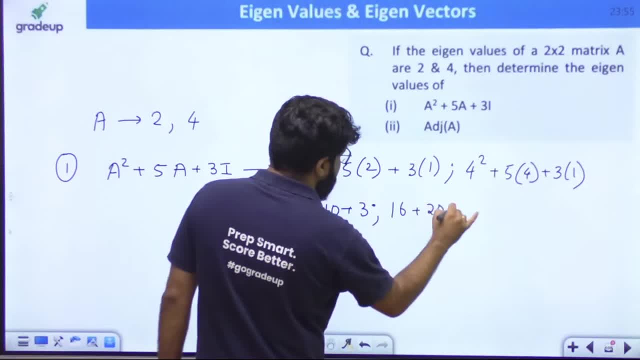 that's it. so this is equal to 4 plus 10 plus 3. next one is 16 plus 20 plus 3, so plus 3. next one is 16 plus 20 plus 3, so plus 3. next one is 16 plus 20 plus 3, so you get now, oh yeah, 17 and the next: 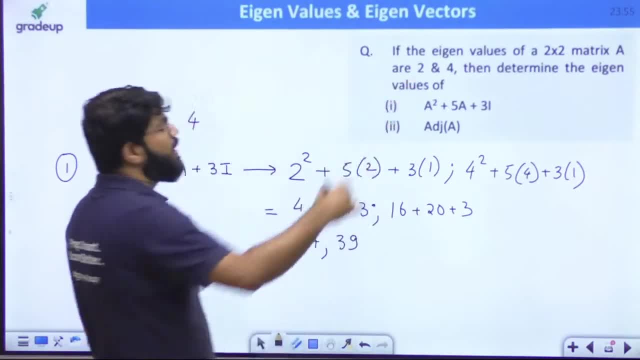 you get now, oh yeah, 17. and the next. you get now, oh yeah, 17. and the next eigenvalue is 39. the eigenvalues of the eigenvalue is 39. the eigenvalues of the eigenvalue is 39. the eigenvalues of the matrix: a square plus 5, a plus 3i is 17. 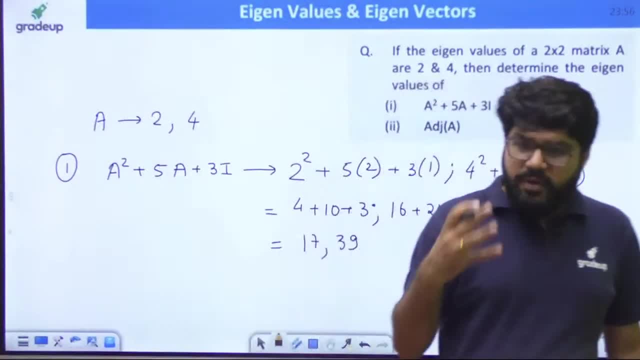 matrix a square plus 5 a plus 3i is 17. matrix a square plus 5 a plus 3i is 17 and 39. simple obviously, what a check. and 39? simple obviously, what a check and 39? simple obviously, what a check. question to one day we will take other. 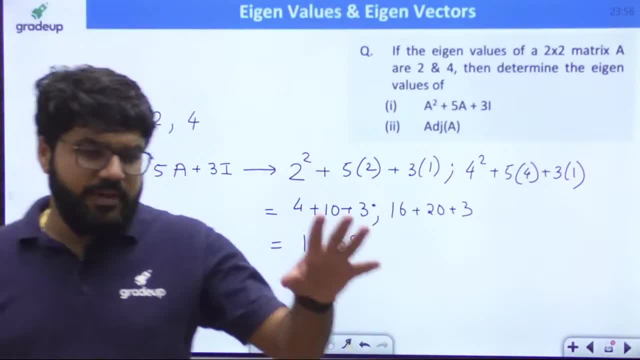 question to one day. we will take other question to one day. we will take other good questions also. now I kill and form good questions also now. I kill and form good questions also. now I kill and form. a converter K determinant does not change. a converter K determinant does not change. 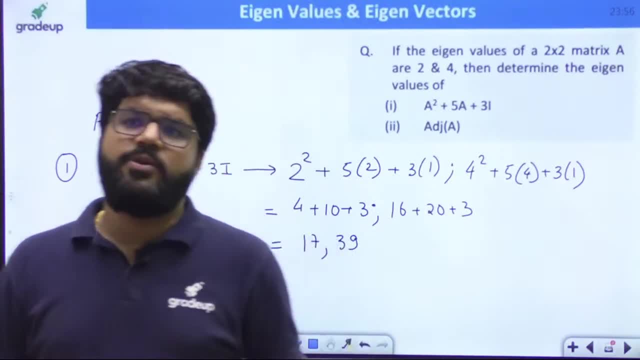 a converter, K determinant does not change which, but on no Pragya eigenvalues are which. but on no Pragya eigenvalues are which. but on no Pragya eigenvalues are defined for square matrices, only ticket. defined for square matrices, only ticket. defined for square matrices, only ticket. now let's see what is the eigenvalues of. 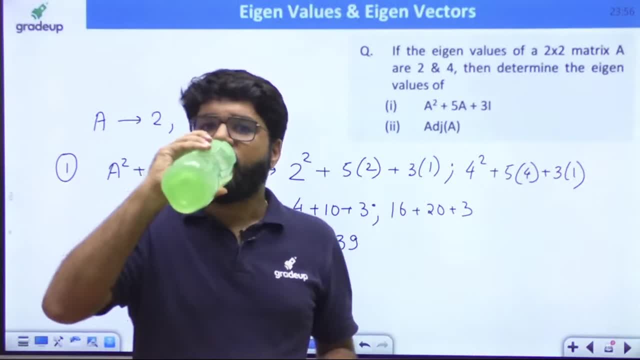 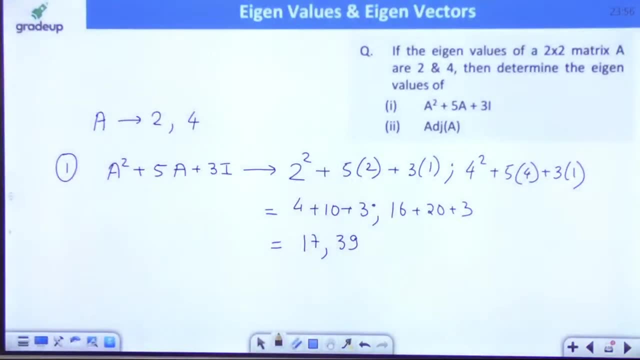 now. let's see what is the eigenvalues of now. let's see what is the eigenvalues of adjoint a here. what should be the adjoint a here? what should be the adjoint a here? what should be the eigenvalues of adjoint a? what should be? 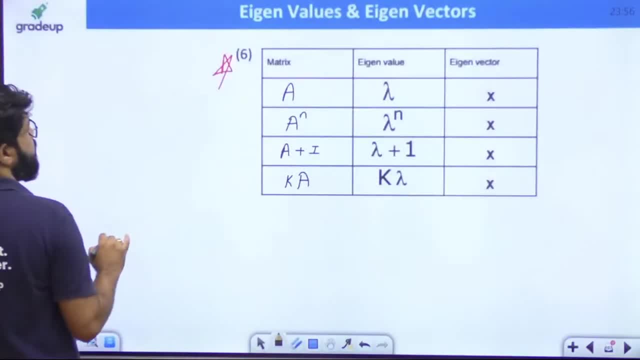 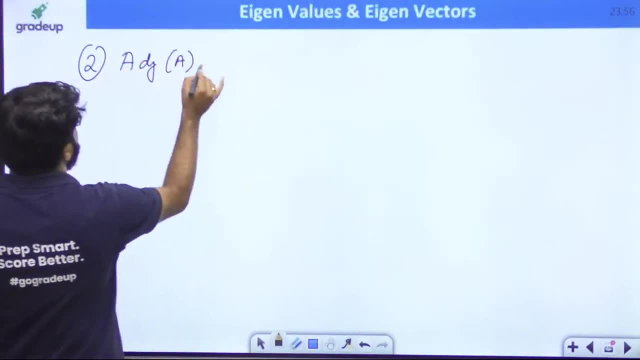 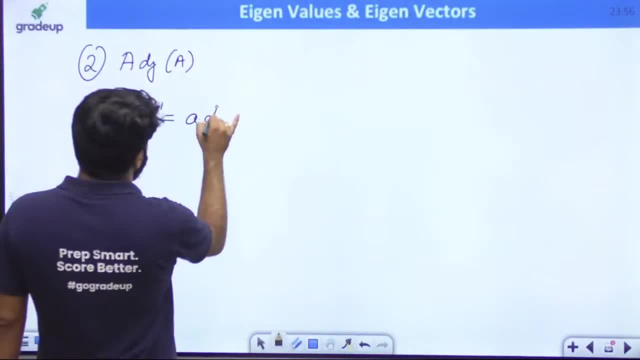 eigenvalues for adjoint a. how do you find out the eigenvalues for adjoint a? how do you find out the adjoint a? so you have to use the adjoint a. so you have to use the adjoint a. so you have to use the formula a inverse. what is the? a inverse? 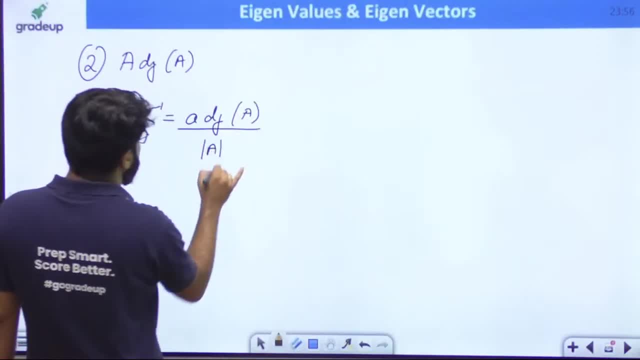 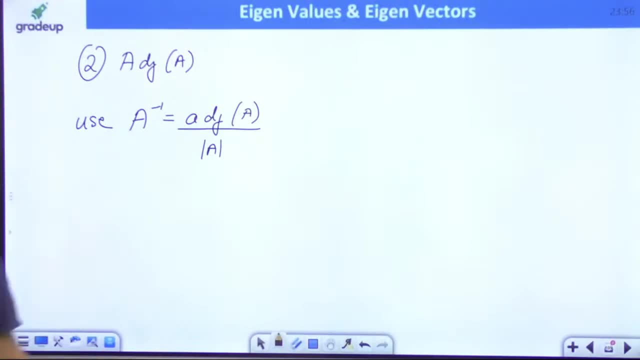 formula: a inverse. what is the? a inverse formula, a inverse. what is the? a inverse formula basic. a inverse formula adjoint a formula basic: a inverse formula adjoint a formula basic. a inverse formula. adjoint a upon modulus of a. okay, okay, a inverse upon modulus of a: okay, okay, a inverse. 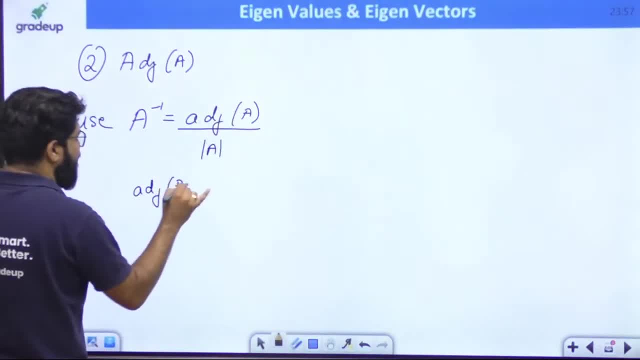 upon modulus of a. okay, okay, a inverse equal to adjoint a upon modulus of a so equal to adjoint a. upon modulus of a so equal to adjoint a upon modulus of a. so, from here, I will write down and joint a. from here, I will write down and joint a. 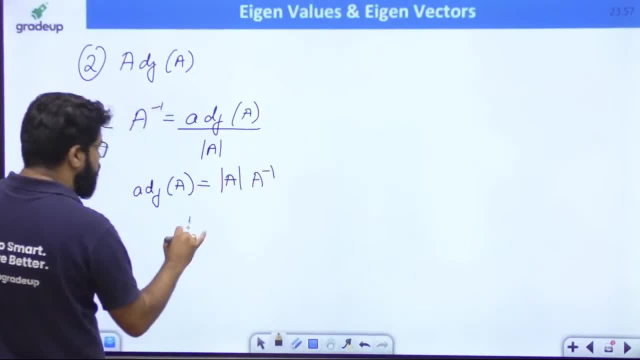 from here I will write down and joint a equal to the modulus of a into a inverse. equal to the modulus of a into a inverse. equal to the modulus of a into a inverse. now, what is the modulus of a modulus of now, what is the modulus of a modulus of? 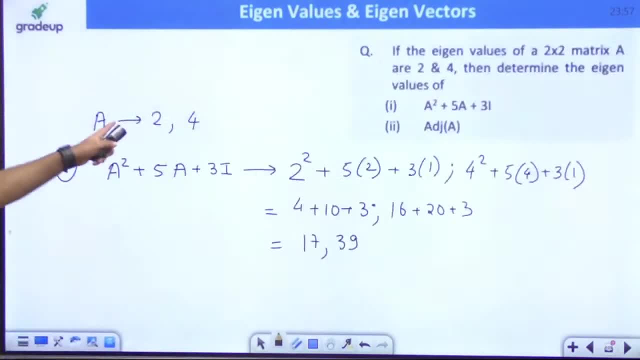 now, what is the modulus of a, modulus of a means product of eigenvalues? we know a means product of eigenvalues. we know a means product of eigenvalues. we know this property and the eigenvalues of a. this property and the eigenvalues of a. this property and the eigenvalues of a are given to me as 2 and 4, so this is 2. are given to me as 2 and 4, so this is 2. are given to me as 2 and 4, so this is 2 multiplied by 4, that is 8 modulus of a. multiplied by 4, that is 8 modulus of a. 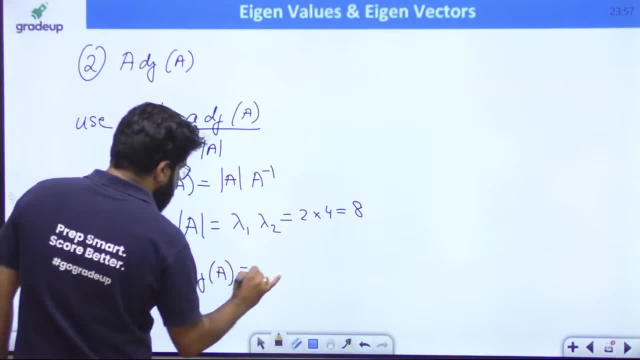 multiplied by 4, that is 8. modulus of a is 8. so what should be the adjoint of a is 8. so what should be the adjoint of a is 8, so what should be the adjoint of a 8a inverse? what is the adjoint of a is? 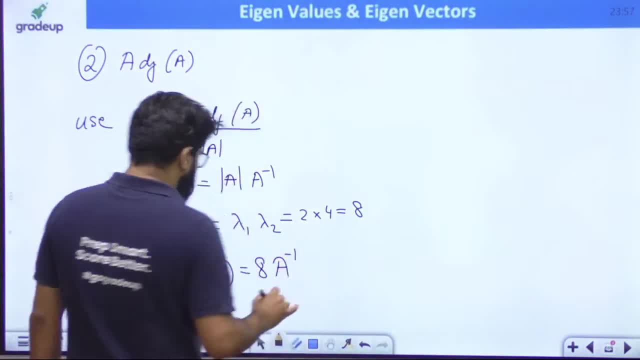 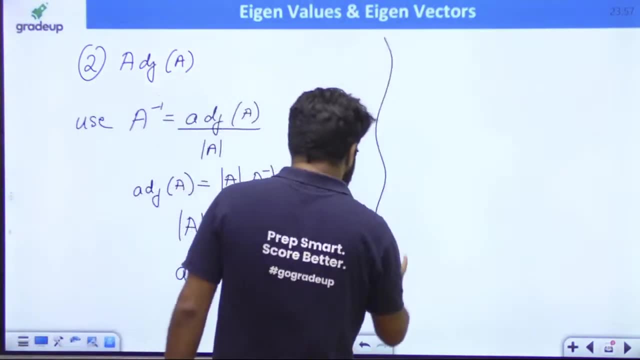 8a inverse. what is the adjoint of a is 8a inverse. what is the adjoint of a is 8a inverse. is known as the 8a inverse. the 8a inverse is known as the 8a inverse. the 8a inverse is known as the 8a inverse. the adjoint of a is 8a inverse. everybody. 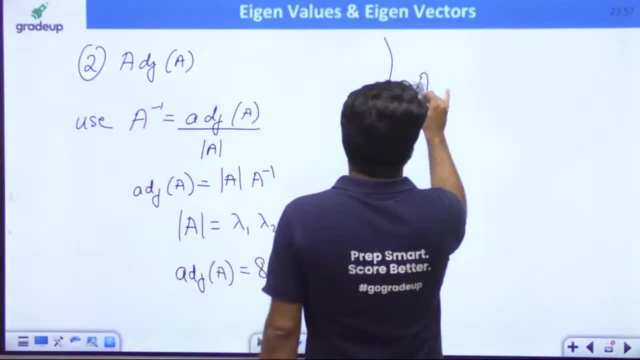 adjoint of a is 8a, inverse everybody. adjoint of a is 8a, inverse everybody, 8a inverse ticket. so now, if a has the 8a inverse ticket, so now if a has the 8a inverse ticket, so now if a has the eigenvalues 2 and 4, what should be the? 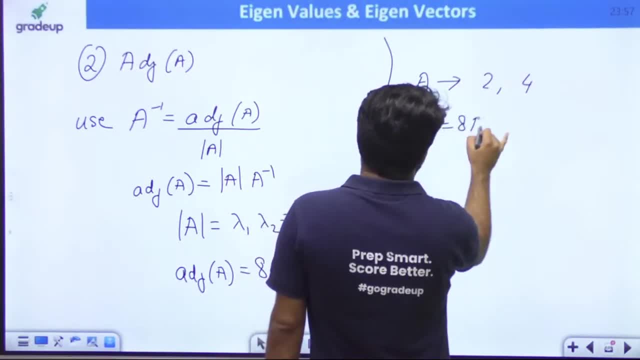 eigenvalues 2 and 4. what should be the eigenvalues 2 and 4? what should be the eigenvalues for adjoint a? adjoint a is eigenvalues for adjoint a. adjoint a is eigenvalues for adjoint a. adjoint a is 8a inverse. so as I told you, whatever. 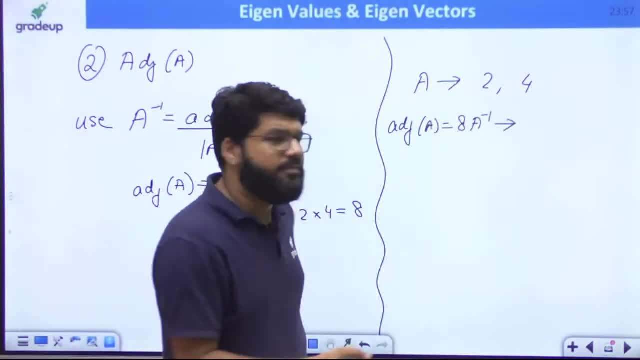 8a inverse. so as I told you, whatever 8a inverse, so as I told you, whatever operation applied to matrix, same operation applied to matrix. same operation applied to matrix, same operation will be applied to the eigen operation will be applied to the eigen operation will be applied to the eigen value. so you can now go 8 into a. 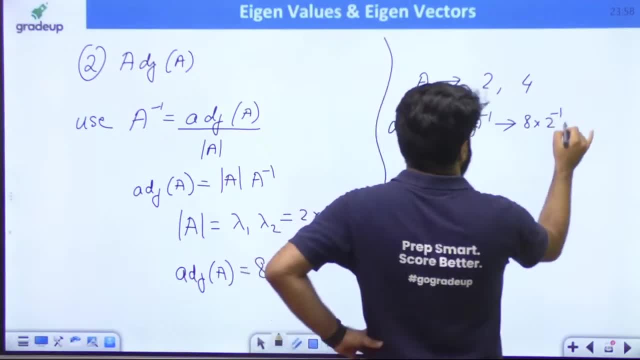 value. so you can now go 8 into a value. so you can now go 8 into a inverse, that is 2 inverse 8 into 4 inverse. that is 2 inverse 8 into 4 inverse, that is 2 inverse 8 into 4 inverse. so this is 8 by 2, 8 by 4 and inverse, so this is 8 by 2, 8 by 4 and inverse, so this is 8 by 2, 8 by 4, and that is 4 comma 2. so these are the, that is 4 comma 2, so these are the. 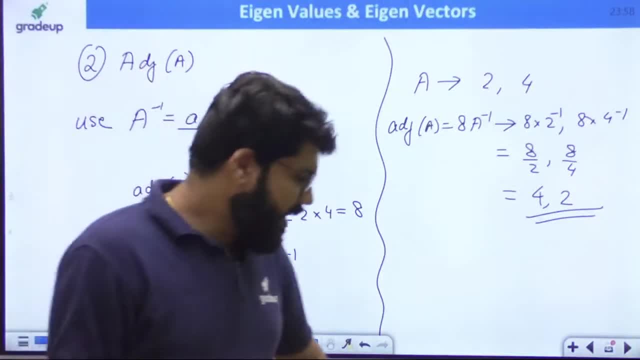 that is, 4 comma 2. so these are the eigenvalues of the adjoint of the matrix, eigenvalues of the adjoint of the matrix. eigenvalues of the adjoint of the matrix. adjoint of the matrix 4 and 2 basically. adjoint of the matrix 4 and 2, basically. 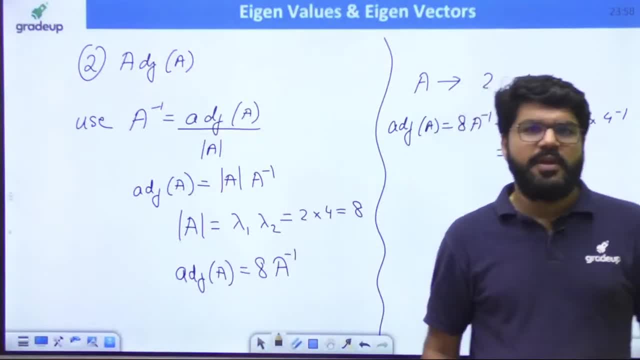 adjoint of the matrix 4 and 2. basically same, but interchange it will be same for same, but interchange it will be same for same, but interchange it will be same for 2 cross 2, but not for 3 cross 3. okay, not 2 cross 2, but not for 3 cross 3, okay, not. 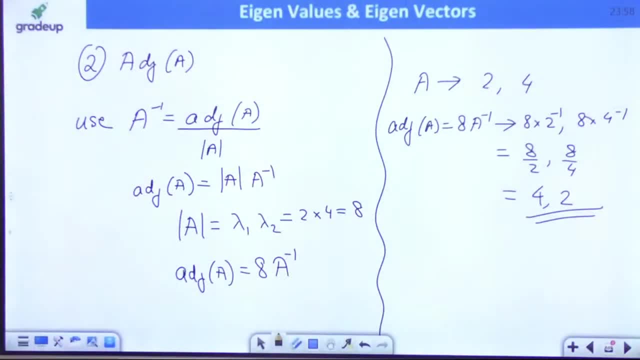 2 cross 2, but not for 3 cross 3. okay, not for 3 cross 3. take a 3 cross 3 Kelly for 3 cross 3. take a 3 cross 3 Kelly. for 3 cross 3. take a 3 cross 3 Kelly. same name yoga. okay, 3 cross 3 Kelly. 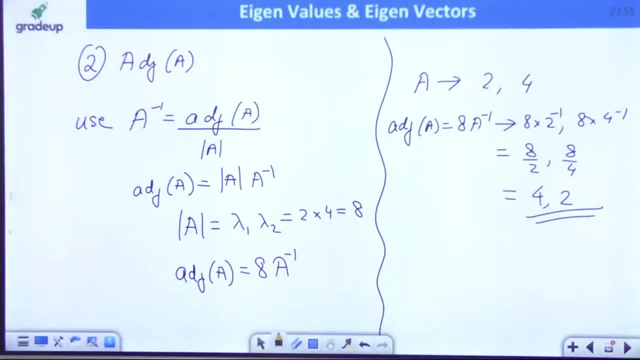 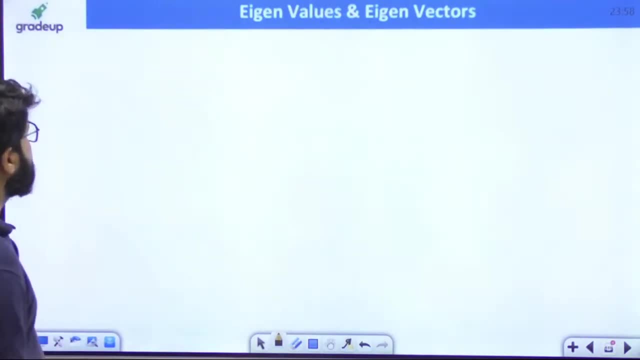 same name: yoga. okay, 3 cross 3 Kelly. same name: yoga. okay, 3 cross 3 Kelly. story will be little different. she can story will be little different. she can story will be little different. she can next, next, next, next. if some of the elements of every row next, if some of the elements of every row. next, if some of the elements of every row or every column is same, then one of the or every column is same, then one of the or every column is same, then one of the eigenvalues of the matrix is equal to. 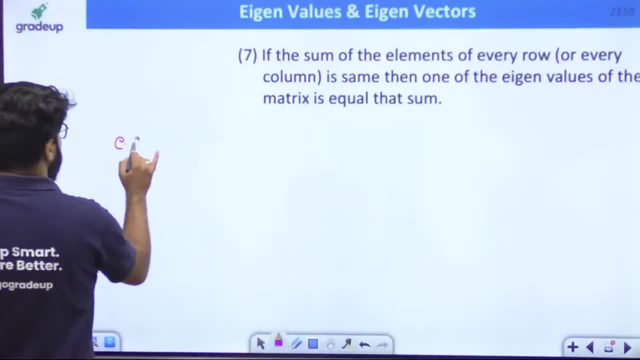 eigenvalues of the matrix is equal to. eigenvalues of the matrix is equal to that sum, for example, for example, for that sum, for example, for example, for that sum, for example, for example, for example. let us consider the same matrix example. let us consider the same matrix. 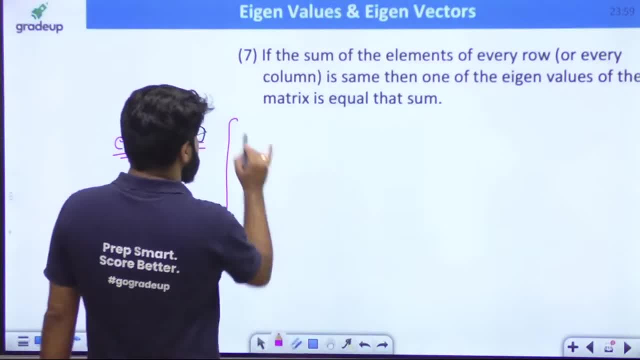 example, let us consider the same matrix: 1 0 1. just be sorry, just call me solve 1 0 1. just be sorry. just call me solve 1 0 1. just be sorry, just call me solve kiata. be 0, 1, 1, 1 0, 1 and 1 1 0 we. kiata be 0 1, 1, 1, 0, 1 and 1 1 0. we kiata be 0 1 1 0, 1 0, 1 and 1 0, 1 0, 1 0. we solve this now. let us take the sum of. 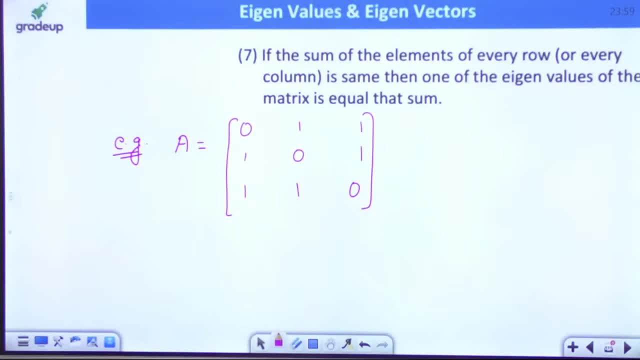 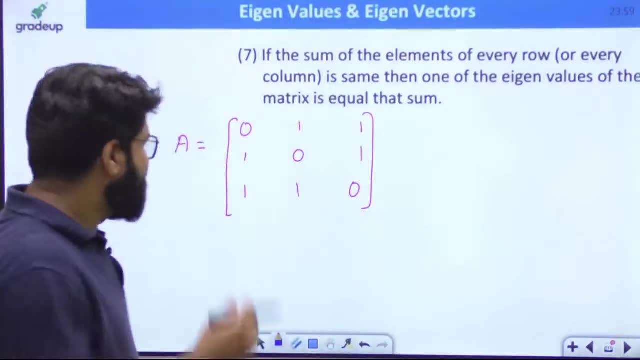 solve this now. let us take the sum of solve this now. let us take the sum of every row. let us take the sum of every, every row. let us take the sum of every, every row. let us take the sum of every row. thank you, saga, for your compliment. 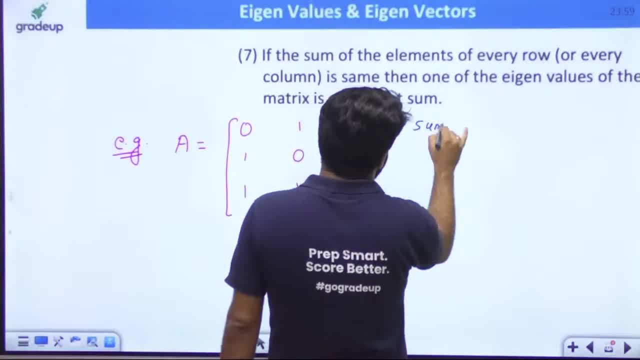 so what is this? what is the sum of the? so what is this? what is the sum of the? so what is this? what is the sum of the first row? sum is 2. what is the sum of first row? sum is 2. what is the sum of? 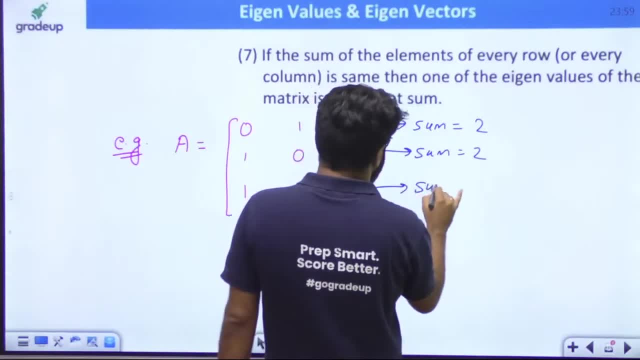 first row sum is 2. what is the sum of the second row sum is also 2. what is the? the second row sum is also 2. what is the? the second row sum is also 2. what is the sum of the third row sum is again 2. so 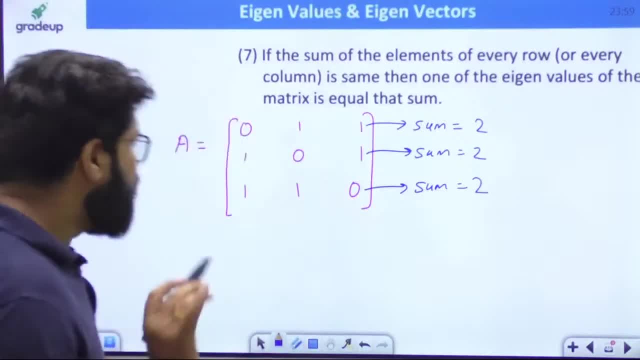 sum of the third row sum is again 2. so sum of the third row sum is again 2. so sum of every row is same. sum of every. sum of every row is same. sum of every. sum of every row is same. sum of every row is same right. and whenever some of 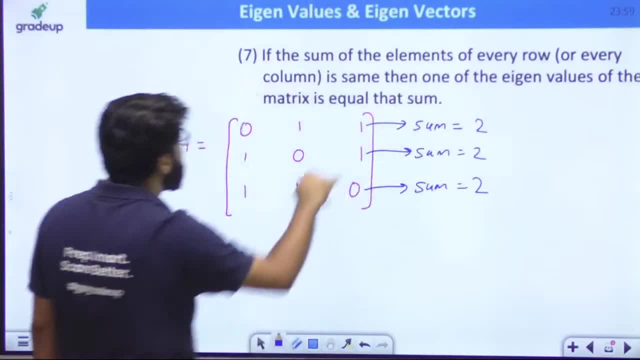 row is same right, and whenever some of row is same right, and whenever some of the elements of every row is same, then the elements of every row is same. then the elements of every row is same, then one of the eigenvalues is equal to that. one of the eigenvalues is equal to that. 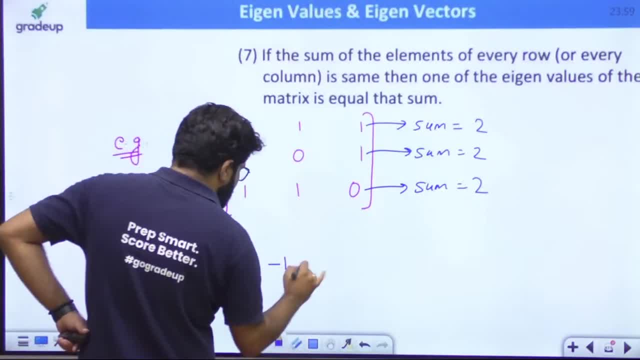 one of the eigenvalues is equal to that sum. for this matrix a. the eigenvalues sum for this matrix a. the eigenvalues sum for this matrix a. the eigenvalues were minus 1, minus 1 and plus 2, and you were minus 1, minus 1 and plus 2, and you. 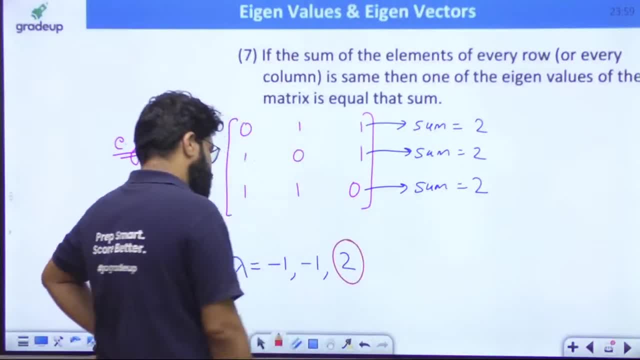 were minus 1, minus 1 and plus 2, and you can note that. you can note that there is, can note that you can note that there is, can note that you can note that there is an eigenvalue plus 2, the sum of every. an eigenvalue plus 2, the sum of every. 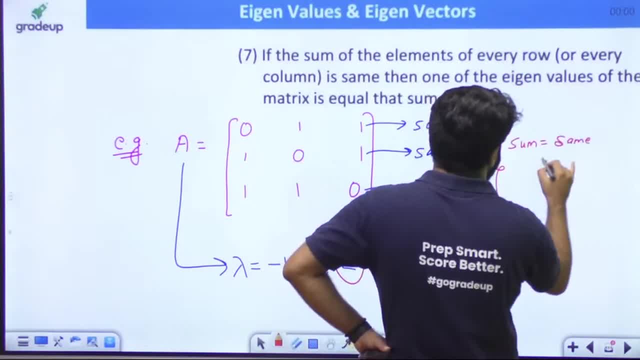 an eigenvalue plus 2. the sum of every row is same. the sum of the elements of row is same. the sum of the elements of row is same. the sum of the elements of every row is same, and that is equal to 2. every row is same, and that is equal to 2. 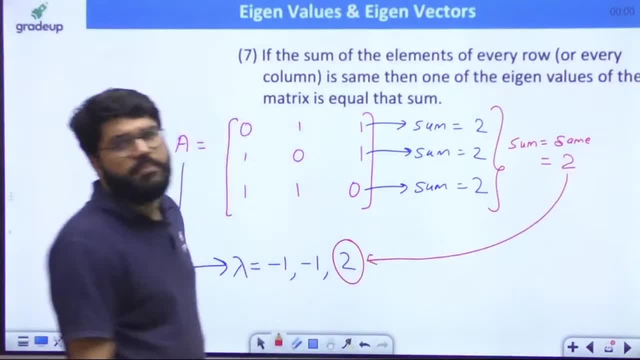 every row is same and that is equal to 2, and one of the eigenvalue is also equal, and one of the eigenvalue is also equal, and one of the eigenvalue is also equal to that sum. it's because questions one to that sum. it's because questions one. 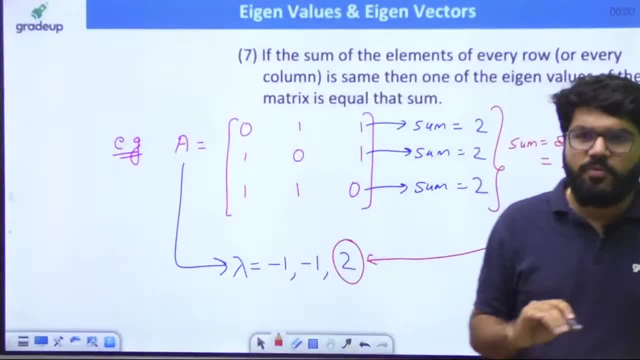 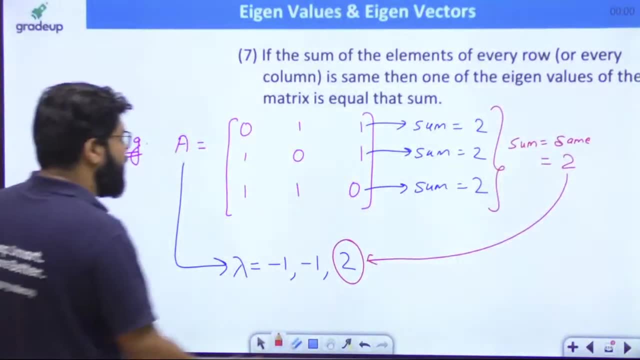 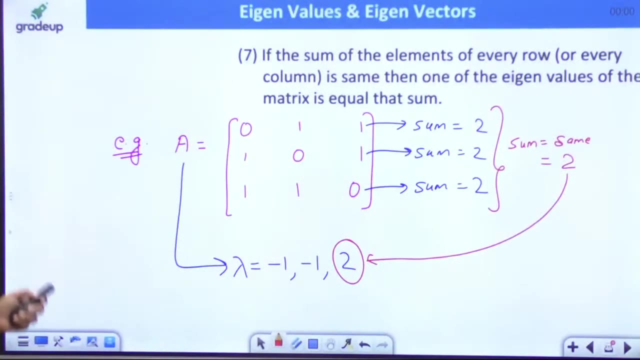 to that sum. it's because questions one thing: okay. all miscellaneous questions thing: okay. all miscellaneous questions thing, okay, all miscellaneous questions will be taken tomorrow. they can be will be taken tomorrow. they can be- will be taken tomorrow. they can be simple, simple question and simple, simple, simple question and simple, simple question and simple, simple question. right, a shallow cool. next, 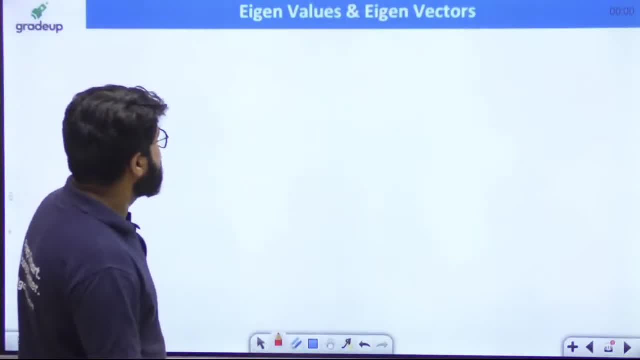 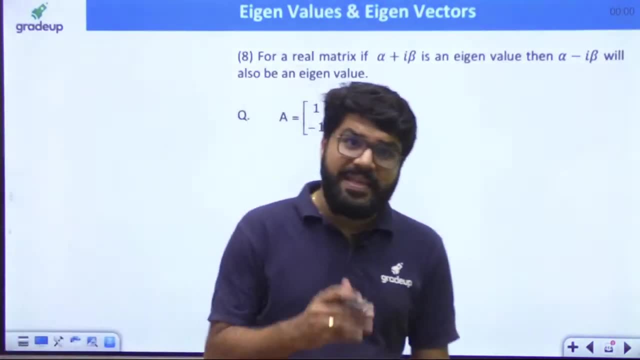 question and simple, simple question: right, a shallow cool next question and simple, simple question: right, a shallow cool next property for a real matrix- now this is a right. a shallow cool next property for a real matrix- now this is a right. a shallow cool next property for a real matrix- now. this is a simple but yet very useful property for. 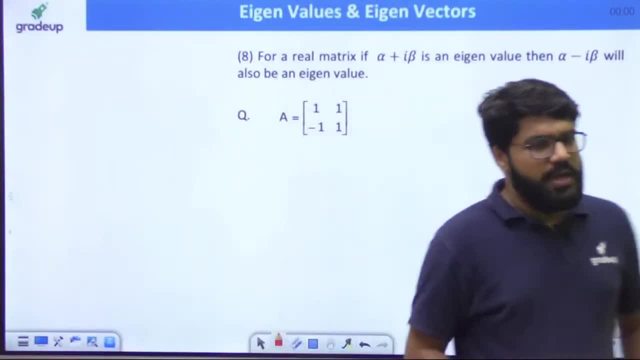 simple but yet very useful property for simple but yet very useful property for competitive exams. you will feel that you competitive exams. you will feel that you competitive exams. you will feel that you will feel that, specially tomorrow, this is will feel that specially tomorrow, this is will feel that specially tomorrow, this is very simple but very useful for a real 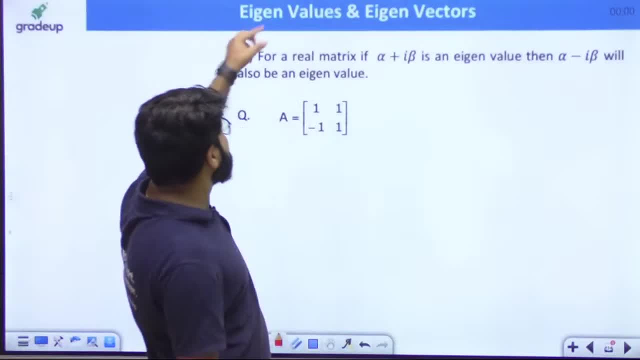 very simple but very useful for a real. very simple but very useful for a real matrix. if alpha plus i beta is an matrix, if alpha plus i beta is an matrix, if alpha plus i beta is an eigenvalue, then alpha minus i beta should eigenvalue, then alpha minus i beta should. 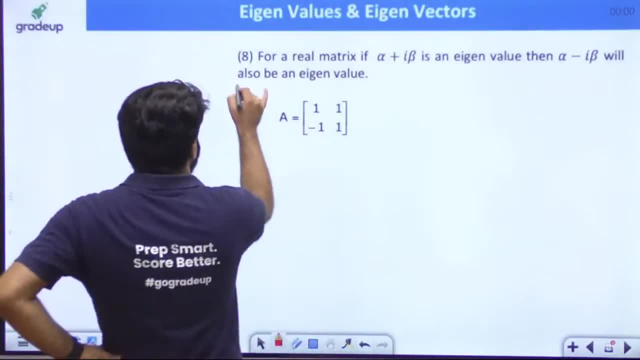 eigenvalue, then alpha minus i, beta should also be an eigenvalue, matlab complex also be an eigenvalue, matlab complex also be an eigenvalue. matlab complex: eigenvalue. in short, I can say that in eigenvalue. in short, I can say that in eigenvalue. in short, I can say that in short. I can say that, if there is any, 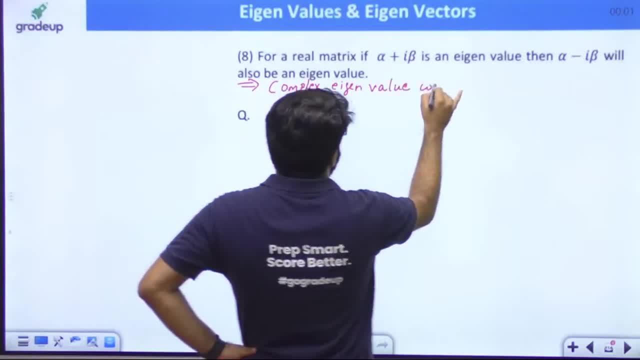 short, I can say that. if there is any short, I can say that if there is any complex eigenvalue, okay, that will always complex eigenvalue. okay, that will always complex eigenvalue. okay, that will always appear. that will always occur in appear, that will always occur in. 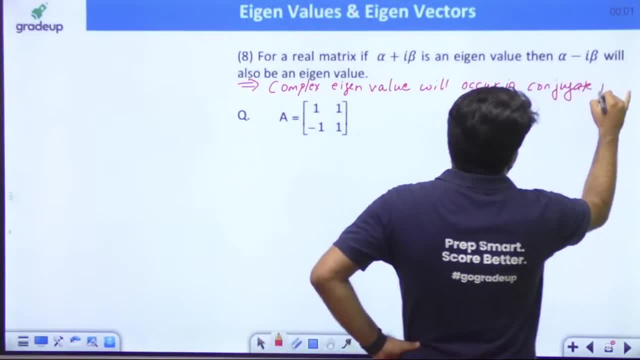 appear, that will always occur in conjugate pair in conjugate pair. if there conjugate pair in conjugate pair. if there conjugate pair in conjugate pair. if there is alpha plus i beta, it cannot be alone. is alpha plus i beta, it cannot be alone. 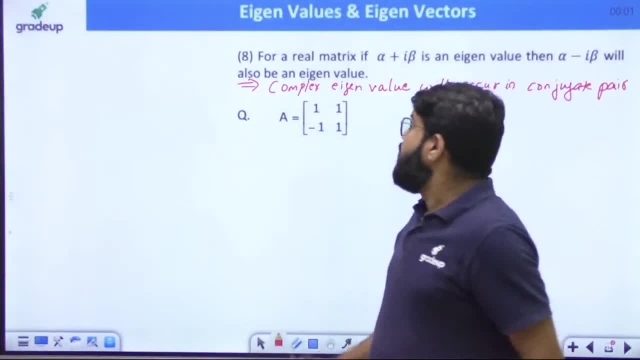 is alpha plus i, beta. it cannot be alone. it has to be supported by alpha minus i for a real matrix for complex matrix now. for a real matrix for complex matrix now. for a real matrix for complex matrix now. what is the real matrix, guys, where all? what is the real matrix, guys, where all? 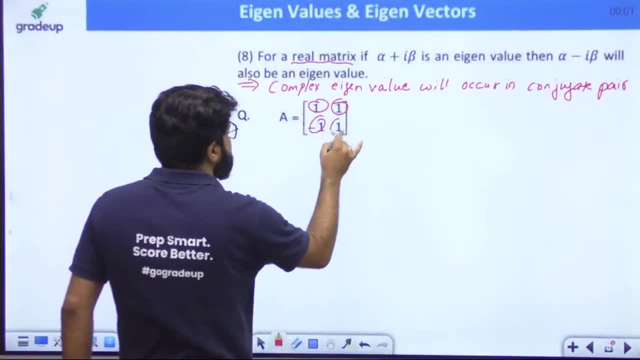 what is the real matrix, guys? where all the elements, all the elements are real, the elements, all the elements are real, the elements, all the elements are real numbers. where all the elements are real numbers. where all the elements are real numbers, where all the elements are real numbers. let's try this with the question. 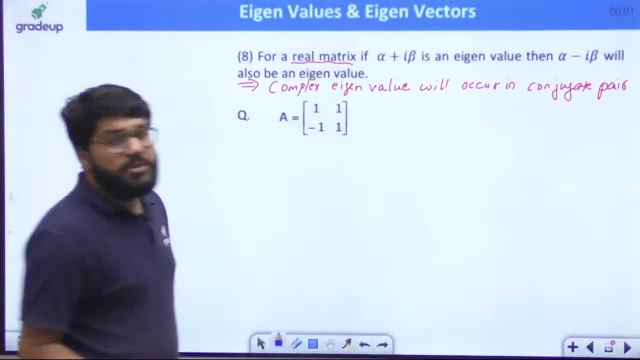 numbers. let's try this with the question. numbers, let's try this with the question. but useful for competitive level. but useful for competitive level, but useful for competitive level questions. so let's try this with our questions. so let's try this with our questions. so let's try this with our numbers. let's try this with the numbers. 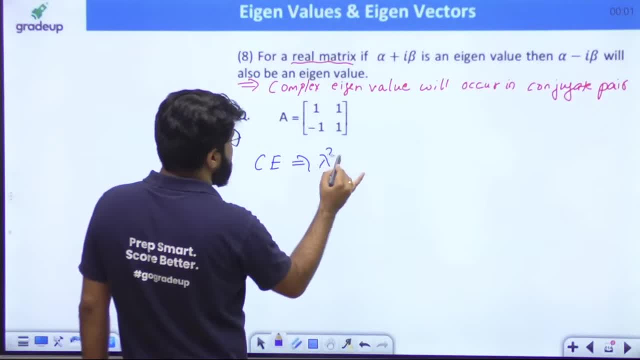 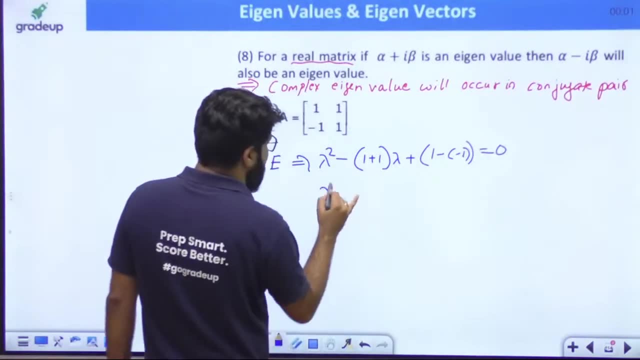 numbers. let's try this with the numbers. numbers, let's try this with the numbers. so it's the characteristic equation: lambda square minus trace plus lambda square minus trace plus lambda square minus trace plus determinant equal to 0 to lambda square determinant equal to 0 to lambda square. 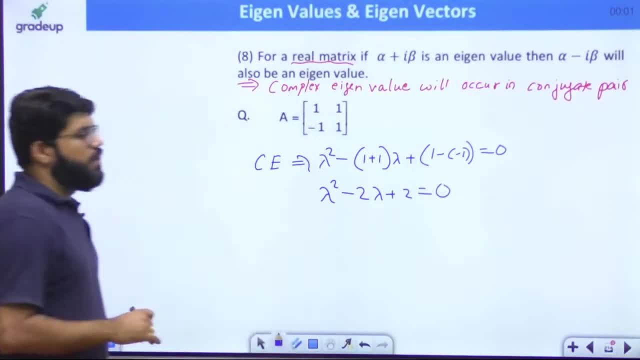 determinant equal to 0 to lambda square minus 2. lambda plus 2 equal to 0 plus 2 minus 2. lambda plus 2 equal to 0 plus 2 minus 2. lambda plus 2 equal to 0 plus 2 equal to the 0 right. so lambda is equal. 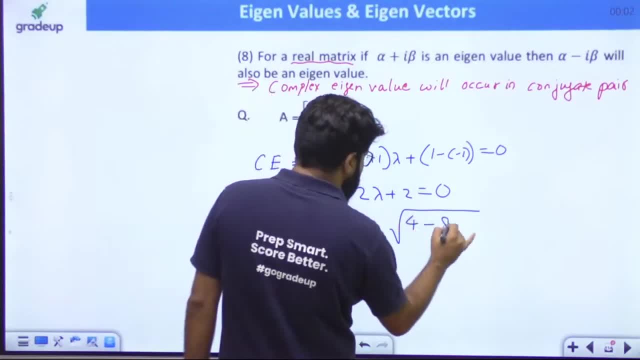 equal to the 0 right. so lambda is equal. equal to the 0 right. so lambda is equal to 2 plus minus root over B square minus to 2 plus minus root over B square minus to 2 plus minus root over B square minus 4 AC divided by 2. a solve it up. this is: 4 AC divided by 2 a. solve it up. this is 4 AC divided by 2 a. solve it up. this is under root of minus 4, which is 2j to say. under root of minus 4, which is 2j to say. 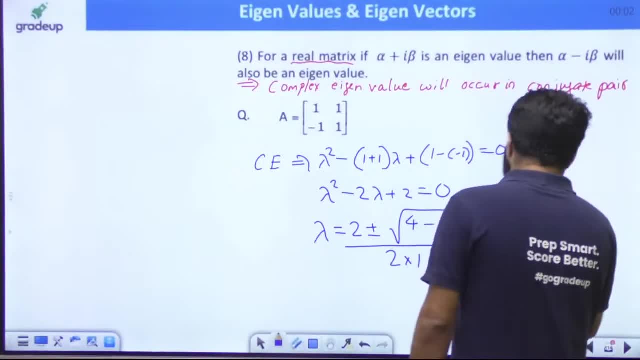 under root of minus 4, which is 2j, to say: cancel kia to 1 plus minus J, yeah, 1. cancel kia to 1 plus minus J, yeah, 1. cancel kia to 1 plus minus J, yeah, 1 plus minus. I imagine a number, Iota. so what? 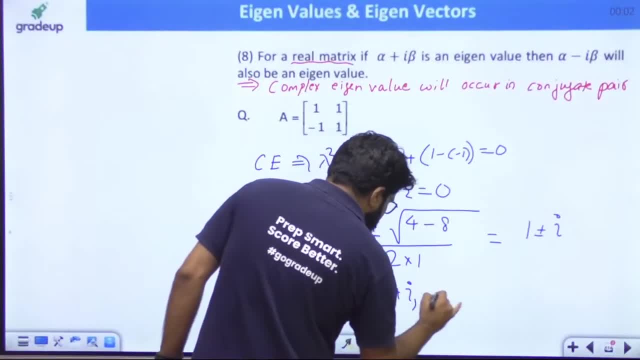 plus minus? I imagine a number Iota. so what plus minus? I imagine a number Iota. so what are the eigenvalues? 1 plus I, 1 minus? are the eigenvalues 1 plus I, 1 minus? are the eigenvalues: 1 plus I, 1 minus I. alpha plus I beta. alpha minus, I beta. 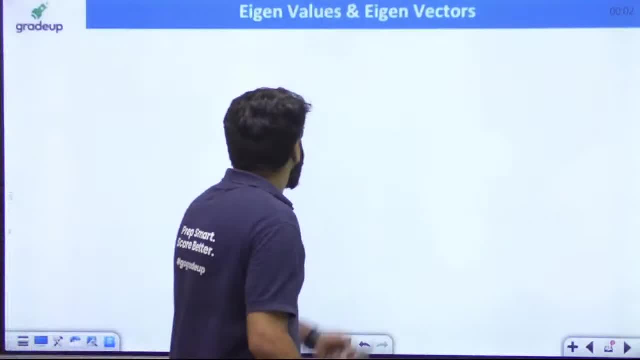 I alpha plus I beta alpha minus I beta, I alpha plus I beta, alpha minus I beta. sat may occur only that is confirm. sat may occur only that is confirm. sat may occur only that is confirm, confirm. confirm, but for a complex matrix: confirm, confirm, but for a complex matrix. 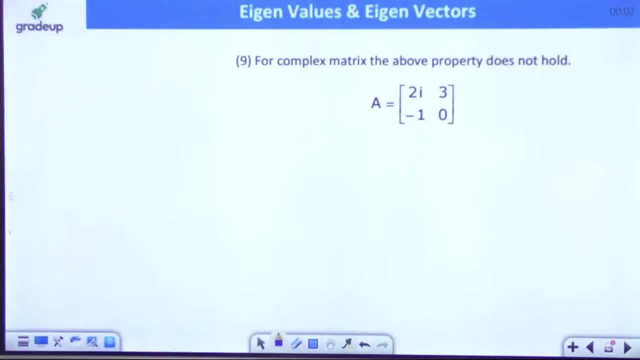 confirm, confirm, confirm, but for a complex matrix, the above property does not hold. the above property does not hold. the above property does not hold. for a complex matrix: the above property does. for a complex matrix: the above property does. for a complex matrix, the above property does not hold. another question for a 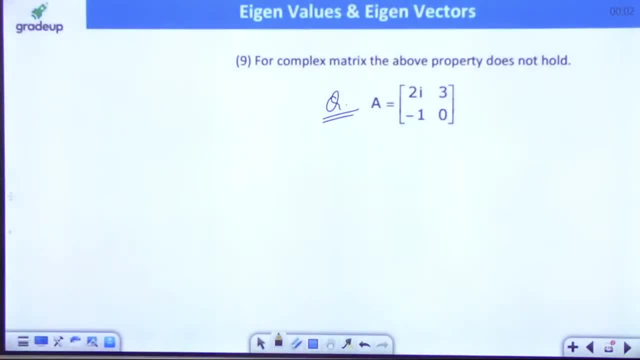 not hold another question for a not hold another question for a complex matrix. the above property does not does complex matrix. the above property does not does complex matrix. the above property does not. does not. does not hold? okay, find out not. does not. does not hold? okay, find out. 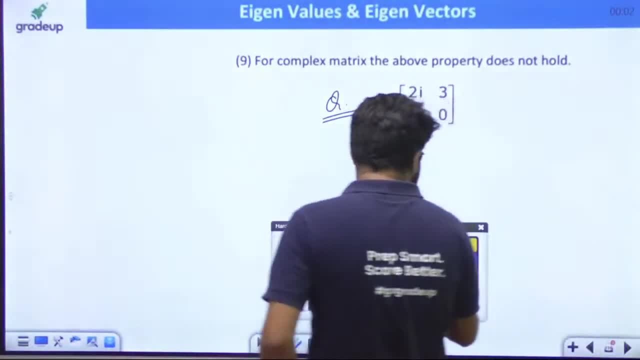 not, does not, does not hold. okay, find out the eigenvalues of this matrix. now this, the eigenvalues of this matrix. now this, the eigenvalues of this matrix. now, this is a complex matrix. why, sir, why this is is a complex matrix? why, sir, why this is? 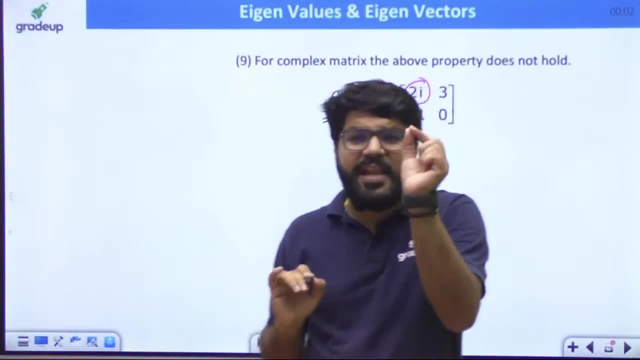 is a complex matrix. why, sir? why this is complex? what is the complex matrix, even complex? what is the complex matrix, even complex? what is the complex matrix, even if a single element is a complex number, if a single element is a complex number, if a single element is a complex number like to I, then the matrix is said to be. 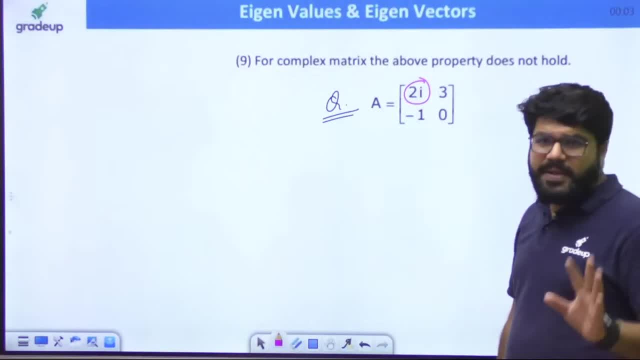 like to I, then the matrix is said to be like to I. then the matrix is said to be complex, even if one or more than one complex, even if one or more than one complex, even if one or more than one element is complex, the eigenvalue said to 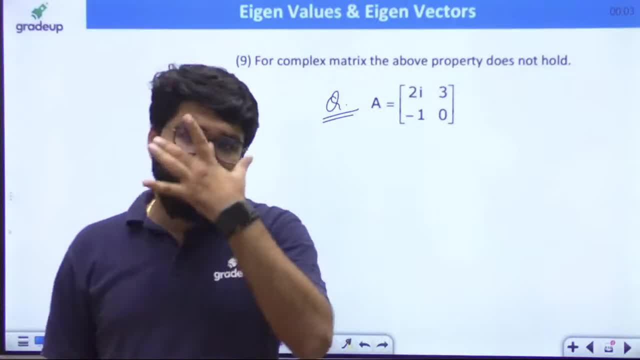 element is complex. the eigenvalue said to element is complex. the eigenvalue said to be complex. the sorry the matrix is be complex. the sorry the matrix is be complex. the sorry the matrix is said to be complex. matrix, now, what is the said to be complex matrix now? what is the? 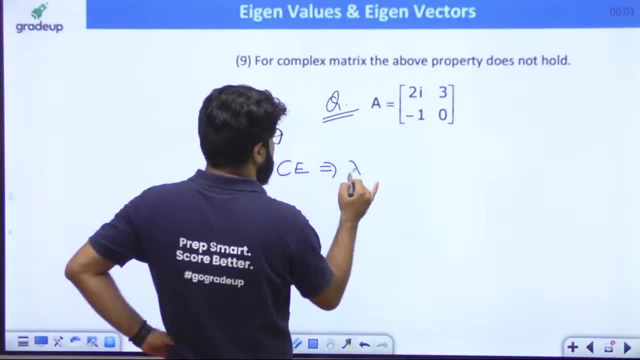 said to be complex matrix. now, what is the characteristic equation of this characteristic equation of this characteristic equation of this complex matrix lambda square minus trace into complex matrix lambda square minus trace into complex matrix lambda square minus trace into lambda plus determinant: 0 minus minus lambda plus determinant: 0 minus minus. 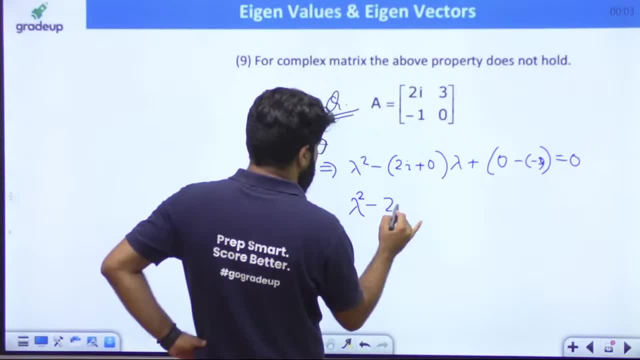 lambda plus determinant: 0 minus minus 3 equal to 0. so I have lambda square 3 equal to 0. so I have lambda square 3 equal to 0. so I have lambda square minus 2i lambda plus 3 equal to 0. 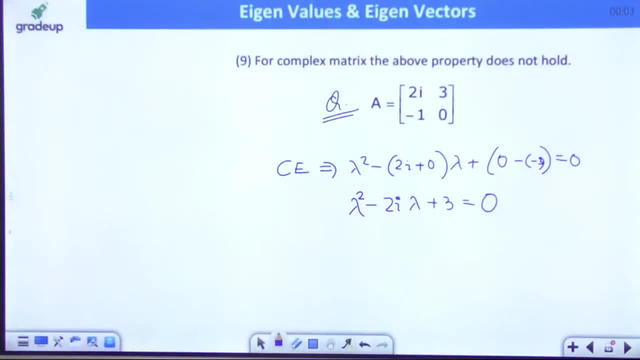 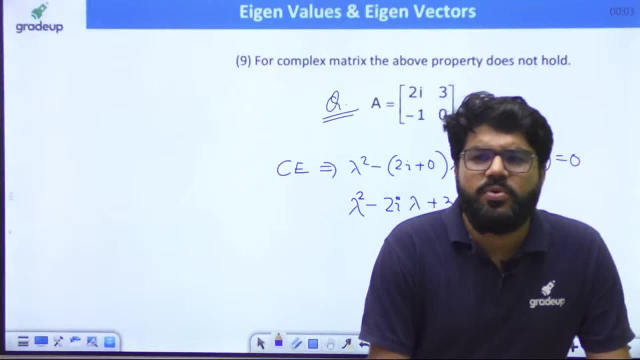 minus 2i lambda plus 3, equal to 0. minus 2i lambda plus 3, equal to 0, everybody. so to find out the eigenvalues everybody. so to find out the eigenvalues everybody. so to find out the eigenvalues lambda. and let me just ask you, let me. 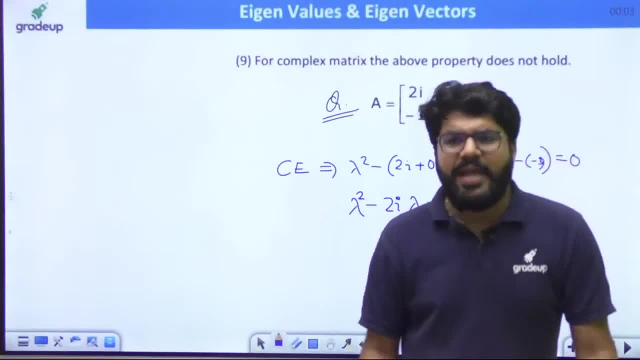 lambda, and let me just ask you, let me, lambda, and let me just ask you, let me just ask you okay, like covering up, just ask you, okay, like covering up, just ask you, okay, like covering up, important questions of linear algebra, important questions of linear algebra, important questions of linear algebra, tomorrow will be the eigenvalue, eigen. 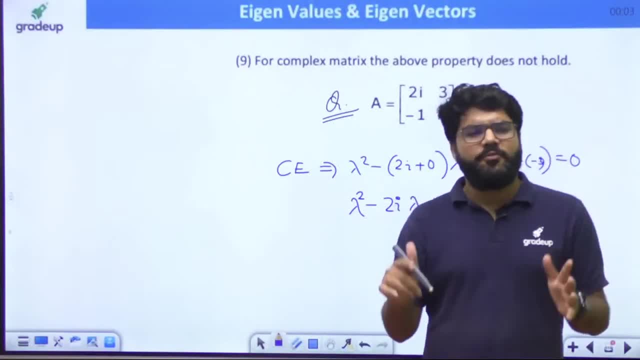 tomorrow will be the eigenvalue eigen. tomorrow will be the eigenvalue eigen, vector part number two. vector part number two. vector part number two. how many of you are looking forward and how many of you are looking forward and how many of you are looking forward and will be interested on a YouTube mentee? 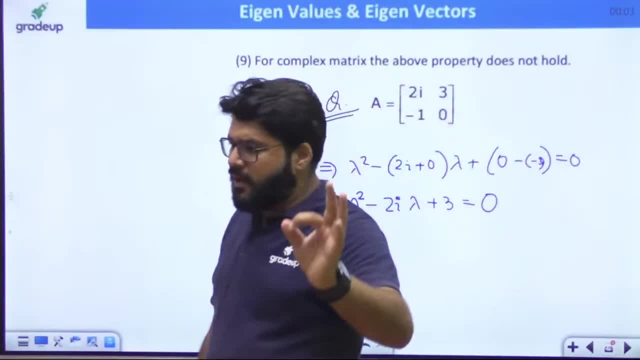 will be interested on a YouTube mentee. will be interested on a YouTube mentee. quiz on linear algebra. how many of you quiz on linear algebra? how many of you quiz on linear algebra? how many of you can be interested for the YouTube mentee? can be interested for the YouTube mentee. 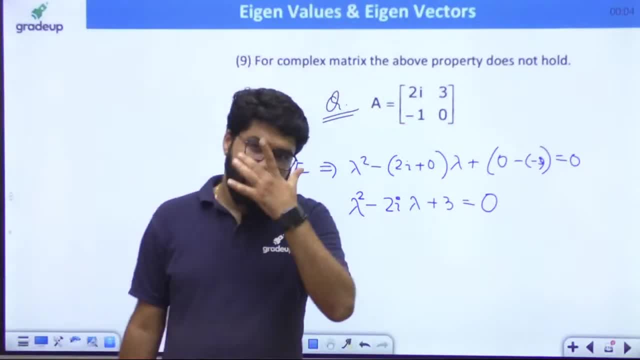 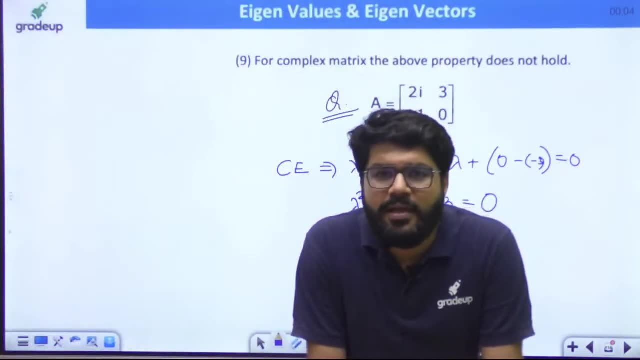 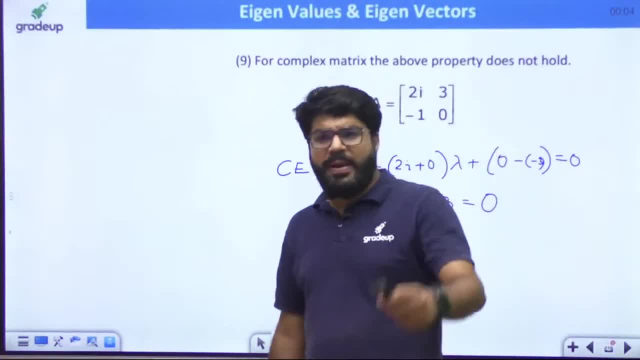 whatever important questions and concepts, whatever important questions and concepts you have learned, can we also plan a mentee you have learned? can we also plan a mentee you have learned? can we also plan a mentee quiz? the you know mentee quiz, YouTube quiz. the you know mentee quiz YouTube. 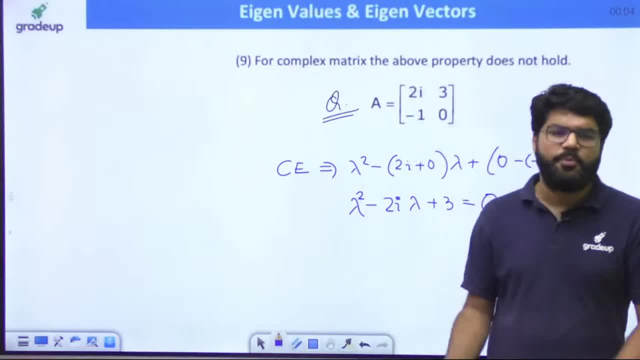 quiz the you know mentee quiz, YouTube as a manipulative quiz to test your as a manipulative quiz to test your as a manipulative quiz to test your knowledge with leaderboard with fun knowledge with leaderboard with fun knowledge with leaderboard with fun based event. okay, with some exciting. 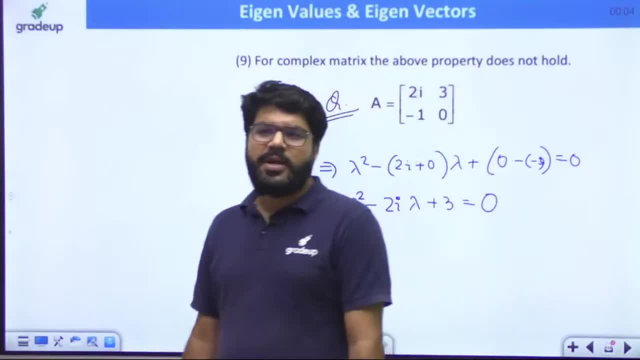 based event. okay, with some exciting based event. okay, with some exciting rewards also with some exciting prices. rewards also with some exciting prices, rewards also with some exciting prices also. so let me see your interest level also. so let me see your interest level also. so let me see your interest level, then I can plan a mentee quiz so that 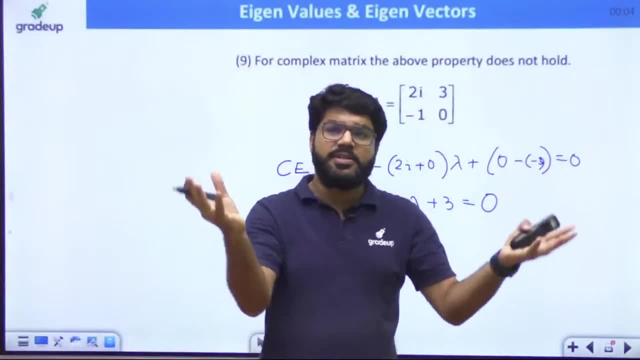 then I can plan a mentee quiz, so that then I can plan a mentee quiz, so that will summarize. you know that will, will summarize. you know that will, will summarize. you know that will summarize, that will summarize even some summarize, that will summarize even some summarize, that will summarize even some more questions. okay, for our questions. 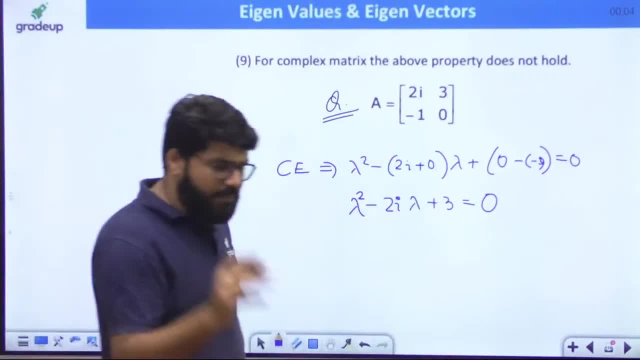 more questions: okay for our questions. more questions: okay for our questions. miscellaneous questions: Linga. miscellaneous miscellaneous questions: Linga. miscellaneous miscellaneous questions: Linga. miscellaneous questions: Linga. but let me see questions Linga. but let me see questions Linga. but let me see the number of comments and then I'll. 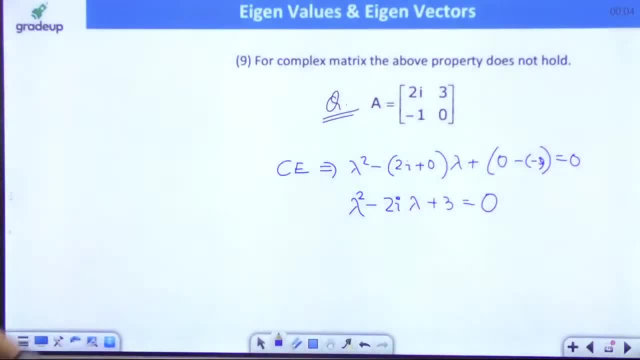 the number of comments and then I'll the number of comments and then I'll decide. everybody, let me know, decide everybody, let me know, decide everybody, let me know. solo. so lambda square minus 2i. lambda solo. so lambda square minus 2i. lambda solo. so lambda square minus 2i. lambda plus 3, equal to the 0 ticker. so yeah, 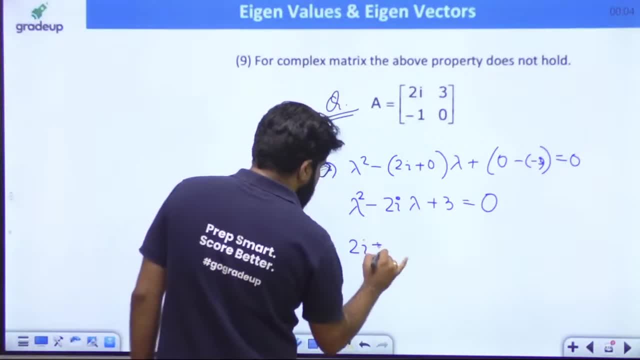 plus 3 equal to the 0 ticker. so yeah, plus 3 equal to the 0 ticker. so yeah. ketna ho jayega lambda is minus B plus. ketna ho jayega lambda is minus B plus. ketna ho jayega lambda is minus B plus minus. root over B square, that is minus. 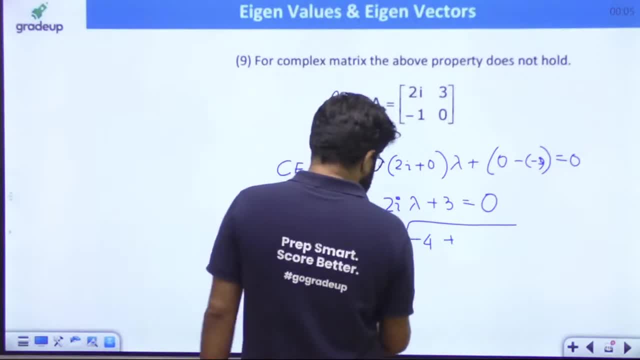 minus root over B square. that is minus minus root over B square. that is minus 4. 2i square minus 4 plus sorry B square 4. 2i square minus 4 plus sorry B square 4. 2i square minus 4 plus sorry B square minus 4. AC to minus 12 whole divided by: 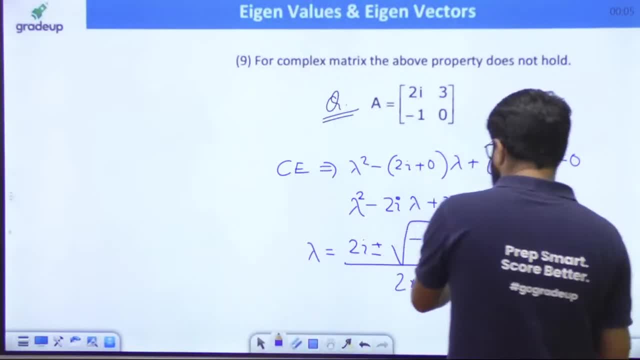 minus 4 AC to minus 12 whole divided by minus 4 AC to minus 12 whole divided by 2a. so you hope your 2i plus minus under 2a, so you hope your 2i plus minus under 2a, so you hope your 2i plus minus under root of minus 16 is 4i divided by 2. so 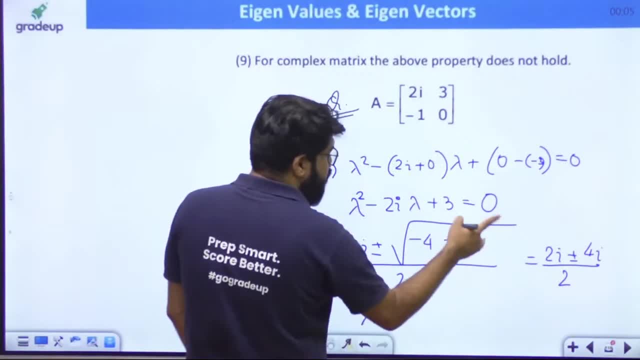 root of minus 16 is 4i divided by 2. so root of minus 16 is 4i divided by 2. so see lambda coming up here: is 2i plus 4i. see lambda coming up here: is 2i plus 4i. 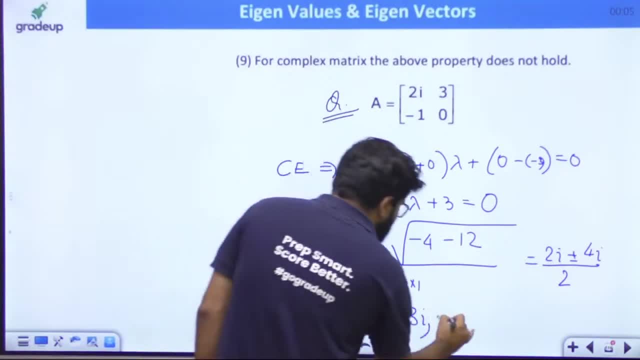 see lambda coming up. here is 2i plus 4i, 6i by 2 is 3i minus 2i by 2 minus I, and 6i by 2 is 3i minus 2i by 2 minus I and. 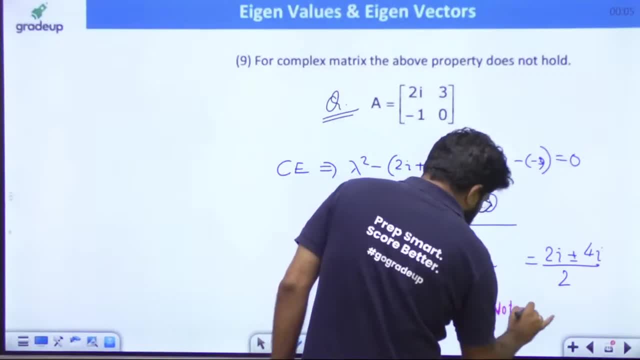 6i by 2 is 3i minus 2i by 2 minus I, and does it make the conjugate pair? no, does it make the conjugate pair? no, does it make the conjugate pair? no, these are not conjugate pair. this is not. 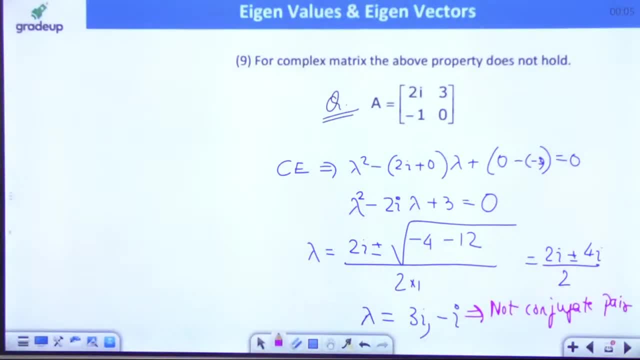 these are not conjugate pair. this is not. these are not conjugate pair. this is not the conjugate pair. this is not the the conjugate pair. this is not the conjugate pair. okay, not the conjugate conjugate pair. okay, not the conjugate conjugate pair. okay, not the conjugate pair. mente quiz, you can feel an? 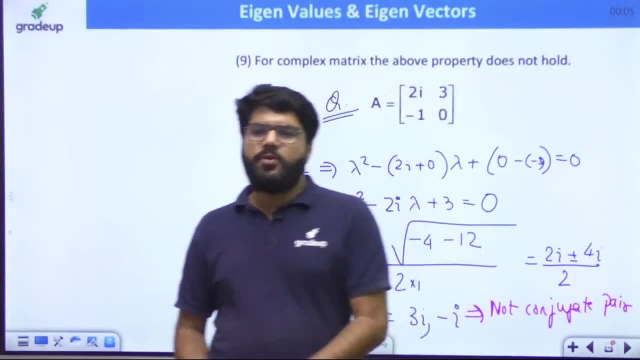 pair mente quiz. you can feel an pair mente quiz. you can feel an interactive quiz on YouTube. interactive quiz on YouTube. interactive quiz on YouTube. okay, interactive quiz on the YouTube there. okay, interactive quiz on the YouTube there. okay, interactive quiz on the YouTube. there will be the interactive quiz of the. 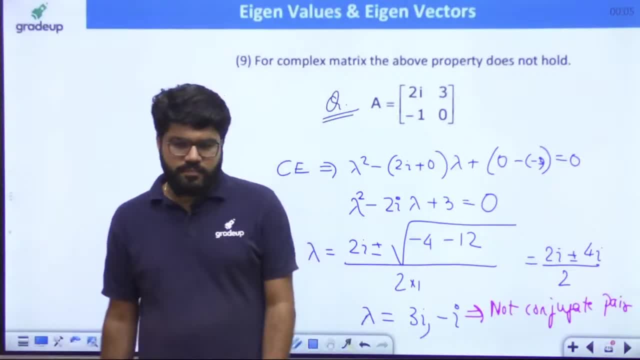 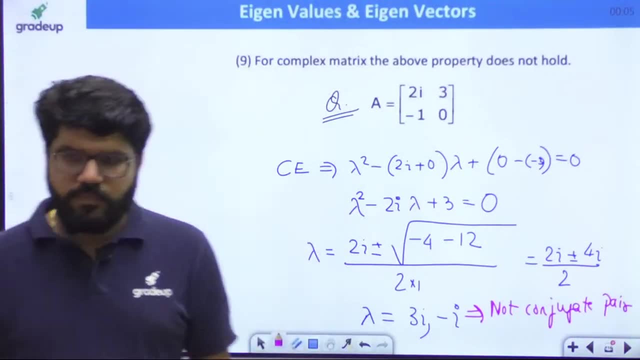 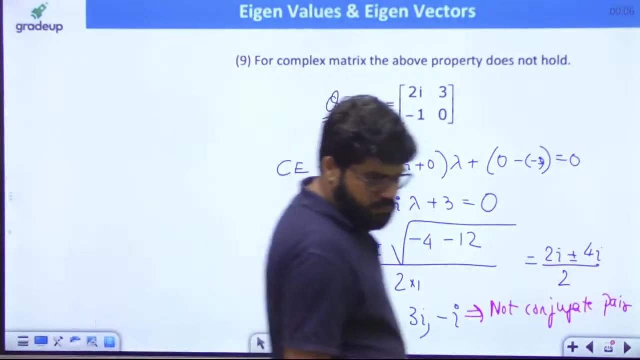 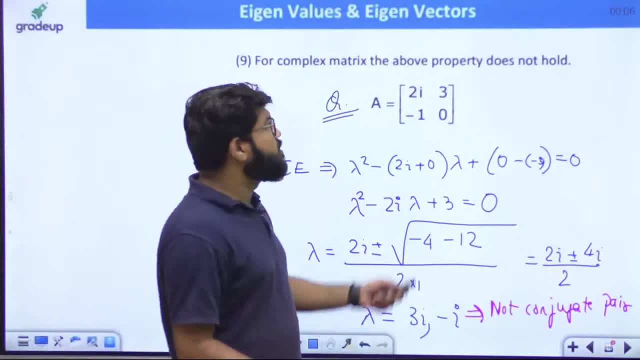 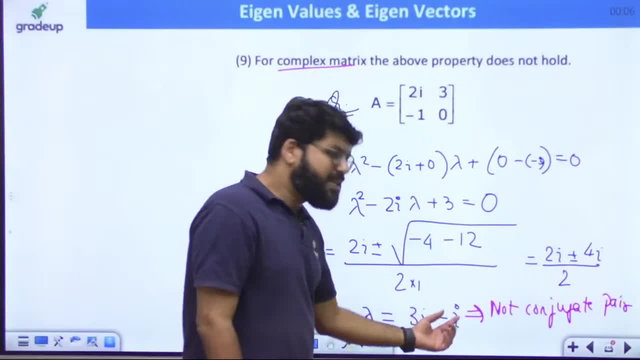 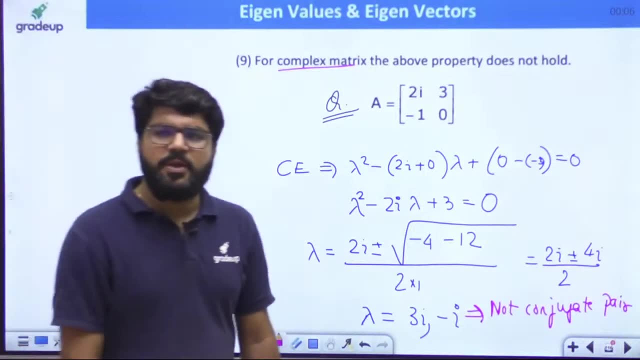 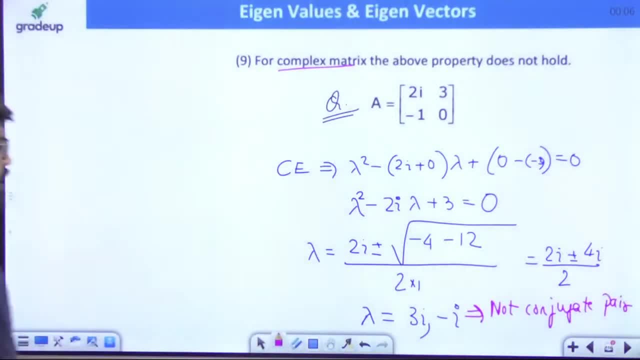 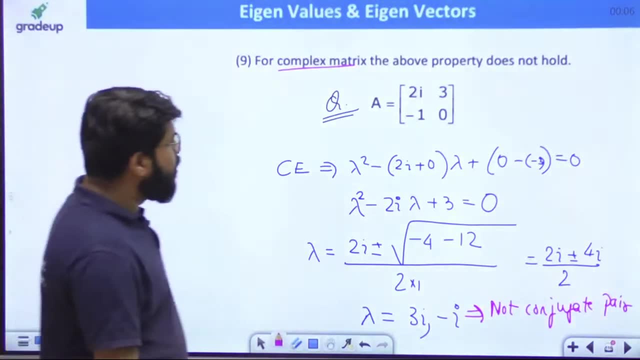 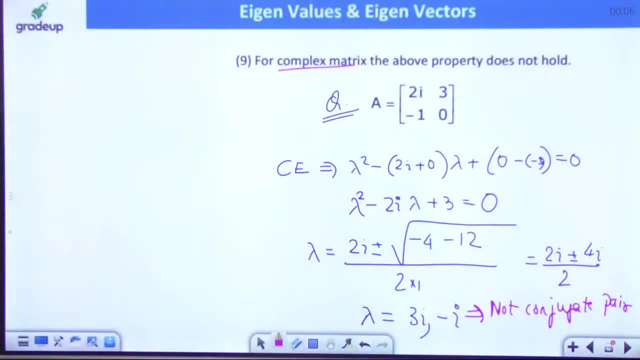 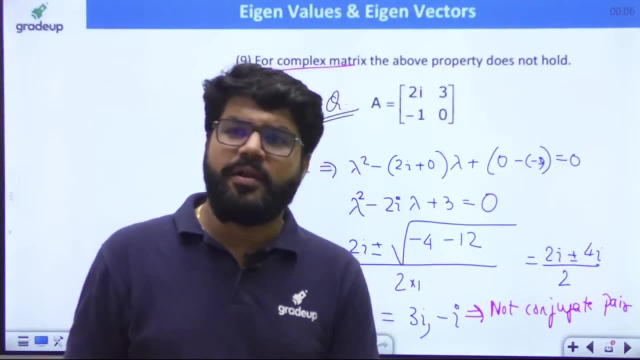 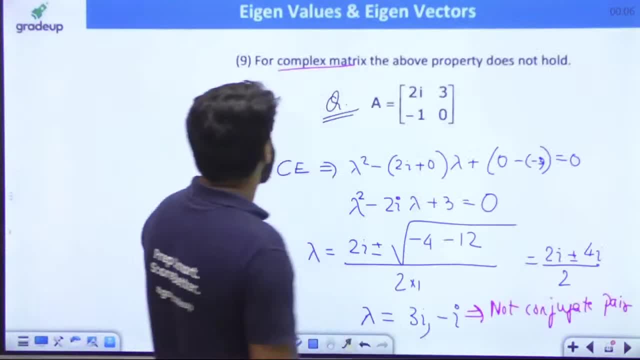 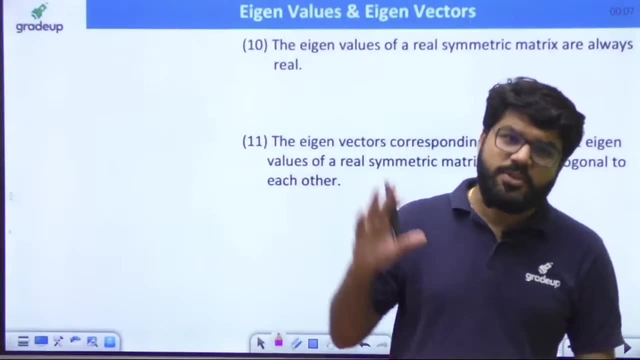 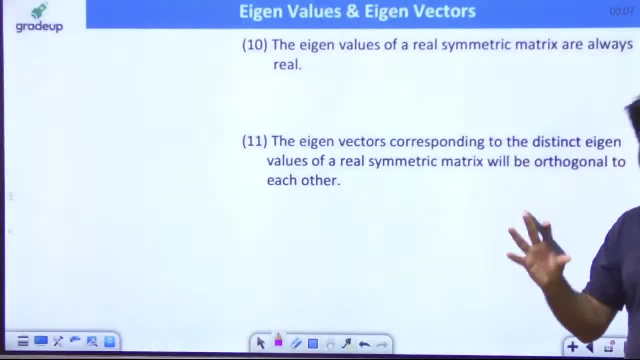 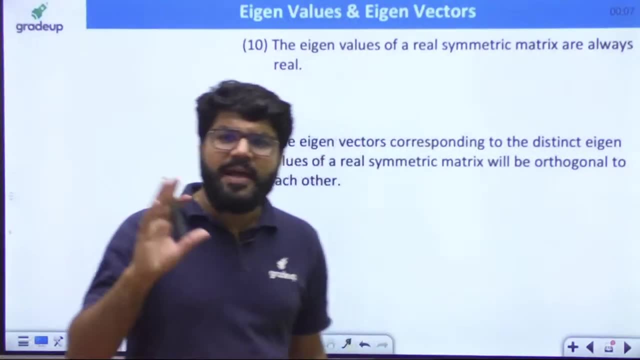 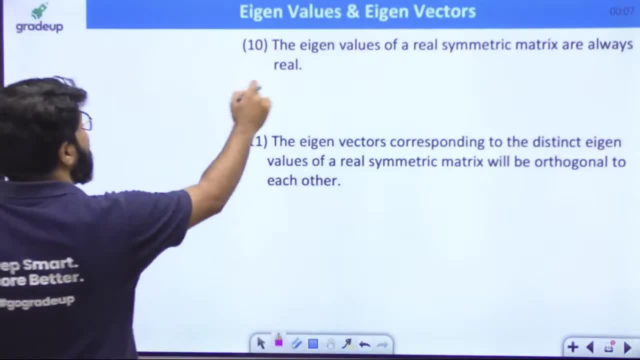 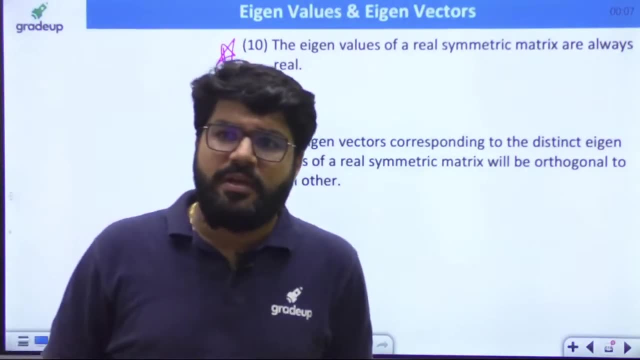 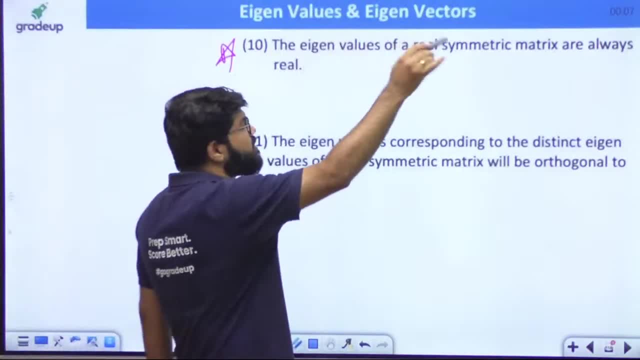 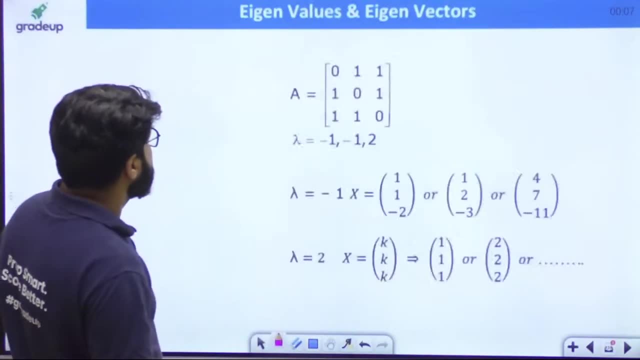 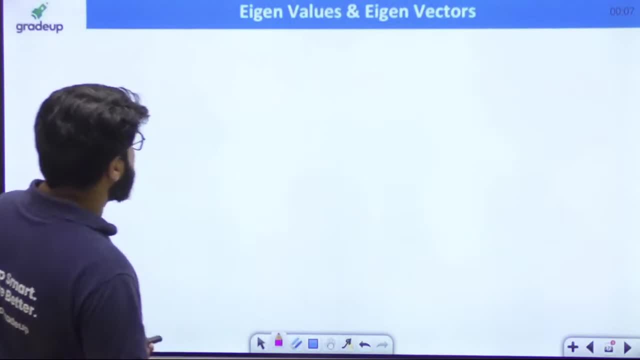 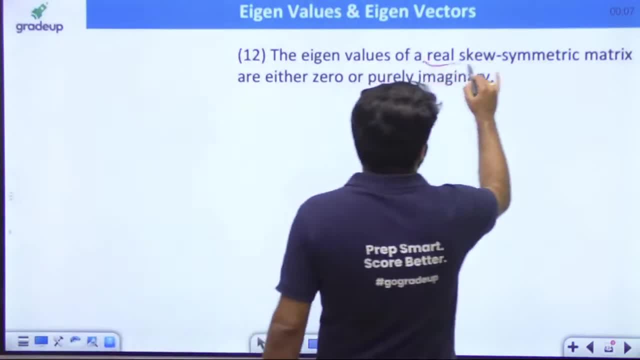 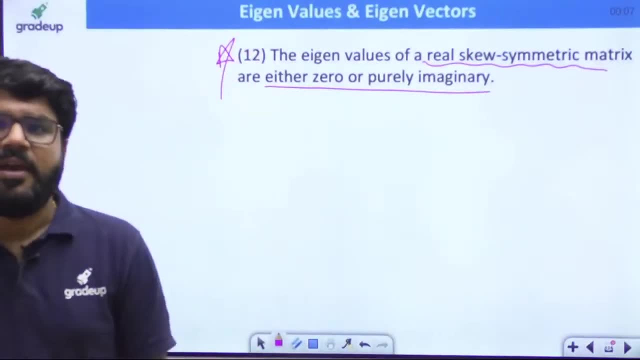 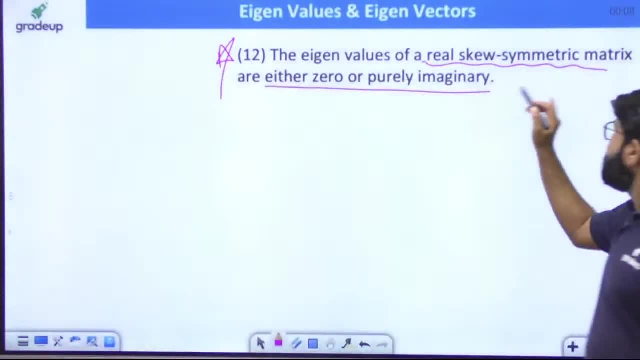 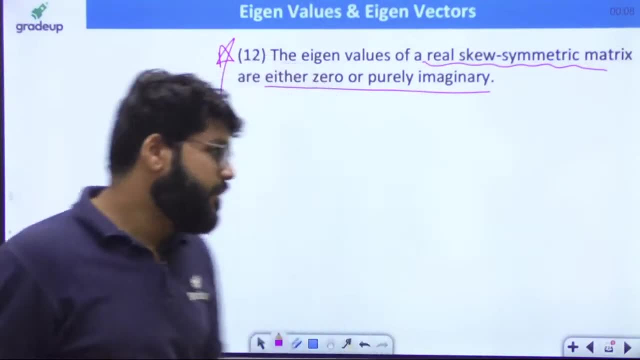 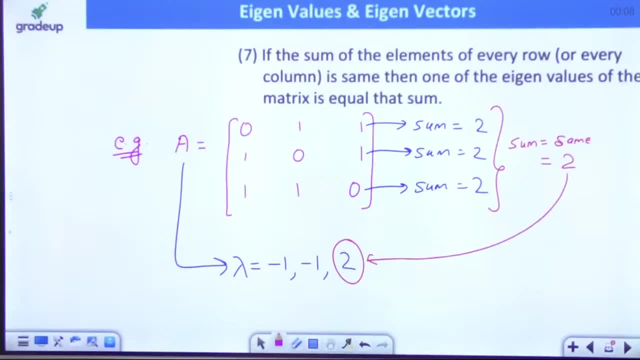 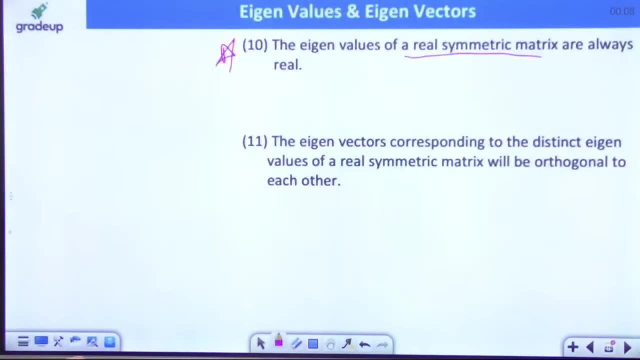 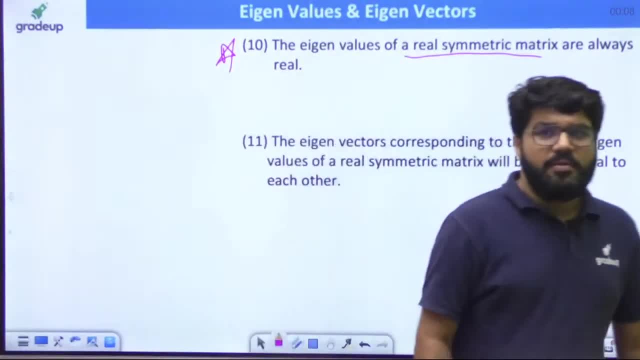 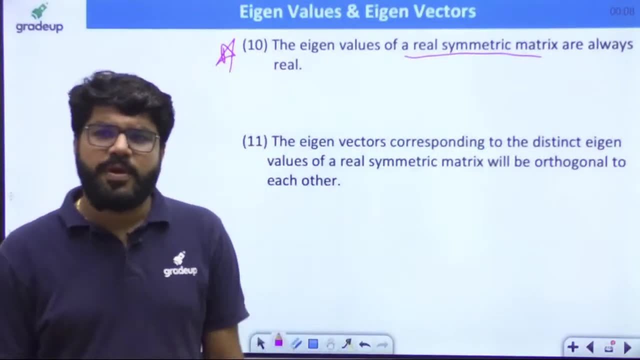 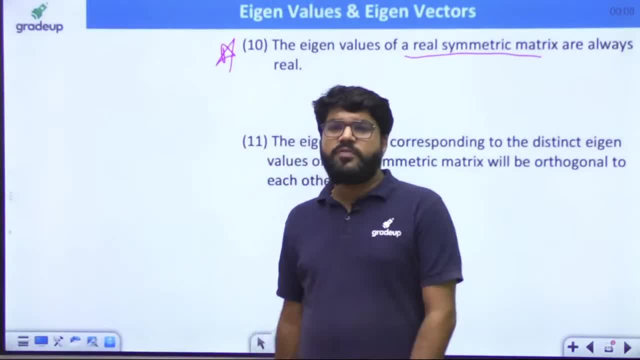 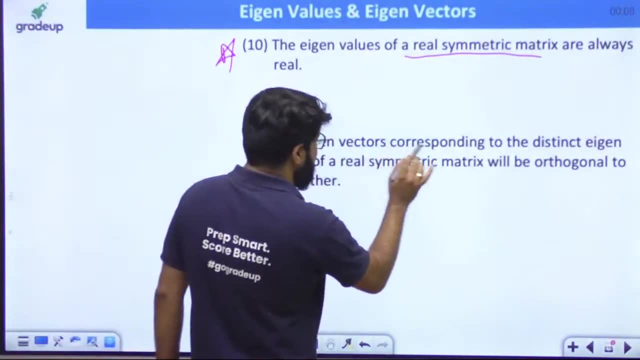 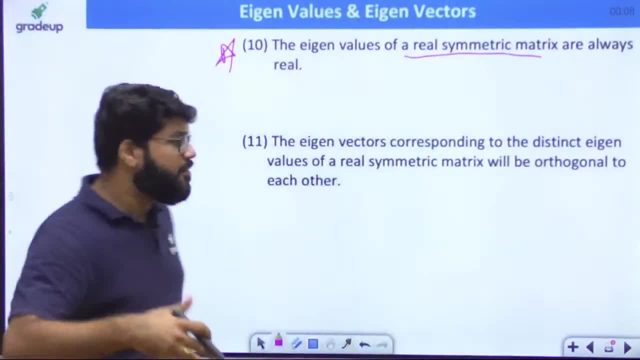 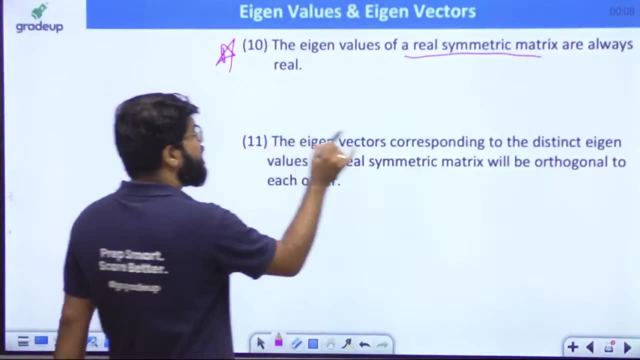 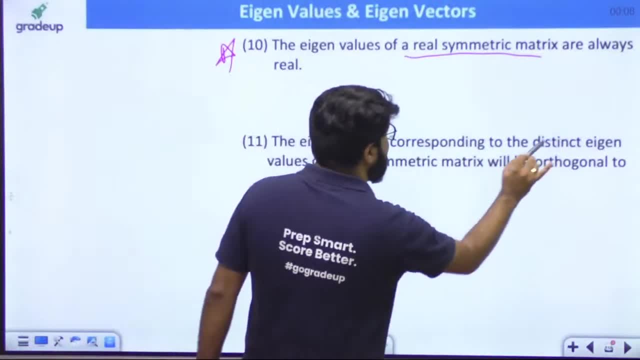 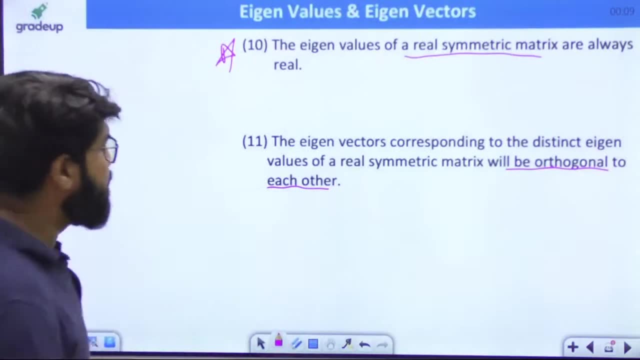 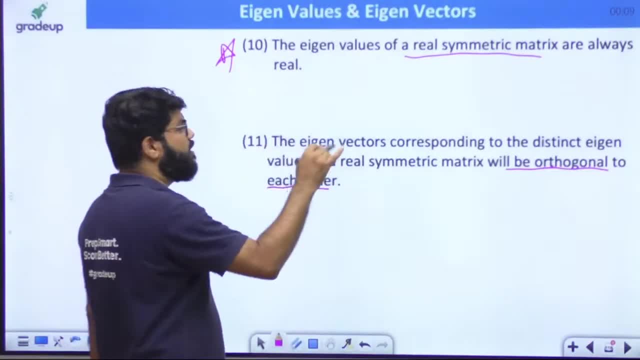 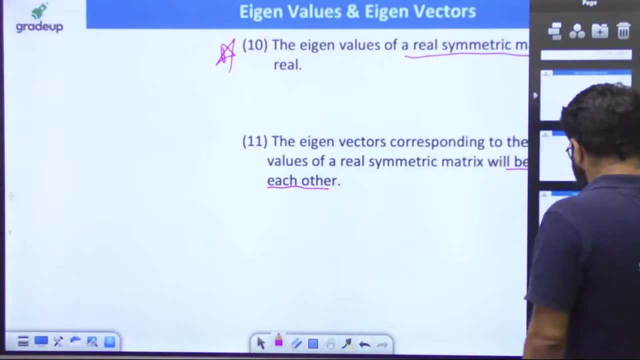 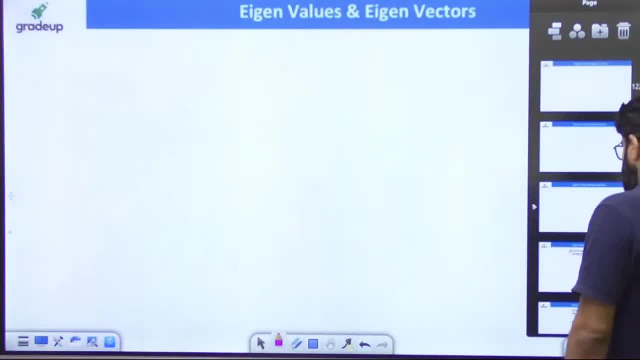 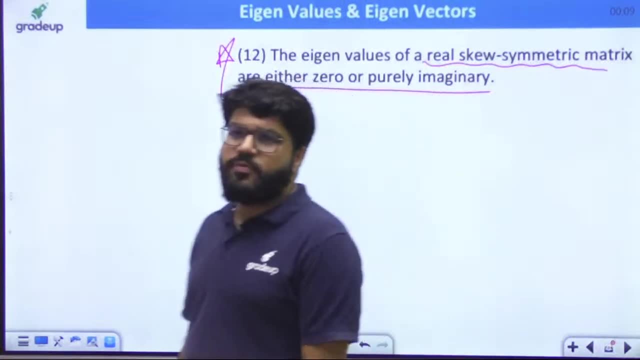 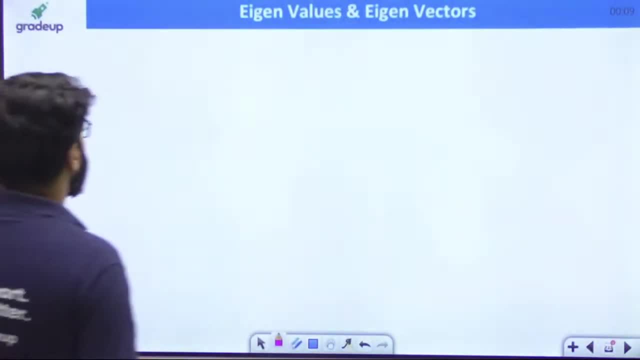 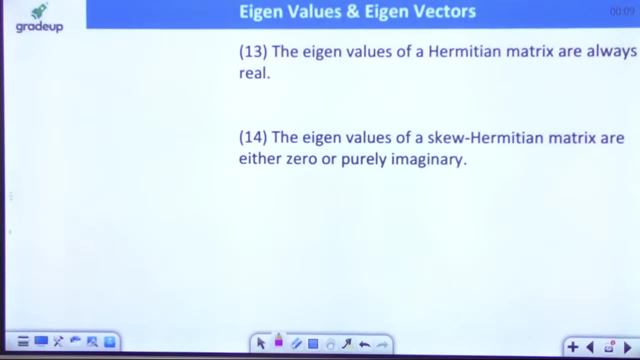 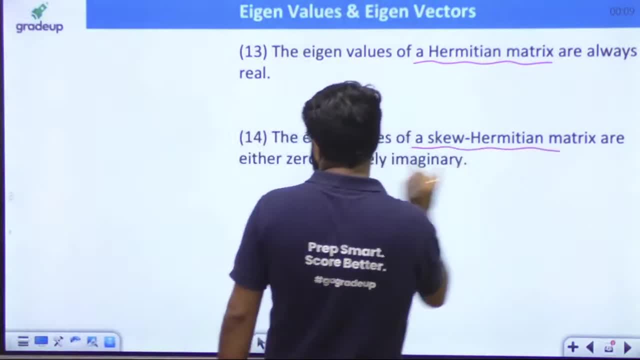 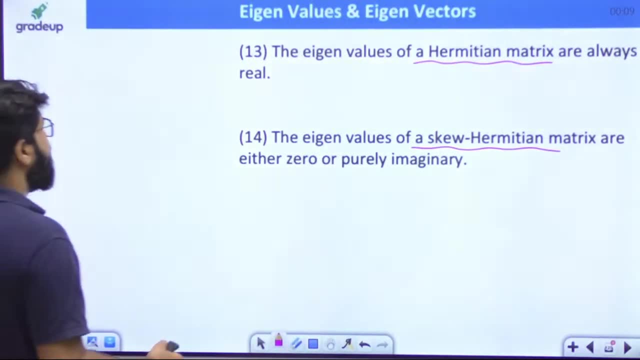 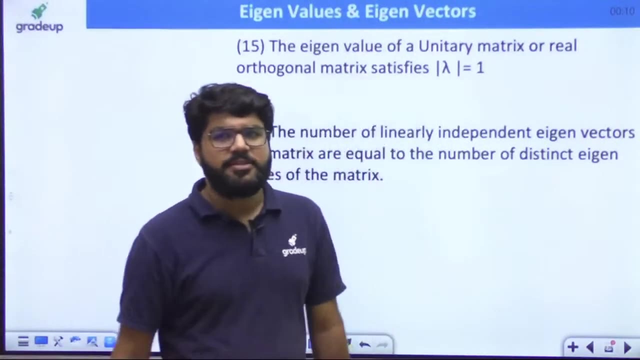 one mark question and eigenvalues of a skew hermitian matrix are again either 0 or pure imaginary, or either 0 or pure imaginary, right, I hope you know what is hermitian, what is skew hermitian? okay, orthogonal means perpendicular, eigenvectors being perpendicular to each other. 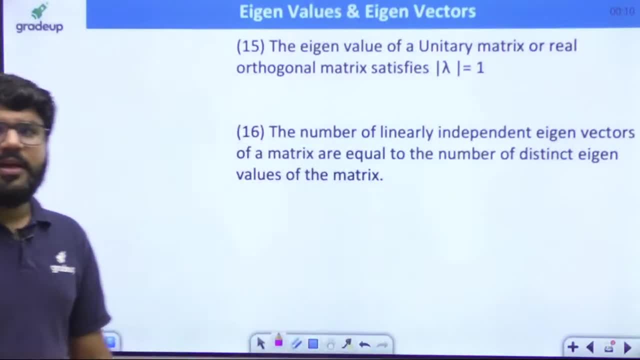 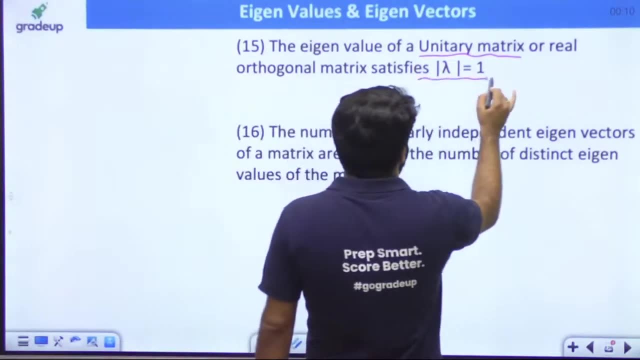 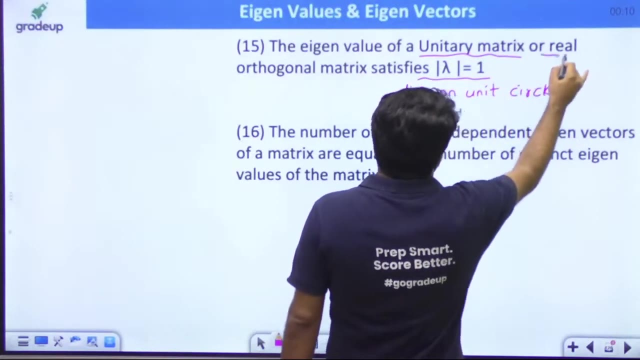 for gap perpendicular: the dot product in a product 0 eigenvalues of a unitary matrix, of all a real orthogonal matrix, will lie on unit circle. will lie on the unit circle. okay, eigenvalues of a real orthogonal matrix or a unitary matrix will lie on the unit circle. so of course in this 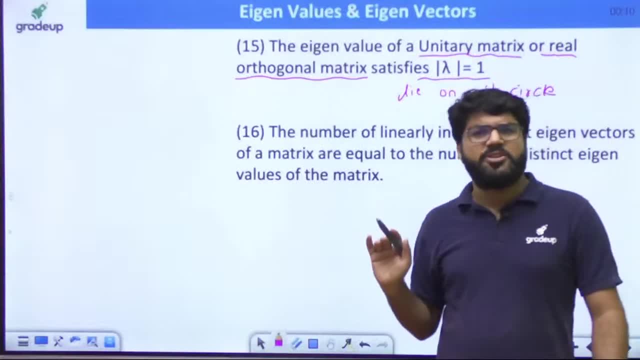 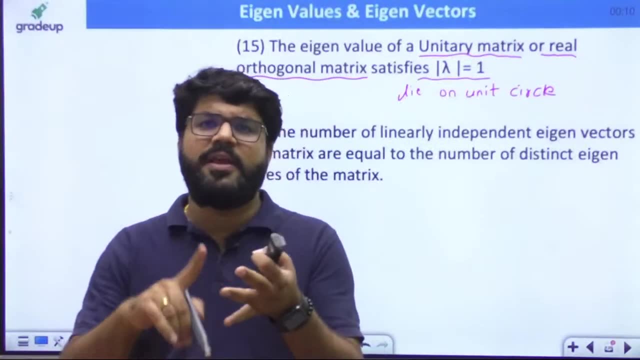 series. I have not taken the basics of matrix, I have not taken the classification of matrix, so you can just go through them once. okay, what is skew symmetric? what is symmetric? what is hermitian? what is skew hermitian? what is orthogonal matrix? what is unitary matrix and etc. okay, the number of linearly independent. 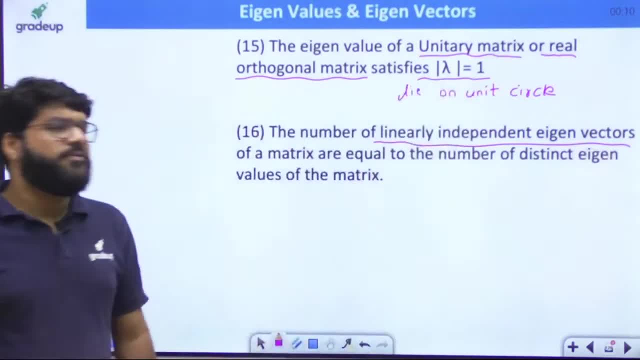 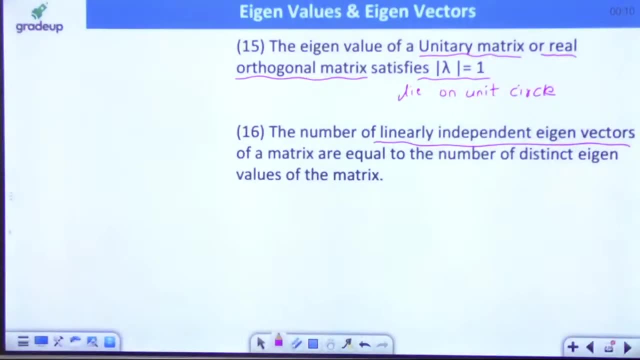 eigenvectors of a matrix is equal to the number of distinct eigenvalues of the matrix. is equal to the number of distinct eigenvalues of the matrix. the number of linearly independent eigenvectors of a matrix are equal to the number of number of distinct eigenvalues. 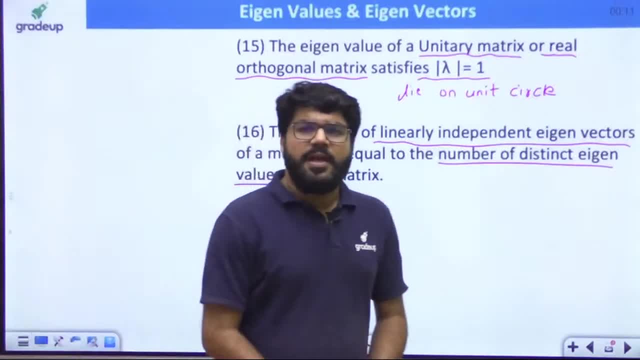 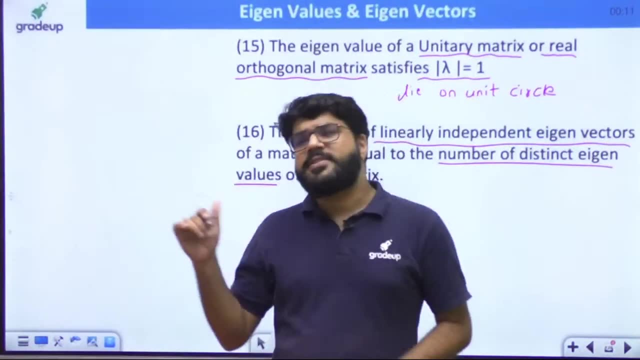 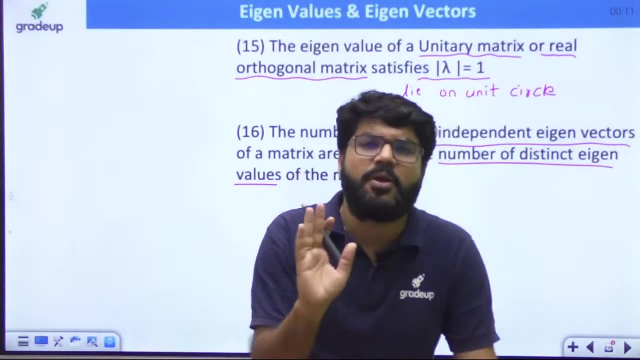 different eigenvalues. right, okay, practice will remember everything, pk. so the last six, seven properties which I have told, pay attention, the last six to seven properties that I have told is important, mostly for factual questions or for some indirect one mark question. what are those indirect questions? I will show. 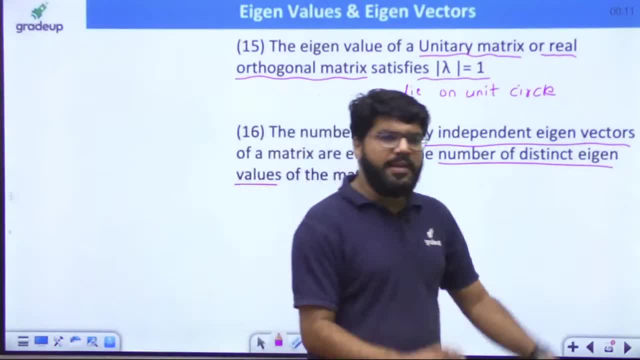 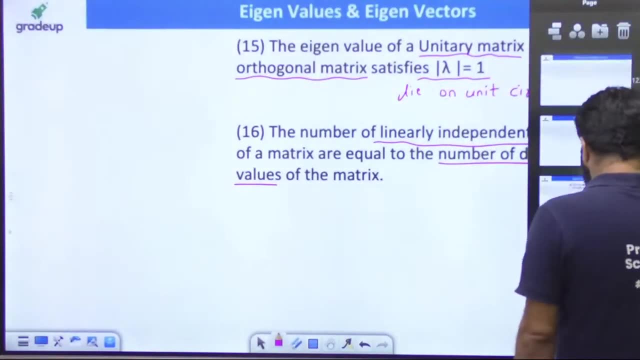 you that tomorrow? okay, I will show you that tomorrow, because tomorrow will be a continuation of the today's class. don't worry, tomorrow will be the continuation of the today's class. okay, now let's go to one one more case. okay, let us go to the one more case which I'm going to cover up here. just wait a second. 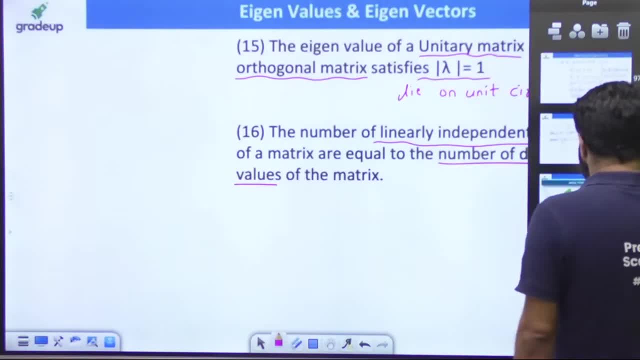 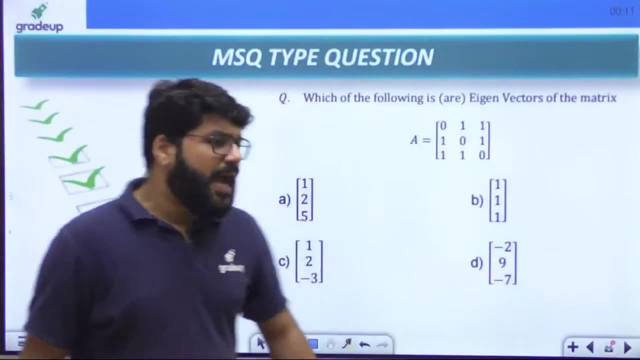 okay, yes, yeah, I'm a list of Sarah properties deca. now let us come to one eigenvector question now. there can be various question on eigenvector coming up tomorrow, but one question of eigenvector and I am selecting it as a multiple select question. I am choosing a multiple select question. 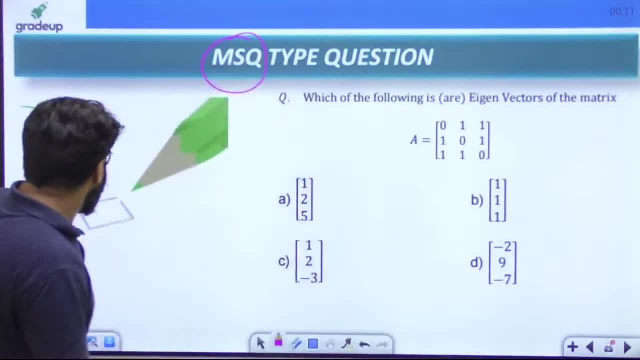 msq type question. you know what is multiple select question, where one or two or even third, one or two or three or four, maybe all options are there and right now you are considering it as a multiple select question and you will get to the next question. it is one or two or 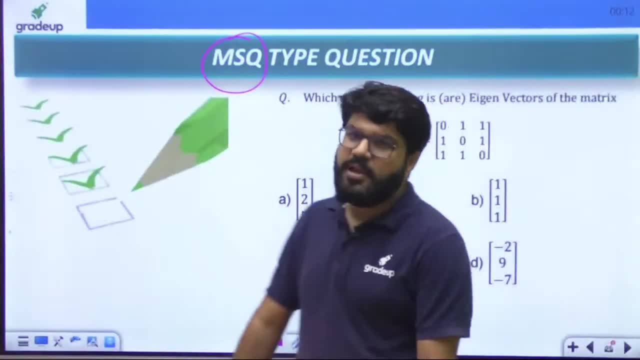 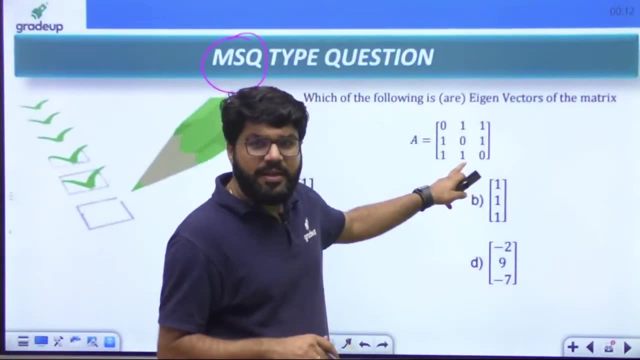 even third, one or two or three or four, or maybe all options are available. so this is the can also be correct. That is what is a multiple select question. Which one of the following is, or are eigenvectors of the given matrix? The matrix is same. We have solved the eigenvalue of this. 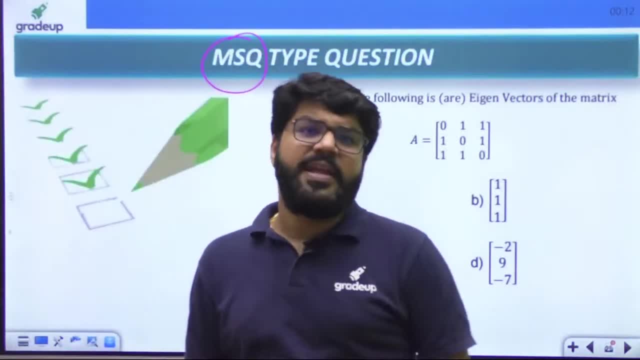 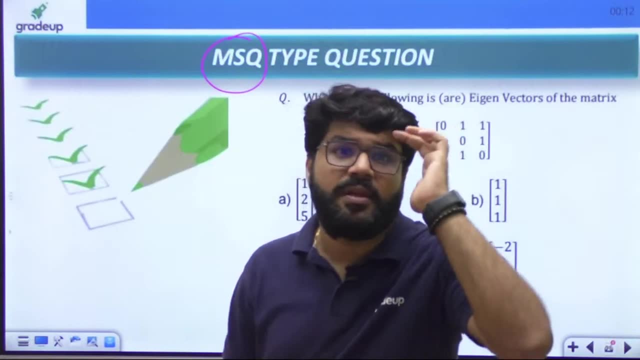 matrix Eigenvector. Solving in detail for eigenvector is of course lengthy, But how can I solve the objective MCQ or MSQ or NAT type question? There can be even NAT question on eigenvectors. I will show you tomorrow. But let us learn that whenever there is a competitive 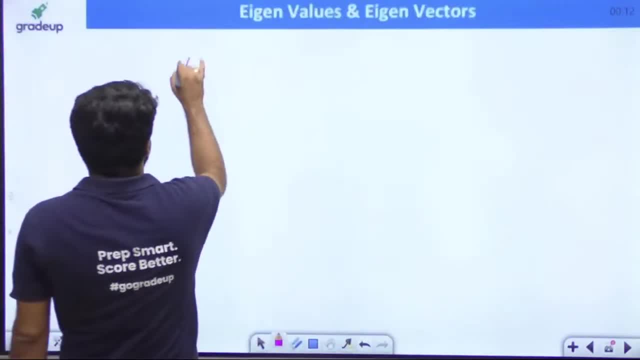 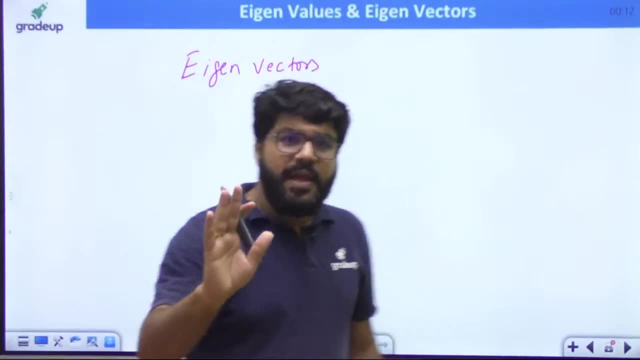 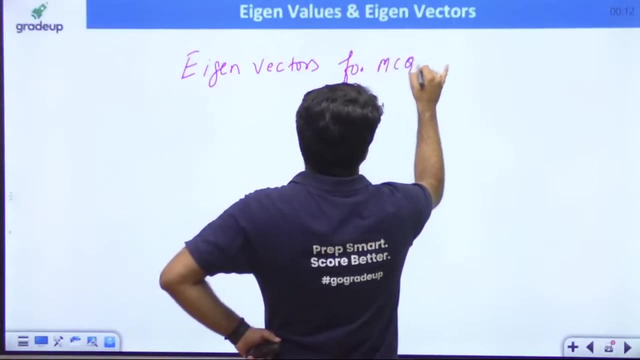 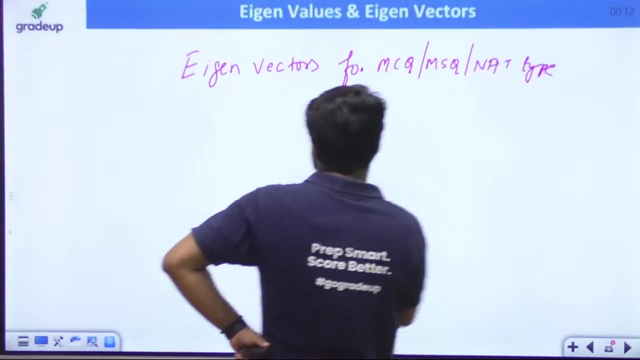 question, whether it is MCQ or MSQ, Okay, Everybody, please make a note, Very important point, And then from this point I will solve all the eigenvector questions and tell you all All One type of question: Eigenvectors, Okay For MCQ, or whether it is MSQ or NAT type, Whenever the question is. 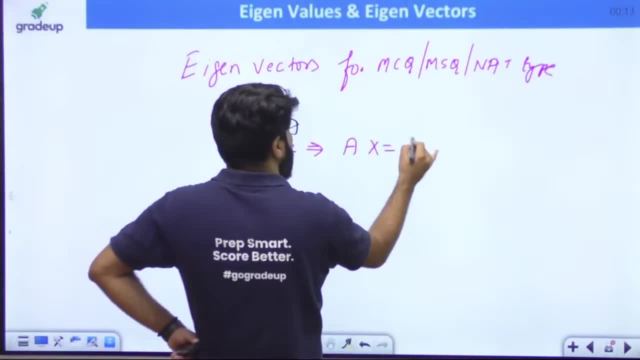 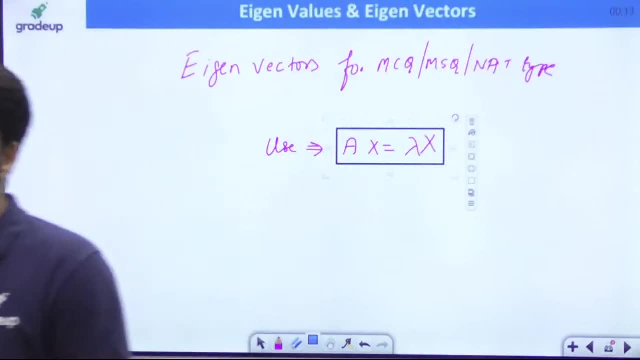 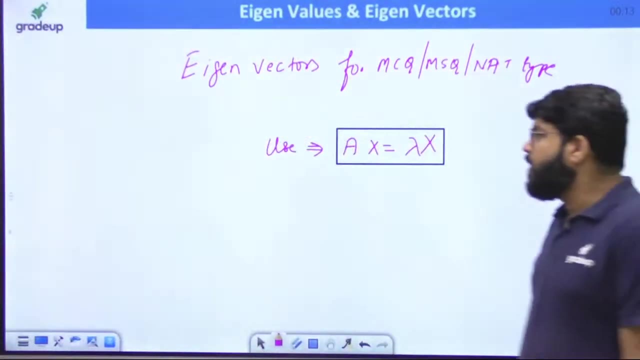 used the basic definition of eigenvector. What was the basic definition of eigenvector from which we started? AX equal to lambda X- The vector X satisfying AX equal to lambda X- The vector X, such that AX equal to lambda X is known as the eigenvector. So can we try this with the options? 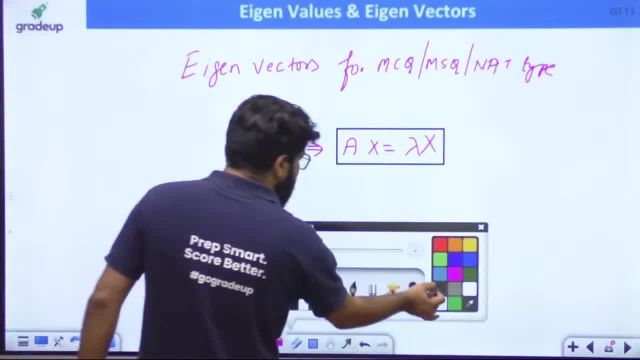 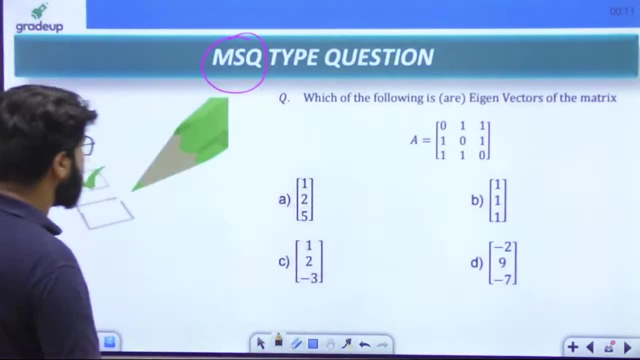 Yes, We can try this with the options. So there is a matrix given to you And there are four options And I need to check all four because this is a MSQ question, Intentionally when I MSQ here, so that we have to check with all options. Option number A. Option number A: A. 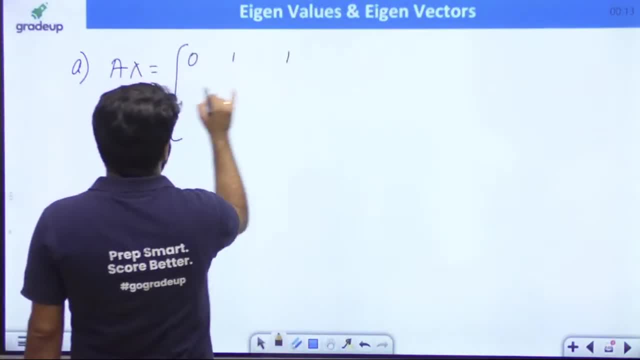 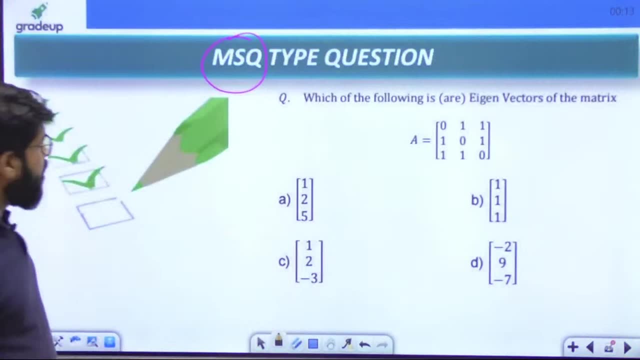 into X. Okay, What is the A matrix? 0, 1, 1, 1 0, 1 1 1 0.. Multiplied by the X vector. What is the X vector of the option number A, Sir? it is 1.. It is 2.. It is 5.. It is 1, 2, 5.. Okay, Now multiply How. 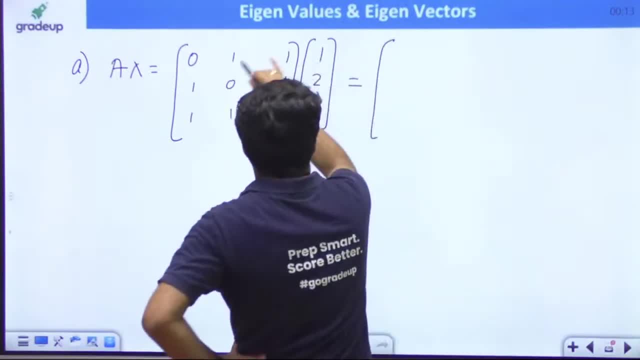 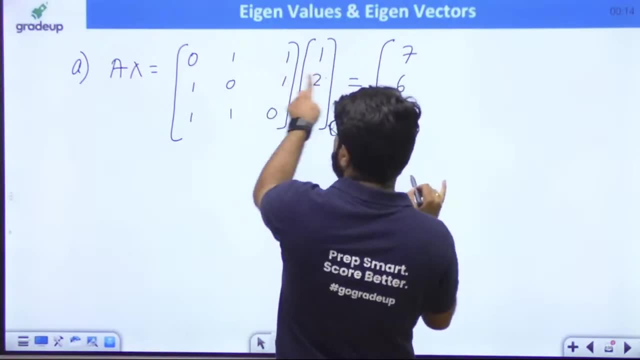 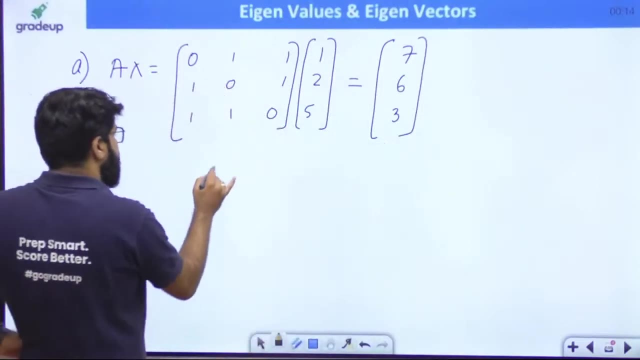 do you multiply? You know to multiply the matrix First row into first column. So 0 plus 2 plus 5.. 7.. 1 plus 0 plus 5.. 6.. 1 plus 2 plus 0.. That becomes 3.. 7, 6, 3.. Now my question is My question. 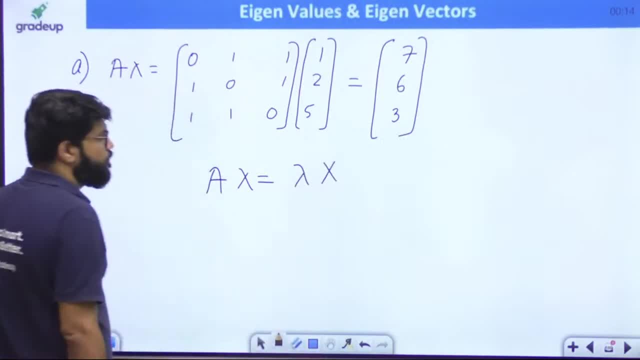 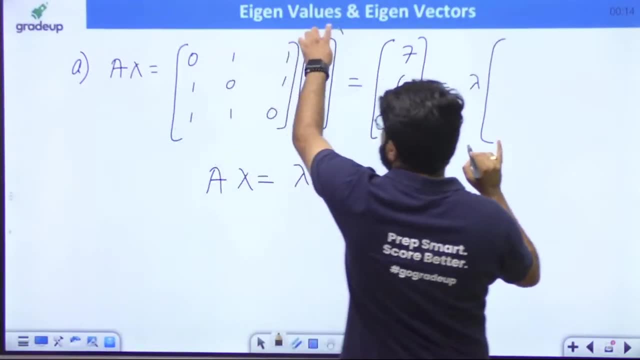 is: Is AX equal to lambda X? Why is AX equal to lambda X? Can this be written as lambda into X? What is the X? This part is the X. Can this be written as lambda into 1, 2, 5?? Can you write it? 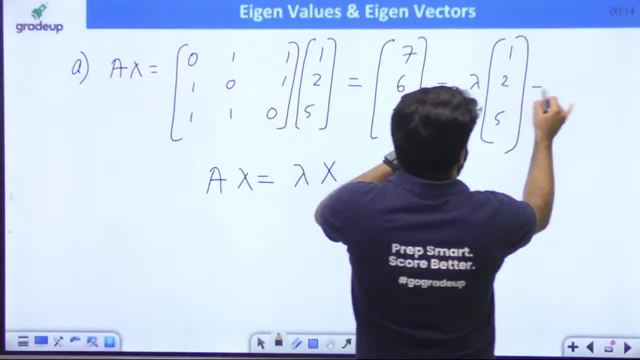 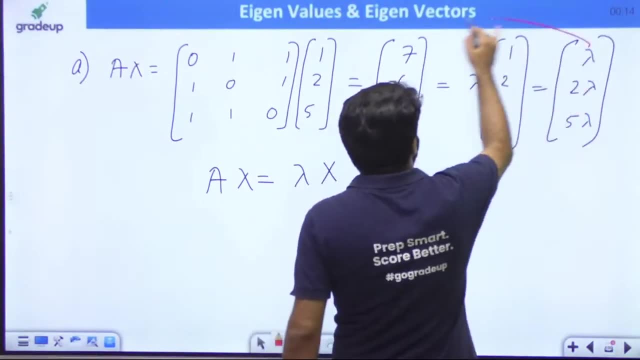 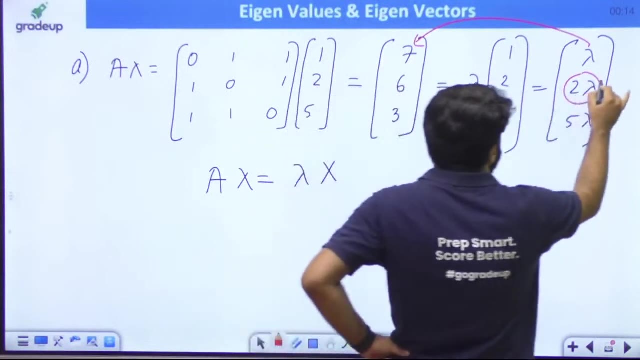 This is true, Suppose. if this is true, Then what should be the value of: lambda- This is done. Lambda- this is done. 2 lambda- this is done. 5 lambda- Suppose. if this was true, Okay, Then lambda should be 7.. But, but, but, but, but. If lambda is 7, then 2 lambda- Okay, Should be 14.. Okay, 5. 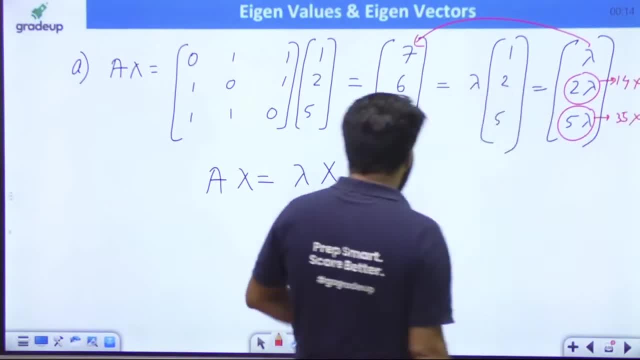 lambda should be 35. So this does not match. This is 6.. This is 3.. So, of course, the left hand side not equal to right hand side, And if this is true, Then what should be the value of lambda? 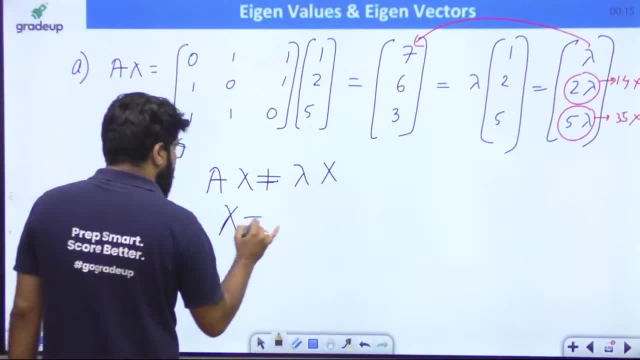 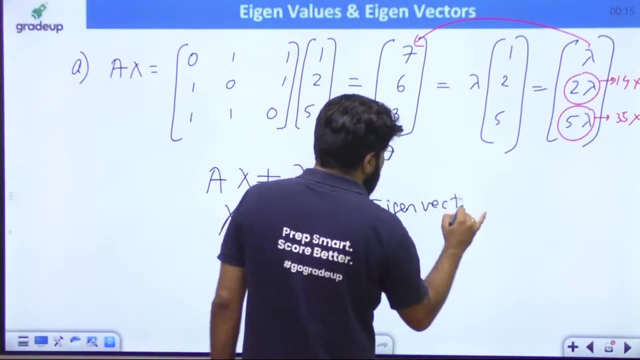 AX is not equal to lambda X And if AX not equal to lambda X, X is not an eigenvector. If it does not satisfy AX equal to lambda X, It is not an eigenvector. It is not an eigenvector If there is. 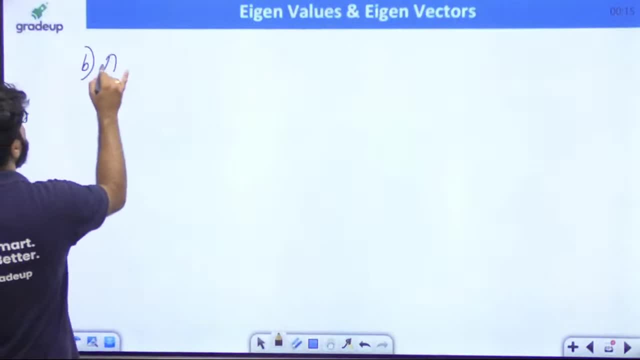 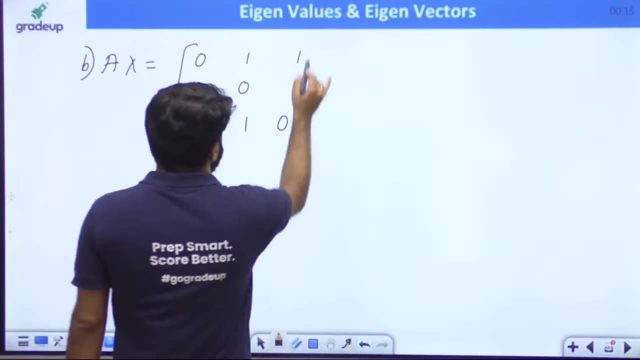 any doubt? Then let us study the second option more. For any confusions of the calculation, Please follow the second option. I will again multiply the matrix A with the eigenvector X. Now, what is the eigenvector X here, See? 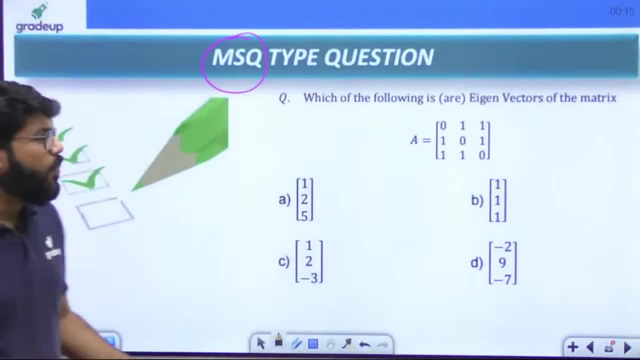 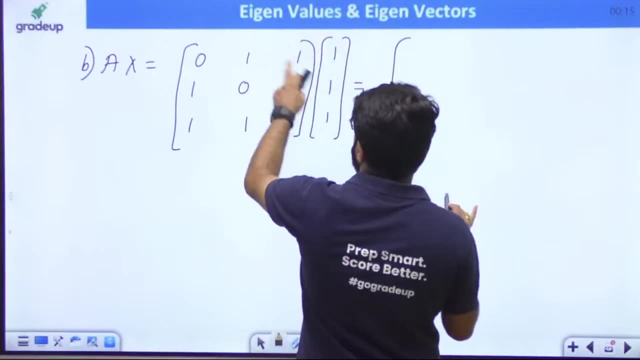 What is the eigenvector X here? 1, 1, 1.. Option number B: 1 1, 1.. Take this: Option number B: 1, 1, 1.. And that is equal to first row 0.. Then 1., Then 1.. This is 2.. Then 1, 0, 1.. This is also 2.. Then, on the third: 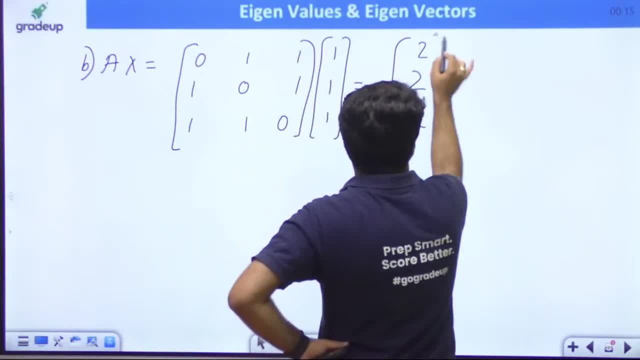 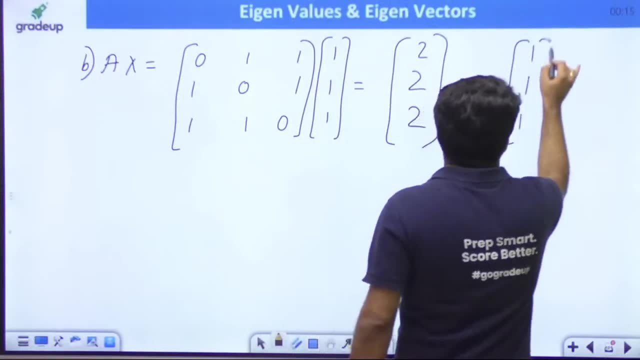 row 1 into plus 1 plus 0. This is also 2.. This is perfectly 2 2 2.. So what I can easily do: I can take the 2 common And then write down 1 1 1.. I can take the 2 common and write down 1 1 1.. And 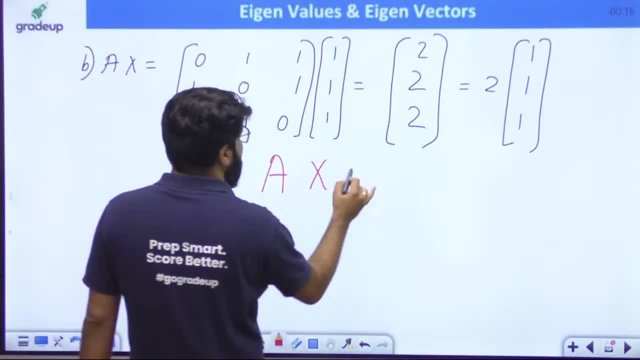 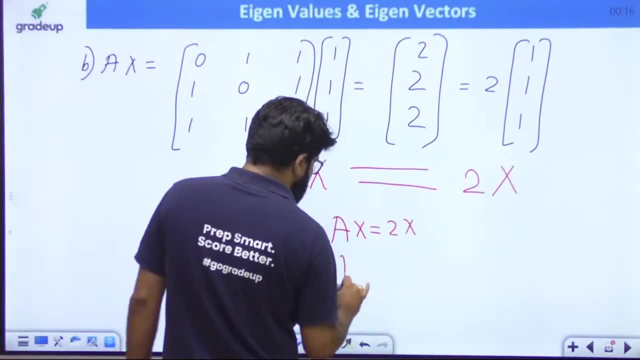 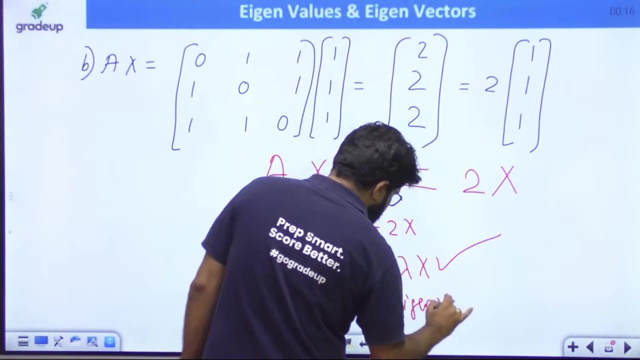 now, clearly, I am able to say that this is: A into X is equal to some number, 2 into X, AX equal to 2, X AX equal to lambda. X is satisfied. So X is an eigenvector, X is an eigenvector. Yes, sir, This. 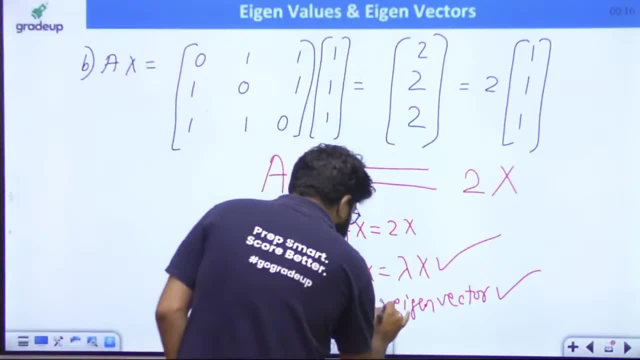 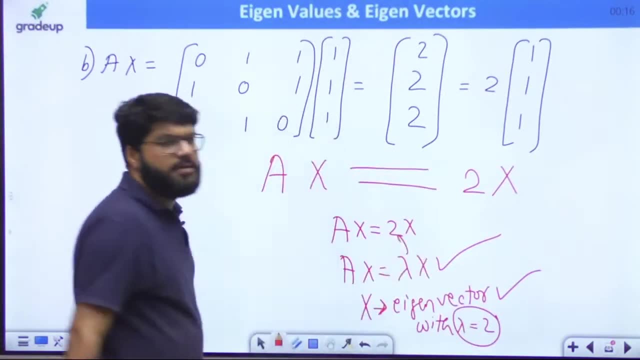 possible vector in the option number B is an eigenvector, Is an eigenvector with corresponding eigenvalue. What is the corresponding eigenvalue, Boss? lambda instead of 2 came Right, Lambda, equal to 2.. Everybody, Everybody Next. So 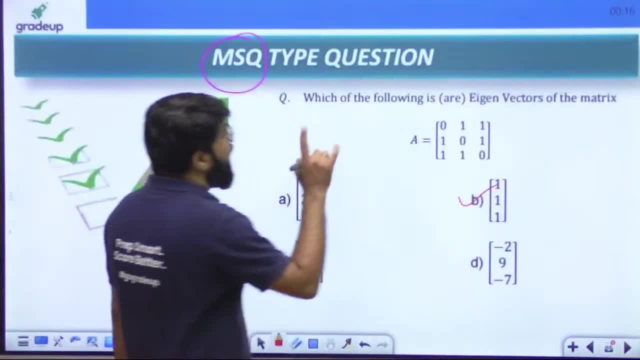 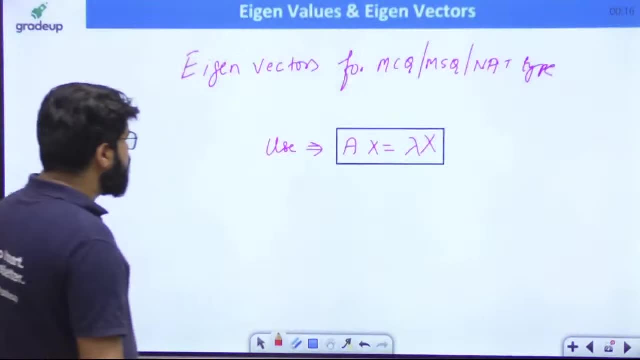 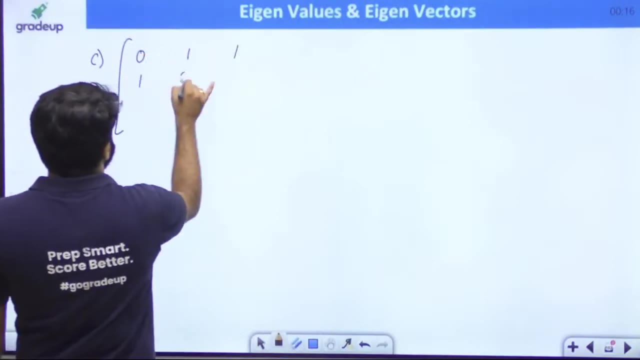 definitely, definitely. option number B is correct, But I cannot stop with any one option because it is multiple. select More than one can also be correct. So I need to check for C now: 1, 2 minus 3.. 1, 2 minus 3. 0, 1, 1. 1 0. 1. 1 1 0.. 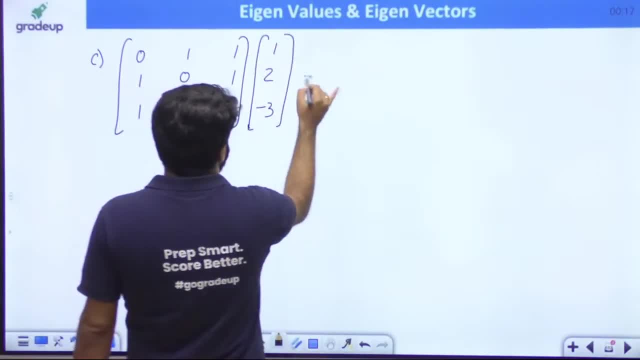 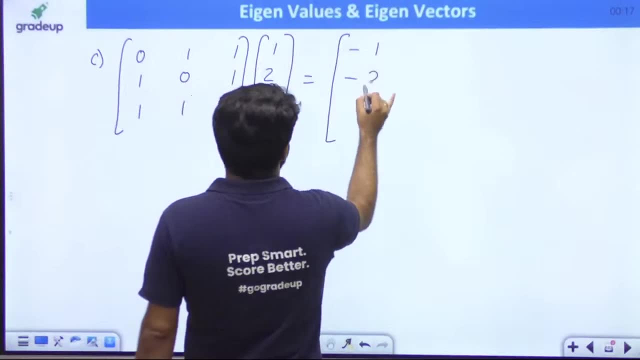 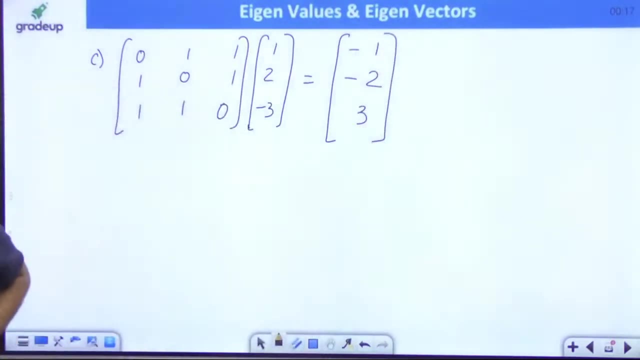 1, 2 minus 3 is equal to how much? 0, 2 minus 3, which is minus 1.. 1, 0 minus 3, which is minus 2.. 1 plus 2 plus 0, which is equal to 3. Which is equal to 3.. Right Now, now, now, I just. 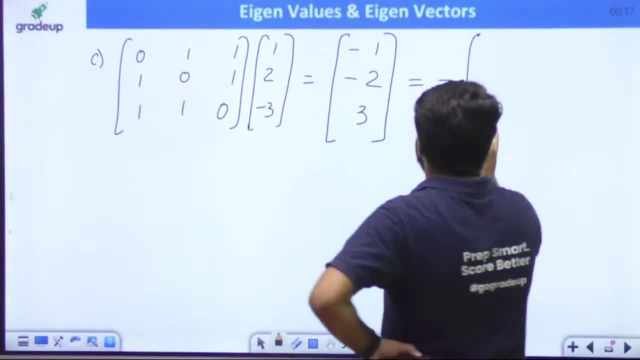 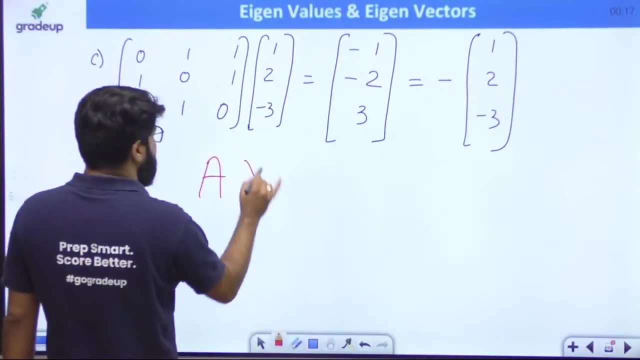 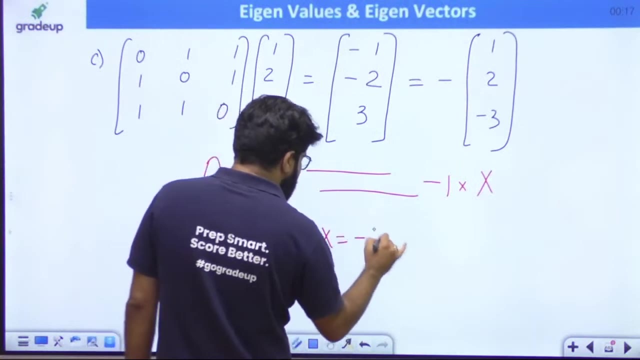 take minus sign outside, I just take minus common and I write down 1, 2 minus 3, which is same as X. Everybody again make a note: a into x is minus 1 into x. right, a into x is minus of x. that means again. 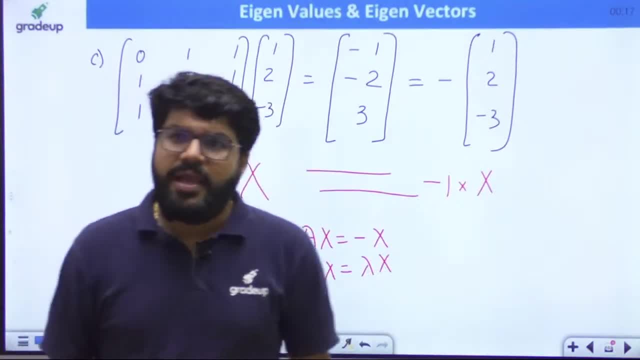 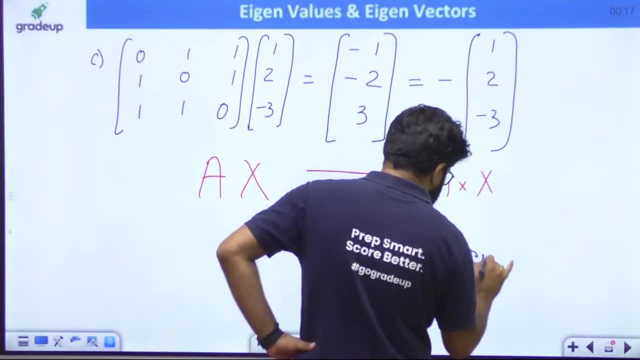 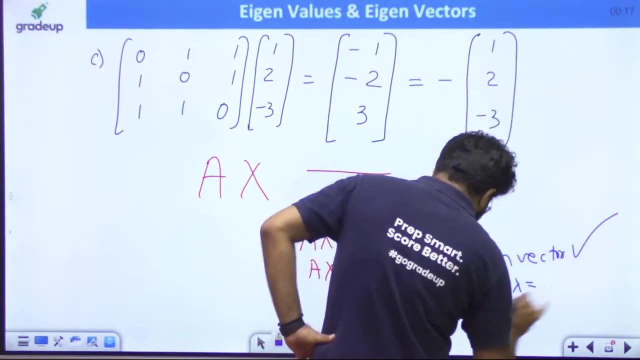 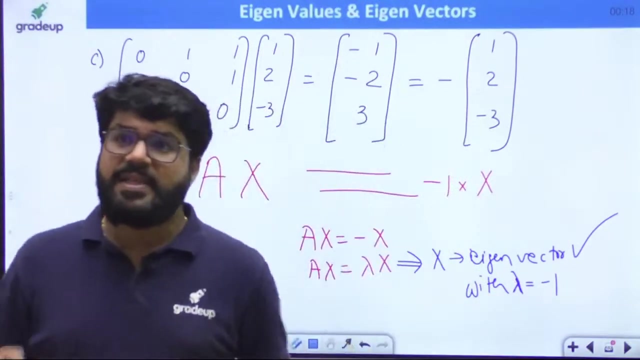 a x equal to lambda negative. b ho sakta hai a x equal to lambda x. a x equal to lambda x. right. so x is an eigenvector, right? with what eigenvalue? with lambda equal to minus 1, with lambda equal to minus 1, x is an eigenvector with lambda equal to minus 1, simple. 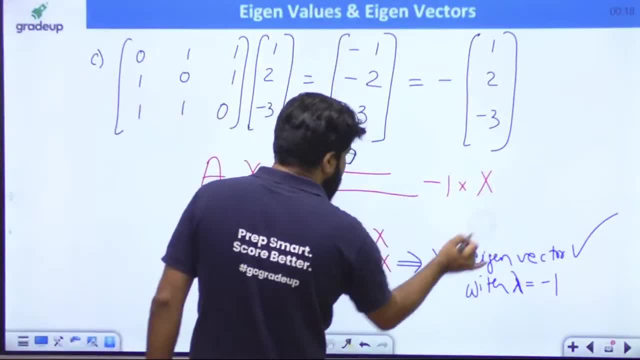 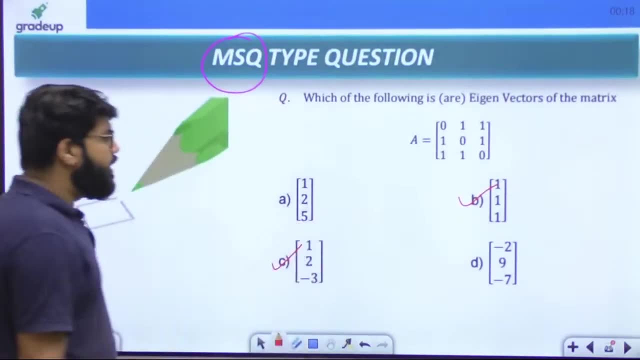 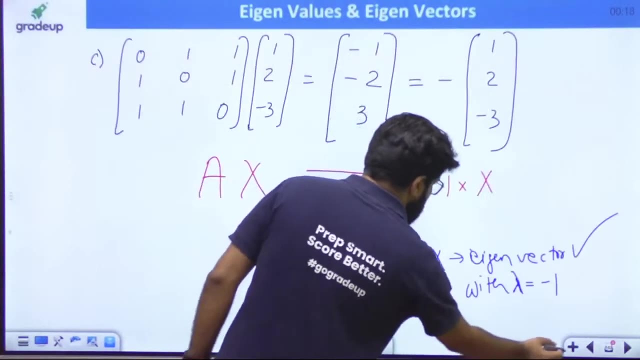 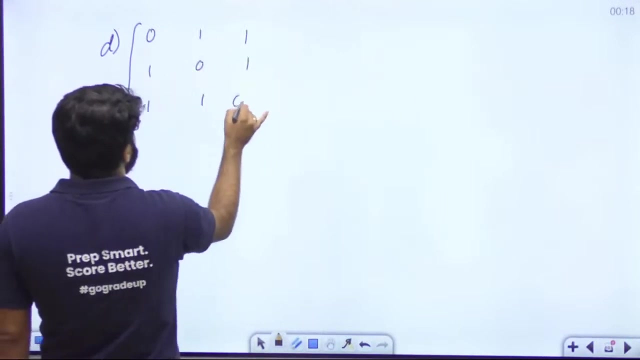 okay, let me mark this option. first of all, c is correct: d minus 2, 9 and minus 7 minus 2, 9 minus 7. option number d: 0 double 1, 1, 0, 1, 1, 1, 0 minus 2, 9 and minus. 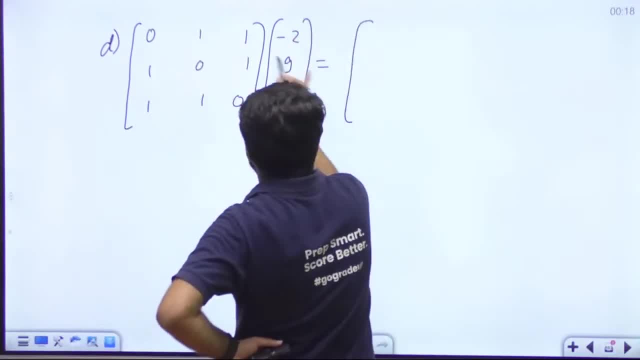 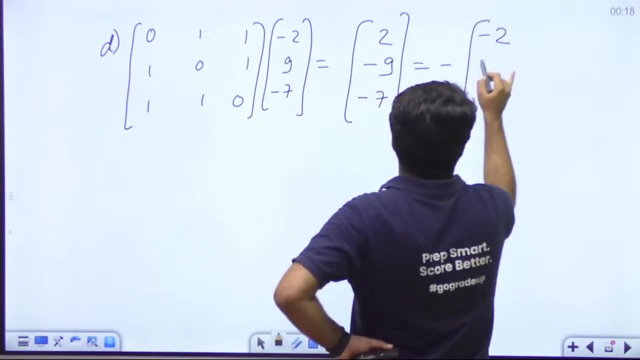 7 is equal to the first row 0, then 9 and minus 7, which are 2 minus 2, 0 minus 7, minus 9 minus 2 and plus 9 minus 7, again again minus outside. so minus 2 plus 9, plus 7 minus 2, 9. 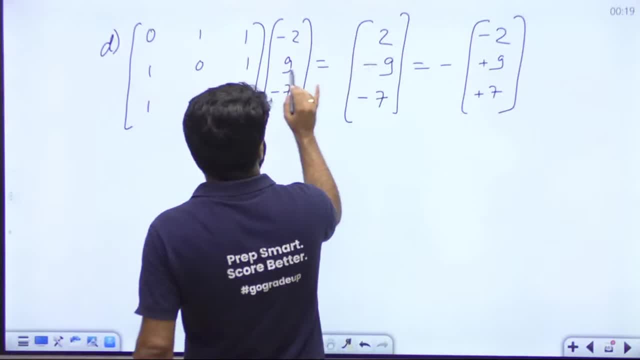 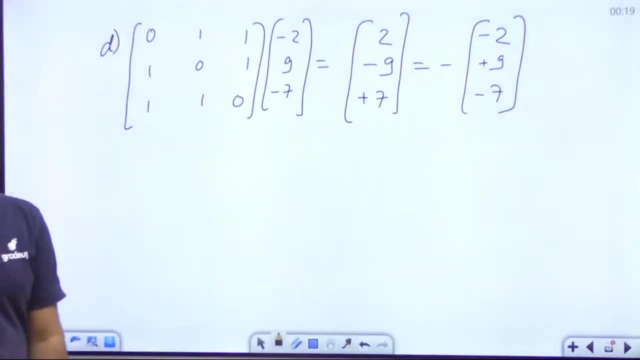 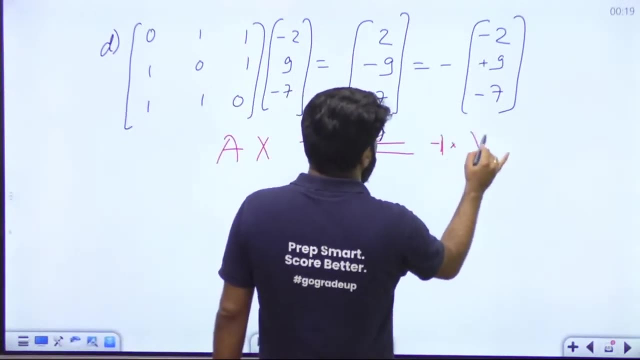 this is 1 minus 2 plus 9. this was plus 7, so here it should be the minus 7, here it should be the minus 7. yes, right, so a into x is again equal to some number minus 1. multiplied by x. a x equal to minus x. 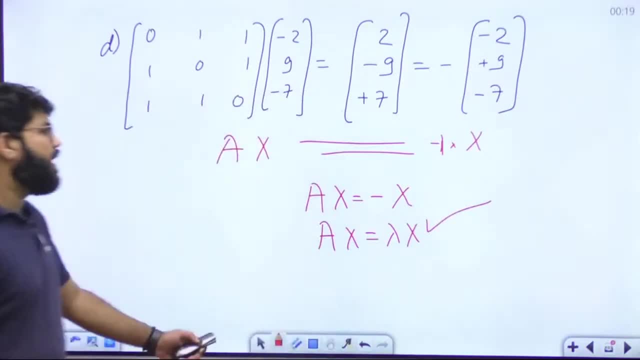 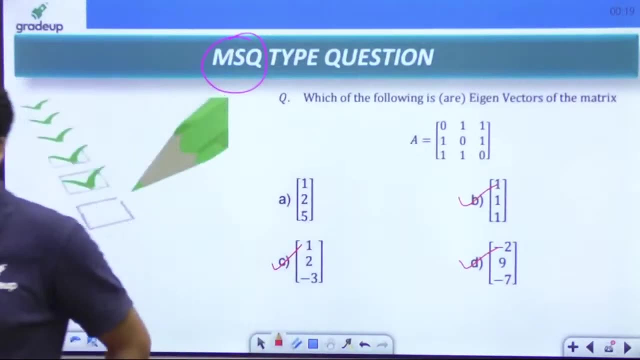 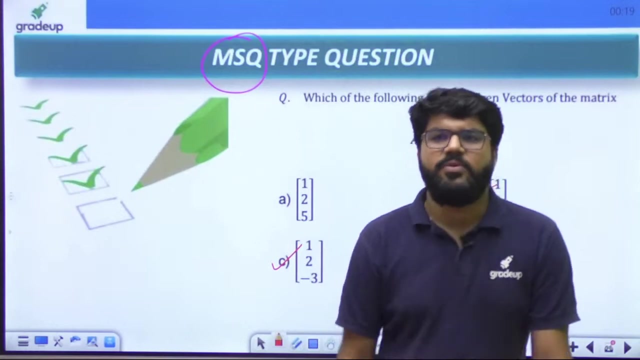 a x equal to lambda x, satisfied. so x is also an eigenvector. so option number d also correct. if it was mcq question, then they can stop here, right? no eigenvectors corresponding to their eigenvalues can never be unique. they can be multiple eigenvalues, right, pragya? yes to hindas minus one is the value of the eigenvalue. 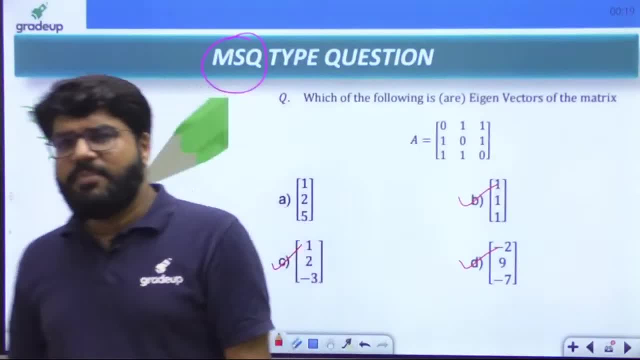 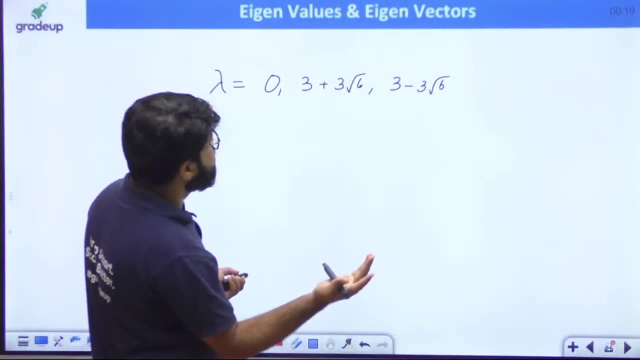 great right. yes, same previously. because chandan. why say that? because chandan, why say that? because chandan, why say that? because name is coming. i will tell you. i will tell you again: up they could get. we solve the eigen k Bangkok. yes, we solve the eigenvalue of the same matrix. now, earlier. 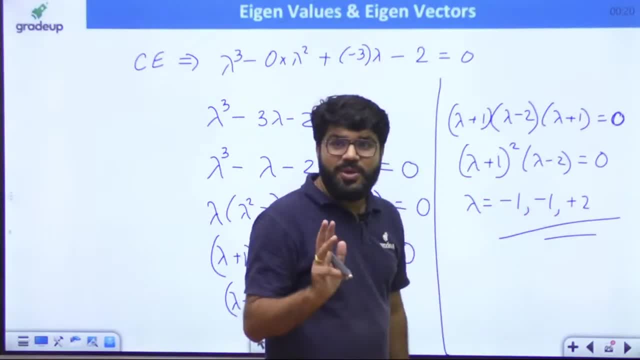 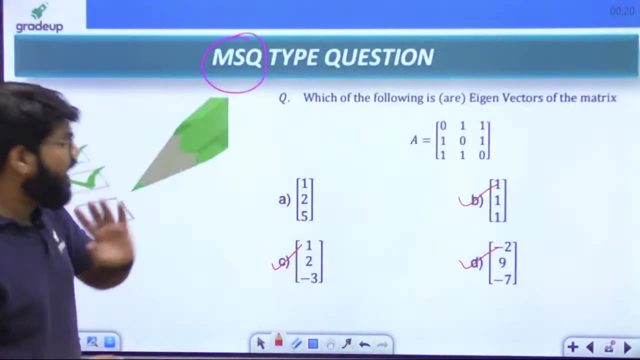 and what were the eigen values? minus 1. minus 1 and plus 2. so actually only two unique eigenvalues are there and minus 1 reputation. go order. they are only two unique eigenvalues. there are only two distinct eigenvalues. so whatever lambda is going to come in this question, whatever lambda is going to come in this, 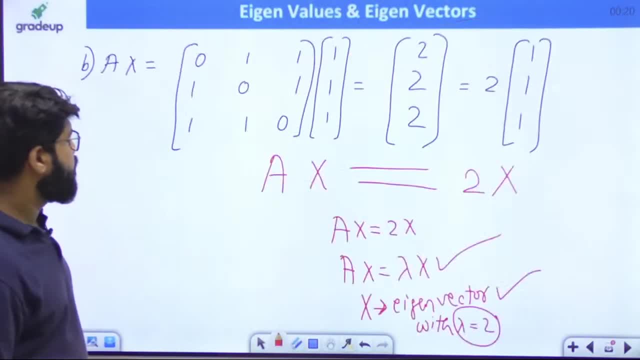 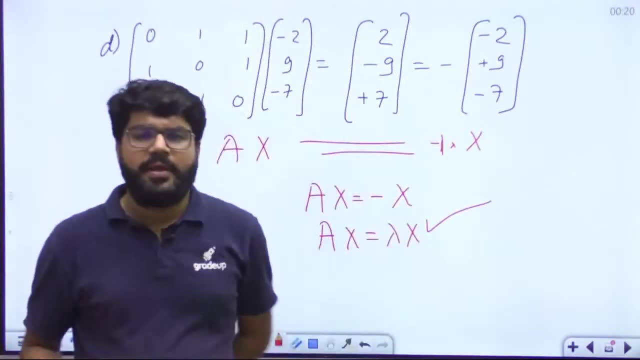 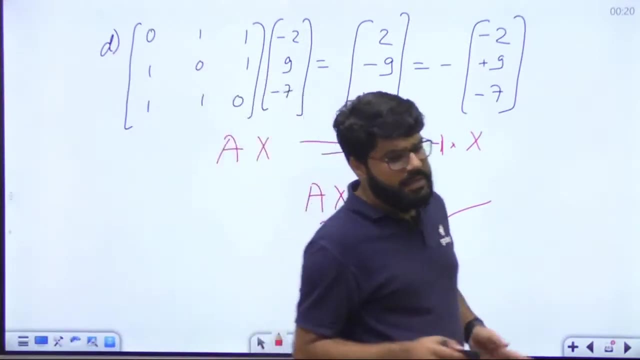 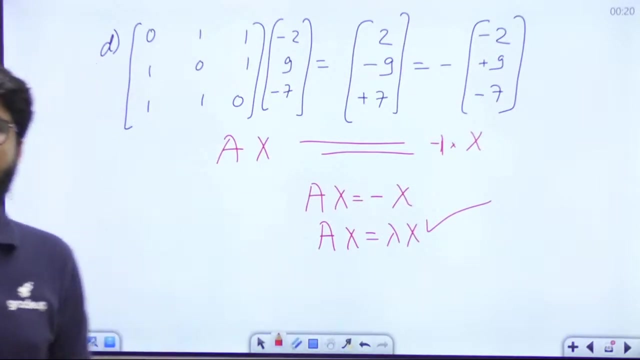 question: it is either 2 or minus 1 here, also minus 1. okay, and Pragya, again I say: eigenvectors corresponding to a single eigenvalue also are not unique. there can be multiple eigenvectors corresponding to a second eigenvalue. okay, all right. all right, that's what? okay, so this is how. now we will take many. 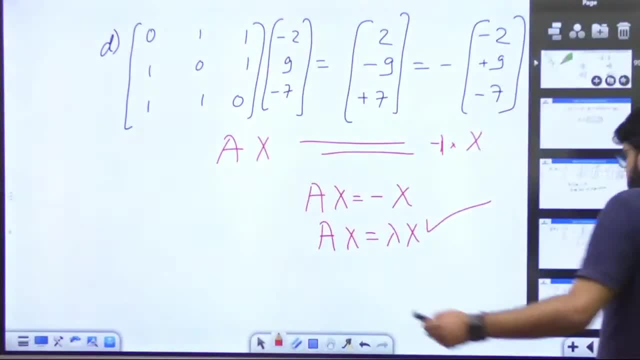 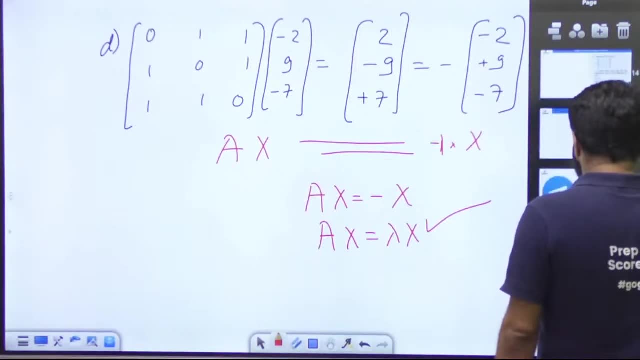 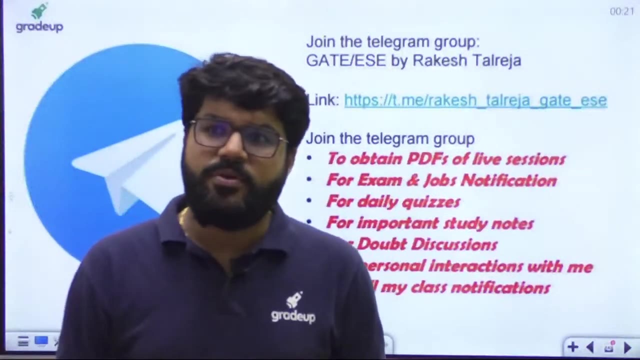 many, many, many, many more questions on eigenvectors. need not worry, or my quiz be up. kills can never allow. so we have taken some basic questions today. we have taken some basic questions today through the tricks, through the simple solutions. okay, and yes, it is. it is mentioned Ashok and it is also. 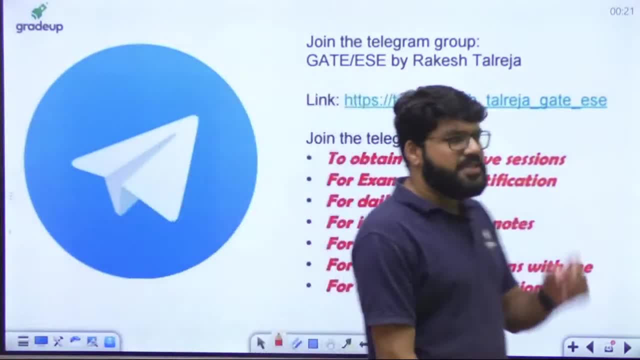 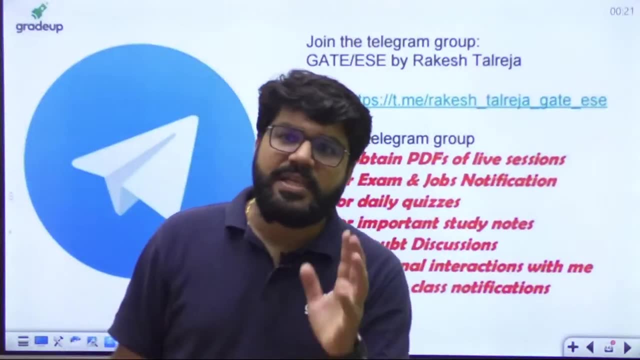 symbol. it is also symboled the the boxes is the symbol of Ashok. okay, okay, Yes, so we'll stop already. Time is today 12.21.. Very enthusiastically, time went away. Okay, went away. Yes, we'll check all the questions of Eigenvector from here. 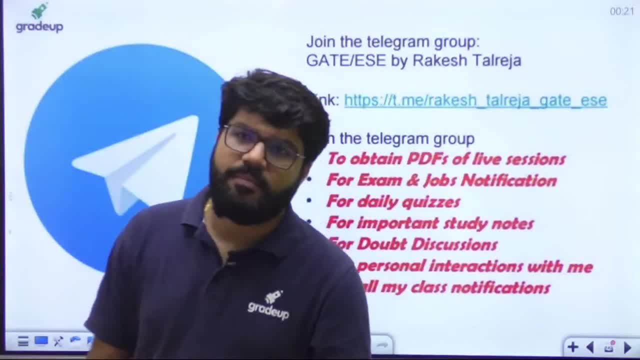 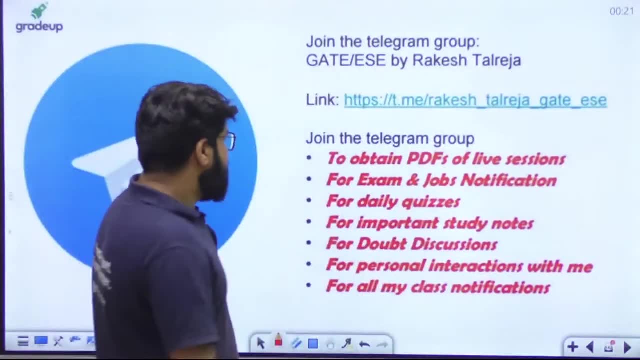 Tomorrow we'll take few more questions of Eigenvector and you're going to take it up. You're going to take it up. Okay, so now PDF will be there in this particular group: Gates slash ESC by Rakesh Talreja. 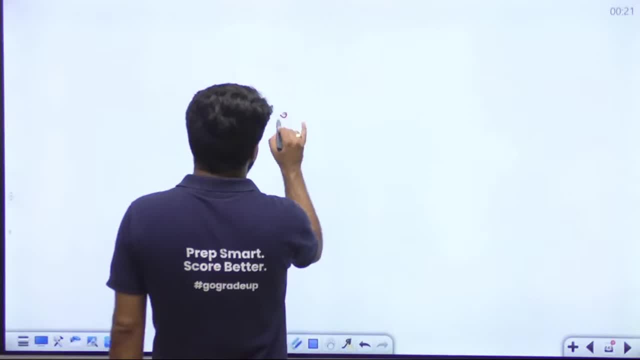 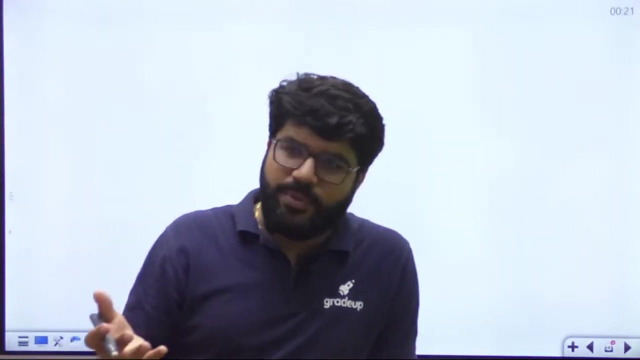 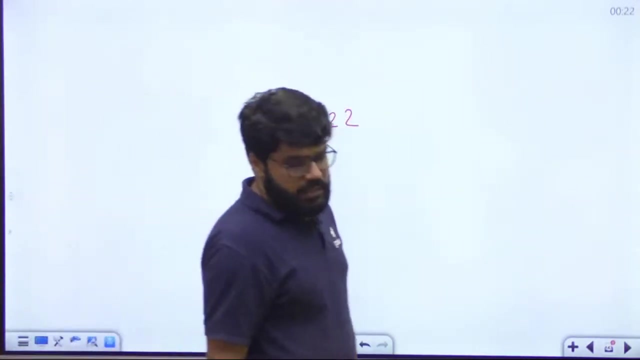 Okay. so, as you also know, As you know, we make the random passwords every day, So today is the random password for today's PDF. That is EV Eigenvalue- EV222.. Okay, EV222.. Without any space, EV222 is the password for today's PDF. 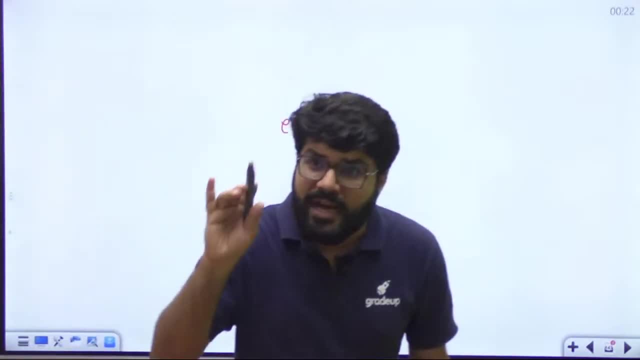 So all those who are live, it's around 12.25 AM. It's going to be 12.30 AM. You're not even knowing, Neither I'm knowing nor you're knowing, But it's going to be 12.30 AM. 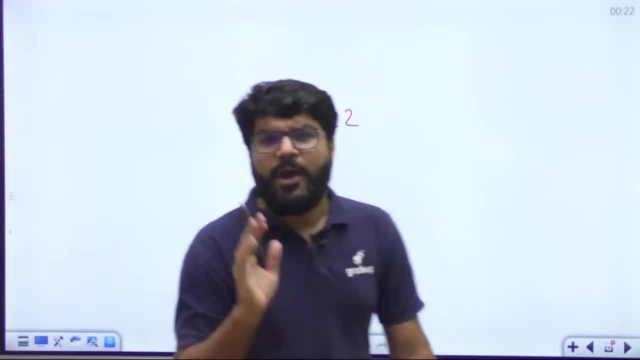 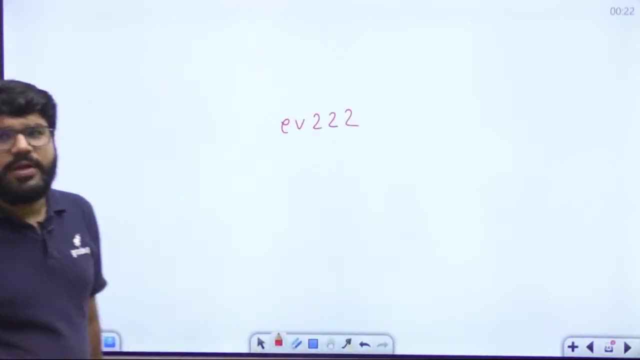 And many of you are enthusiastically live, And that is why I always say PDF is the property of the live student. That should be the personal and private property of the live students. Okay, Okay, so EV222.. And where you'll get the PDF? 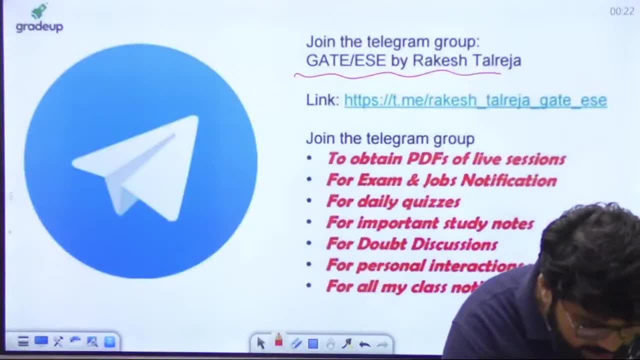 On this group: Gates slash ESC by Rakesh Talreja. I shall share you the link shortly. Those who are not in the Telegram group. Those who are not in this Telegram group, You can join this Telegram group. Okay, you can join this Telegram group. 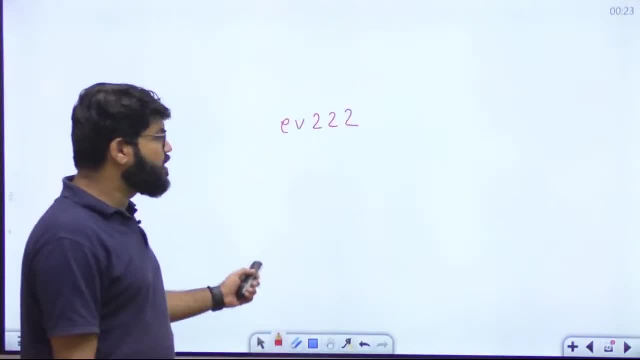 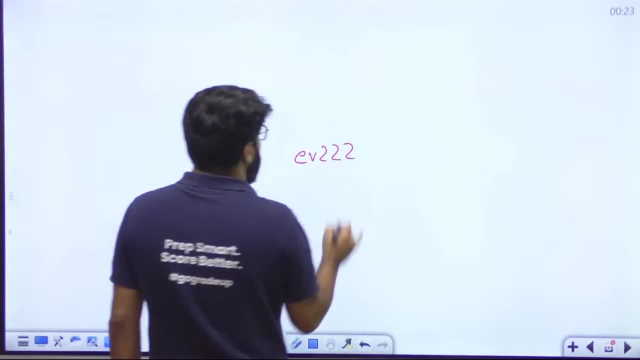 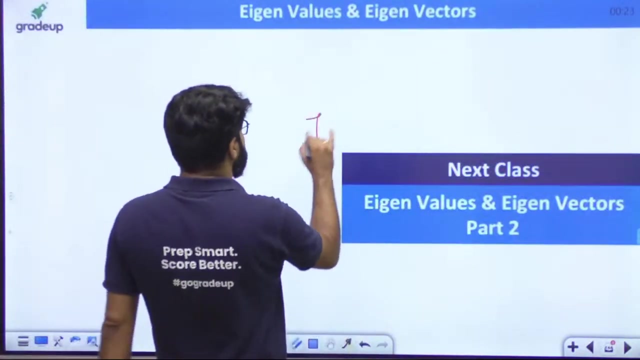 The link of the Telegram I have shared. You can join the Telegram group. The password is again, I repeat, EV222.. Without any space, EV222 will be the password of the PDF on this Telegram channel. The next class: Eigenvalues and Eigenvectors. as again tomorrow. 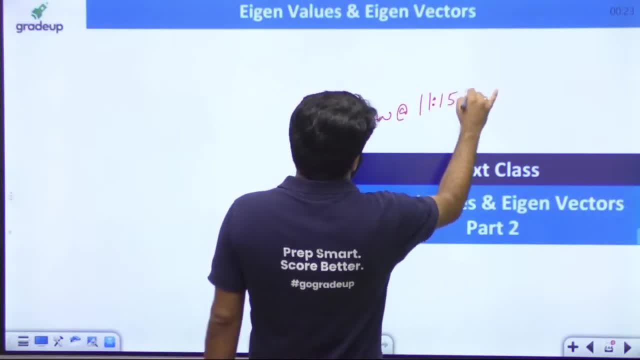 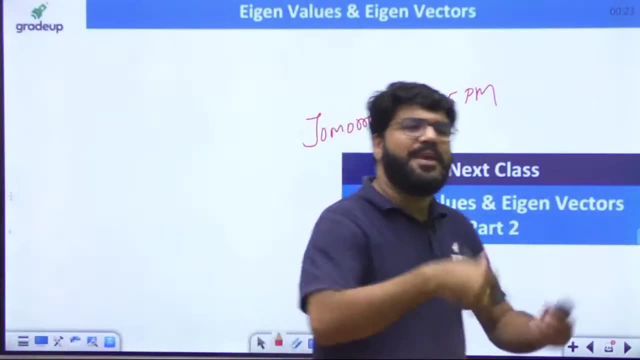 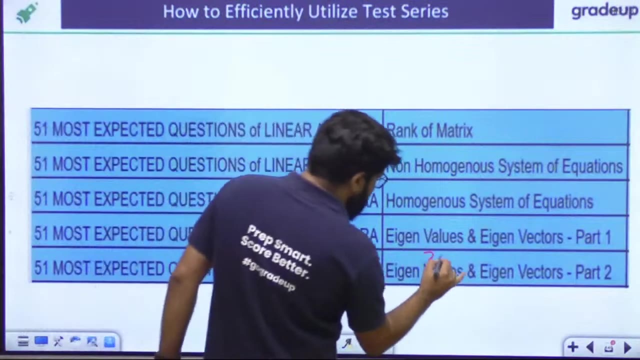 Same time: 11.15 PM Tomorrow. actually today Date changes, We end it, Date changes. But yeah, obviously we call it as tomorrow, 11.15 PM. Right, So that is the last class. Okay, but I am adding: 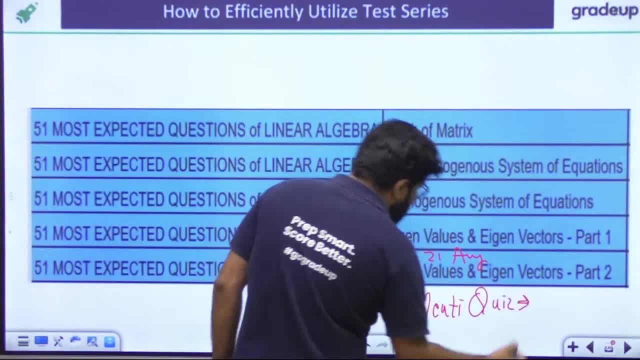 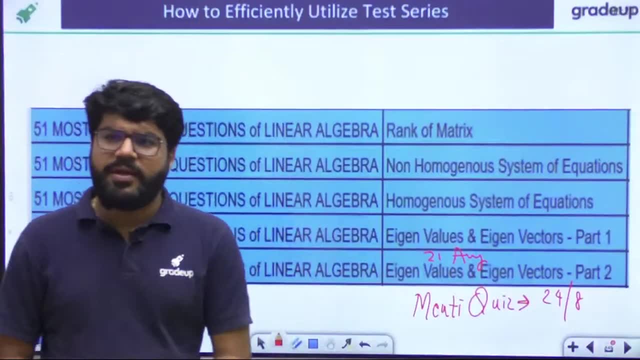 As per your interest, I am adding a mentee quiz. I will tell The date soon. most probably 24 August, most probably 24th of August. I will tell you the date of the mentee quiz very soon. Okay, I shall tell you the date of the mentee quiz very soon.